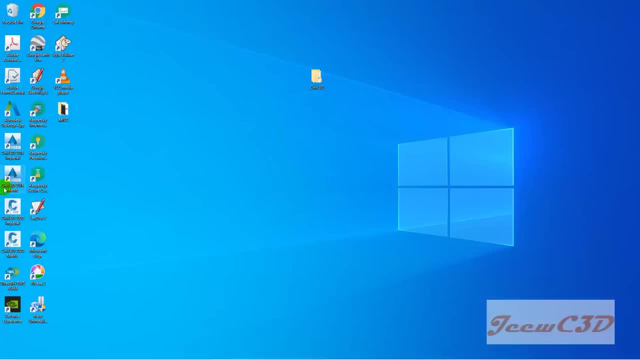 I want you to double click this CivilTrader 2016 in your case, whichever the version you use- CivilTrader 2016 or CivilTrader 2018.. But I want you to click on the metric version. that is the version we use for in our work. 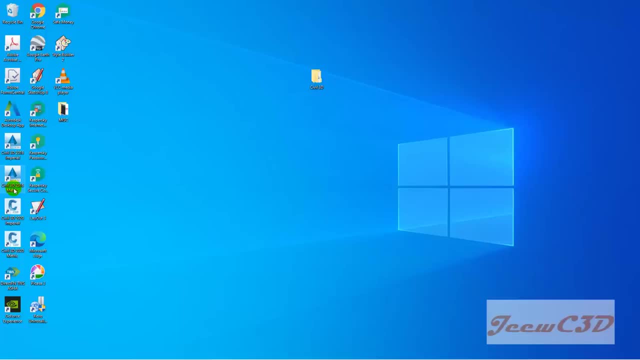 Metric version is using the units as meters, So that is the units we are using in Sri Lanka, So that is why we are using the metric version. I want you to select this CivilTrader metric version shortcut icon and double click to open that. 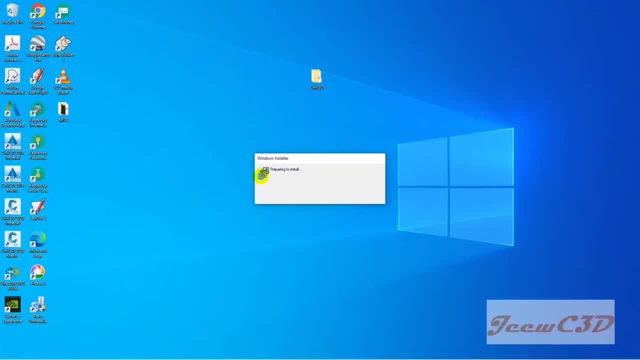 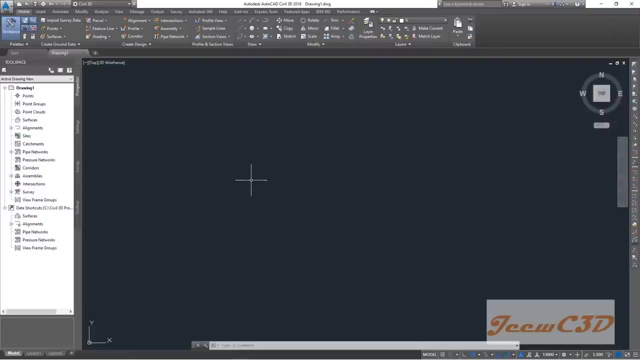 So you can see that my CivilTrader software has turned on. after some time it will be loaded. Now you can see my CivilTrader software has turned on. This is the basic interface of CivilTrader software, So depending on your version, you may see some kind of small differences. 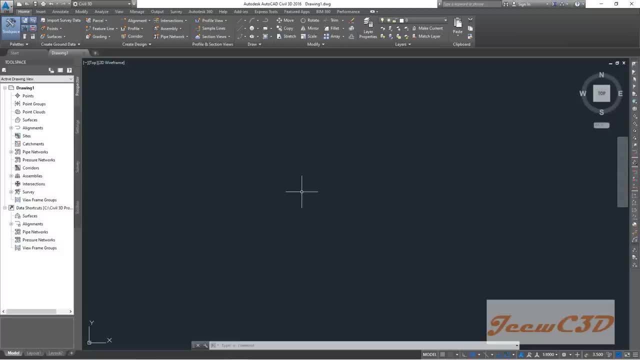 in the basic interface, But more or less this is the interface that we are going to use for our CivilTrader software. So this is the interface that we are going to use for our CivilTrader software. This is the interface that we are going to use for our CivilTrader software. 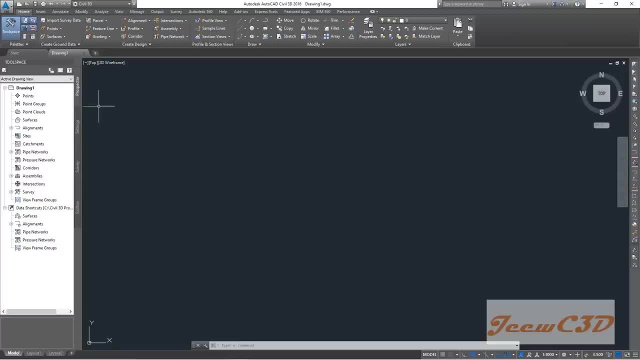 And now, like you see, my series is same, So you will be seeing that you may have something called drawing one. I will now explain about the interface of CivilTrader. In the top left corner you have something called application menu browser. Once you click this button, you will see there are some kinds of icons appearing on the tape. 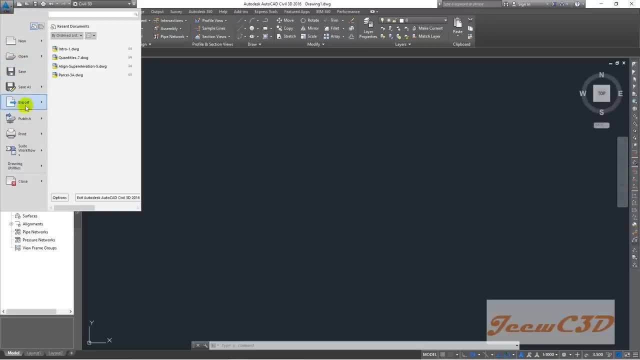 It is like only the mouse click and it will automatically load automatically normalised 인데요ывать on the up side, But of course for that the interface is same window. so these are same as Microsoft Office or Excel. so by this you can open a new drawing. 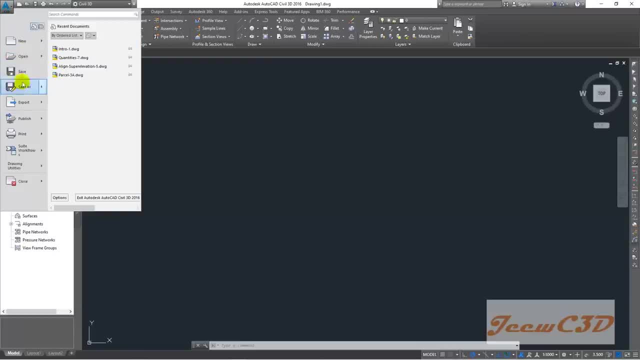 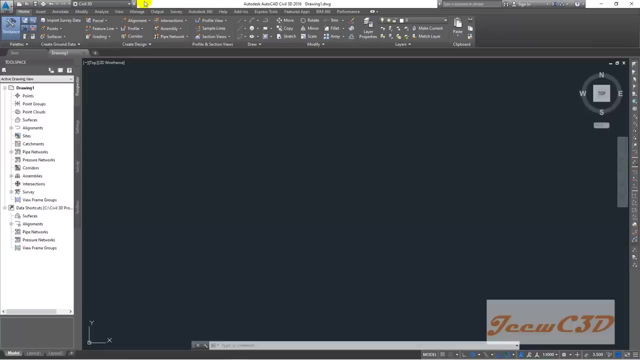 by this you can open an existing drawing. here you can do save, save as and some other functions. so if you have problems with any commands, you can type here and get details of that. so that is about application menu browser. then here you have something called workspace. 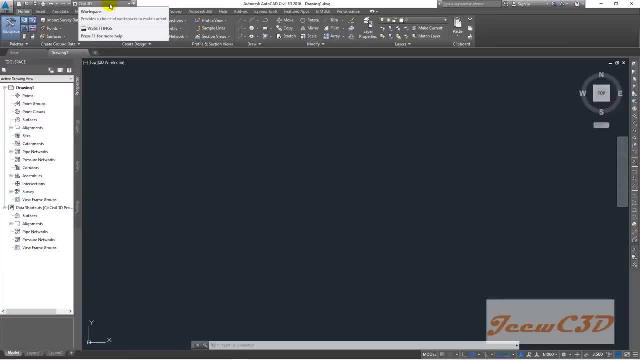 when you place the cursor here, it will be highlighting what it is so here. this is the workspace. there are several workspace. once you click on here, you will see there are four workspaces here, but what we are doing is civil 3d workspace. then you have some quick access. 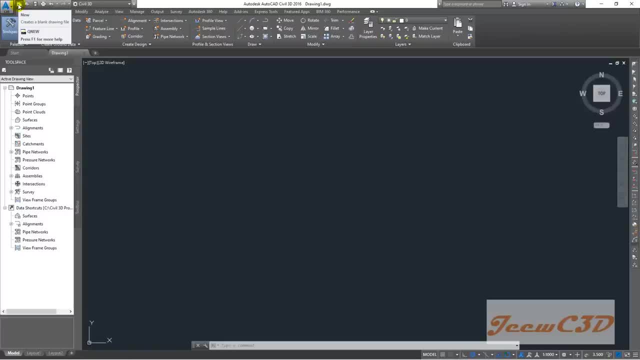 toolbar buttons here. here you can create a new drawing, you can open a drawing, you can save, you can print or plot, you can do or undo and redo- things like that. you see these kind of things in word excel too, so I think you may be familiar with these things. then here you have the tabs. 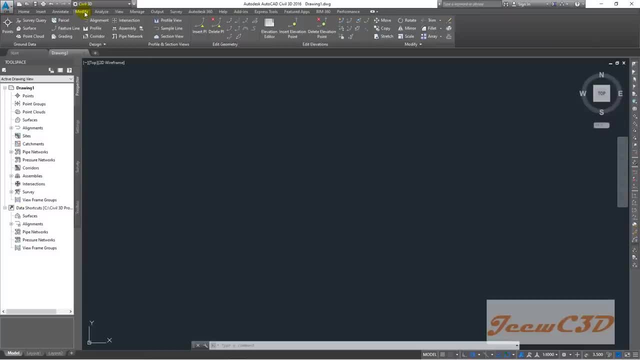 form tab: insert tab, annotate tab, modify tab likewise. so most of the things we do are the same thing, but in the form tab of civil 3d interface. so inside this interface you have something called panels. so this is palette panel. you can see it is. it has a border from. 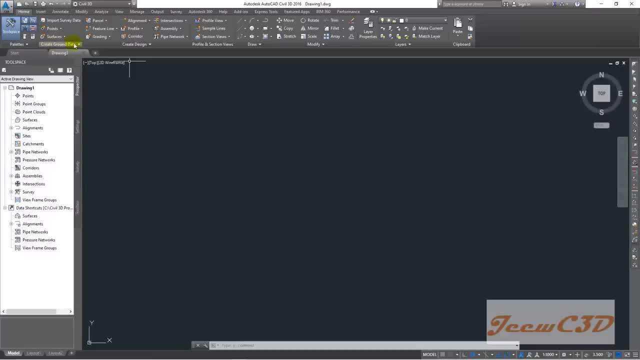 from the others. this is palette panel, this is create ground data panel. so inside these panels you have some other options. this is point drop down, then this is surfaces drop down. likewise, you have create design panel. in that create design panel, you have some kind of data. then you have 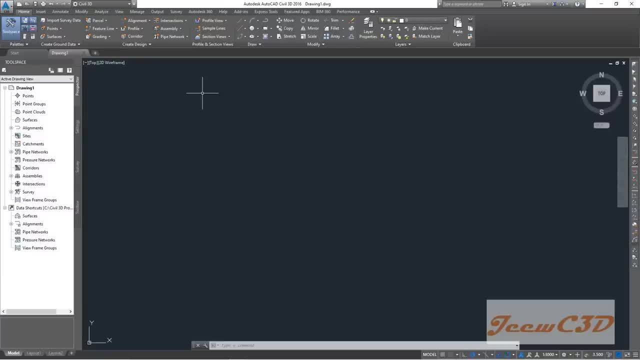 profile and section view panel. so each of these panel have specific civil 3d data. in other tabs also, you have separate panels. here you have import panel, infraworks 360 panel, block panel likewise. so i move back onto my home tab. then this one is called the tool space. this is where you have all the tools and data stored in. 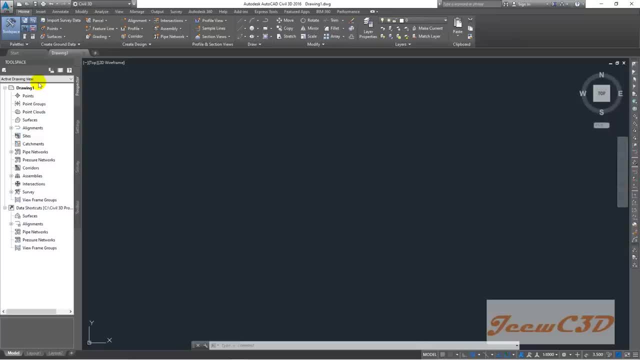 civil 3d you can access all the stored data and settings in this tool space. in tool space you have four tabs: prospector settings, survey and toolbox. in prospector tab you have all the data. inside. you can view all the data within the civil 3d drawing. 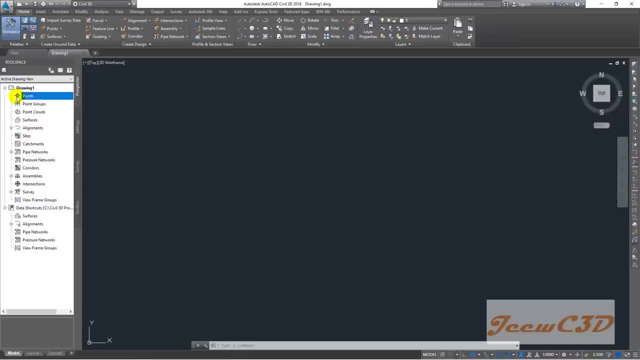 through here. so if you have a have point data, it will be showing here. you have point data. so if you have alignment, it will be showing that you have alignment here. so i will show you once we go forward with the lectures. then you have the settings tab. it has all the settings that we need. 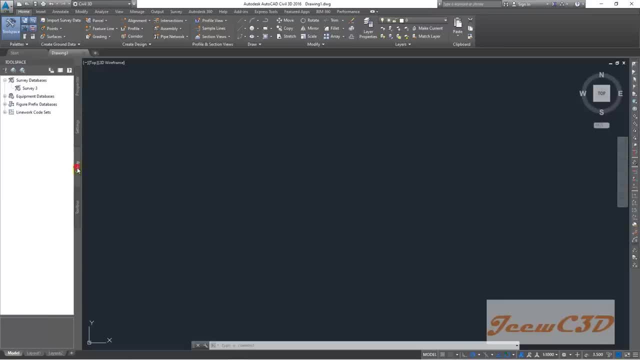 to do work with civil 3d software. then you have the survey tab. that will be useful for the surveyors, not uh much useful for engineers. then you have the toolbox tab. here you can use the report manager to create output reports from civil 3d drawings. so i moved up to prospector tab. here we work. 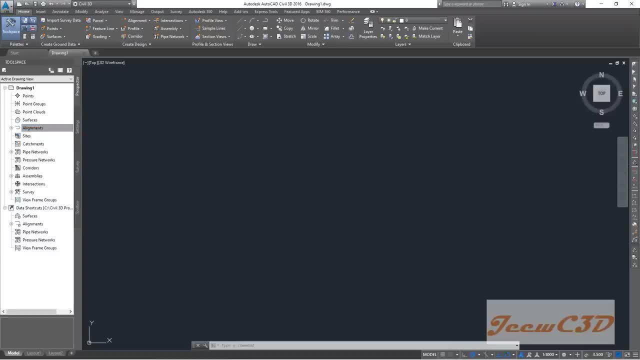 so much in civil 3d. so if you couldn't find any of these tabs, you can turn it on or off through these buttons. if you click this button, your prospector would be gone. so if you click this again, your prospector will be appearing. so if you click this button, your 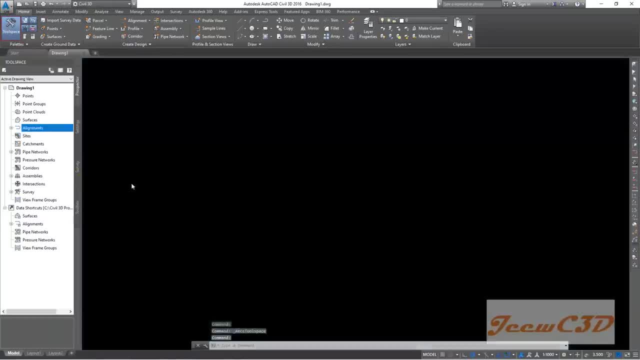 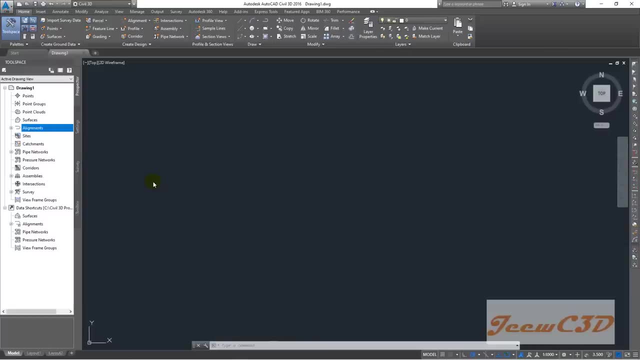 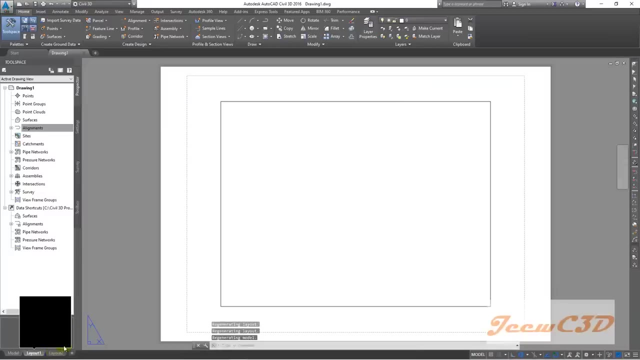 tool space would be gone. so once you click it again it will be appearing. so if you lose that, lose the tool space, that is how to get it back. then you have model tab where we work. then you have to layout tabs so they will be used to get the output drawings. but we are not going to 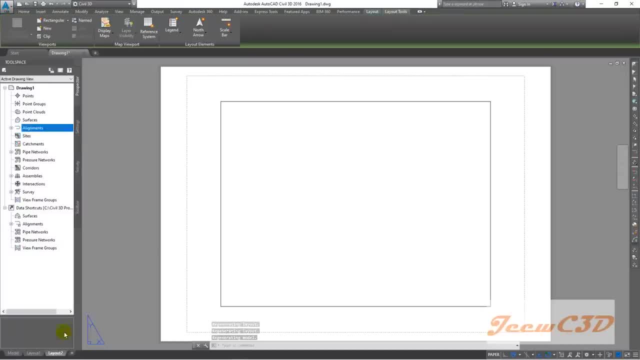 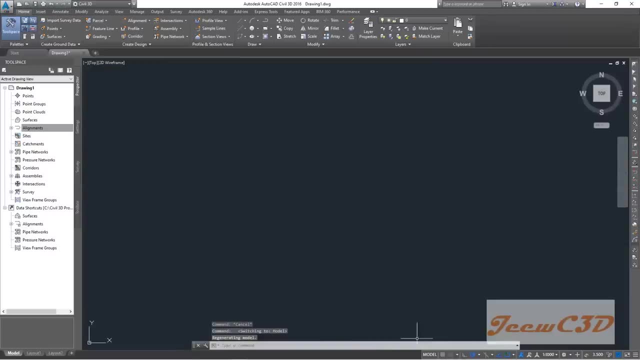 learn them inside this course. We are mainly working in the model space. Then you have the command bar where you type all the commands. So if you are familiar with AutoCAD, that is same as Civil 3D. So you have to type the commands here and you can do whatever the 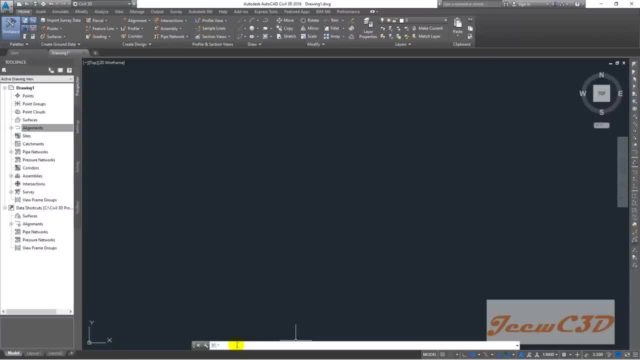 thing you want to do in Civil 3D, same as AutoCAD, For example, if you want to draw a line, you type line here in the command bar, so it will give you the line command once you press enter. then you can create a line like this, So this: 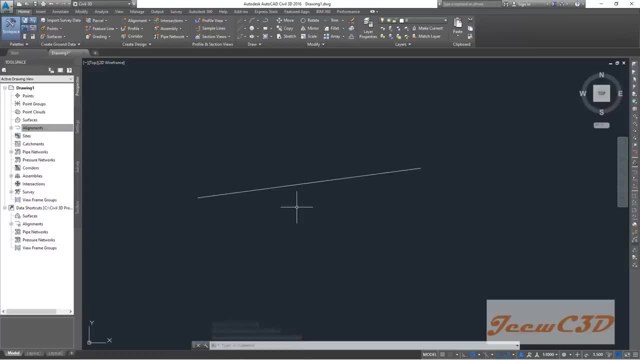 is a simple line which is an AutoCAD entity. So there is a difference between Autocad normal or pumpkin normal. So this is an Autocad entity. Why this is talked about It is to understand that both AutoCAD and civil 3d the major difference is civil 3d is a more intelligent software. 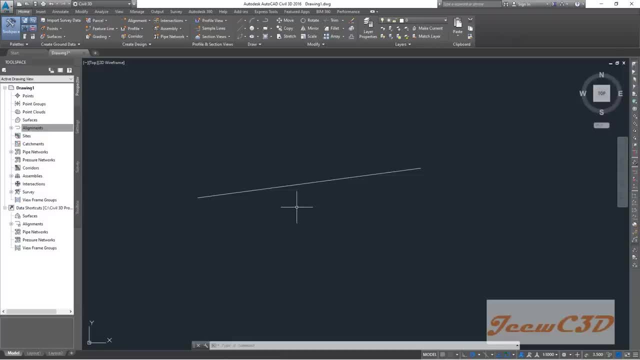 civil 3d has intelligent objects. once we go through the lectures i will show you. it can change according to the situation once we change the parameters. but AutoCAD cannot do that. civil 3d can do that. that is why we call civil 3d a intelligent software. in here you have. 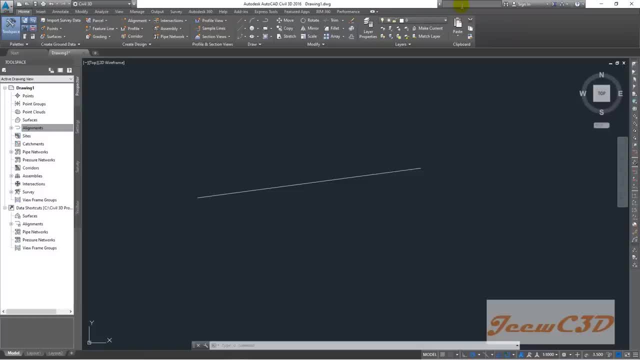 the help section. you can get help from anything you want related to civil 3d or AutoCAD from here. then again, you can sign in if you have a. if you have, when you want to log to the online account, you can sign in from. so also, you can use the online map for this function after signing in, so that 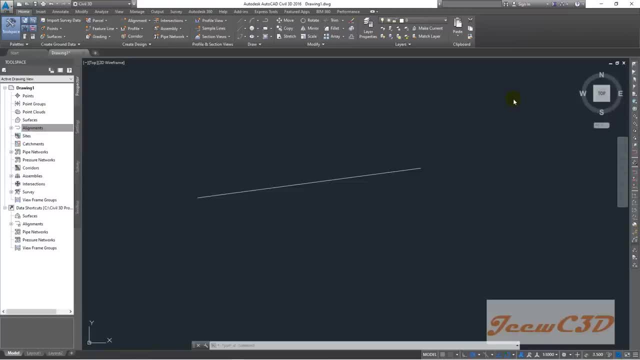 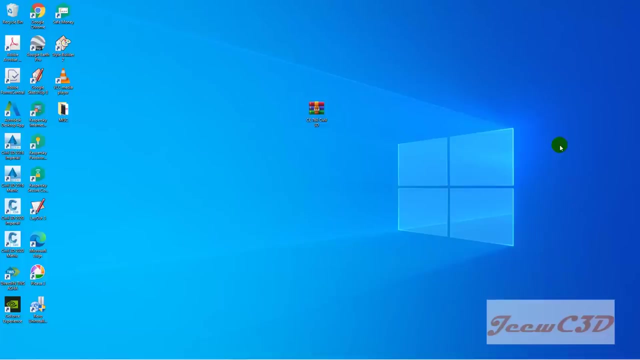 is about a basic introduction about civil 3d, then in the next video we will learn how to set up civil 3d interface to work with civil 3d. from here onwards you in this video, we will be starting a new drawing and synchronize the civil 3d. 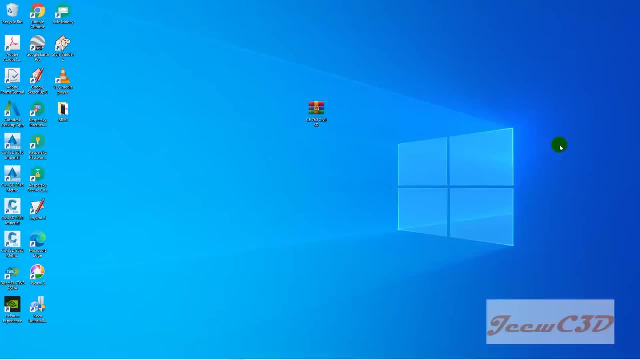 interface, with my interface and your interface, and making both our interface identical so that you will not be getting much problems by the interface, and making both our interface identical so that you will not be getting much problems by the thing with the civil 3d videos. so before that, I have send you an email. 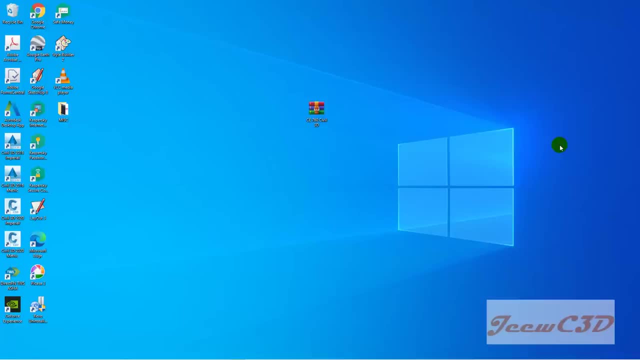 related regarding the data we need to use in this civil 3d lecture series. so you may have received something like this: CE760- civil 3d. it is a RAR file, or in other words, a zip file. first you need to copy this to a. 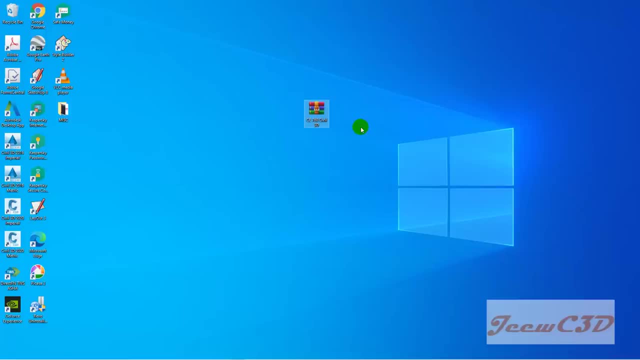 place where you can easily access. I have copied mine to the desktop. then you have to extract this using something like extract here, so you will be having this folder. after extracting, then you have to open the civil 3d software, the metric version. if you have already done that, you don't need to do that. 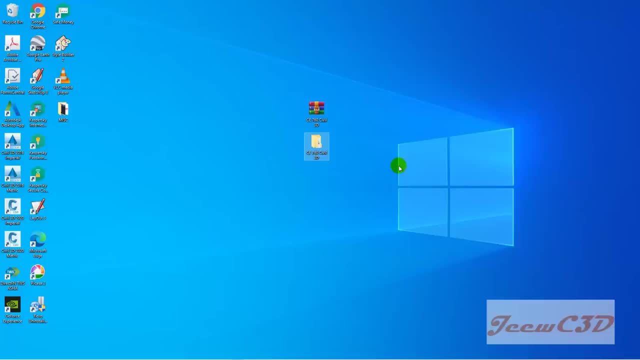 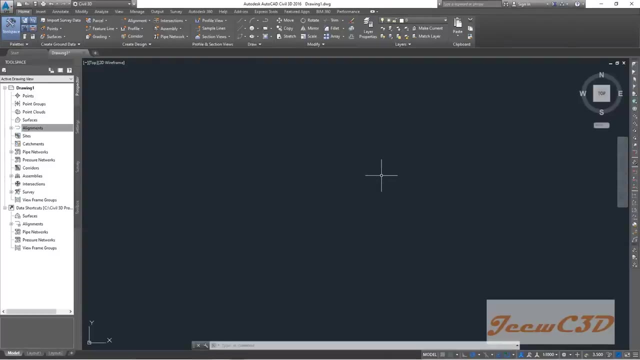 you don't need to open it at the end, you just go into the civil 3d version. now I am going to open a new drawing using a template. so a template means a drawing where all the standards and settings are stored to do our drawing so in 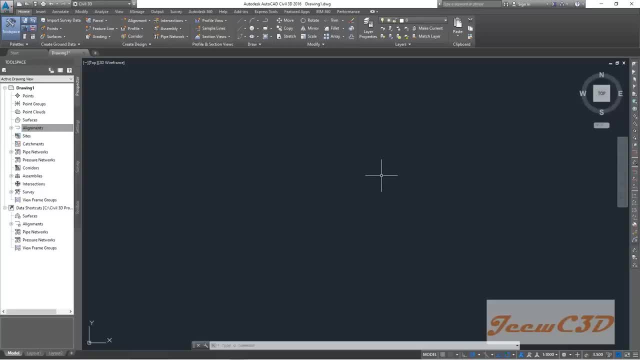 your company are working in a company, they may have a civil 3d template where you can use for your civil 3d works. so various companies have various drawing templates to do with their civil 3d work. so so now i am going to start a new drawing with a new template. so what you have to do now is 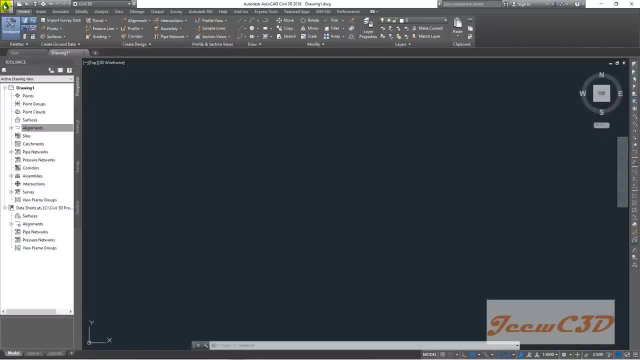 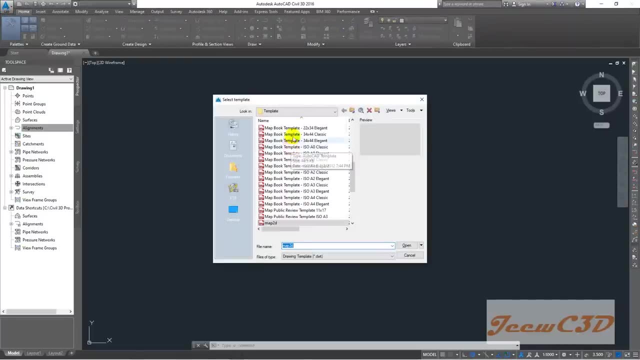 you go to the application menu browser, you click here and then go to new. then i want you to browse to the file where i gave you that is the ce3760 data folder. so that is in my desktop. i am moving here and i go into the template. so the ce7c. 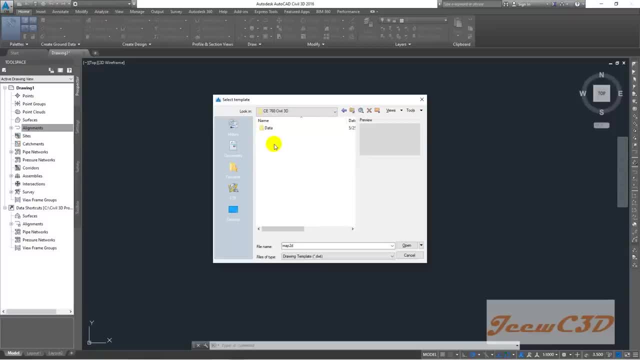 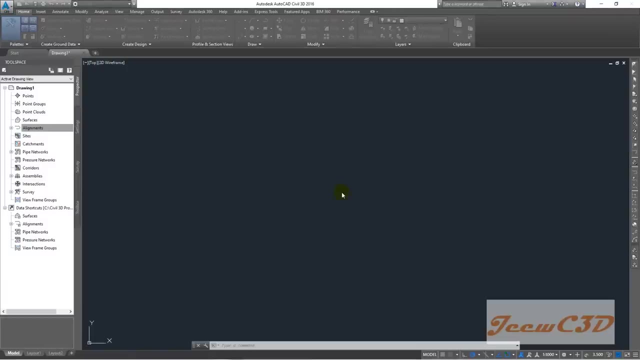 0, 7, 3d folder. so inside that you have data folder. in that data folder you have something called new road template, something is a file called new road template. so you have to open that file. so every time you start a new drawing you have to use a new template file you can use. 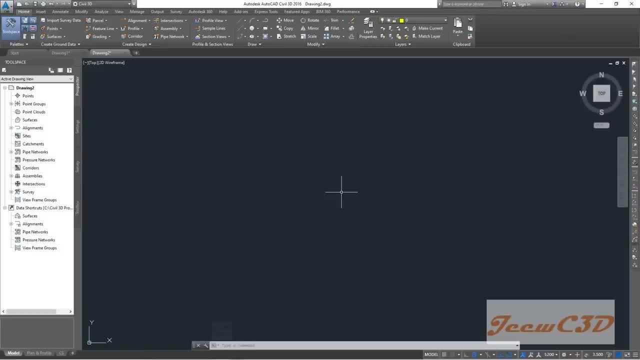 existing template file. anyway, you have to use a template file. so I have opened this drawing tool with the new wrote template file. so I will close this drawing one and click this assign and no to save changes. so, guys, nothing will be saved. now my drawing tool is open, is open using the new wrote template. now what I 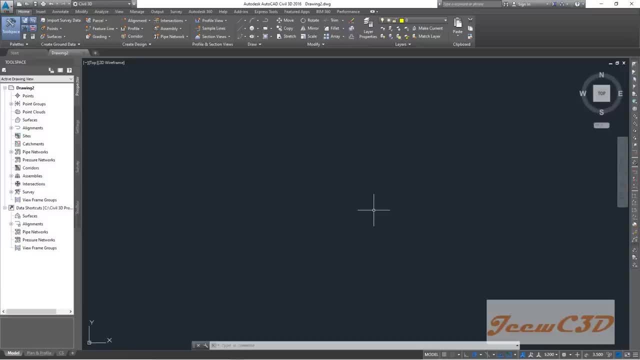 am going to do is I am creating some settings, for I am making some settings so that my silly 3d interface and your sample is not affected by the new template and you can use the new template. now I am going to do is I am creating some settings, or I am making some settings so that my silly 3d interface and your 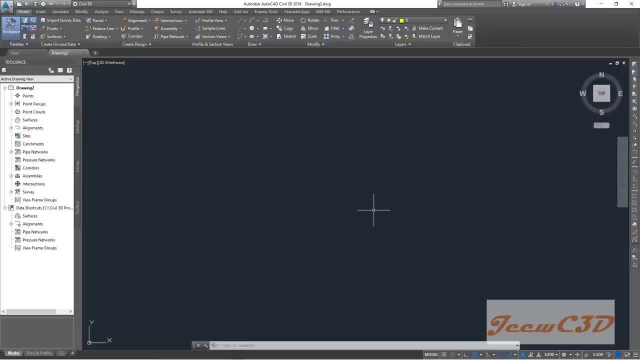 3d interface become identical. so here, what i want is: i want to press your shift key on your keyboard. press your shift key on your keyboard, then right click, click your mouse button. right click the mouse button shift key plus right click, then you got osnap settings. 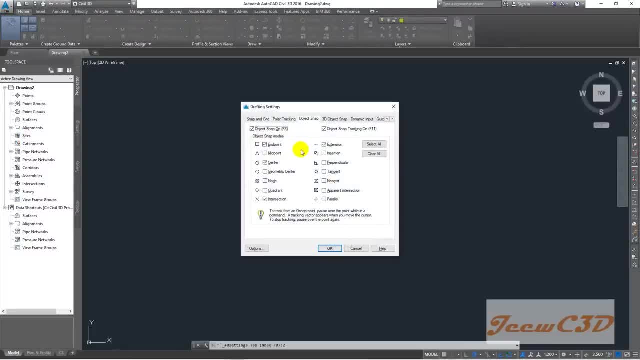 click here. then you will get something like this: you then uncheck this option, osnap on. uncheck this one, then osnap cracking this one also uncheck. then you move on to this snap and grid should be unchecked. polar cracking should be unchecked. object snap will be already unchecked. it is okay to have these things checked. 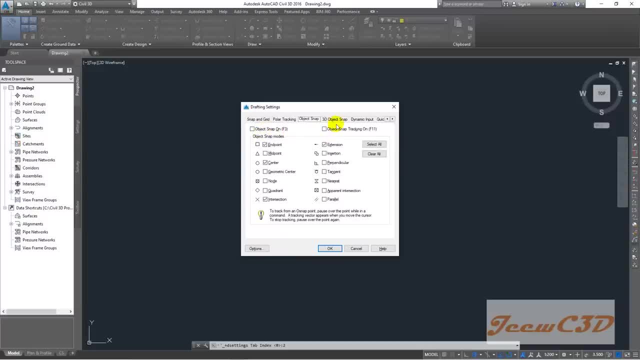 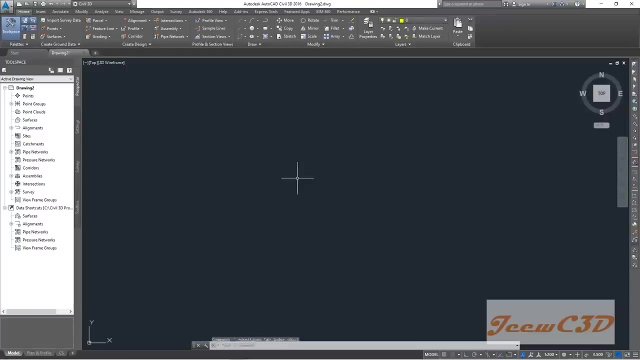 but main thing is to uncheck these two things in 3d object: snap: make sure it is also unchecked. dynamic input: make sure this is this one is okay to have, but there's another settings to be changed. i will tell you next. so after setting all those things, you click ok. 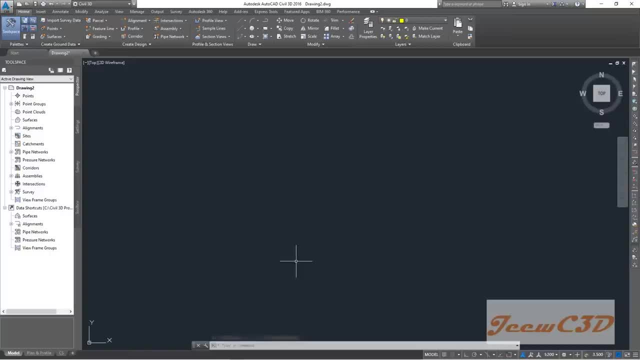 now you just type some commands. you put your mouse cursor here somewhere in the middle, then you type some commands. so if your commands are typing on the command bar, that means your dynamic inputs are turned off. so to ensure that or to change the dynamic input mode, you have to press f12 on your keyboard. so the modern, modern laptops- you have to find f12 key by pressing function or fn key plus f12. so make sure that what kind of keys are to be pressed to get the f12 key on your keyboard? in my laptop i have to press function key plus f12. so 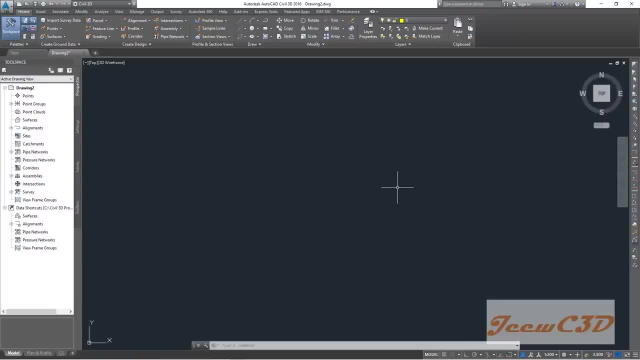 in your laptop or computer. just make sure what are the keys to type to get the f12 function. So what I am going to do is I am pressing F2L on my keyboard so nothing will be happen. but when you type you will see the typing is happening here. the cursor is there. so 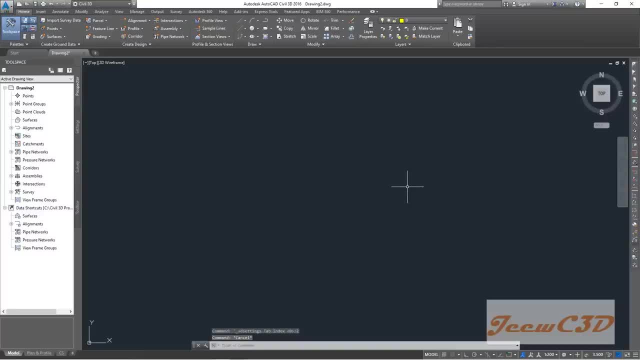 if you press F2L again, you will see the typing is happening on the command bar. so I want the typing to be happen on the command bar. that means your F2L should be turned off or the dynamic inputs should be turned off. now, that is the main options. what we have to be. 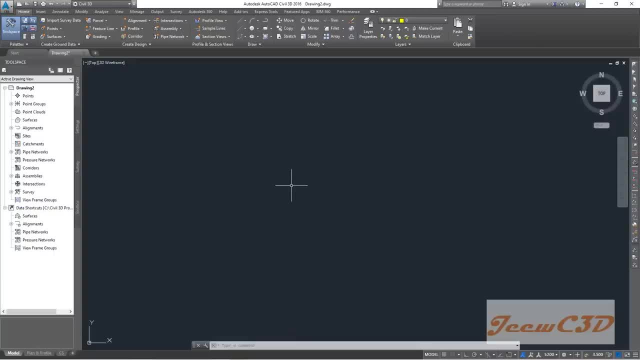 set to synchronize my screen with your screen in terms of Civil 3D. So I am going to press F2L on my keyboard so nothing will be happen. but when you press F2L again, you will see the typing is happening on the command bar. that means your F2L should. 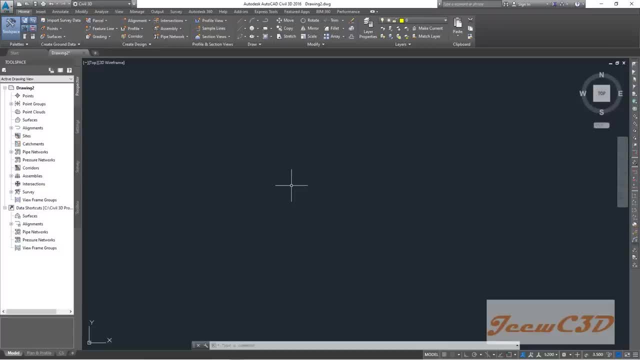 be turned off or the dynamic inputs should be turned off. now, that is the main options. what we have to be set to synchronize my screen with your screen in terms of Civil 3D. You don't have to save the drawing in this moment, but keep the drawing open in the 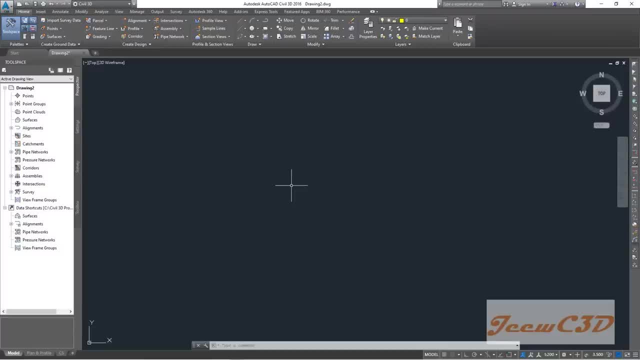 next video I will tell you how to start a project with Civil 3D for your design. Then you have selected the site for your design, what you do at the first. So, once you have finalised the trial, alignments and everything, as I told you in highway design, 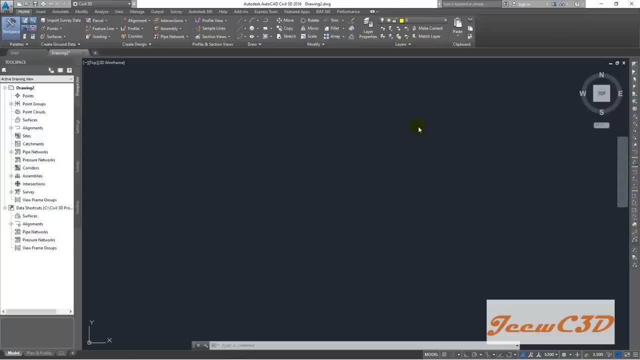 lectures. what you do is you are going to survey that area. a surveyor will be going to that site and he or she will be surveying in that area. we call it doing a TODO survey, we call it doing a TOBO survey. 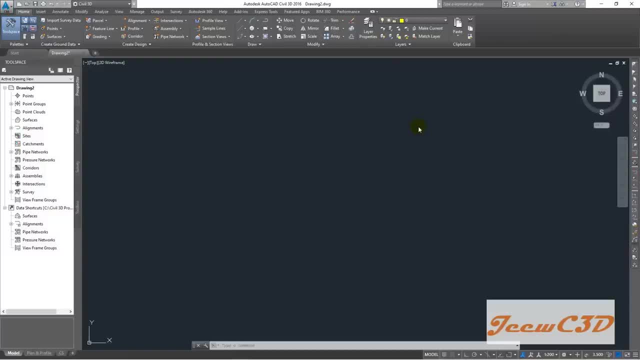 get the features in that area as well as the elevations in by the means of points. so the surveyor goes there and taking elevations as points and also he is taking the objects or features in that area. so the surveyor will give you us the point file where we have the elevations. then we can use that. 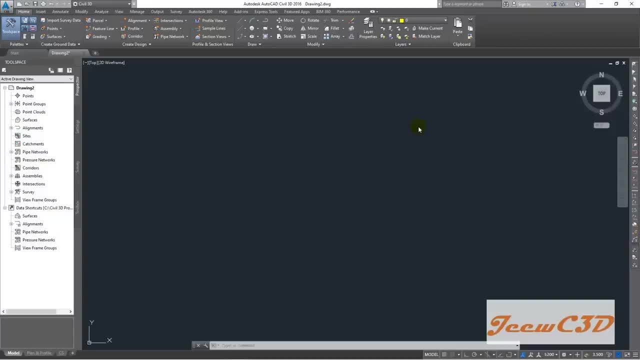 elevations to create a civil 3d model. the points will be used to create the civil 3d model, what we called a surface, that is, the ground surface of that area where the surveyor has surveyed. so on that ground we will be creating a. 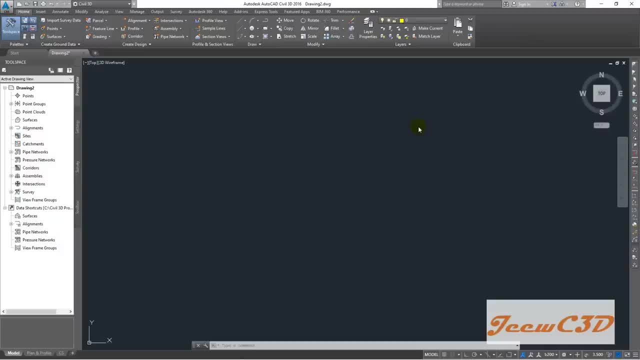 so I hope all of you have this drawing open by now, without closing, from the previous video. so this drawing is open using the new road template, which I has have done in the earlier video. so now what I am going to do is import points into this drawing. so to do that you have to go to home tab. then you have 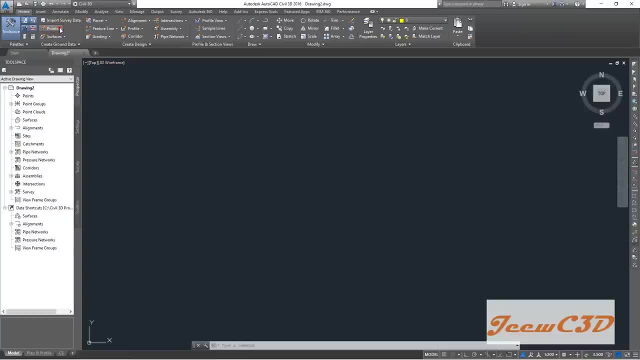 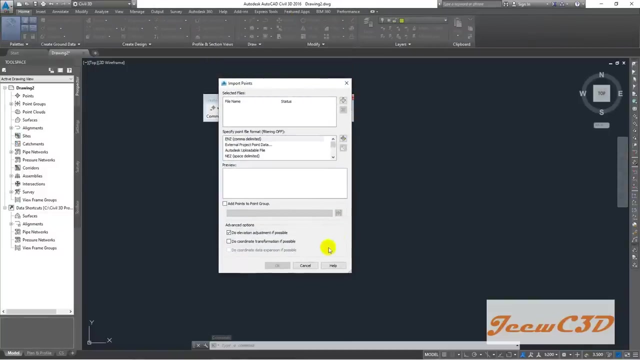 a something called points. here you click this drop-down, you go to point creation tools, then small bar will be appearing. you can drag it here. then you click this button, import points button- then another small window will be appearing. that is import points window. then here you can select. 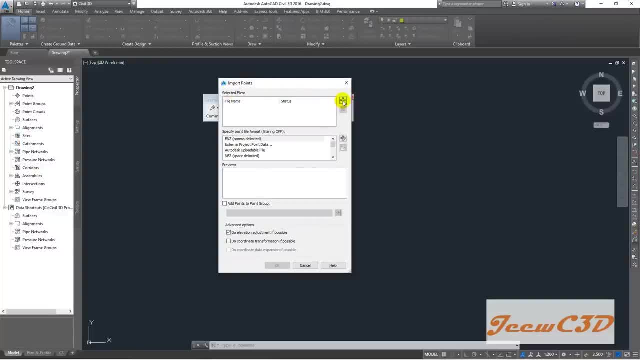 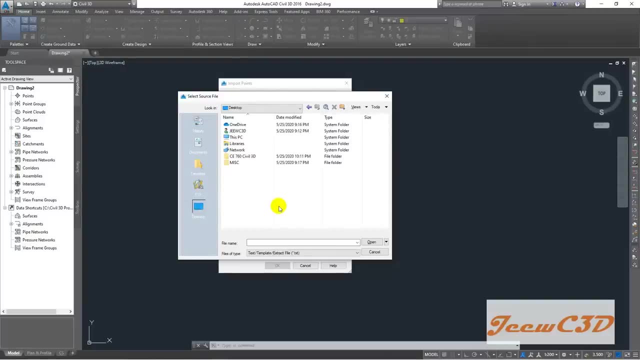 the files. you click this button and then you can see the import points window, now n the upload point. now you can click this plus sign. then you go to your desktop. in my case that is my desktop. here the data are saved. so I go to ce 760 folder and go to data folder and make sure your file type is CSV, this type: 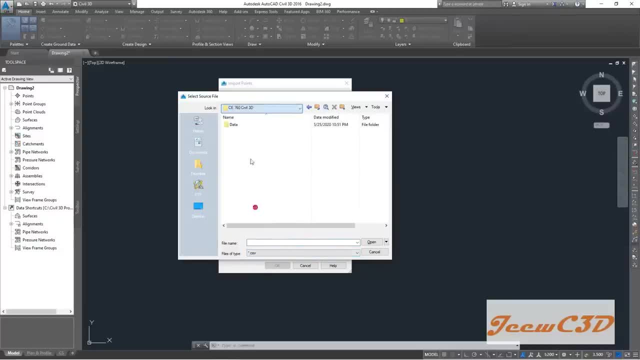 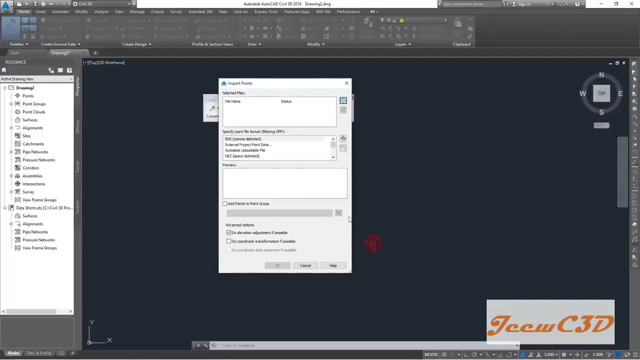 CSV. then you will see inside this data folder, data folder, topo, survey points. you click this point, click this excel file, this kind of excel file, and click open. so in Sri Lanka the surveyors are usually doing the surveyors surveying with the file format called PNEZD. that means 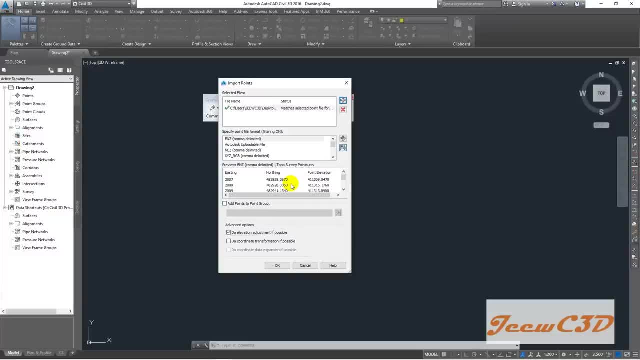 point number for PN means nothing, E means Easting, PNEZ means the elevation, D means the description. so you have to specify the point. file format. so you have to go down here. you will see PNEZD, comma delimited option. then you will. you have to select that one, then you will see. 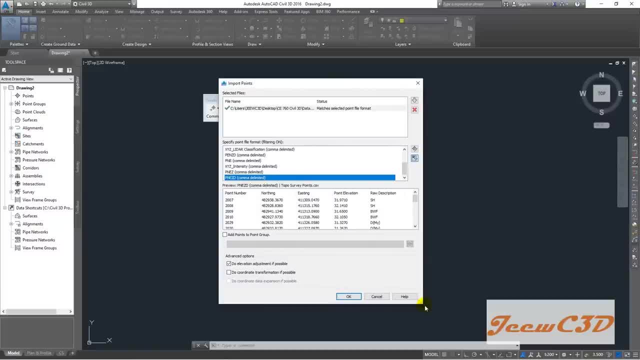 PNEZD comma delimited option, then you will. you have to select that one. then you will see. I am dragging here to enlarge the window so you will see the point numbers, nothing Easting point, elevation and description in these points. so these are the points in this drawing, even though you have small number of points. 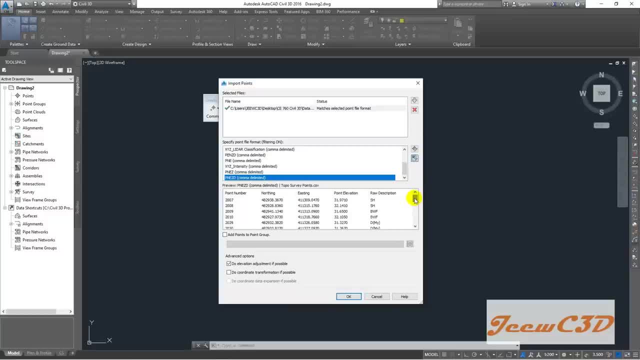 here. it is only a preview. so you have so many points inside this file. so if the file is successfully imported you will see a green check mark here. then you have to put a check here. add points to point group. then you click this to give a name for the point group. 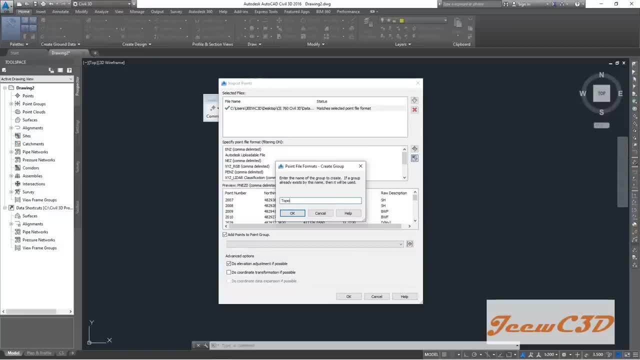 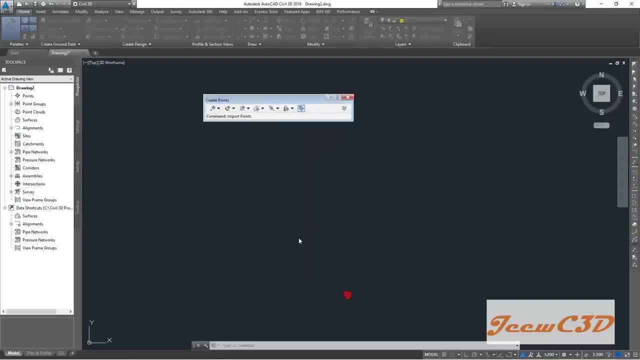 we are importing. we say topo survey points, then we click OK, so we will uncheck this option, uncheck the both of these options and we click OK. so your point file will be imported to your civil treaty, but you will not see anything at the first place because you cannot. it is imported to a. 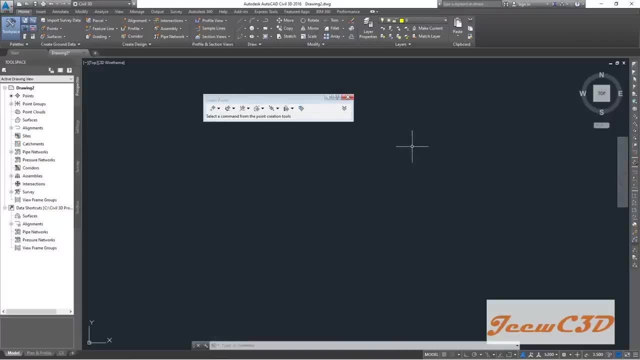 location we are, we can't see in this screen. first I will close this toolbar, then I will double click my mouse wheel. you should have a mouse with a mouse wheel to do civil treaty or to get work. otherwise it is very hard to work with civil treaty or. 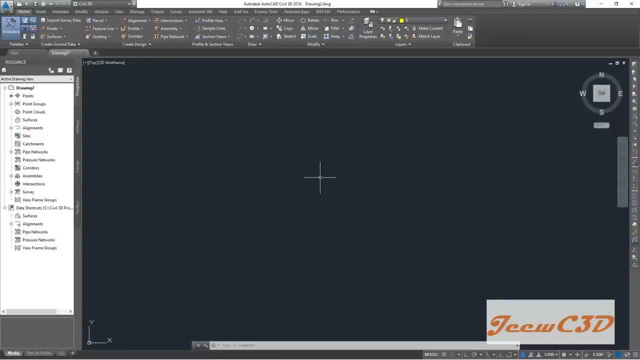 to get base of task. so definitely you should have a mouse with the mouse wheel. so what you have to do is you have to double click the mouse wheel, the middle button. you have to double click the mouse wheel, then you will see the points are appearing inside this drawing if we zoom. 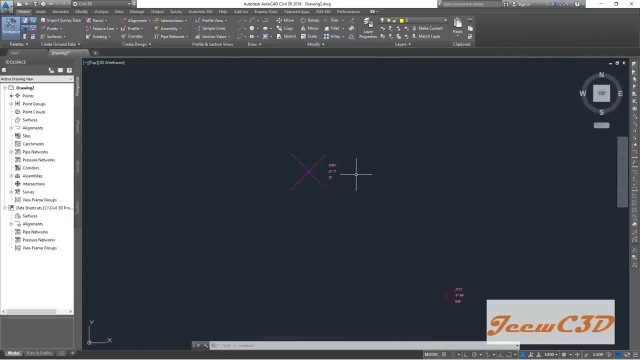 in here you can see the point detail. this is the point number, this is the elevation and this is the description. TE means tar edge, the existing edge of a road. so if we come here, this is the center line of the road. likewise, you have so many point now some kind of 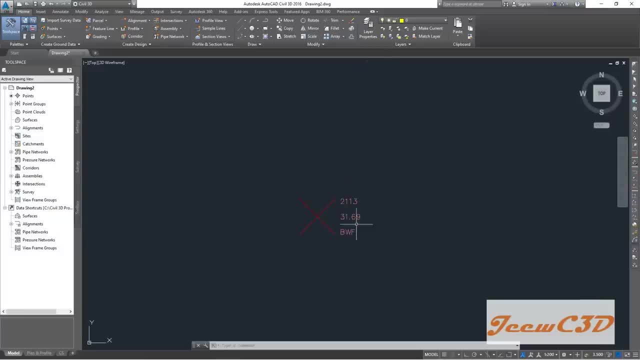 this might be a boundary wall. so these descriptions, survey point descriptions, will be given to you by the survey. here you have tar edge points. this is telephone post. likewise you have so many points, which is which are taken by the surveyor, so we have imported the points into our drawing. now we are going to save this. 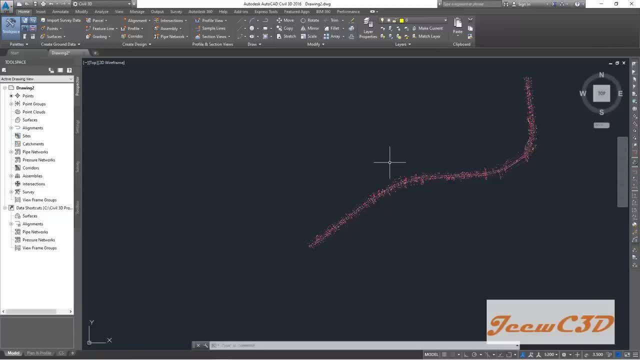 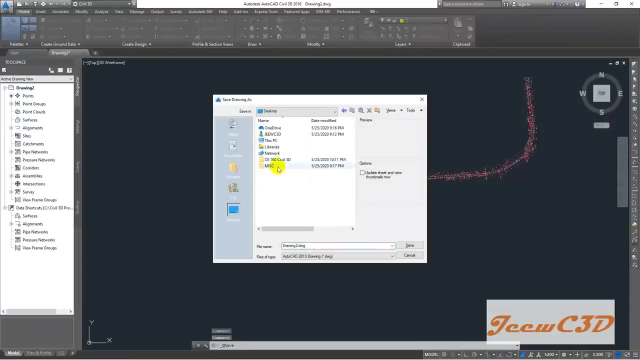 drawing with a name. to do that, I am clicking save here, save option here, although otherwise you can go to application menu browser and click save. then I am going to my desktop and go into this file and not in the data folder. outside the data folder I will save my drawing. 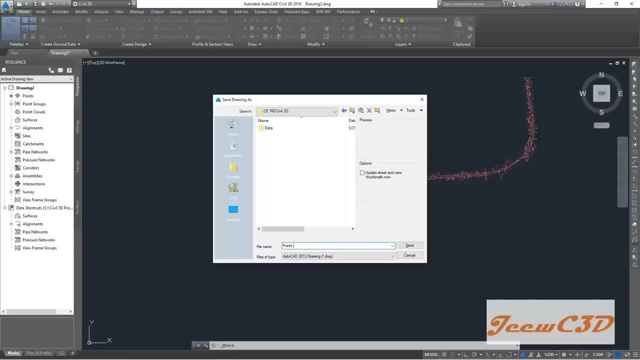 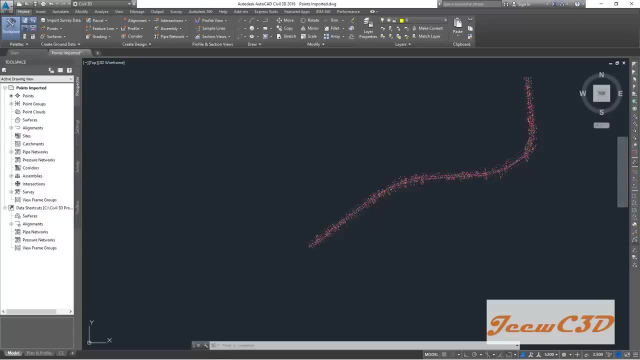 as points imported, then I click save. so up to this point we have. we have imported civil 3d points into the civil 3d drawing. in the next video we will be discussing something called extra, something called external reference, so we will be looking at that. 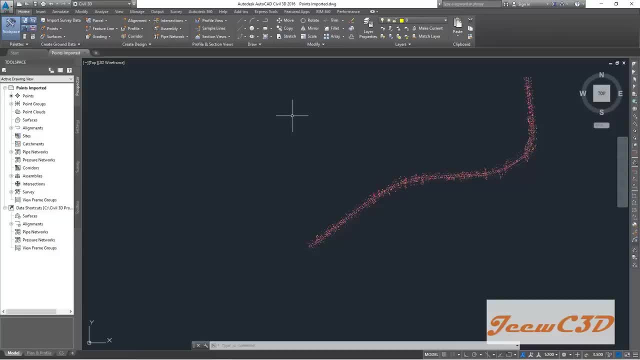 in the next video. please don't the. please don't close the drawing. so you can work with the with this drawing in the next video. also in this video we are talking about a concept called externally reference drawing. in the previous video we have imported civil 3d points into our 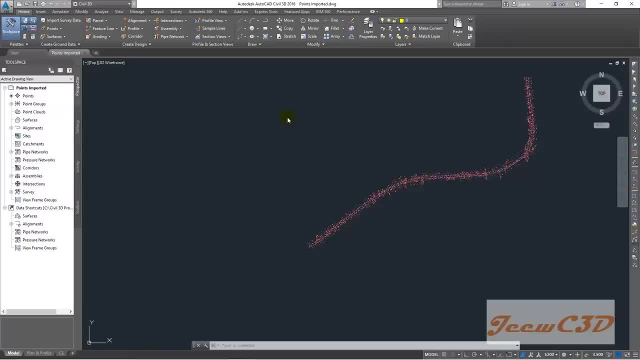 drawing where a survey has been taken, the survey points, and we have imported that points into our drawing. but we still don't know whether these points are imported to the correct location. there's no clue for us whether we have imported the points to the correct location. so to 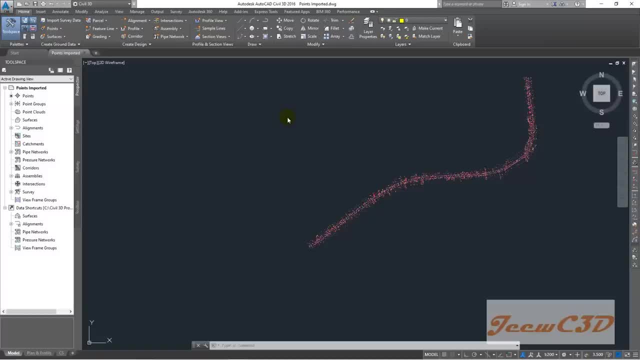 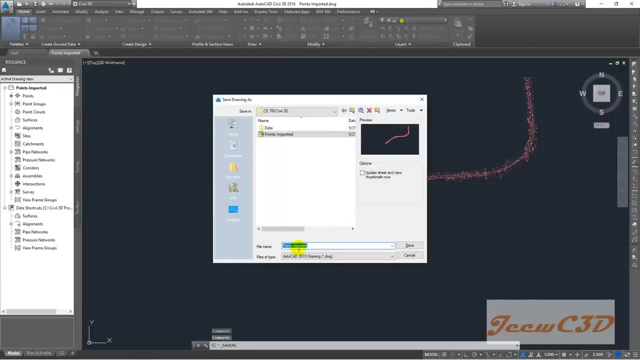 ensure that we are doing something called externally reference drawing. so we are going to do that now. first I have, I am going to save this drawing as a separate file. to do that, I go here: application menu browser, then you go to save as. then you type the file name as external. 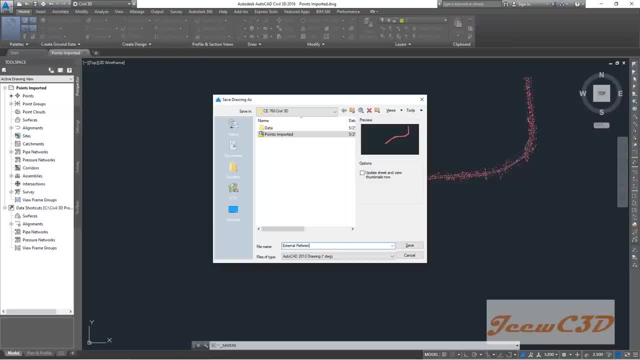 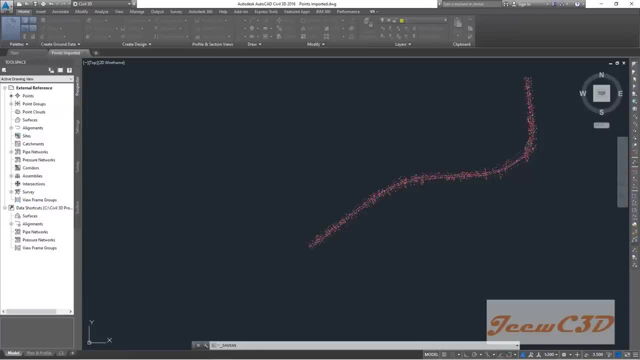 reference- external reference- then click save. now what I am going to do is I am going to externally reference the drawing into this current drawing. to do that, I am typing x- rest in my command bar. paste the cursor in my command bar, then type x- rest, xres and press enter. so you will be getting a small window like this. you can drag here and 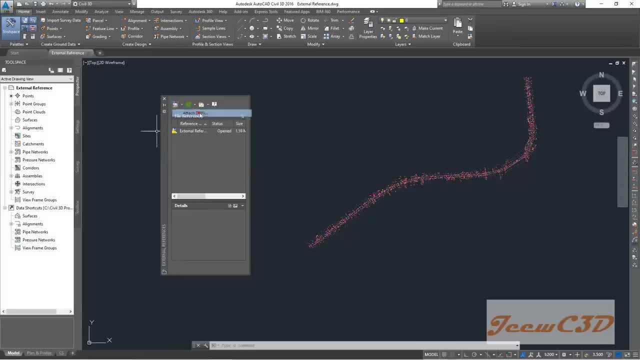 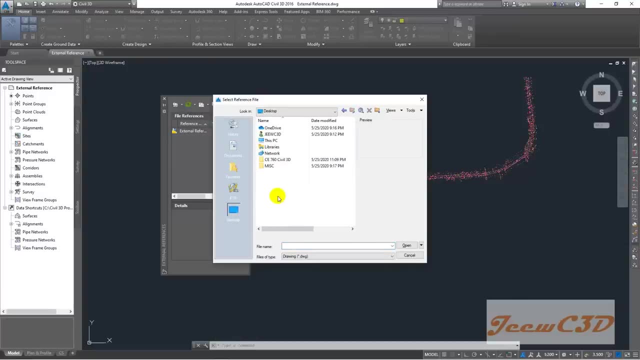 click here, this small drop down click- attach drawing. then you go to desktop- in my case it is desktop- and you have to go to the cvtd data folder which i gave you. then you click on this data folder here, then click on this topo survey drawing, click on this topo survey drawing and 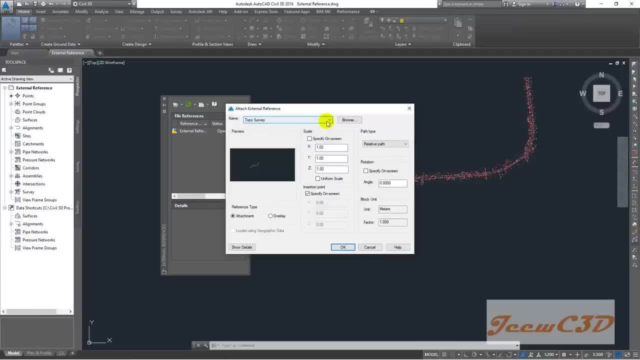 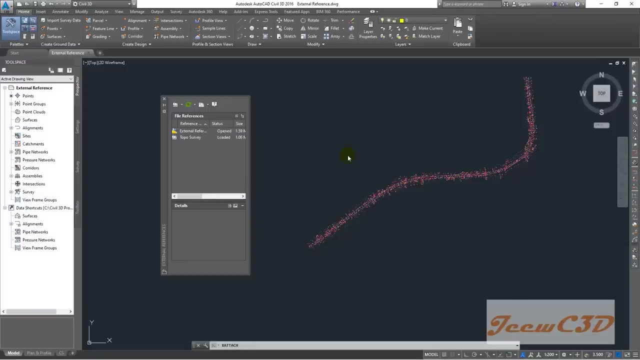 click open so another small window will be appearing. make sure this scale button is unchecked. this insertion point is unchecked. all these points are unchecked. and make sure the drawing. you need some meters. then click ok, then you will see there is a survey drawing appeared in our points drawing. it is: 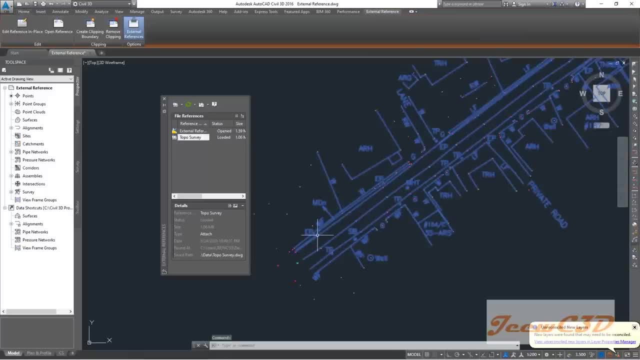 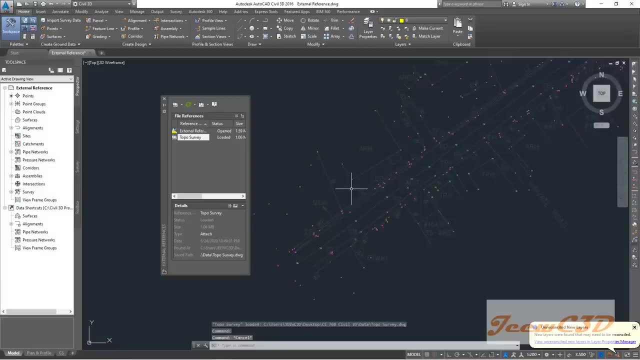 an external drawing. it is not in this drawing. it is an external drawing, so we are creating an external reference, like we are looking something from a butter sheet, so we have something like that. so this is at the background, not inside this drawing, not on top of this drawing. it is. 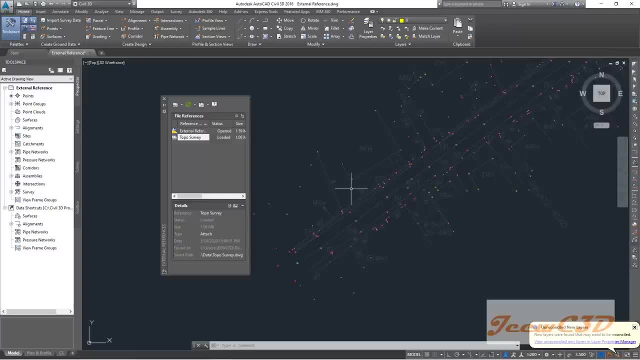 inside the background you will see the survey. so that is what you call externally referencing a survey. so if we have done something wrong in our point import option, that means if we have imported the points to the wrong location, so this survey and the points will not be. 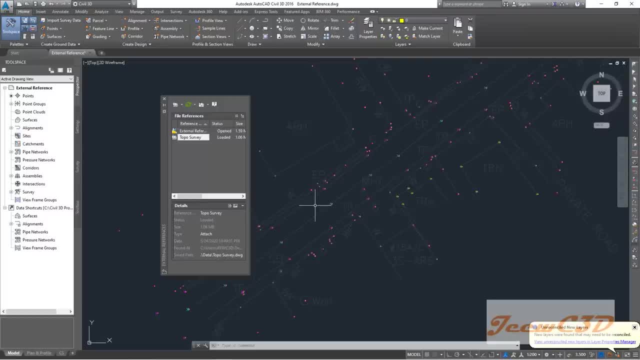 coincide with each other. that is how you and make sure that your points are imported to the next location. so if you both survey and points are at your own at rom locations, we can't help for that one. but if they are at the correct locations, but we have not surfaced the values, for where are 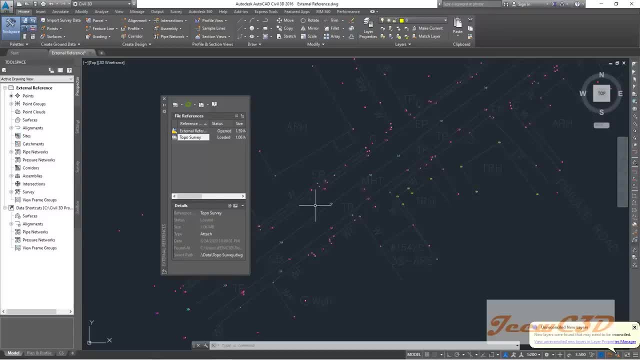 the points with the right location. if the points are at the right location, we can tell we beached. If we have done it in the wrong way, we can make sure that we have done something wrong by external referencing the drawing. If we have done something wrong, this external reference drawing will not be coincide with this drawing. 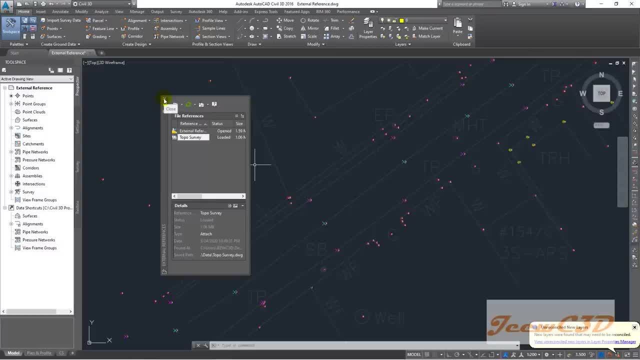 So I will close this external reference manager. Then you will see the points. are these star edge points? that means the edge of the road points are connecting through a line. Then you have some other lines also Here. you have another road going outside. 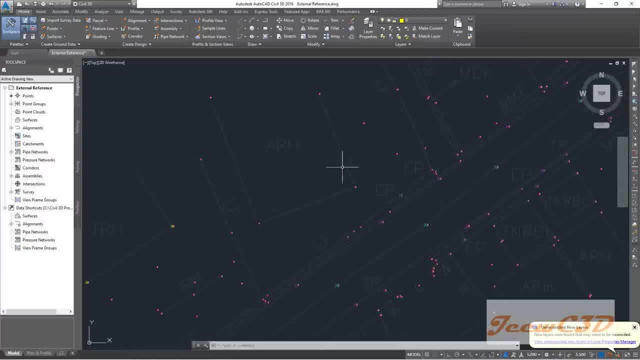 Likewise, there you have building edges. So that is how to externally reference a drawing. So if you don't need it, If you want to see this drawing, you can unload it. So to unload it, you type: extract again in your command bar. 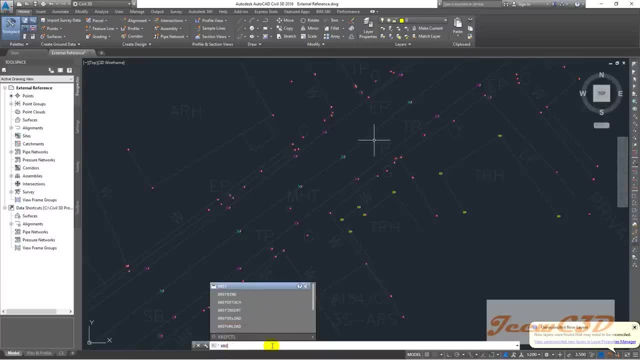 And you go here and press extract And then press enter. So to avoid to hide this survey, you have to unload this one. Right click and unload. If you want to reload it again, you can reload it, Unload and reload. 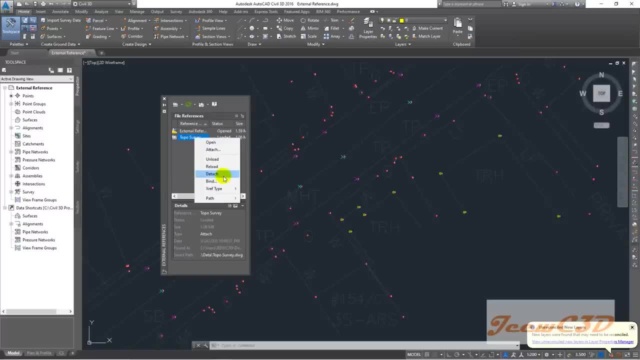 Likewise, if you want to remove this attachment from this drawing, you have to click this detach button. But I am not going to do it, So instead I can do unload for a moment if I need. Otherwise, you can keep it with you by reloading the drawing. 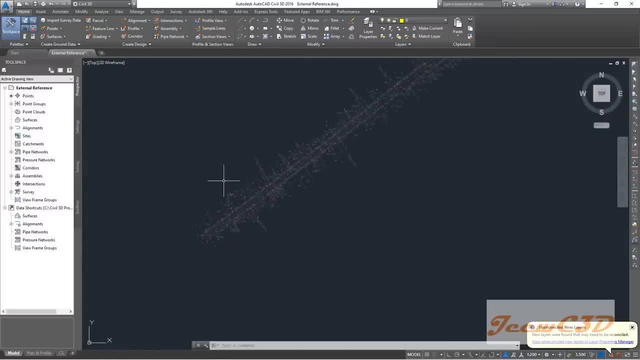 That is how you create an external reference to a working drawing. So in the next video we are going to create a ground data module or ground module from the imported points In this video. what we are going to do is we are going to create a surface or the ground data module from the points we have imported. 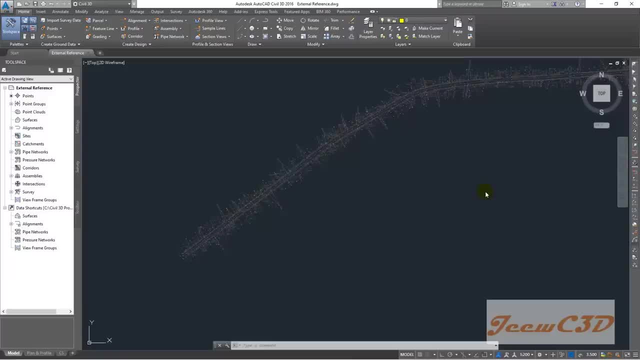 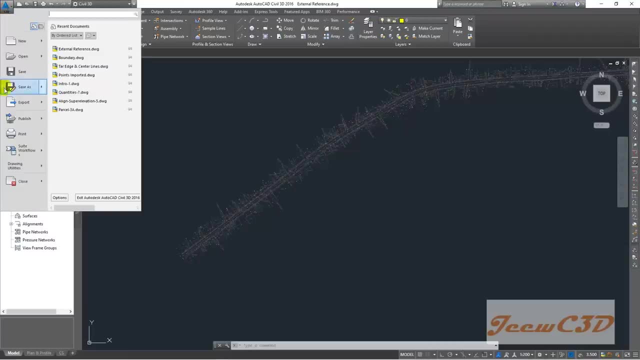 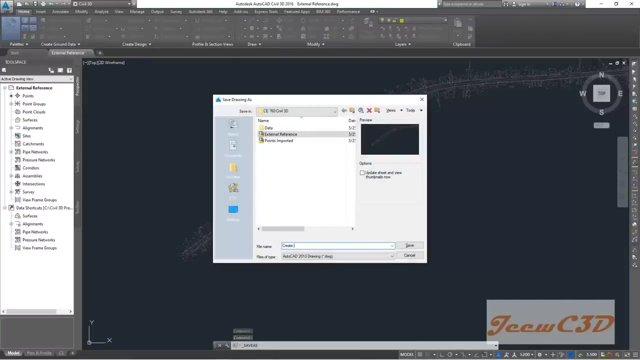 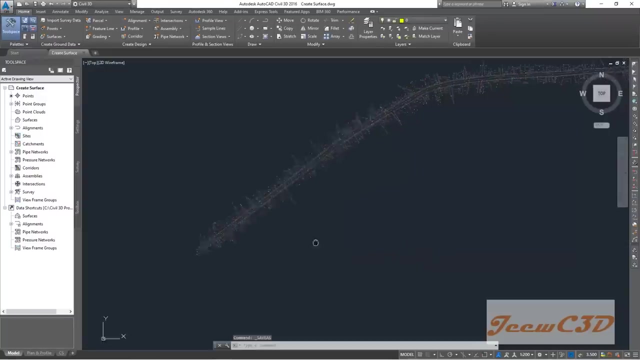 Before that I will change this drawing name as create surface. To do that I go to application menu browser, Then go to save as, And I change my name as Create surface And then I click save. So it seems like my external reference is making a little bit of a problem here. 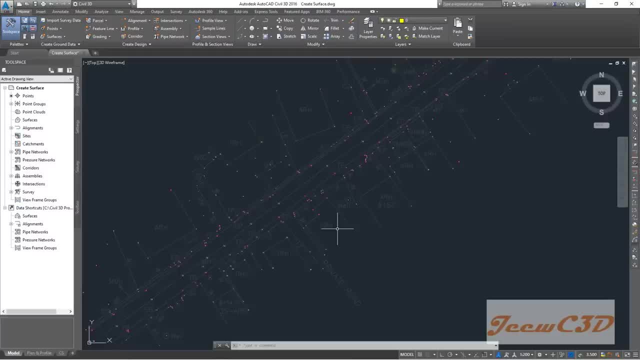 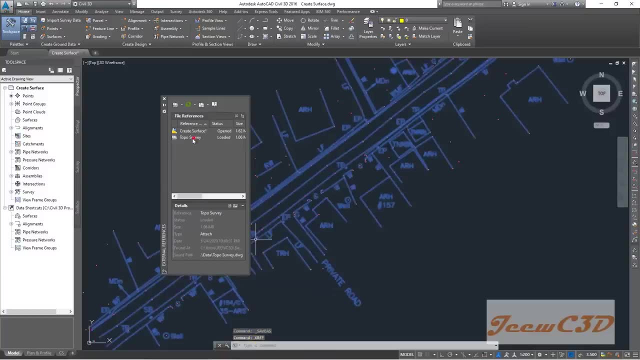 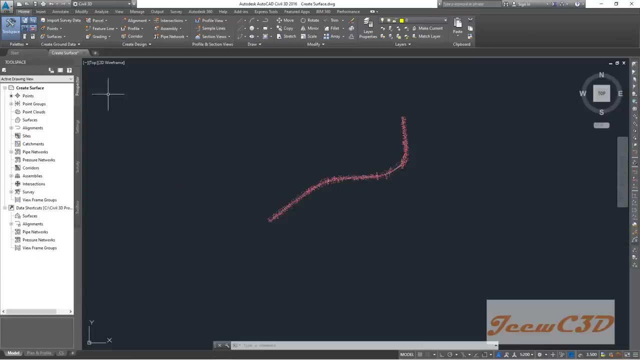 So I will hide this one. To do that, I type extras, Extras in my command bar, Press enter. Then I click this propose a way button Drawing and right click Unload. Then I close this external reference manager. Then what I do is I go to prospector. 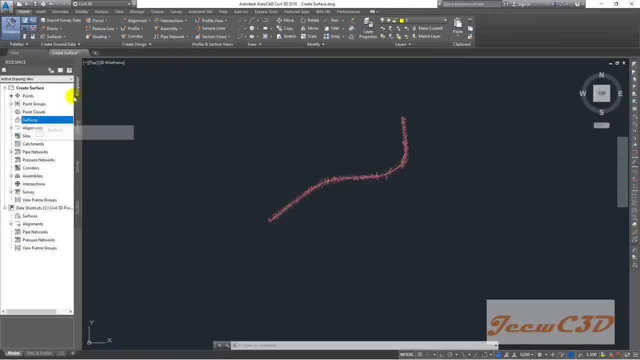 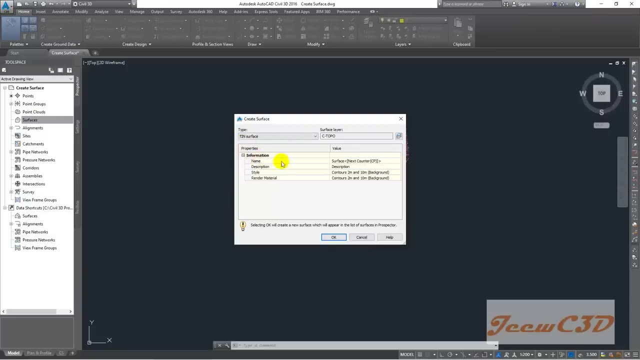 Then here surfaces. Make sure you are going in the prospector tab, Then surfaces, Right click, Then create surface, Then your type would be tinsurface, Then the name would be existing ground. Let us say eg existing ground. You can say the description as existing ground. 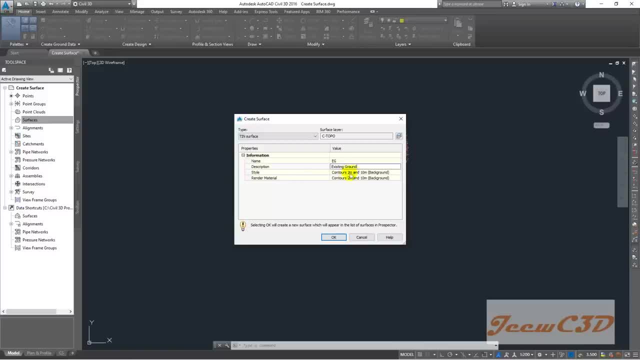 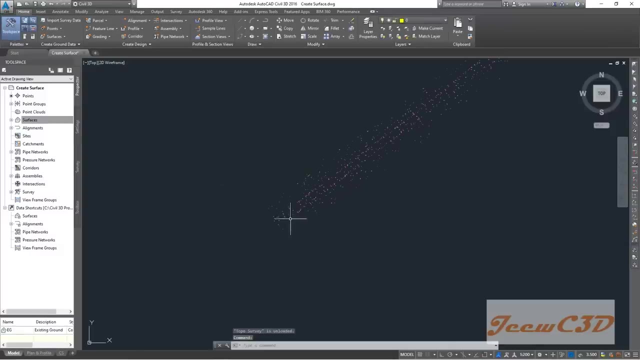 So this surface will be display as It's a contours, stylus, contours unit and unit background. You can change it. You can change it later. For the moment, I click okay. Still, we have created the name for the surface. 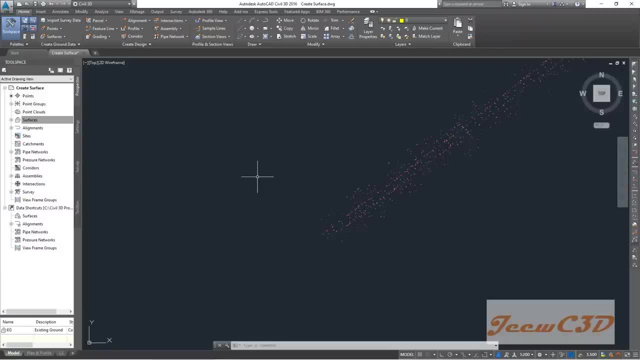 We haven't add any data to this surface. To do that, we go to prospector again And surfaces. you will see that now it is populated with the name for eg But there is no data here. In my first videos I told you that any other data is available. 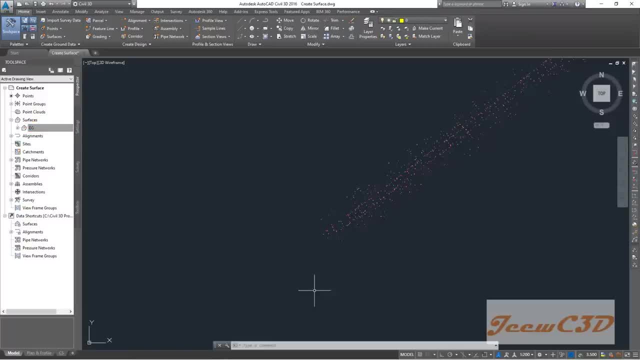 available. it is showing in the perspective. in my drawing we have civiltrative points. so it is giving me a bullet sign here, giving me a notice that we have points here. so these points are shown in this preview area. if you drag it somewhere up you can see the point number and everything will be shown to you. 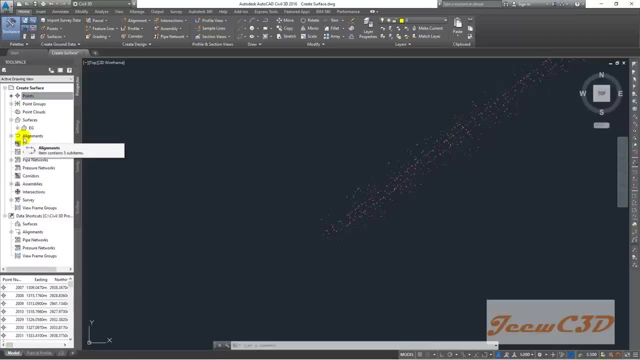 so that is happening when you have points, but here we have only the surface name. we don't have any data here, so it is not showing in the preview area. so in this, what we are going to do is we are going to import- sorry, we are going to add data to our surface. 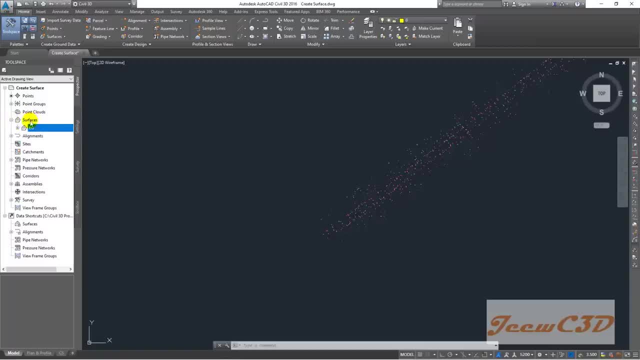 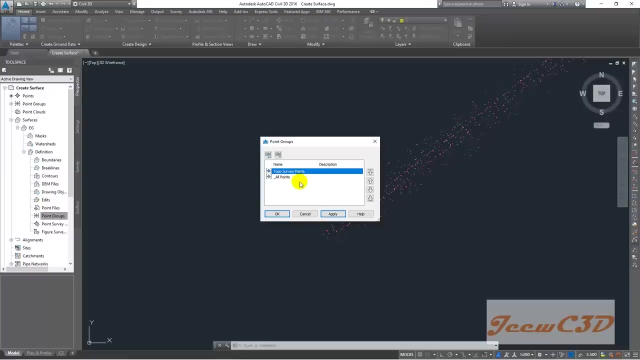 to do that. we go here, expand the surface. then you have EG- I will expand it again. then you have definition. we expand that again. then you have something called point groups. you right click there and go to add. then you have two point groups, which here you have, that is all points- and toposurvey points. both are same. 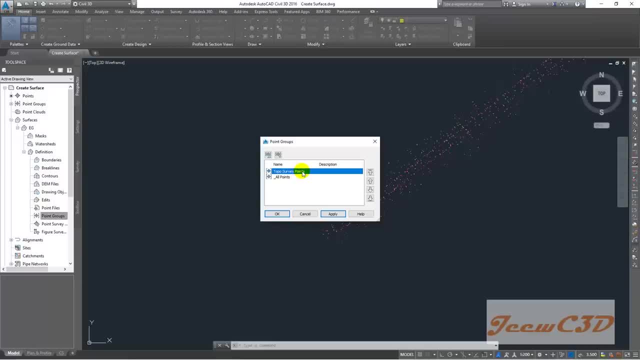 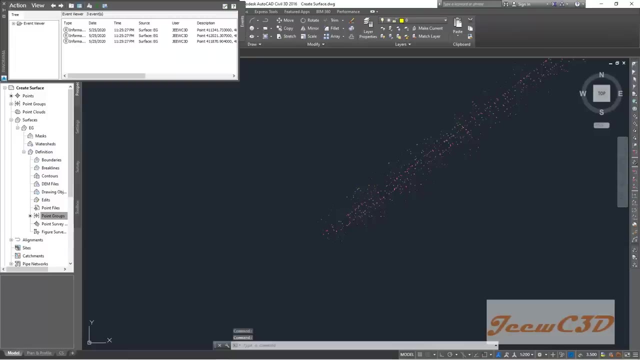 but you have to select the toposurvey points. that is the point group we have imported in few minutes earlier. so I select proposal waypoints and click ok. you will be seeing that the surface is appearing on your drawing. so this is the surface, these are the contours, this is the ground data surface. so I will, if you, 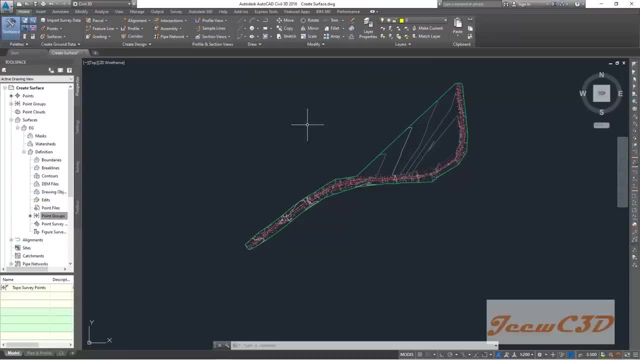 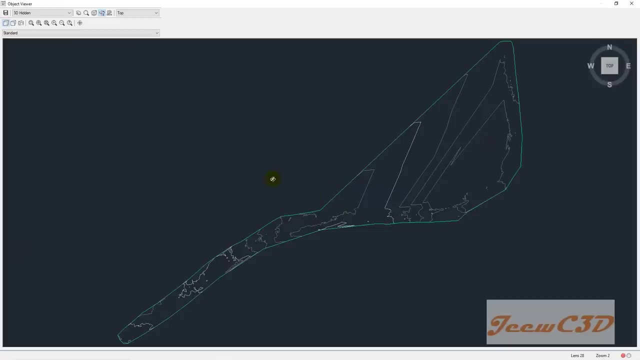 got a message like this: you just click here to turn off that one. then click somewhere in this gray output or this green line and right click, go to object viewer. object viewer- then you can maximize this one, this in here. just drag the mouse, you will see some kind of a 3d model in this area. 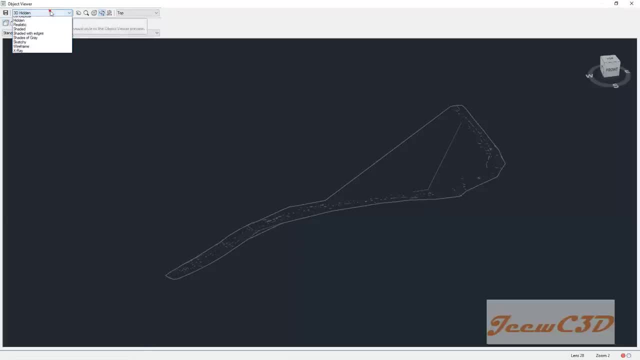 you will see some kind of a 3d model in this area. you will see some kind of a 3d model in this area. so you can in this type from, so you can in this type from, so you can in this type from here. so then you will see that things. 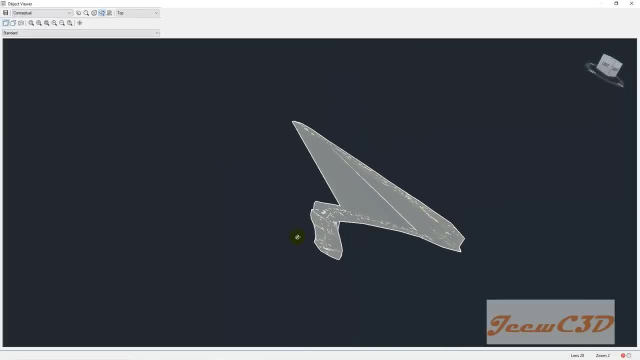 here. so then you will see that things here. so then you will see that things very clearly, very clearly, very clearly you will be seeing. now there is some you will be seeing. now there is some you will be seeing. now there is some kind of road going on the middle. you can. 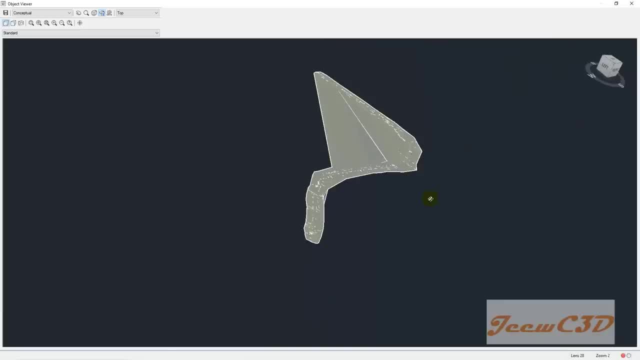 kind of road going on the middle. you can kind of road going on the middle. you can see it here, some kind of a road going in. see it here, some kind of a road going in. see it here, some kind of a road going in the middle. and I will close this for the. 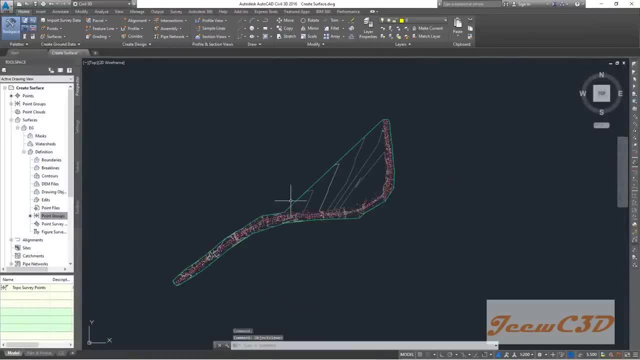 the middle and I will close this for the the middle and I will close this for the moment. and you can see the surface this moment and you can see the surface this moment and you can see the surface. this green area is the surface border, so you green area is the surface border, so you. 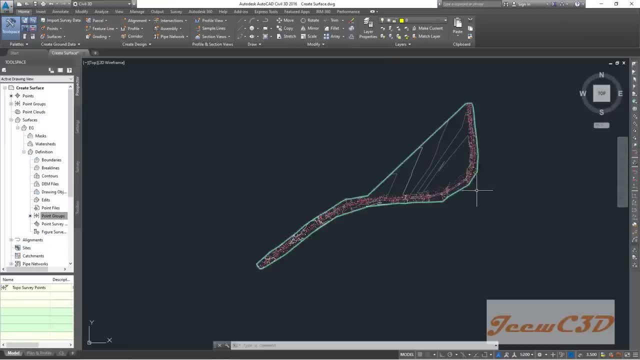 green area is the surface border. so you can see the point. details are in this. can see the point, details are in this. can see the point: details are in this area but the surface is also appearing in area. but the surface is also appearing in area, but the surface is also appearing in this area. so, yes, something problem is. 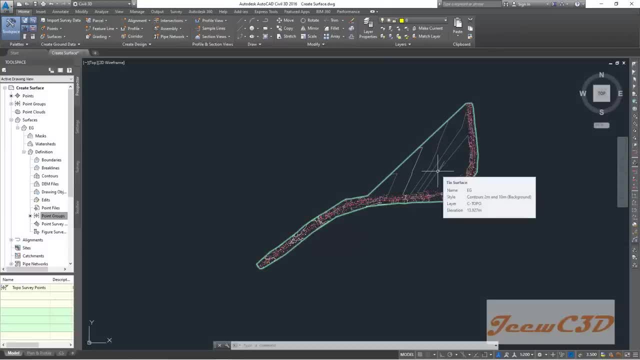 this area. so yes, something problem is this area. so yes, something problem is there. so without point detail, you can't there. so without point detail, you can't there. so without point detail, you can't have a surface, but just connecting these. have a surface, but just connecting these. 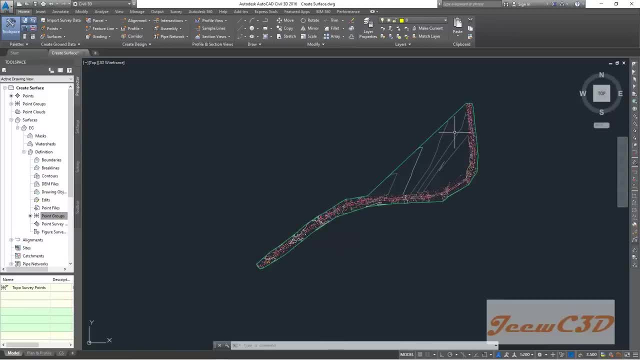 have a surface. but just connecting these points, from this point to this point, it points from this point to this point, it points from this point to this point. it is creating a surface, but in the middle is creating a surface, but in the middle is creating a surface, but in the middle of this area, we don't know what, what are? 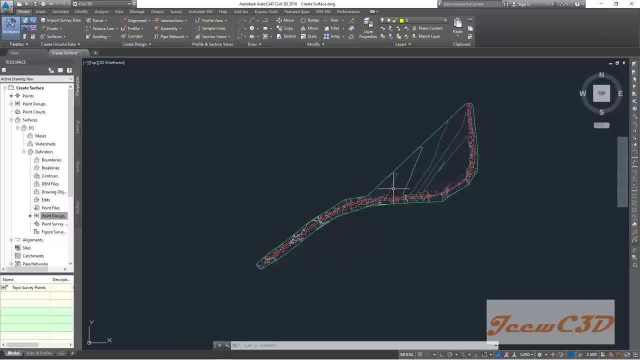 of this area. we don't know what. what are of this area? we don't know what. what are the things are they are, so we can't say the things are they are, so we can't say the things are they are, so we can't say this. so in this area, the surface is. 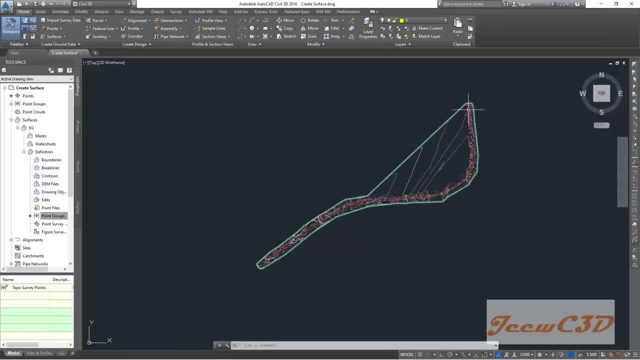 this. so in this area, the surface is this. so in this area, the surface is great, it should be going like this. they great, it should be going like this. they great, it should be going like this. they are. you have the points, so you have to. are. you have the points, so you have to. 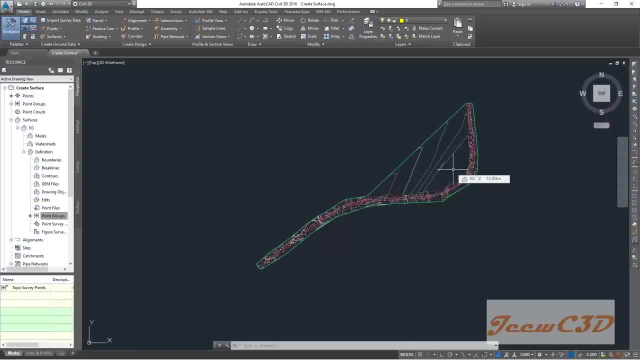 are. you have the points, so you have to correct this one to correct this. you need correct this one to correct this. you need correct this one to correct this. you need to apply a boundary to this surface. so to apply a boundary to this surface. so to apply a boundary to this surface so that we are telling the surface you have. 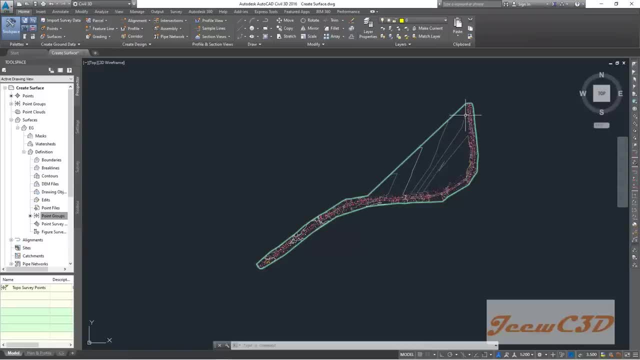 that we are telling the surface you have that we are telling the surface you have to go within the boundary we give to you to go within the boundary we give to you to go within the boundary we give to you, so that boundary would be the edge of. 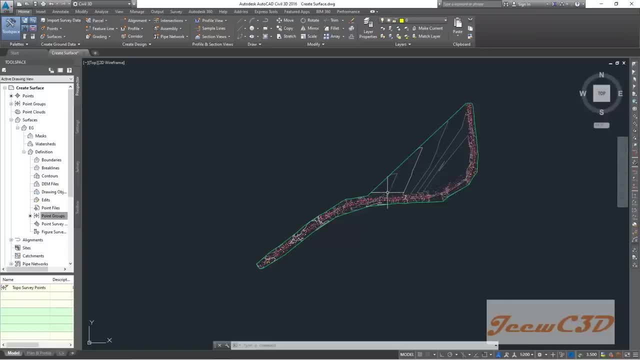 so that boundary would be the edge of, so that boundary would be the edge of the points, the points, the points in our, in our, in our drawing, drawing, drawing. so to get the boundary, so to get the boundary, so to get the boundary, i want you to go to the drawings folder. 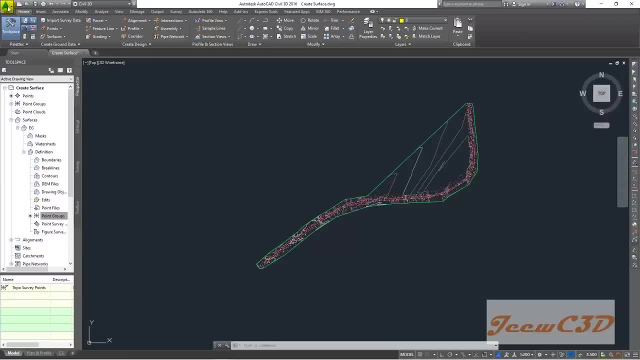 i want you to go to the drawings folder. i want you to go to the drawings folder. that means that means that means you have to go to this application in. you have to go to this application in. you have to go to this application in your browser, your browser. 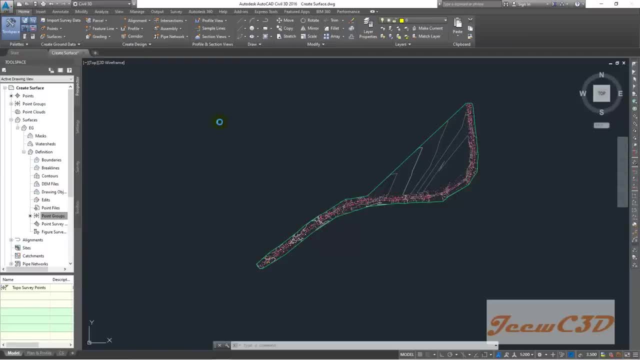 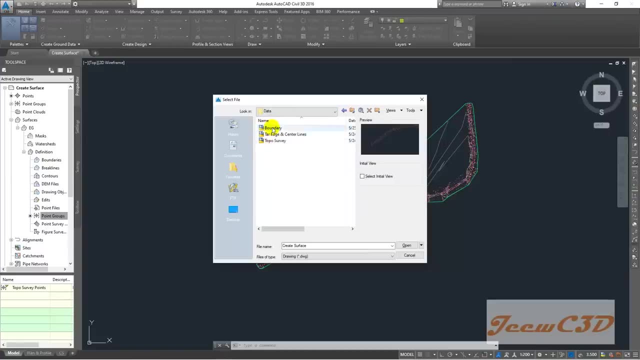 your browser, then this time you have to open, then this time you have to open, then this time you have to open and go into your and go into your and go into your 3d data folder, 3d data folder, 3d data folder. then we have something called boundary. 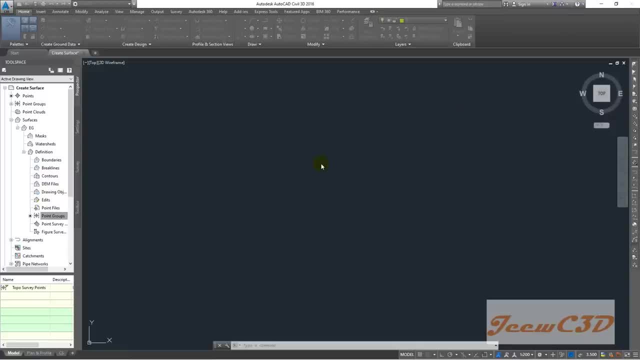 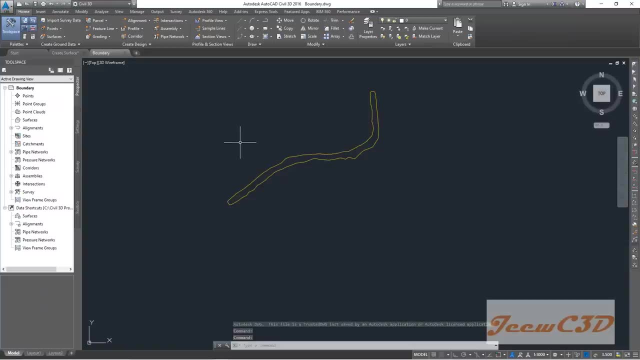 then we have something called boundary, then we have something called boundary. then click open so you will see a boundary like this, a polyline like a boundary like this, a polyline like a boundary like this, a polyline like this: that is a boundary, this, that is a boundary, this, that is a boundary. so what you have to do is: 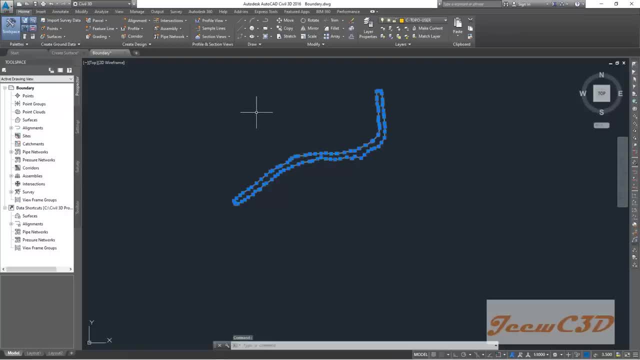 so what you have to do is. so what you have to do is you select this one, then right click, go to clipboard, then select this one, copy this base point. then it is asking a base point in the command line type, in the command line 0,0,0, and press enter so it will. 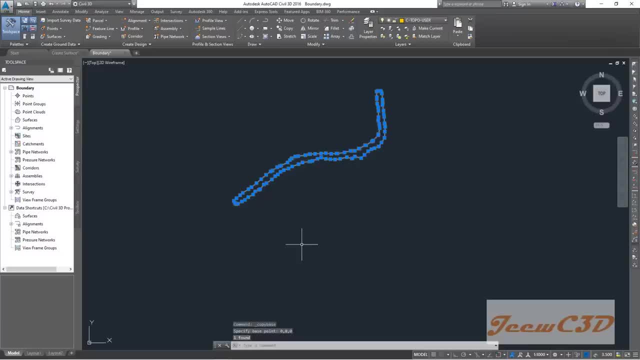 be copied in to your drawing, into your clipboard. then you move on to create surface drawing. create surface drawing. here we have the surface. then right click, go to clipboard, then go to paste. so it will be asking paste, specify insertion point. click, click here and type this one, copy this one. then click in. 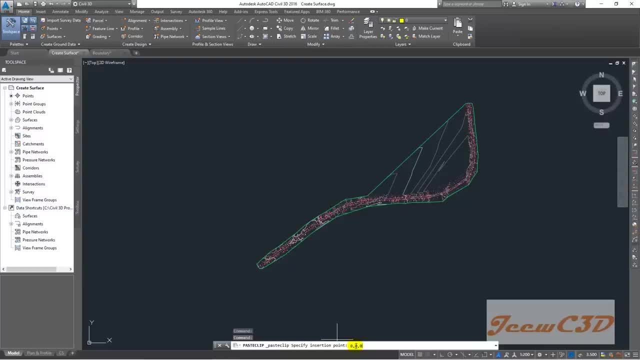 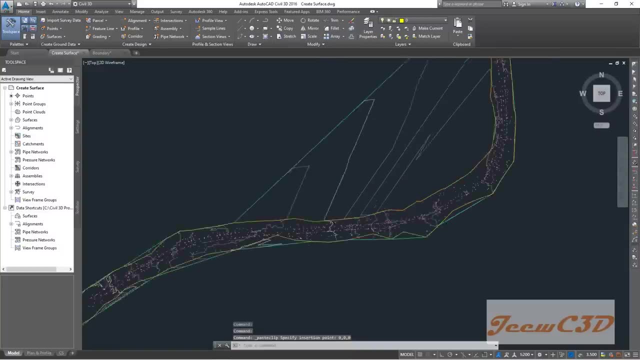 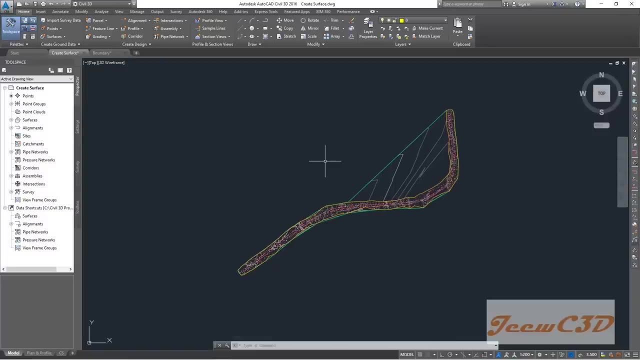 0 comma 0 comma 0. we are you type for this point, similar as that one in presenter, and you will see some kind of a boundary is appearing in the drawing. so even though we copied a boundary, it is not appeared. it is not applied in. 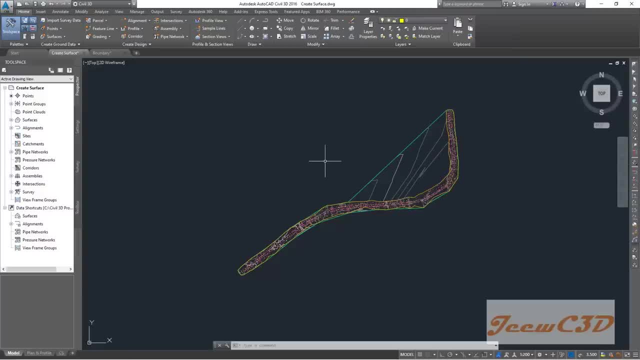 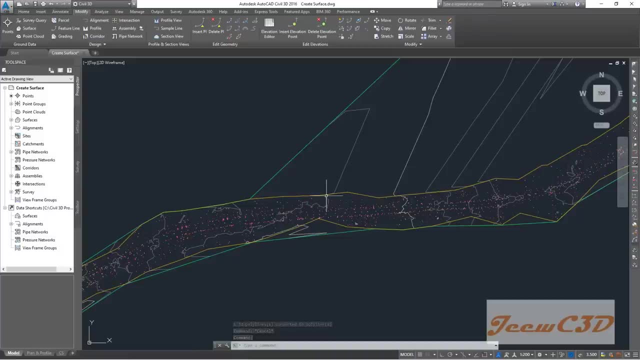 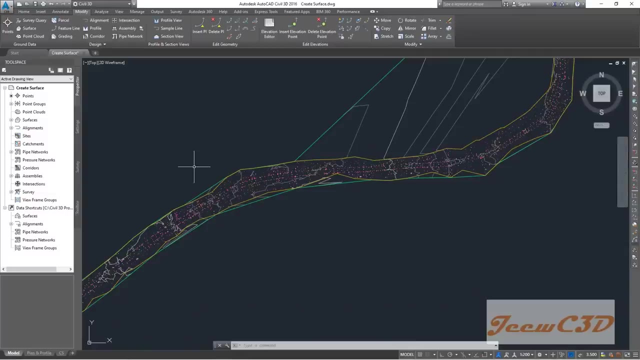 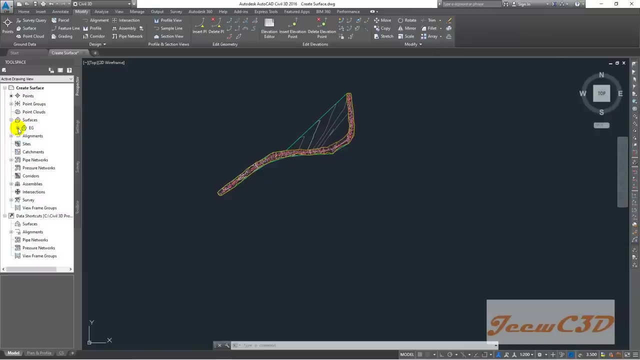 this drawing yet, so we have to apply it. now. we apply this. what we have to do is you go here surfaces. when you go to EG, expand it, can you go to definition? then in divide it xy这是 xz 표, ant xz to boundaries. right click and go to add. 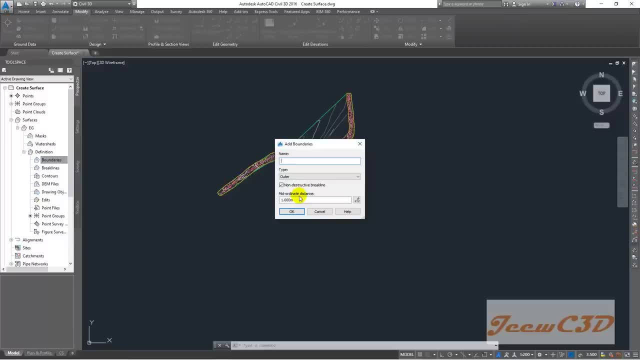 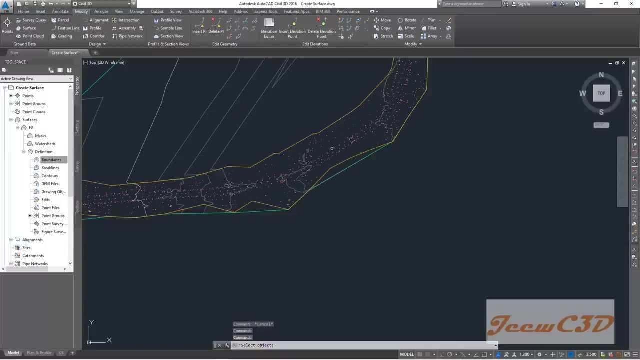 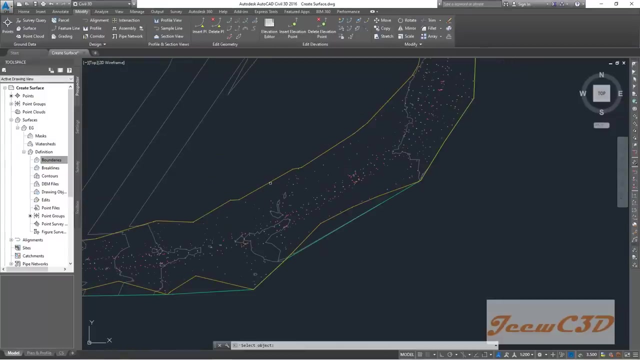 then type your name as outer, then uncheck, don't change these options. click ok. then it will be asking in the command line: select an object. so that is asking to select a boundary. now soon into your drawing and select this yellow coloured boundary. copy there here this yellow colour boundary. copy the area and pick. 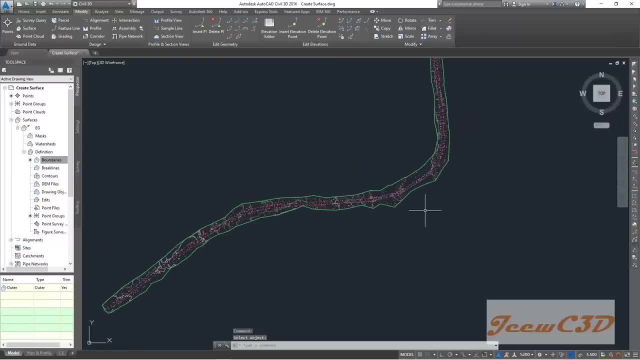 it. so you will see your boundaries eat into, you are absorbing, syncing into. no new boundaries. you are all boundaries. soon, king, into your Śrinkāś air doctrine, your all new boundary, so that you do the drawing a new realistic view without the unrealistic edge initially posed in this location. so that is about creating a surface in the next video. 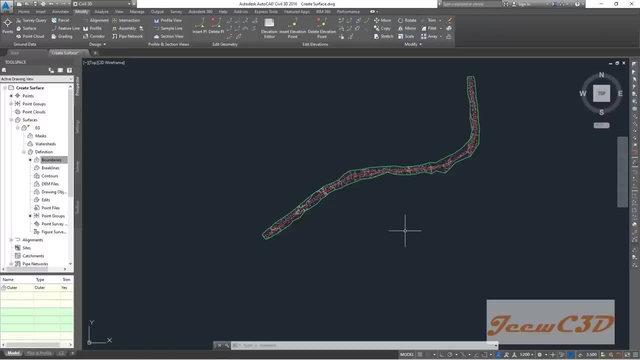 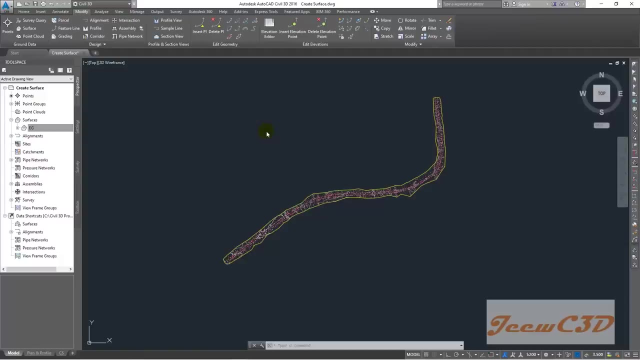 we will be talking about applying break lines and exporting and importing- exporting the surface to a planned extended version. in this video, what we are going to do is something called adding break lines to a surface. so that is something important when you are doing a 7kd work, when you are creating a 7kd. 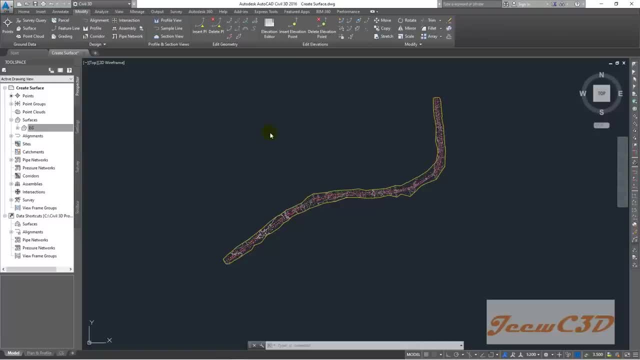 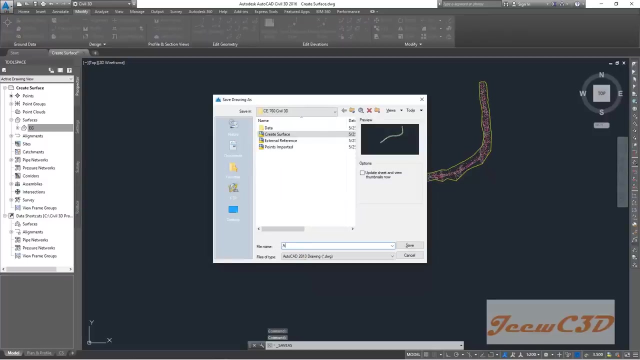 surface especially, you have to add break lines. break lines are something for items where you know whether, when items where you know the surface changes at the definite point. so i will show you that. to do that you have to, uh, change this drawing name as at break lines. so i go here and click save as and change the nameness. 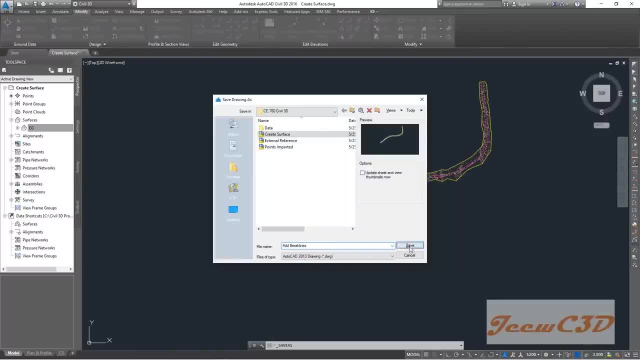 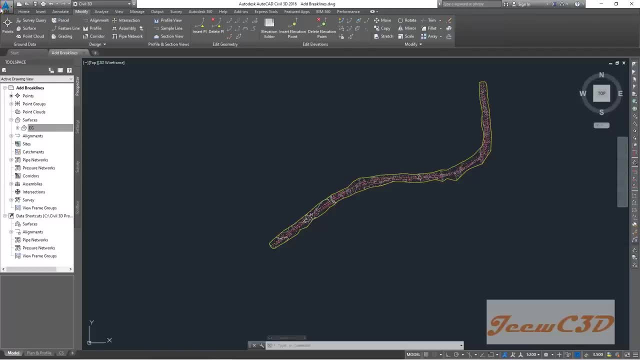 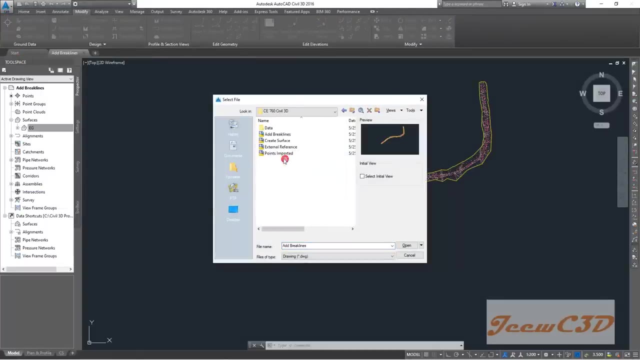 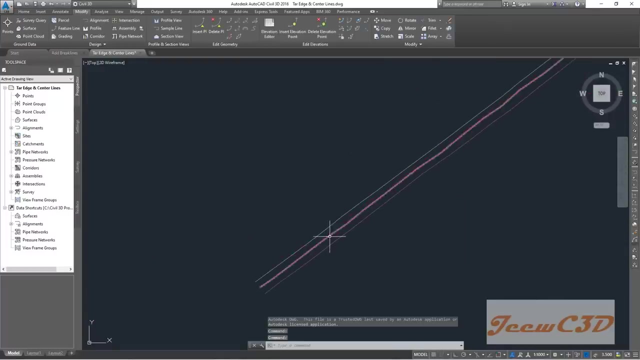 at break lines and break lines, click save. then again i am going here, i am going to open a new drawing. so in your data folder you have tar edge and centerline lines that drawing. click that one and click open so you will see something called see the tar edges and centerline of the road- existing road in the 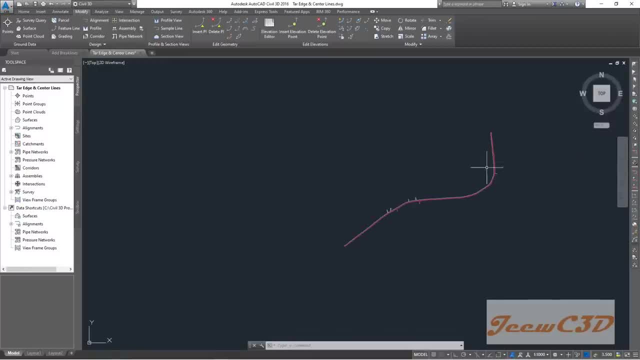 drawing we are working with so it is extracted to a separate place in here. so it is giving only these lines in this drawing. but you see, here it is showing these lines, these center lines. they are marked as a line. so it is giving those lines in a separate drawing. 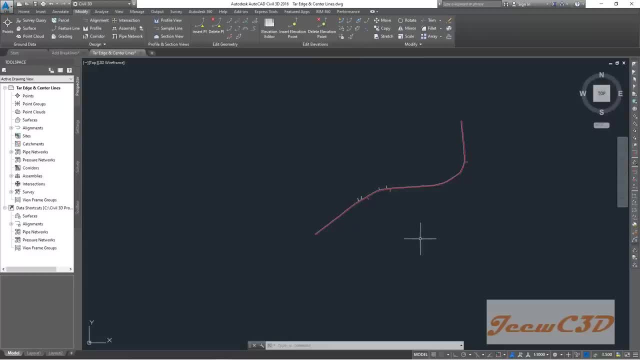 so what we are going to do is we are copying this line into that drawing. so to do that, select all the objects. select all the objects, right click this board, appropriate page point, then zero comma zero will be your base point. click enter. then go back to your add breakup drawing and brake lines drawing. 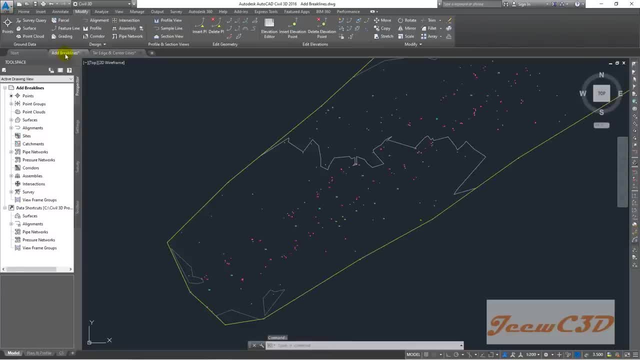 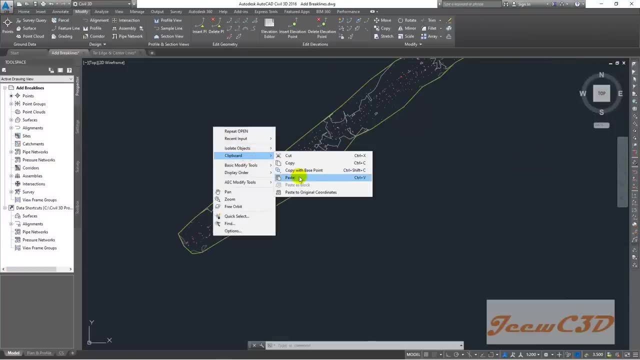 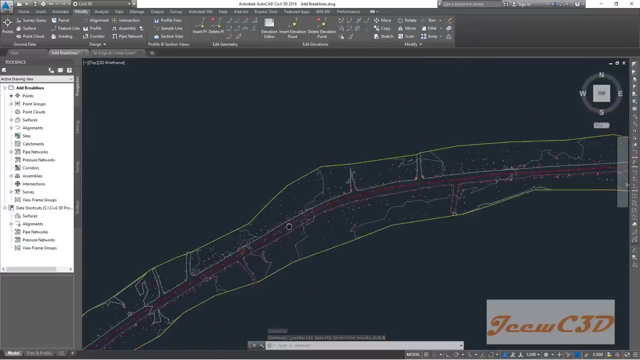 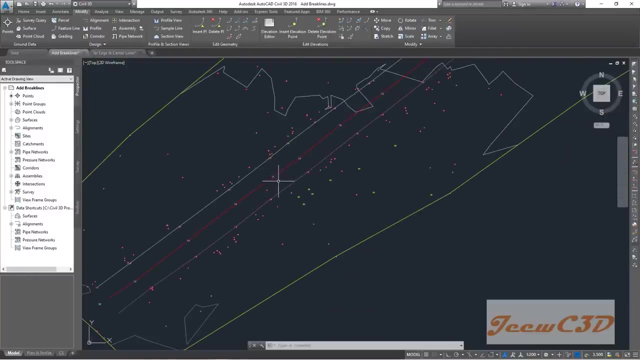 at break lines drawing this drawing. right click clipboard paste. then you type 0 0 0, 0 comma, 0 comma 0 as your insertion point. press enter. you will see the lines are coming into this drawing. so what we are going to do here is we know that within the arched lines and centerline, that means 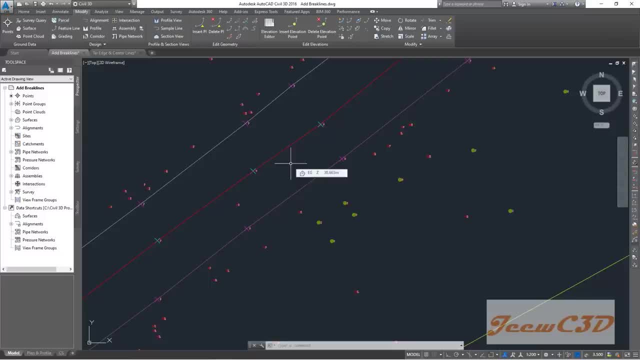 within the existing road. the road have a definite shape because the road have a definite slope and a definite shape between the road edges and the centerline. it is different from the existing round. it has the definite shape when it comes to the road. so if you think of a dam, 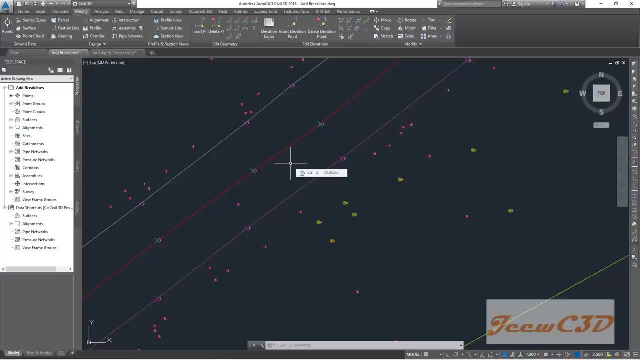 it has a definite shape. so they are. the slope of the object is where the slope of object can be identified without any problem. we call that line as a break line, so you can identify the edge of the lane and center of the lane easily. so we call them as break lines. in terms of a dam, top of the. 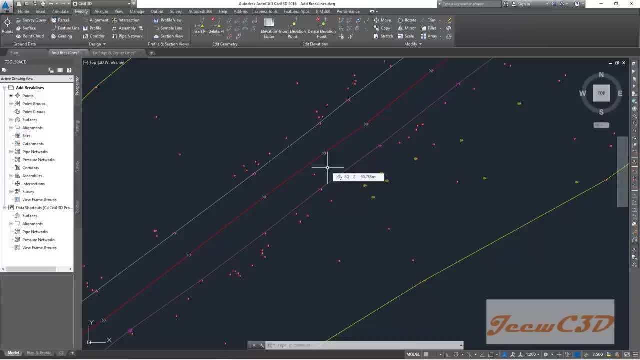 dam will be a break line because you can see at the top the slopes are changing from that damage line. so that is how to identify break lines. if you consider of a channel or an irrigation canal, you will see the bottom of the canal, the slope changes and at the top 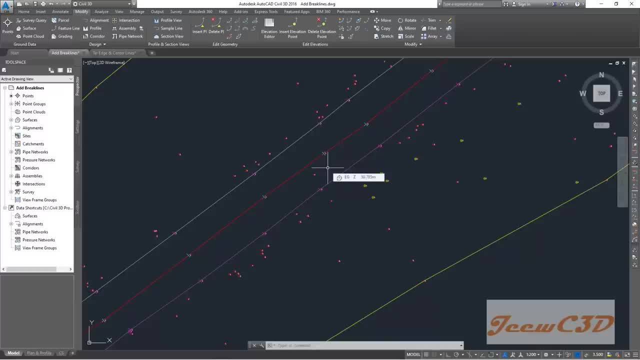 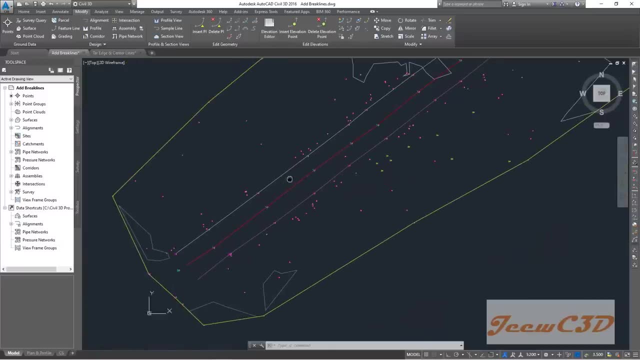 of the canal also slope changes, so those lines would be break lines. so here we have the road edges as our break lines, so we will be applying them into the surface to get a more accurate surface, so to to make sure that we are getting a more accurate surface. 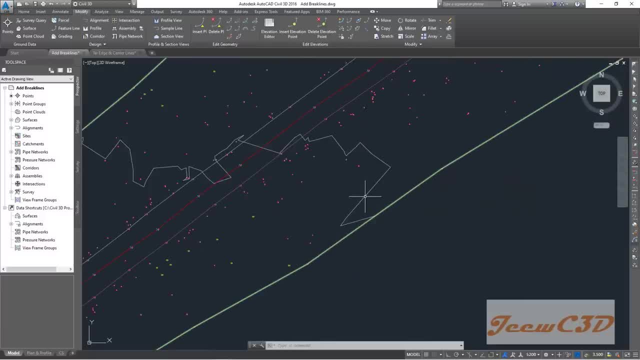 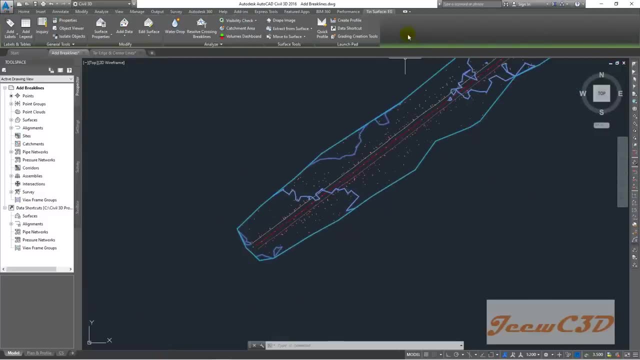 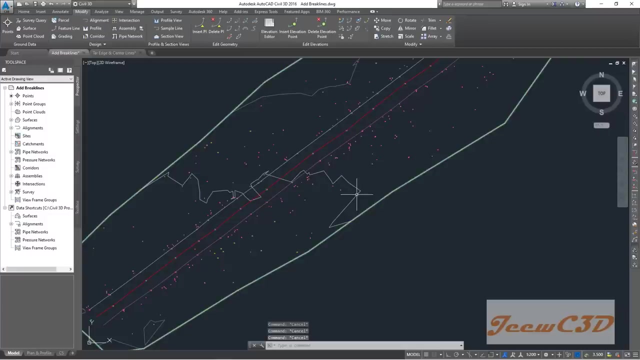 i want you to click this one of these contour lines so you will be getting whole surface selected. so you will have to be seeing something like this in surface ag. so if you don't see something like this, press state bar on state button on your keyboard. then again select this line, then you will see this. then right click and go to object viewer. 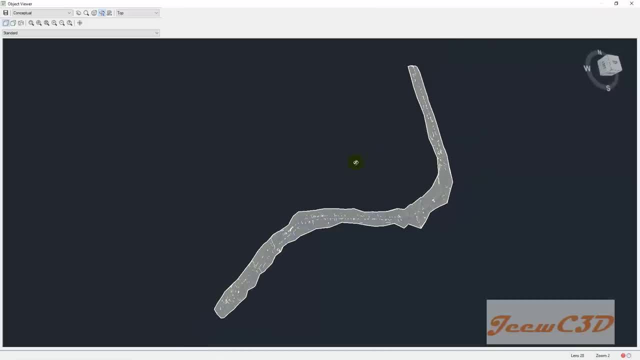 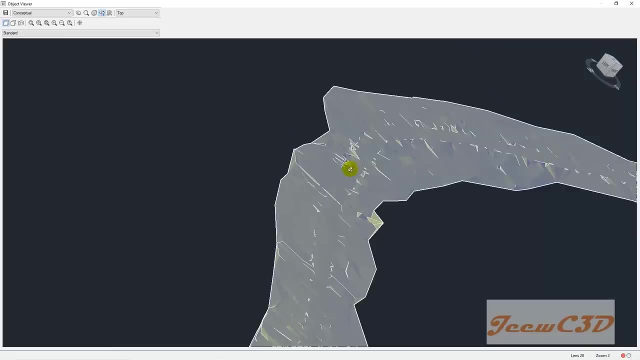 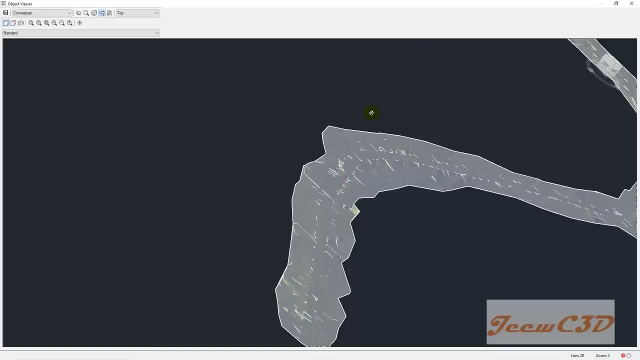 so once you just click this, let this mount somewhere here, you will see some kind of a road is going on the middle. even though it is going, you can see the road is not smooth. even though you can see a road, the road is not smooth. that is what we see at the moment when i press close here to close that one. 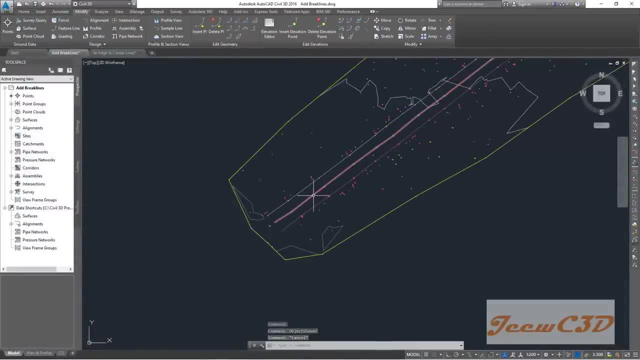 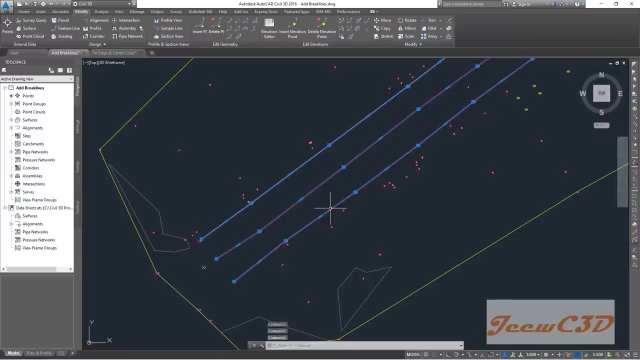 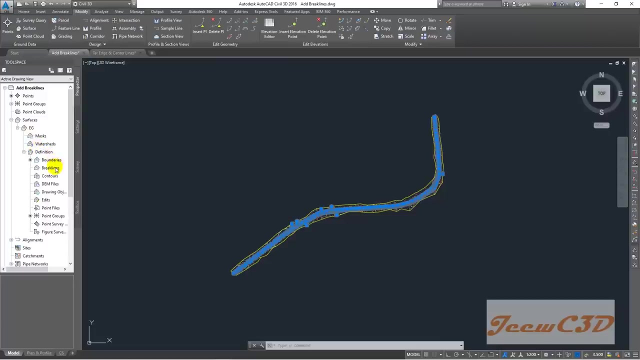 then i select these three lines. that means this red line, this light blue line and the pink color line. only these three lines and all things will be selected. then i go to prospector surfaces, eg, and then definition. as we go on earlier we click break lines, then go to add. 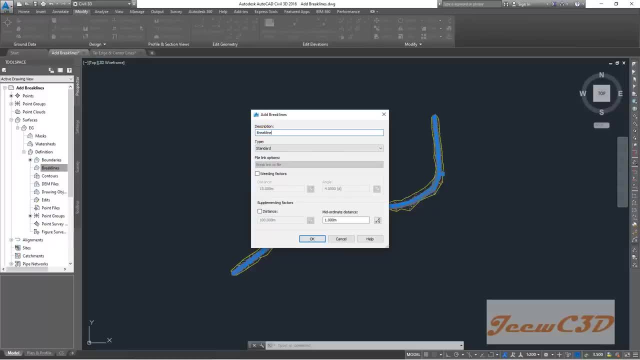 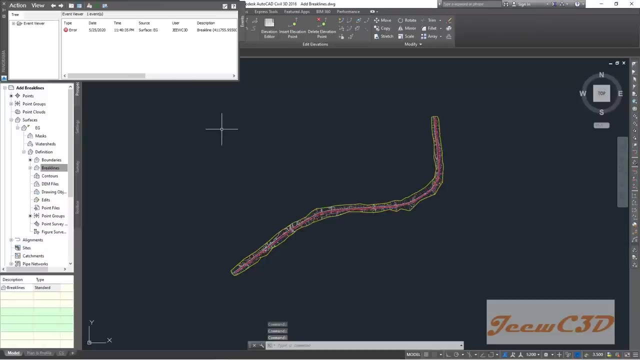 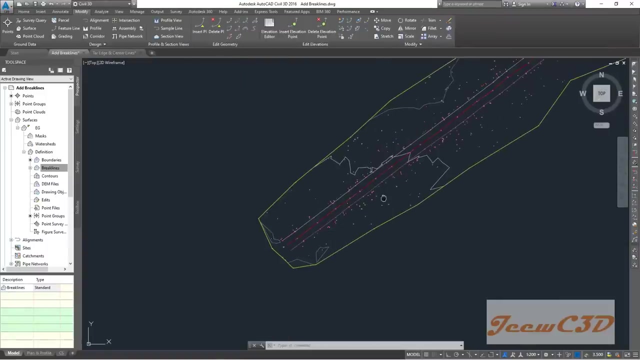 as the name, the type, break lines and your type would be proximity, and we click ok. while they are selected, there will be a small error, but you have to ignore that. so minor problem. then what i do is i click this contour line, one of the contour lines. 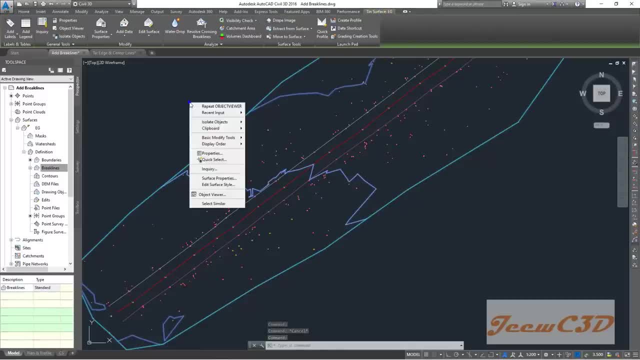 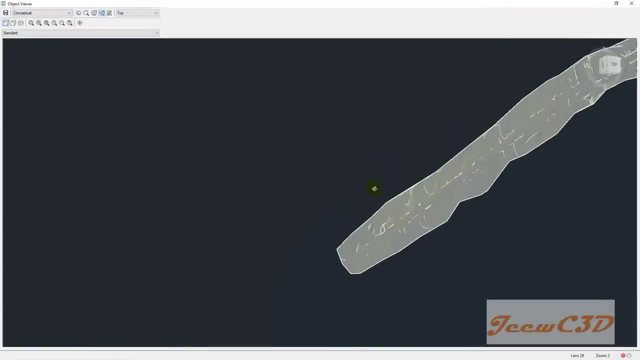 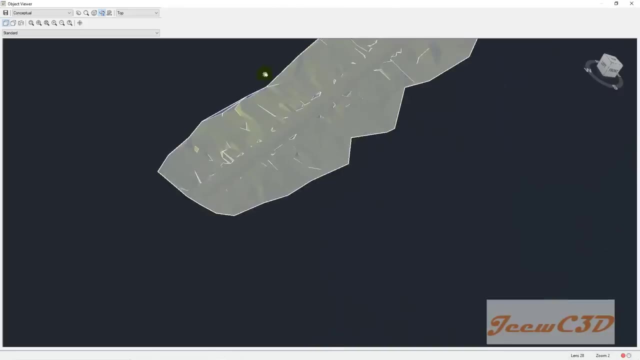 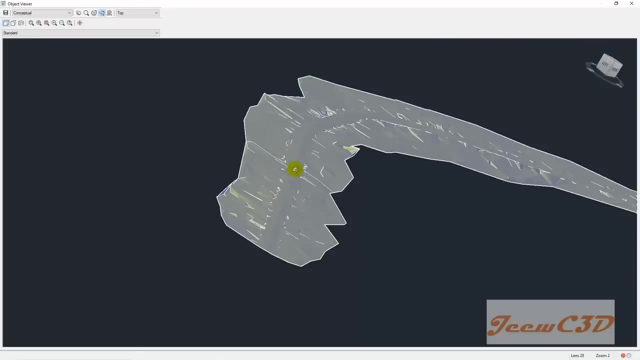 so we will be having something like this. then again i right click and go to object viewer. then i again see my drawing. now you will see a more clear road in the middle. in the initial option, your road is something not like a rough surface, not like a road surface. it is something like a rough surface. now. 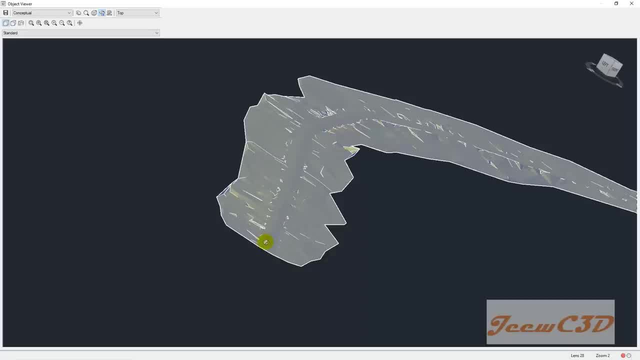 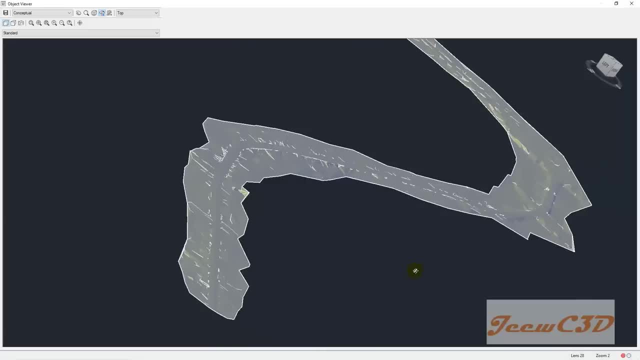 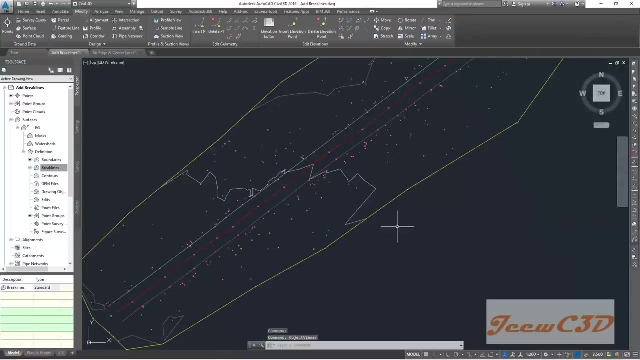 even though the outside of the road looking soft but the center of the road looking more smooth. now that is because of the option we gave by a break line. so that is the importance of break lines in civil 3d. i closed the object viewer in the previous step so you will be having this. 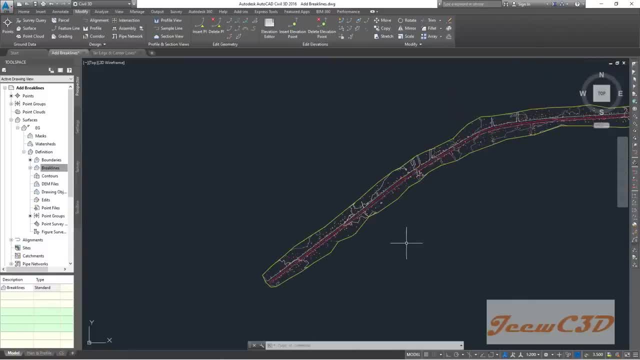 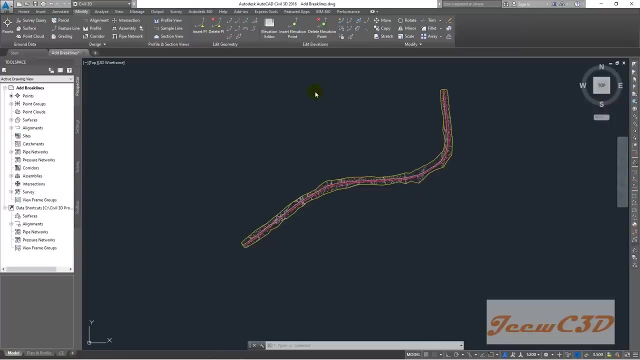 kind of drawing now. so now you know what is the importance of break lines. in the next video we will see how to export our surface into plan 3d simul. so far we have imported points and created a surface. after that we added a surface boundary. then we added break lines to a surface. 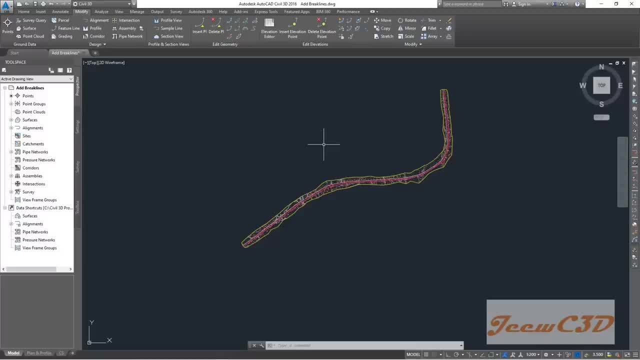 to the surface and make the surface more realistic. and so far we have done with this surface. we have completed everything with the surface. but when you are working with the surface, if you see all these point data and break lines in your drawing, it will be a burden. 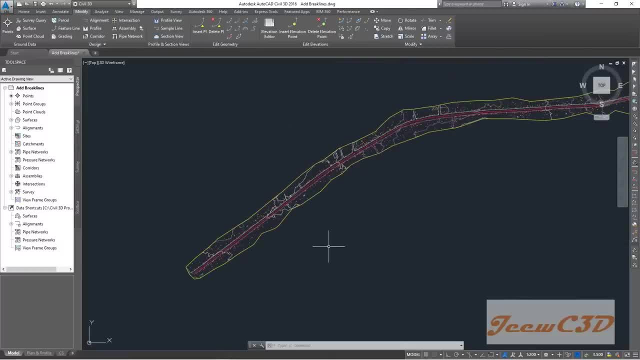 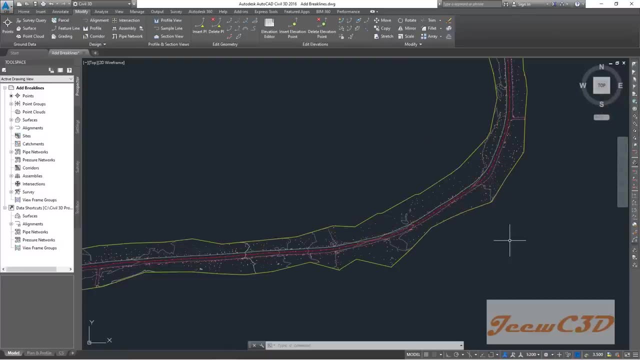 to work forward from that drawing, because you will see all the these, all these things inside the drawing and you can't properly work. so in that case, what we are doing is we are exporting this surface- something called planned XML or some other version- and make the surface more user-friendly so that we can work without much of a trouble of the 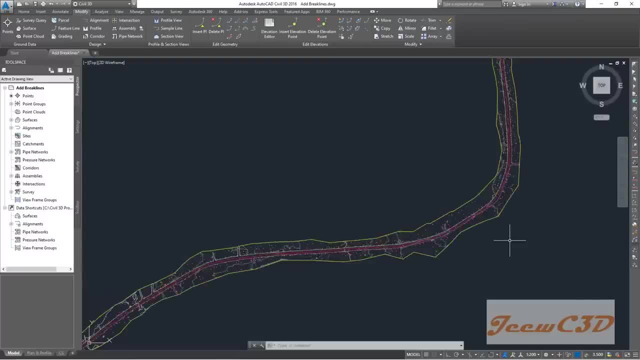 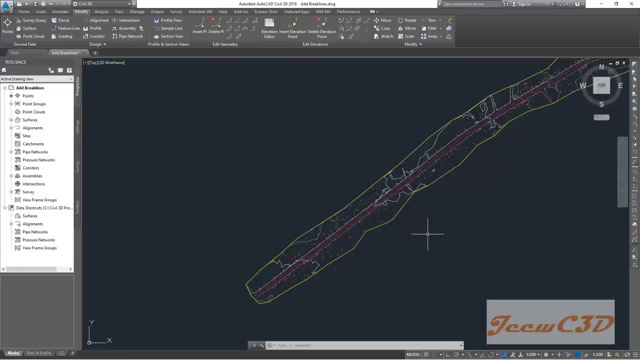 data inside the surface. so first part: we are going to export the this surface into a land XML version. that is kind of a planned XML, is kind of a file type which we use globally to transfer data. so this drawing file would be the drawing file which contains the surface would be transferred to a file type called land XML, where other 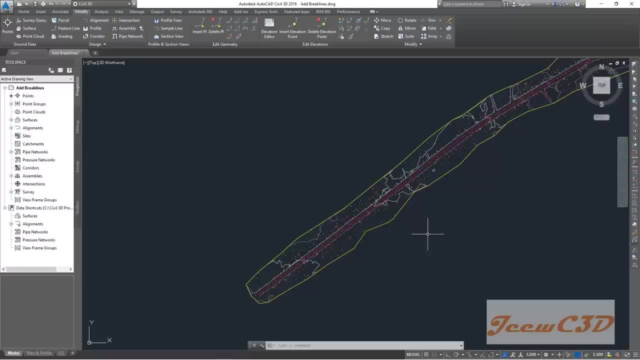 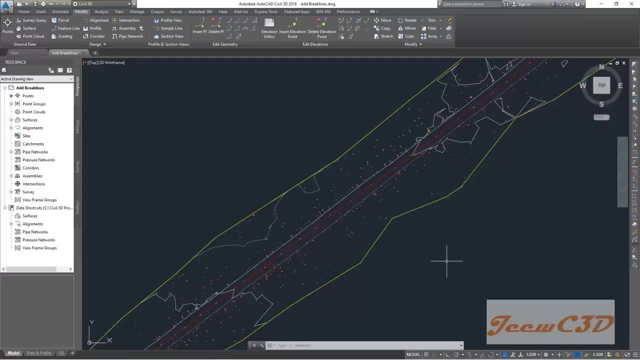 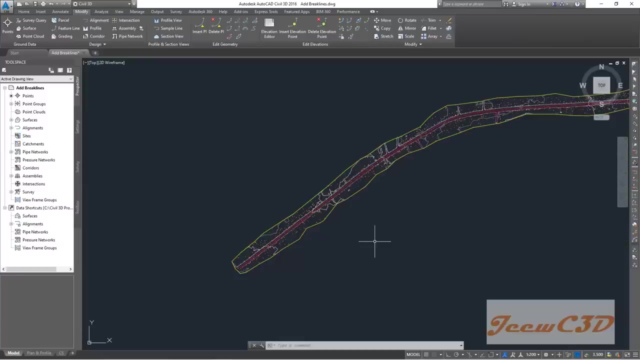 civil 3d users can use it. you can use the surface without seeing these point details and break lines and boundaries, all those things in the land XML version. what you have is the final surface only we have. it will not have the point data and work step. so that is kind of, if you remember a 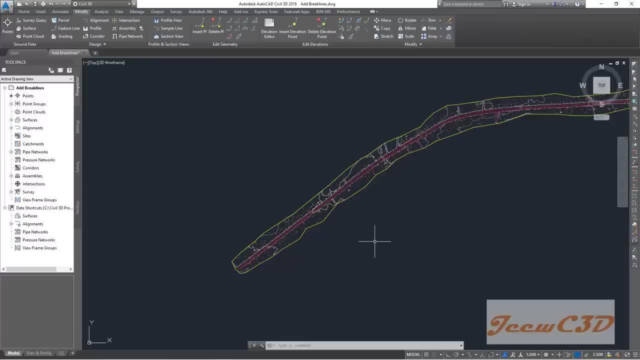 slab of a building. when you are building the slab you have all the form works and all the checks and all these other things we are using to form this slab. but after forming the slab we will be removing all those things. so by land XML also, we are doing that kind of thing. 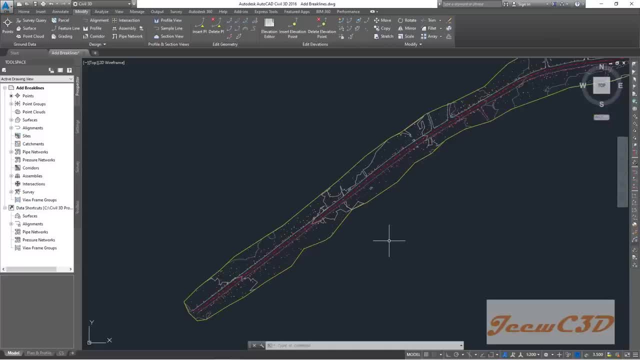 we are removing all the unwanted parts of the surface and we are retaining only the needed parts inside the surface to work with the surface more easily. so that is kind of it. you can see how easy and convenient manner so to do to export the surface into a land. 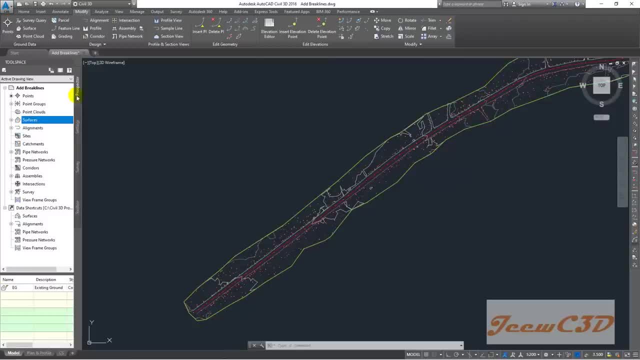 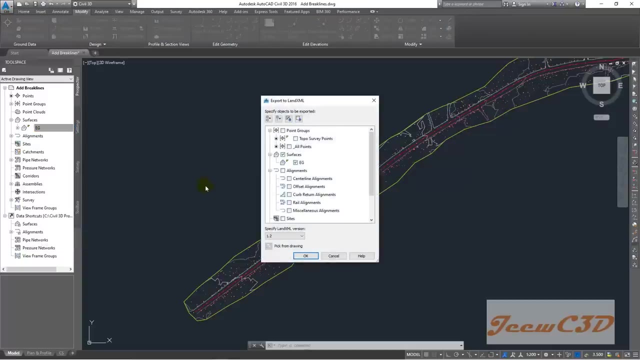 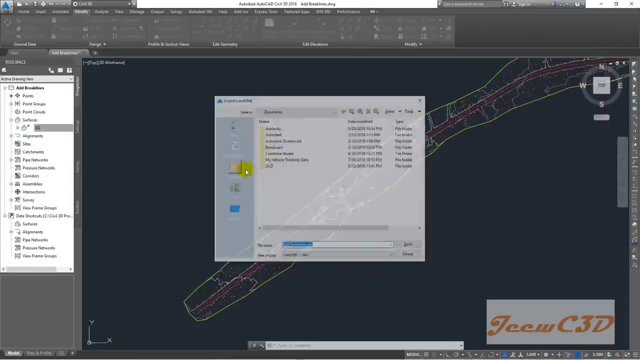 XML version. you go here to prospector surfaces. then you go to EG where your surface lies. you right click here, then go to export land XML. after that you will be seeing a check mark here- surface and EG. then click OK. then you can go to the existing folder outside. then to type the name mass EG, because your 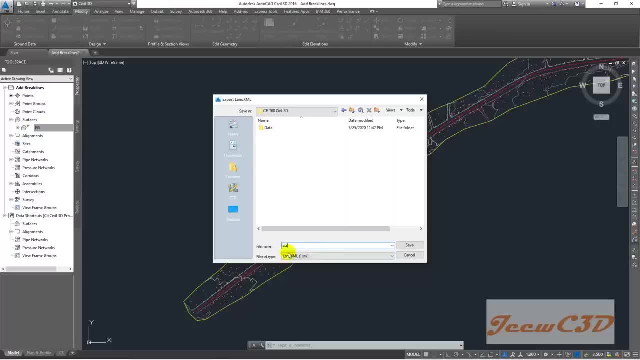 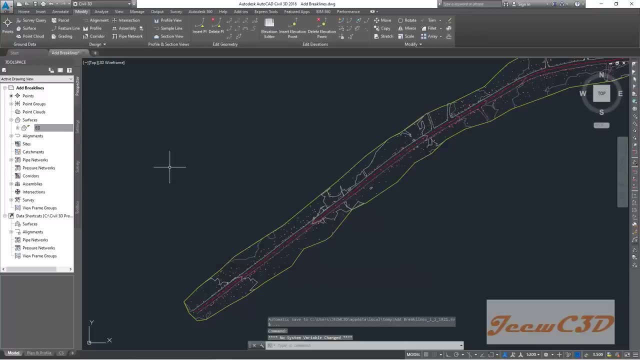 existing ground surface is there and your file type will be land xml. then click save, so your surface would be now exported as a land xml file. so that's it. thanks for watching. bye, bye. now i will show you how to export the surface into a land XML file. 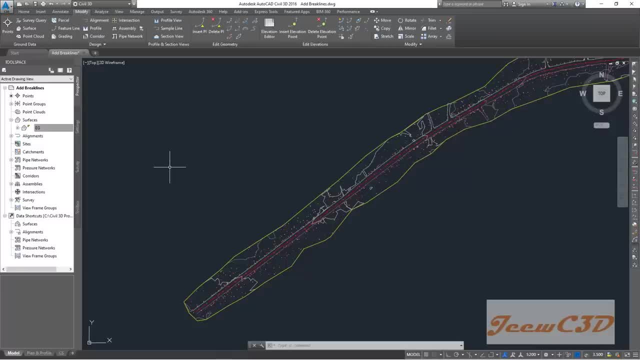 so far what we have done is import points. we add the surface, add the boundaries for the surface, add three plants to the surface and finally we exported the surface. so now we are going to close everything and from the next point onwards we are importing the exported land XML surface. that means we took the surface with the components. 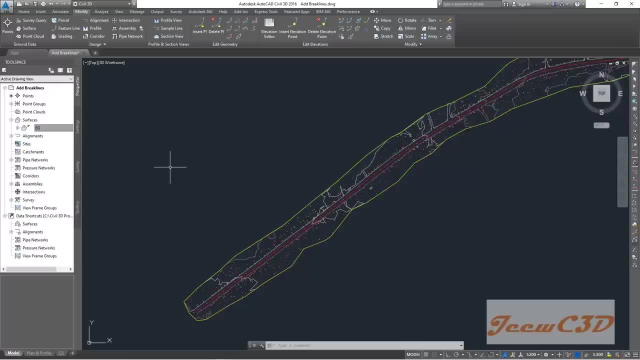 took the surface out of the drawing, then in the next video we will take it into the drawing. actually it is. it will be into a new drawing, not this current drawing. so, after exporting this, i want you to, i want you all, to close this drawing by saving it. 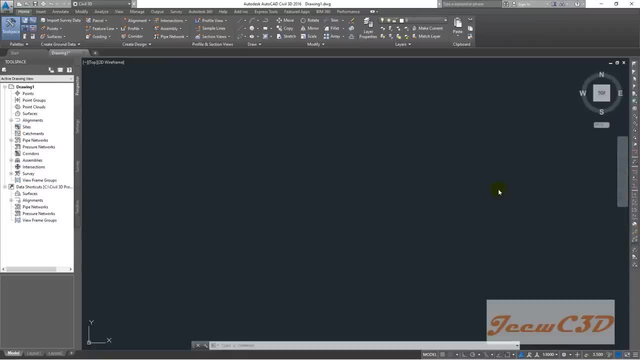 in the last video we knew how to export the surface to a land xml version, in that we created the surface from points and we added boundaries, and then we added break lines and finally we exported that surface which has all those boundaries, point data and break lines to. 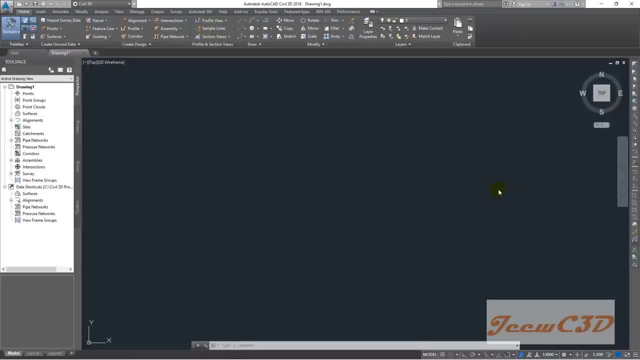 a file version called land xml. in this video, we will learn how to import that into another drawing, so do that. i want you to open autocad civil 3d, whatever the version you have. however, you have to open. you have to open the metric version. then what you have to do is you have to open a. 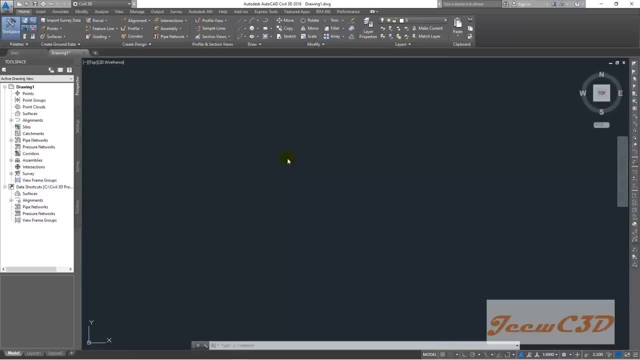 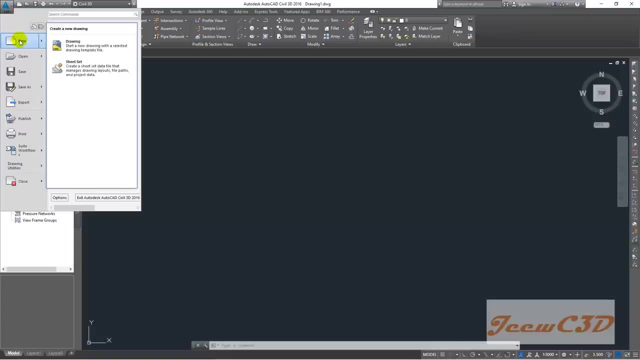 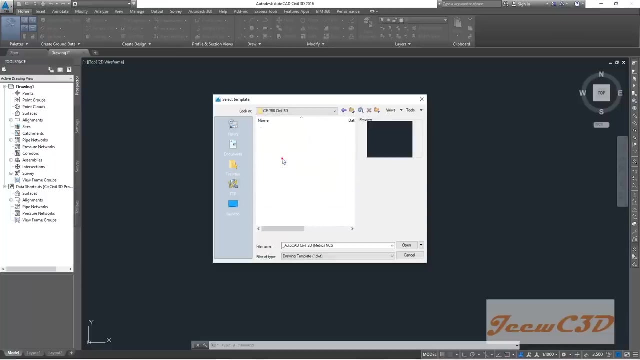 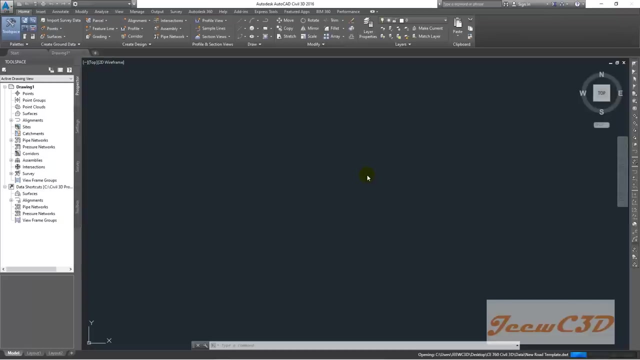 new template from the template i have given to you. so here i go, application menu browser. then go new language VDA, even heremu server here onğimyon dev console. then i'll go to the tab section inибet z1 database which is available here. this drawing hello. 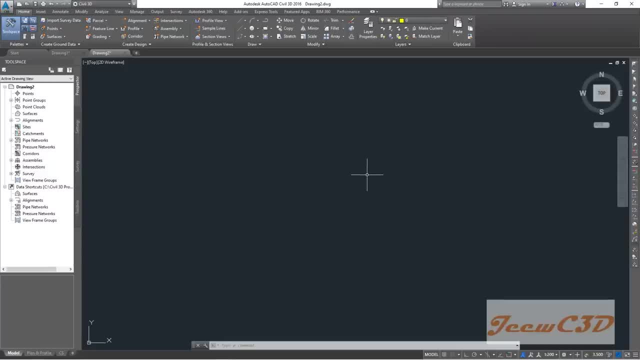 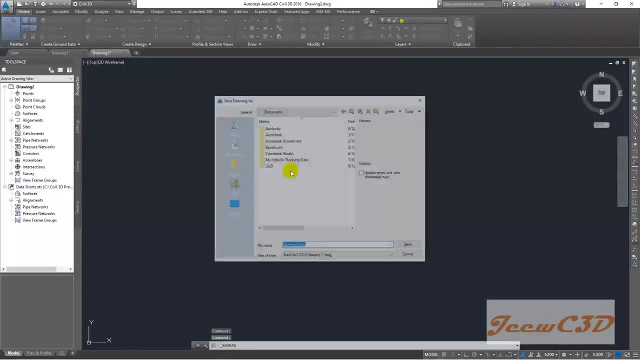 it is available in our catalog as well. i have entered name here. this is what it looks like. the version relationship is ainda skewed, so really good. So to do that, I go here, then save, as I am going to my civil 3D folder. then I save it as import and xml surface. then click save. 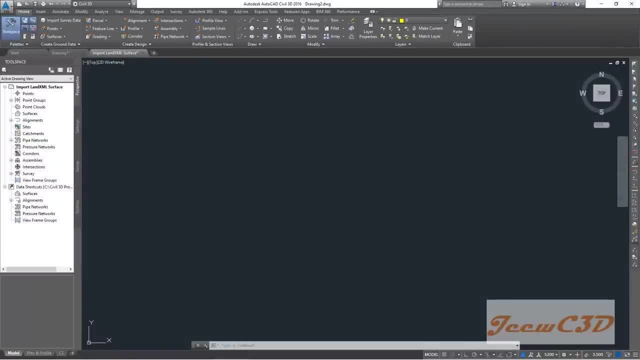 So only we have saved the surface. we don't have any data in here because we opened a blank drawing template. So since my drawing name says that import land xml surface, I have to import the surface into this drawing. Import means we are getting something. 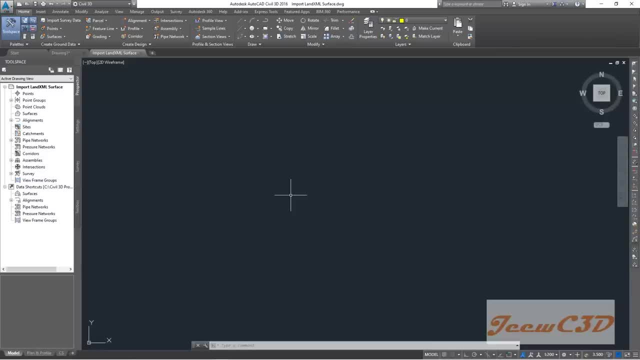 We are getting something from an other source, So that source is a land xml surface. So to do that, I am going to this insert tab here in the ribbon, insert tab. then you have land xml. Depending on your version it may be different, but the view may be different. but you may find in the insert tab land xml. 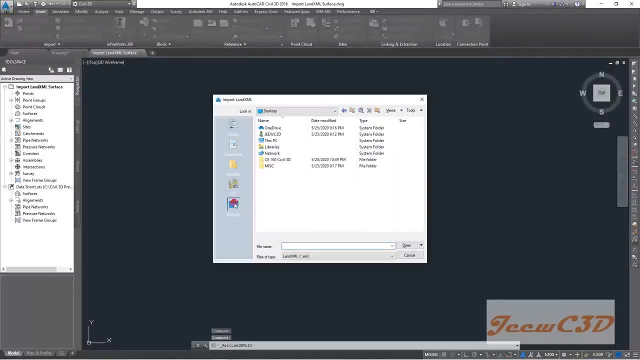 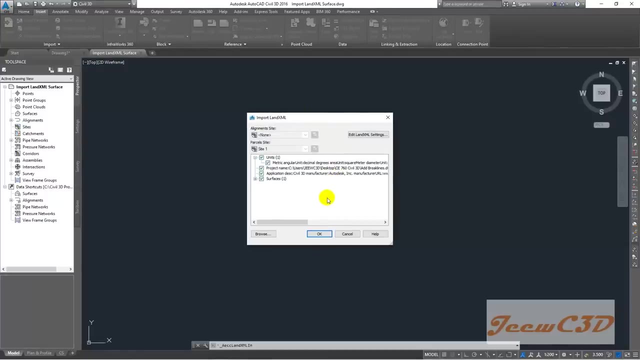 I click here, Then I go to my desktop. here I save that land xml file called eg, then I select it, then click open So you can see a small window appears. You don't have to do anything to this, Just click ok. 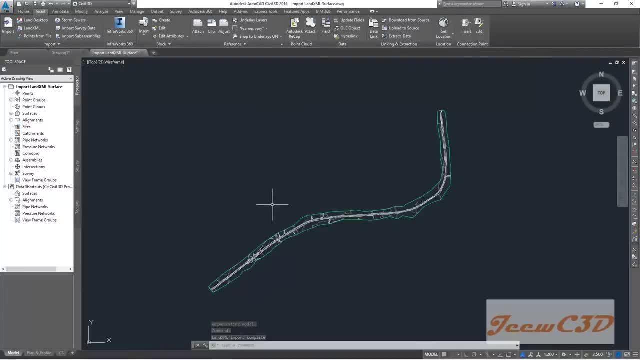 Now our surface will be appeared. in this drawing You can see the break lines are appeared in white So that you can get an idea where the break lines are. But they are not necessary to this surface, So you can delete these break lines. 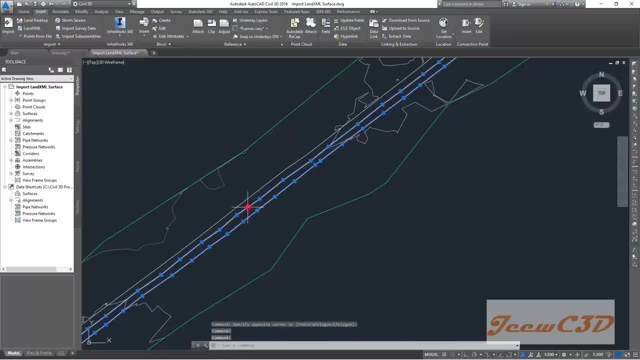 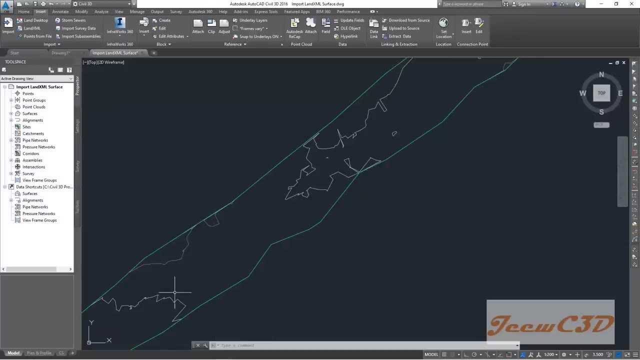 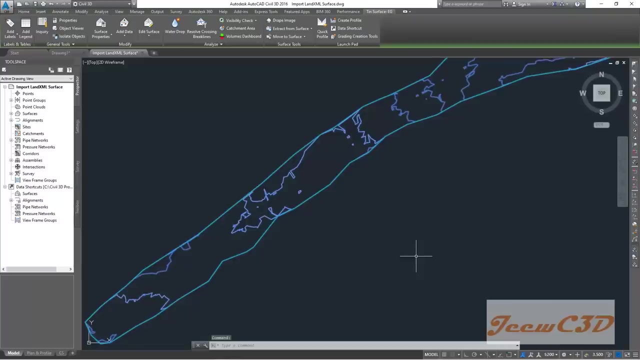 To delete them, you just click them and delete. Press delete on your keyboard. You will see now those lines are disappeared. These lines are actually contours. You can't delete them. So once you select these lines, you will see it appears as thin surface eg. 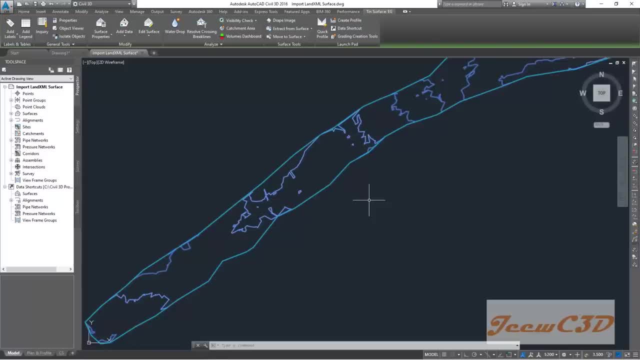 That is. that means it is selecting the surface. So currently the surface is viewed on contour. You can change the view of this Before changing the view of the surface. you can see my surface is still selected. I press escape to deselect the surface. 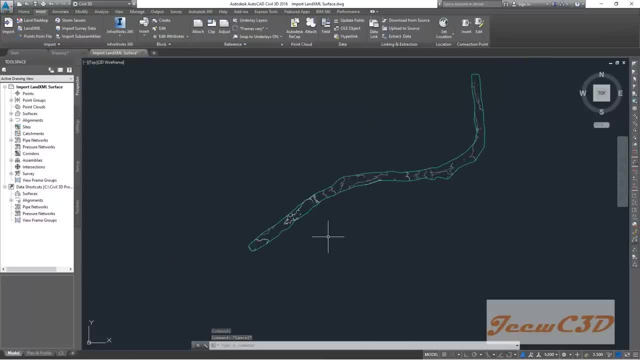 So it will not be selected anymore. So you can see, now there is only a surface. You don't see any boundaries, as we applied earlier, Or you don't see any point data here. So this is the most simple way. 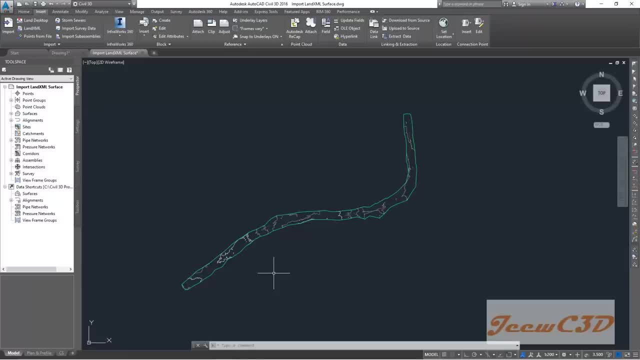 Simplified surface. You must know you can't. Initial surface was a kind of complex surface Because you have all the way You have the point data and you can't see them clearly. You can't see the surface clearly, You have point data all the way. 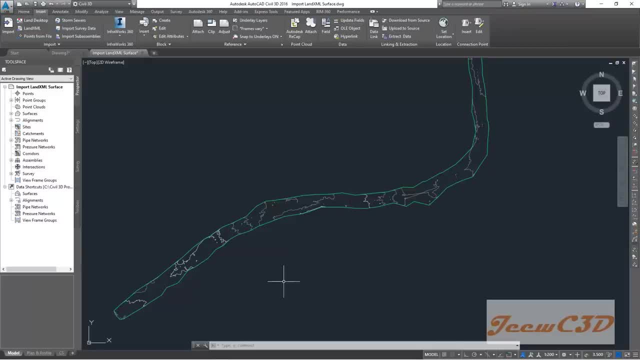 So this surface is kind of a less complicated, A simple surface Which would help you to work with very easily than the previous surface. So that is why we are using the LandXML conversion to create less weight or lightweight surfaces. Now I am going to change the style of the surface. 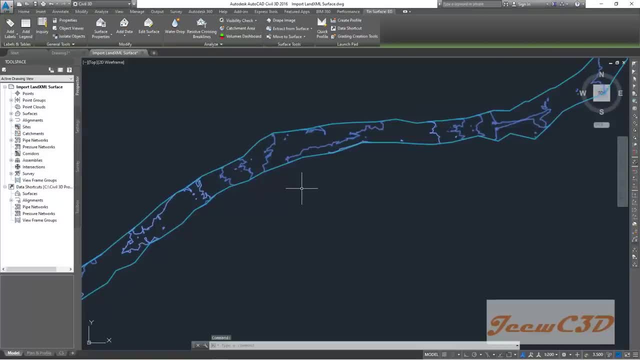 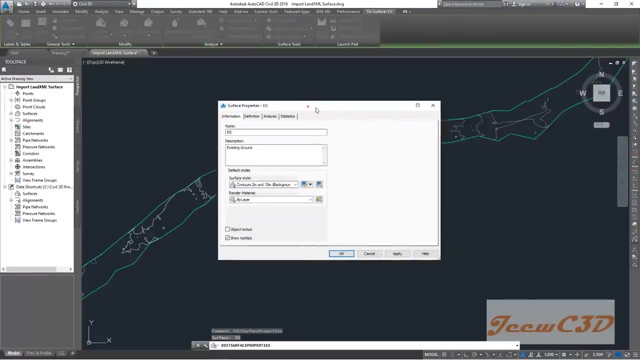 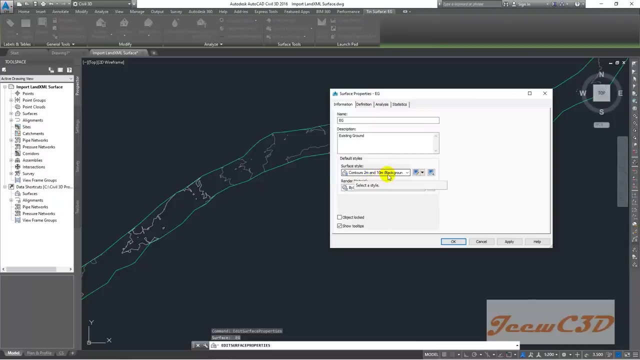 To do that I click here, Then right click on my mouse button, Then I go to surface properties, Then I go to information tab here Information tab, So I can change the style here. Surface style. Currently it is contour 2 meter and 10 meter. 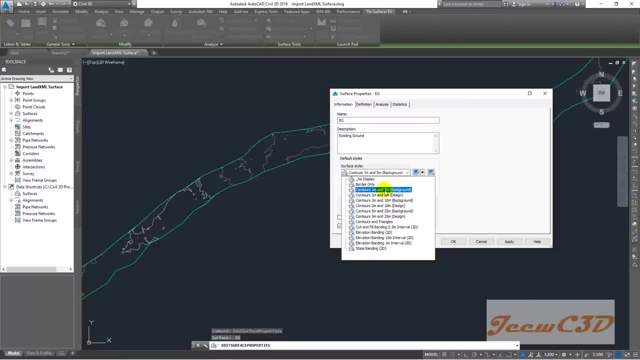 So you can change it to contour 1 meter and 5 meter. Then you click apply, You will see the changes here So you can use other design types and apply And see how they works. So this elevation banding is elevation. 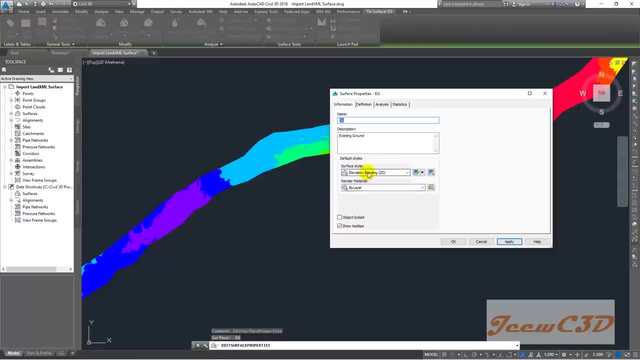 The surface is colored, of course, into the elevation, So the slope banding is elevation, So the surface is colored according to the surface slopes Likewise. So for the moment I will keep this style as border only, So that we will see only the border of the surface. 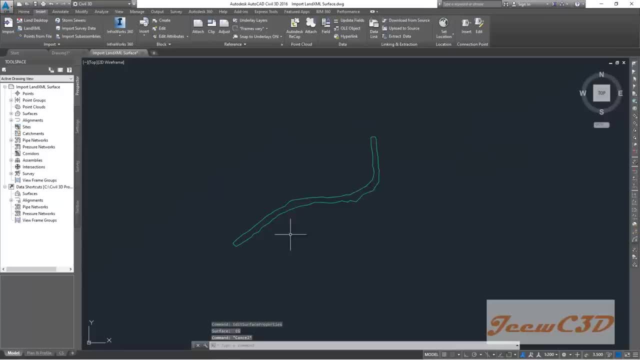 So now you will see only border of your surface. So that is how you import a surface To land xml. In the next video we will look at how to create an alignment in a inside this surface To create a new road to our project. 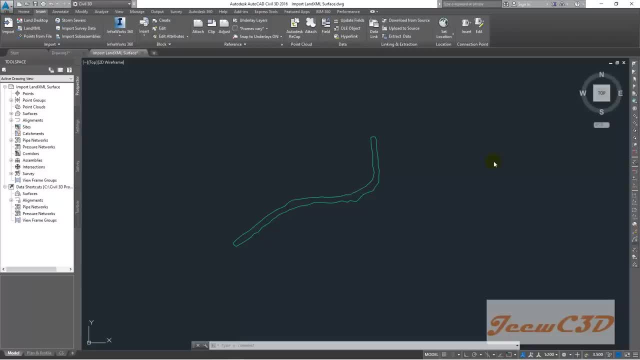 In this video. what we are going to do is We are creating the background to generate or create an alignment within this surface. So before that, I have to tell you, We are still on the import land xml drawing. So we created, imported the surface and we set the surface style to border only. 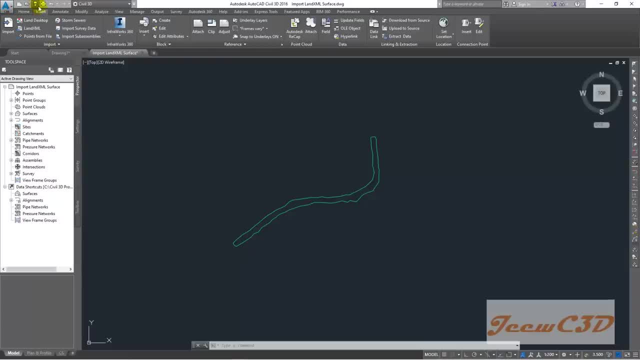 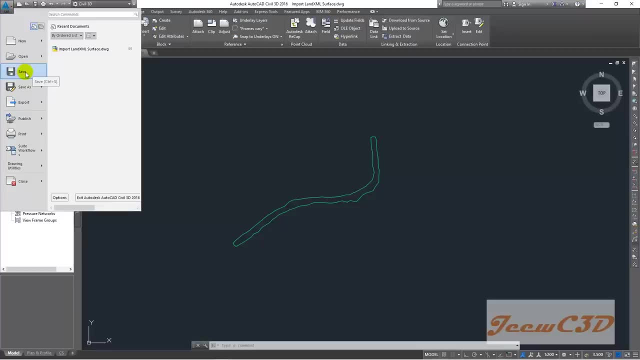 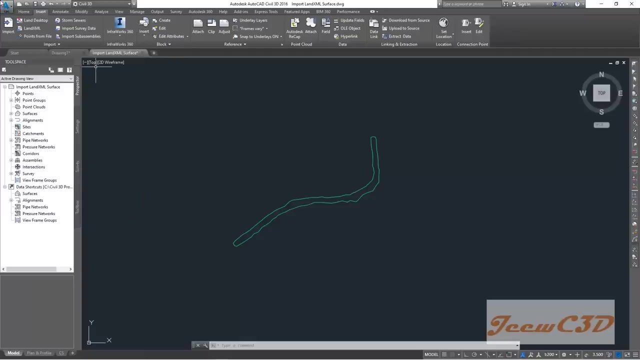 But we haven't save the drawing, So I will save the drawing from here, Or otherwise you can do it from here, And initially we used save save as option. now, Since we are in this drawing, we will use the save option. 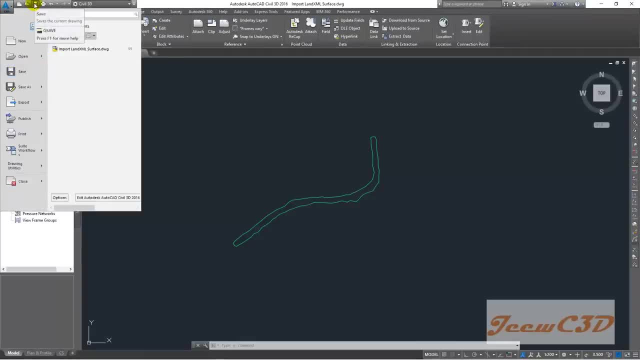 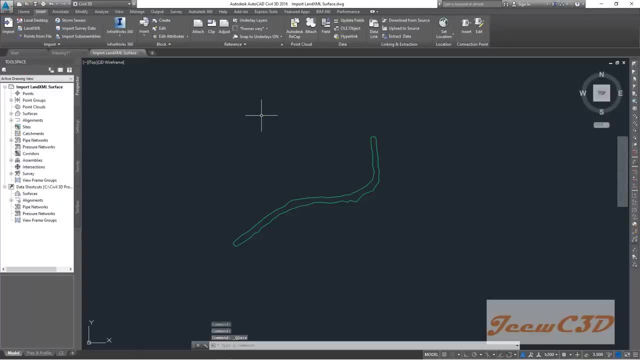 You can use this option, Or else you can use this option: save So I will use it here. Save So this drawing will be saved. So in any time, If you want to exit from the drawing, You can save the drawing and exit from the drawing. 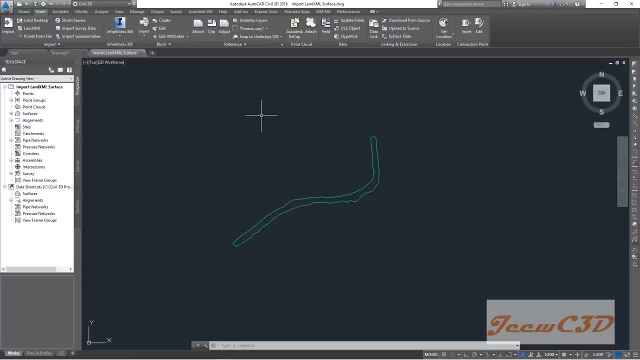 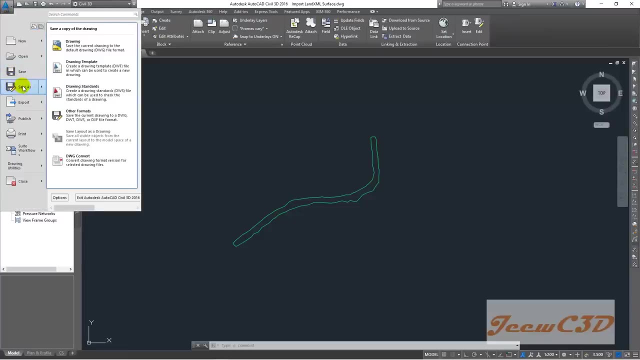 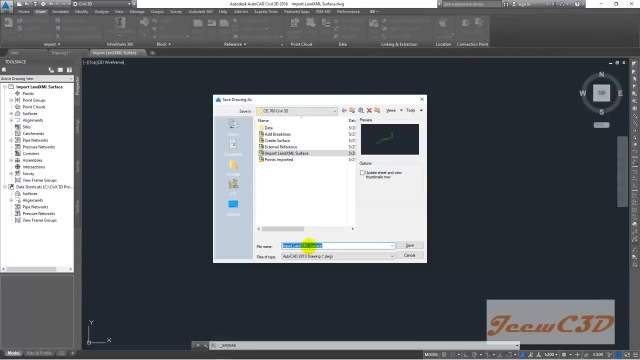 And reopen the drawing in a later time. So, since we have saved this drawing, I will save as this new drawing. Save as this drawing for a new work. That means to create alignment, So I rename the drawing as create alignment. 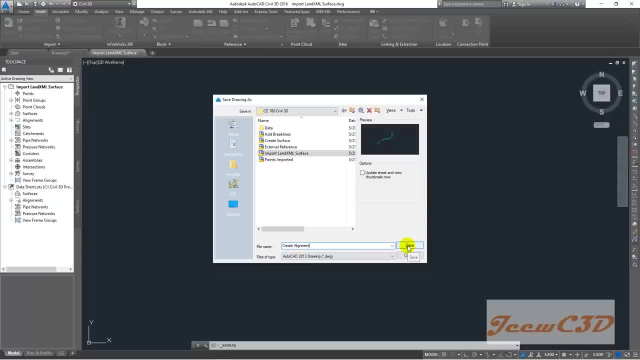 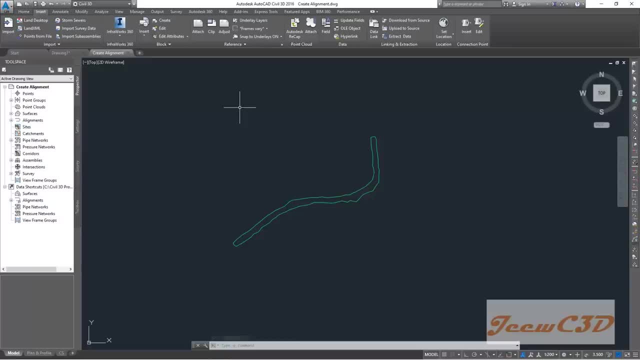 And click save. So now, in this drawing, what we are going to do is We are going to create an alignment Right Now. before creating an alignment, We want to know the topos. We want to know the topos. survey of this area. 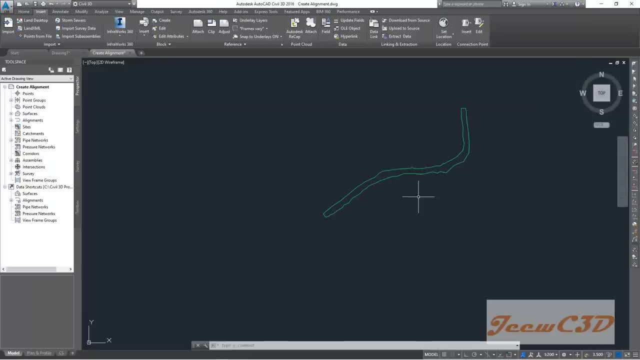 Even though we have a surface, You can't see any topos survey details. So to get that, We want to external reference the topos survey As we did in a previous video. So to do that I will type access in here: 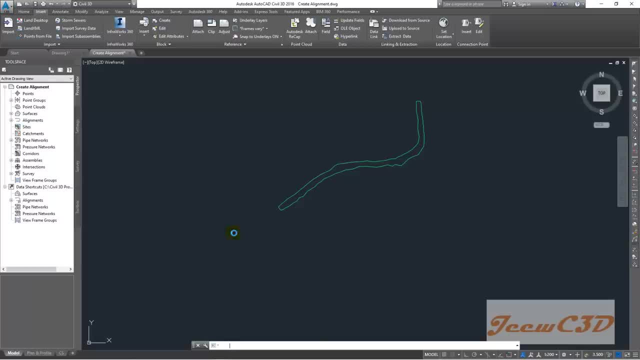 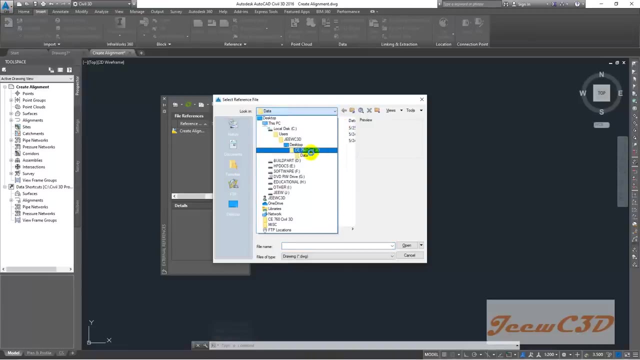 Then press enter So the access manager will be open From here. I click the drop down here And go to attach drawing. And in my data folder, In the CLTB data folder, I have topos survey drawing. I will select that. 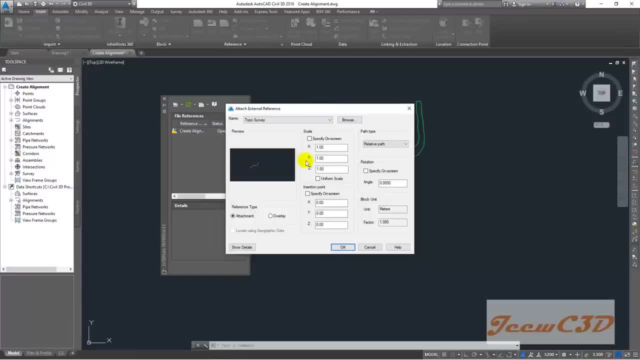 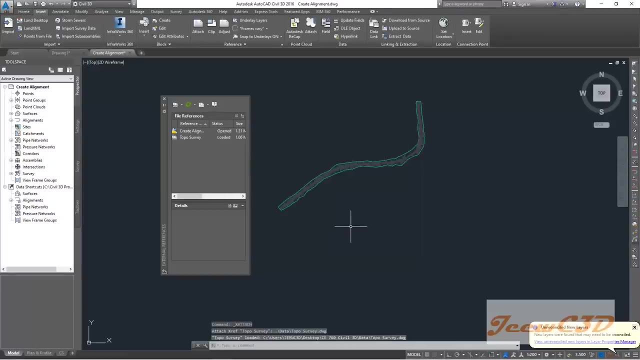 And click open to access the drawing. So make sure you don't have- So make sure you don't have any of these Options saved. They should be unchecked And you have to click ok, So your survey- Topos survey- will be appeared inside the surface. 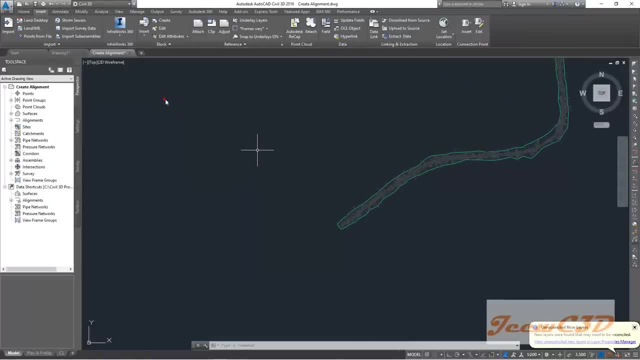 So I will click this one And close that. So what we have to do is You have to create an alignment Between this surface, This surface here, Because that is the area We have the survey data. Currently, we have existing roads. 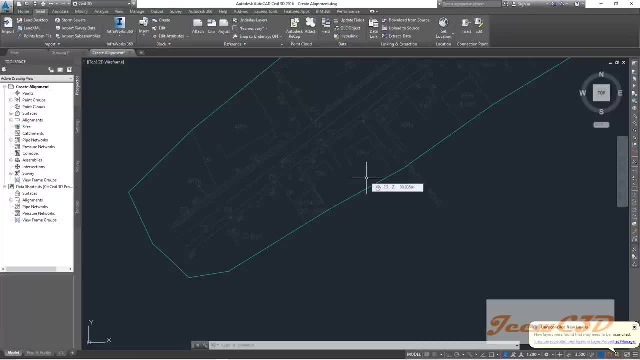 Within this survey area. So what we are going to do is We are creating an alignment Very close to the centerline of the existing road. So the centerline means this line. You can see Throughout the drawing. You have the centerline. 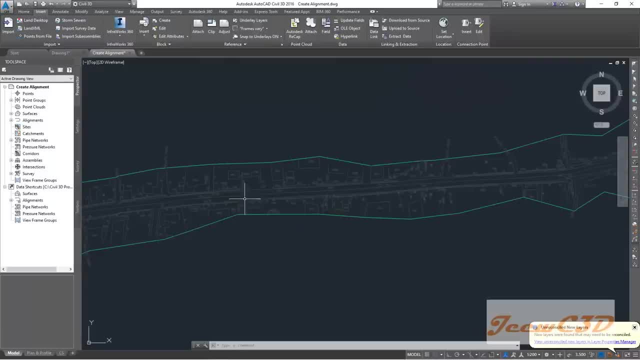 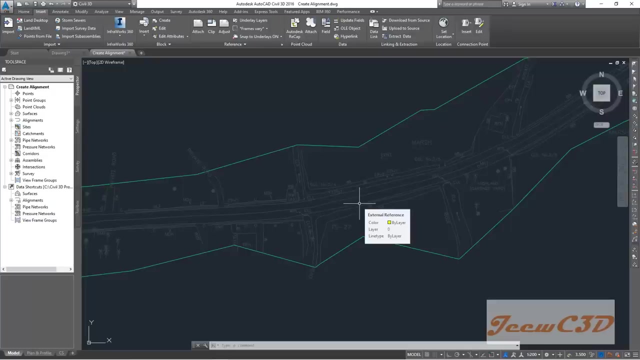 So what we are going to do is We are going to create an alignment, Thinking that To coincide with this existing centerline. We cannot 100% coincide this thing, But we can make this as same as possible. So. 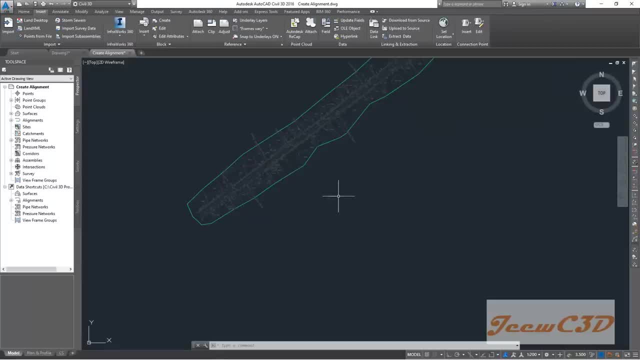 When you are creating an alignment, You need to know What kind of a road you are going to create Or what kind of a road you are going to design. Those data should be given to you, Otherwise You don't know What kind of the data someone needs. 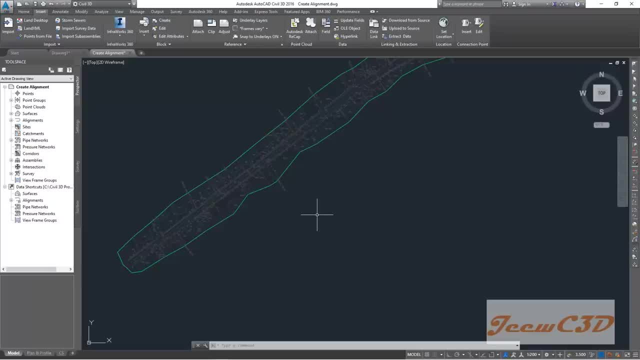 So You have to request that data From the person who required the road From you. In this I have prepared a small data sheet Where you have the road data, So I will show it to you So that you can get an idea. 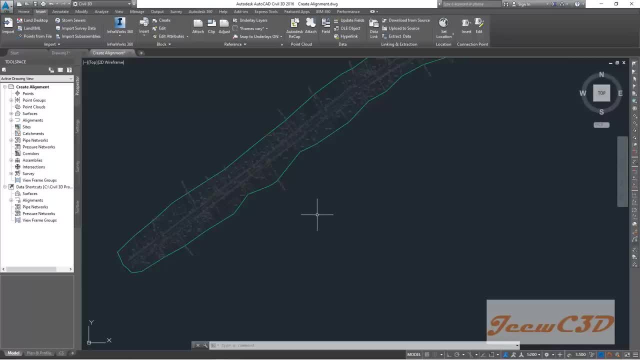 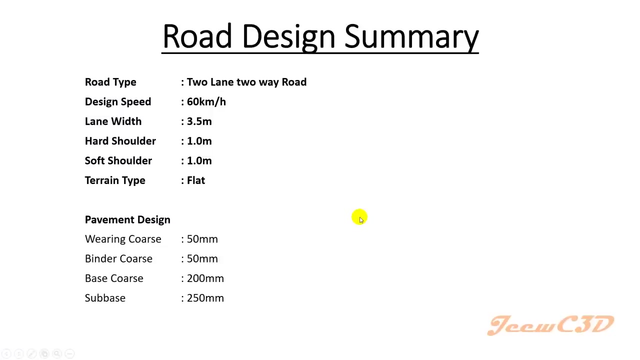 What kind of a road We are going to design In the next few minutes of this video. Thank you, Bye Bye, Bye Bye. So This will be your road design summary. You have to design a road Which is a 2 lane, 2 way road. 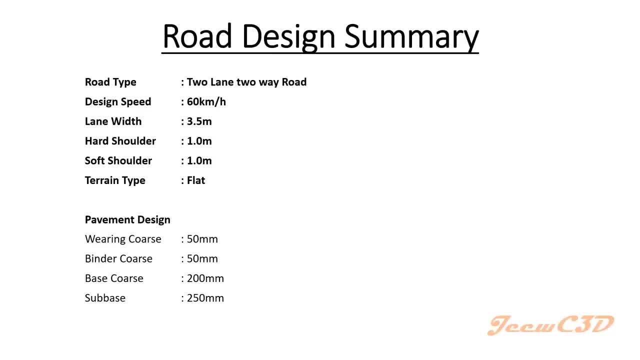 So 2 lane, 2 way means You have 2 lanes And One side for One direction, The other side for Other direction. That is What we call 2 lane, 2 way road. So Your design speed should be. 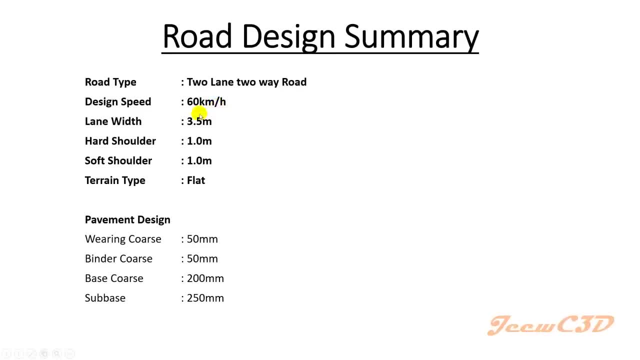 60 km per hour, Then your lane will be 2 lane, 2 way road. So In your lane This would be 3.5 meters, Hard shoulder Would be 1 meter, Soft shoulder Would be. 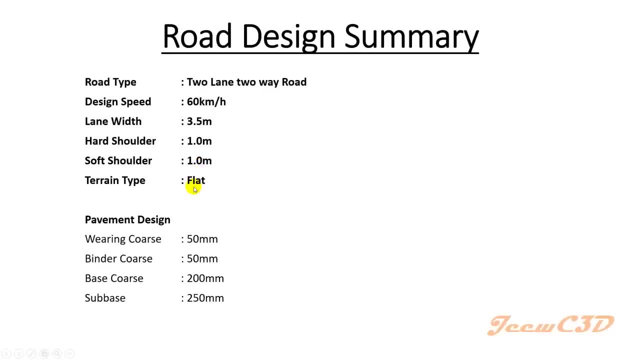 1 meter Terrain type Would be Soft flat terrain And You have. I assume That you have to Do this Like a Local RDA road, 2 lane, 2 way road, So You have to use. 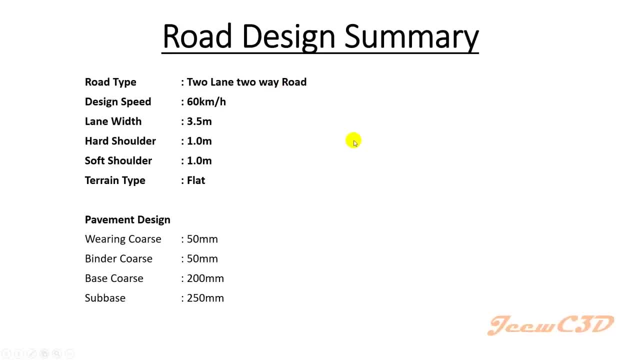 RDA design guidelines. You have to follow the Local RDA road 2 lane 2 way road. So You have to use RDA design guidelines To create This road. So When creating The road, 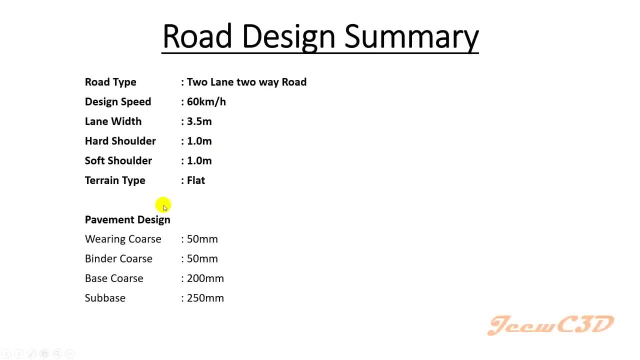 You have Given The Payment Design Thickness. When you There is a Part, You need This one In road Designing, So You need This payment Design Value. It is Given. 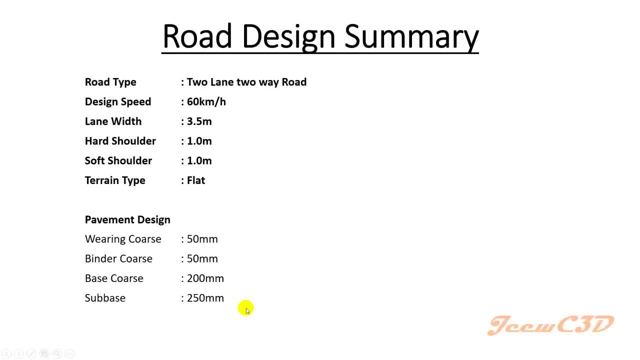 As Wearing Course A: 50 mm. We will be Going To use This data Later In the Civil 3D Video. Now We will Move onto The drawing. Again, You. 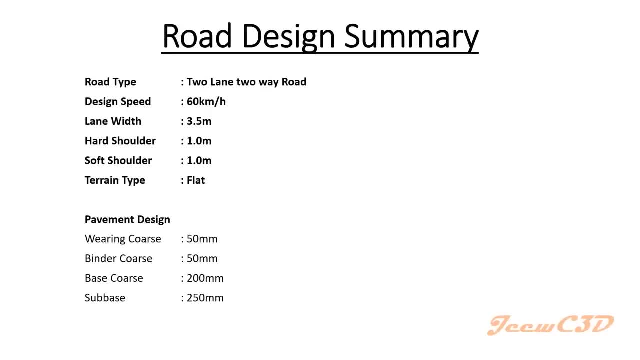 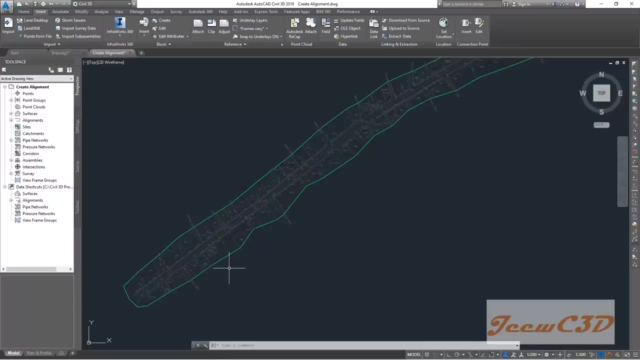 Have To Remember That We are going To Create A road Which Is 60 km Per Hour. Design plane with 10 arch holders applied here. so now i am again inside the drawing. now we are going to create an. 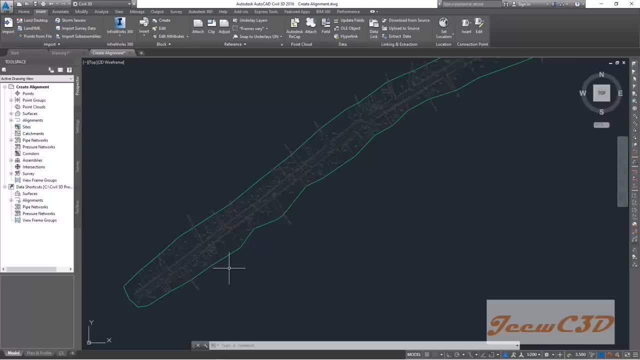 alignment. but before that i have to tell you you have to do a lot more things if you are doing, going to do a real world example, because you have to go to the site, you have to identify the constraints and identify the key locations and you have to place the alignment to satisfy all those needs. but 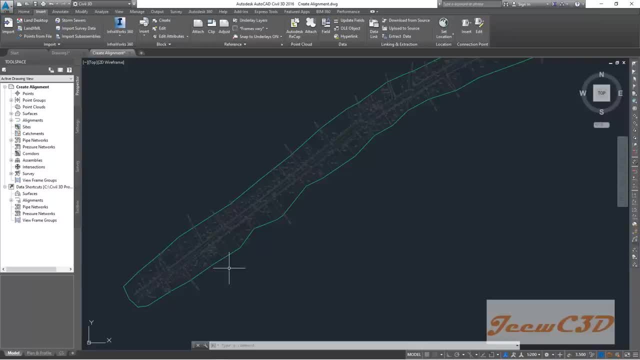 here. what we are going to do is we are just looking at the topos array and place the alignment for the sake of this exercise. now to create the alignment you have to go to home tab. then you have this alignment here- who they are. click the drop down. go to alignment creation tool. 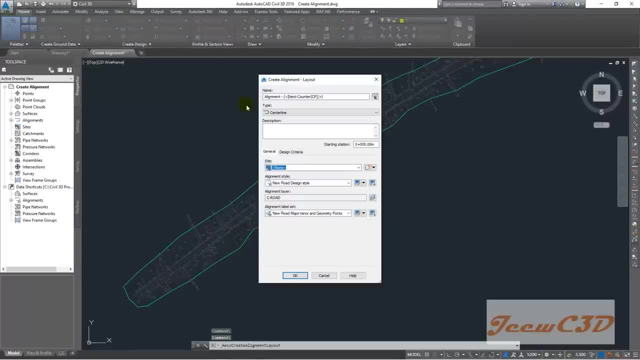 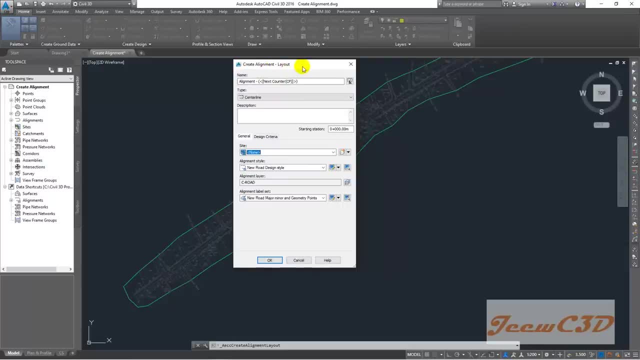 alignment creation tool. click that, then a small window will be appearing. it is create alignment layout. so the name of your road would be, let us say, design road. then for the different type would be centerline for the section. let us say two lane, two way road. then again you can say ldp. this equals 3.5. 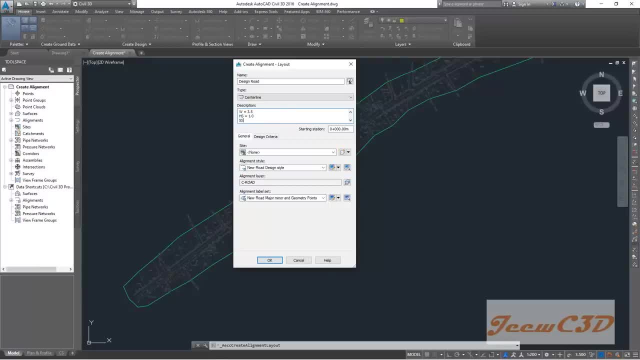 arching equals one meter and top shoulder equals one meter, if you like, otherwise you can just make this blank. so your starting station would be zero here. so if you are designing an existing road at the middle of middle section of the road, so if the if the station or the drainage of that location or the length up to that point, 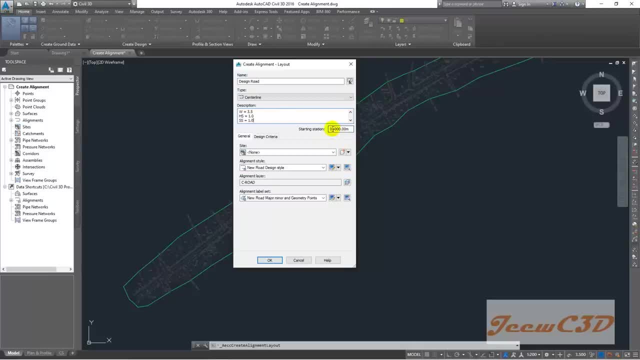 is, let us say, five kilometers. you can start from five here, typing five here. so these are given in thousand which you will have to use. so if to go start at fifth kilometer, you have to just type five here, five plus zero, zero, zero, to indicate five kilometers. so at the moment, we see, we think we are, 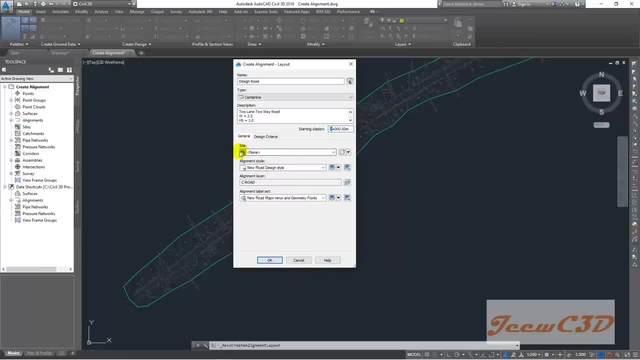 starting from zero station. now you don't worry about grown, you don't have to worry about the site condition here. what you have to do is get this alignment style, which should be- should be new road design style. then alignment labels that would be new road alignment minor. 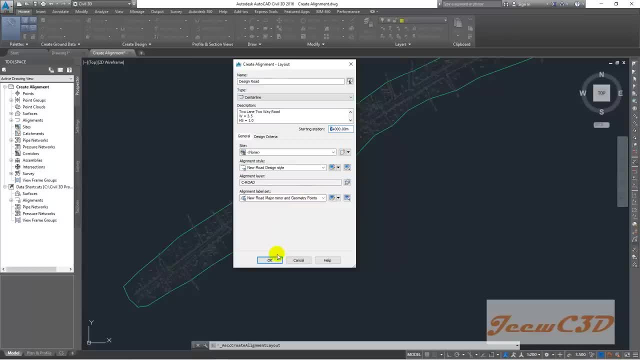 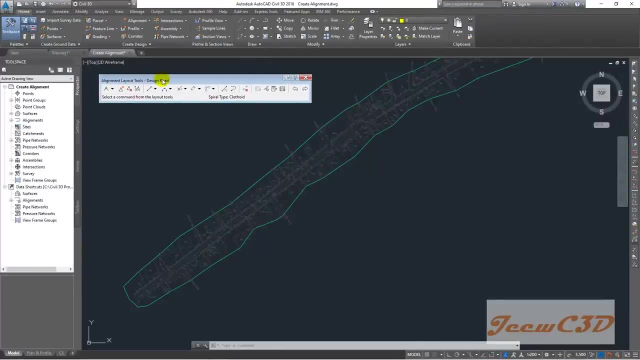 nature, minor and geometry point. then you have to click ok, this kind of a small toolbar will be appeared here. so then what you have to do is you have to create the road according to the existing center line. we are trying as much as possible to follow the existing center line. so what i am doing here is i am going to identify the straight sections. 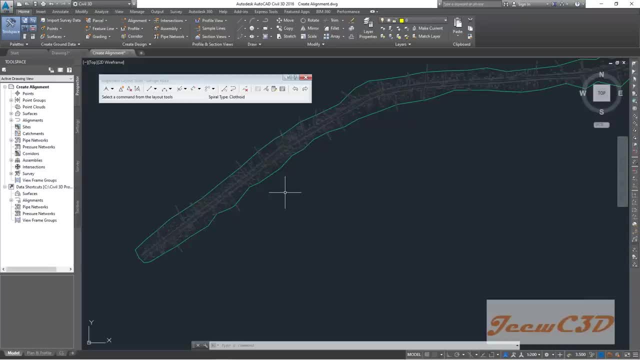 first and create curves in the middle. so first i come here, i draw six line, two points. six line, two point option, again this line, two point option. then i go here, i place the mouse close to this center line and i click. then a line would be starting to appear. 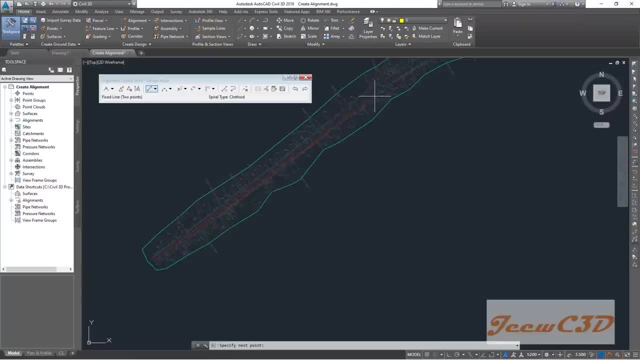 then i drag the line until it is going to be very much straight, so i will stop somewhere. here i have one part of the trait, so it is okay to have them here. and one more thing i have to tell you. it seems like this is very small, the stations are very small, so you can do one, one thing you can. 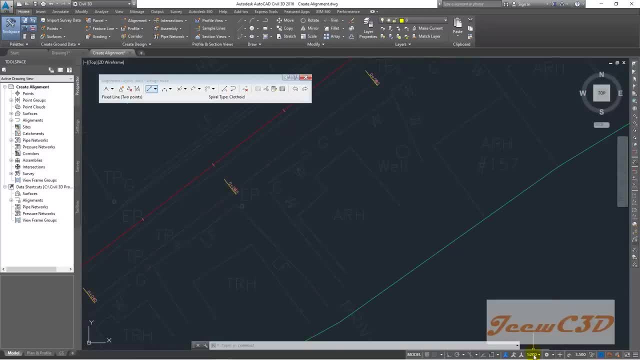 do is you can change the scale. you can change the scale here. usually we are working with the scale of the pages and pieces. so one, two thousand, one in two thousand for you. then we get a more, uh, viewable view of the drawing, that guidance, these labels getting more clear now. now i have create one section of the road. sometimes if we go outside, so if you think you need to change it, you can quickly go inside. you probably also change it. so if you- I speak here language, but i will get aiming it to two edges. so if you think you are you need, then when you change it, you know what my position, which i am going to 봐put in every. 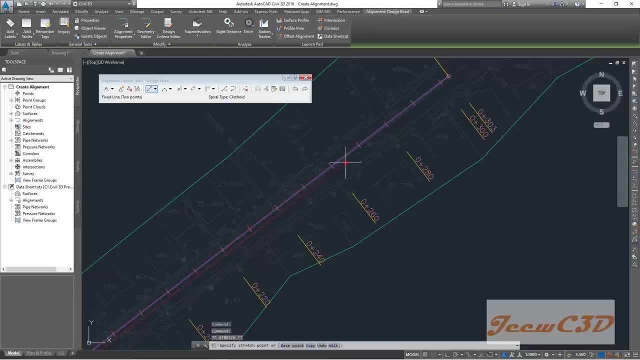 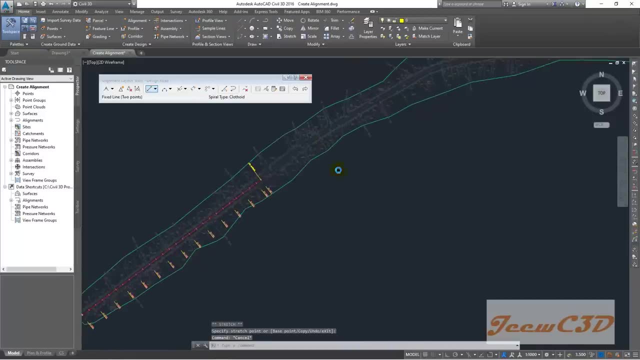 One move to middle. Here you have more. we have to follow it one by one. so now J1, the middle. it is a basic, so this is a minor. I assume you have sort of a class dropdown. so by projected protection just drag it here and you can change it like that. so it seems like you have a curve in this area. 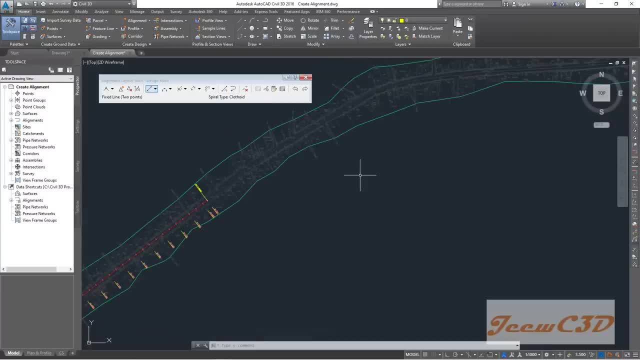 and a straight in this area. so what i'm going to do is i'll create another trace there. yeah, i keep like that the trace. okay, now i have to place a curve in between these two trace. i have one shape here. i have one shape here, so i will be placing a. 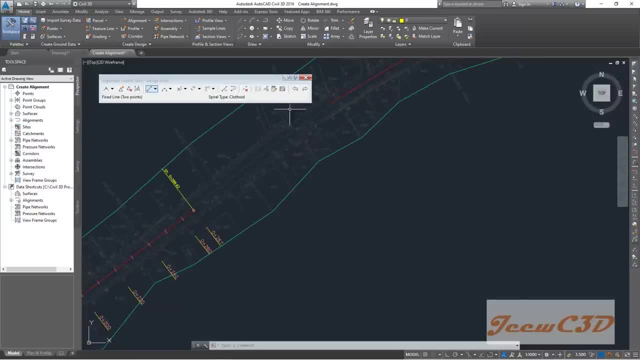 facing a curve hitting this area. so i go here. then i go to this option, free curve, select between two entities through point. i click that one. then the command bar is asking: select first entity. that means the select, select first part of the road. this is the first part. then it is asking the 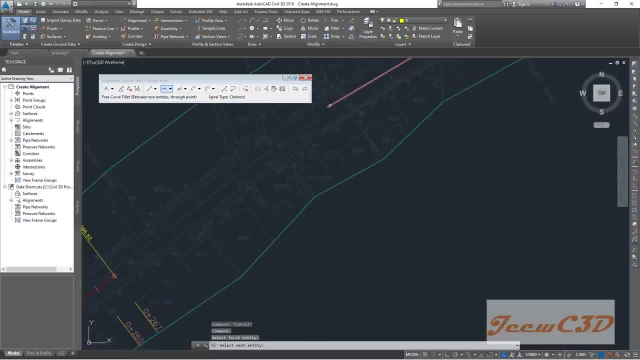 next entity. next entity would be this one. then i have to click here, so i have to move my cursor. you will see small curve- blue color curve will be appearing somewhere when you click the mouse button. so once it is okay, you press enter. so if you feel this should be, 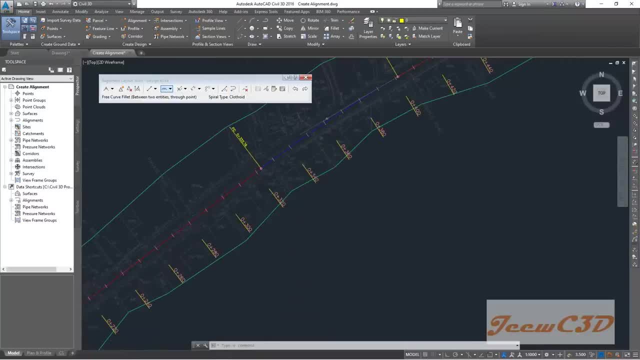 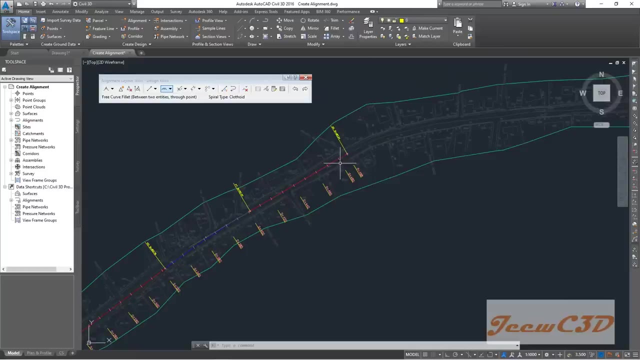 okay, somewhat, you can even do the changes after the alignment is created. so far we have created straight, then a curve, and then, uh, another straight. you can see. see, the labels of the road are automatically placed along this alignment. So it is starting from zero. up to this point, we have a road about 488 meters long. Again. now I am going. 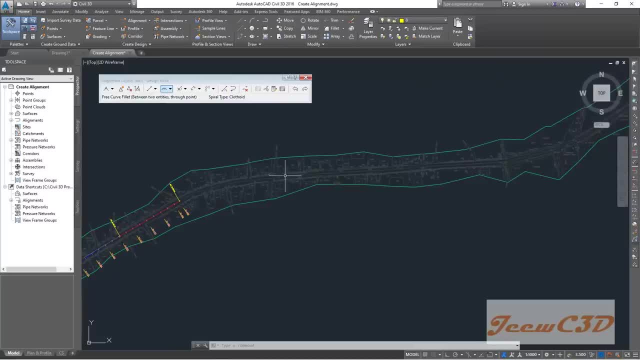 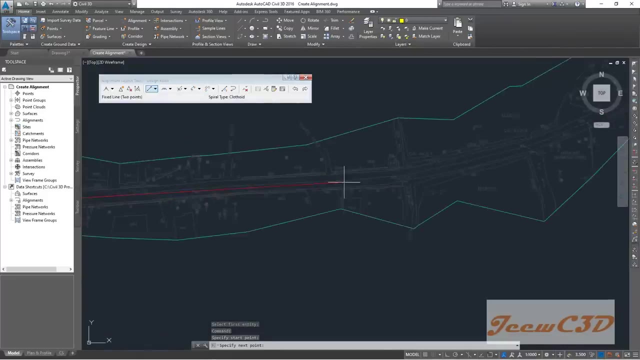 to create a new state which I can see it from here to here. So I go to this option. it's line two points, Then I select somewhere here and I select somewhere here which I see like I am getting a curve, Then I press enter to stop that one. You can see the station all. 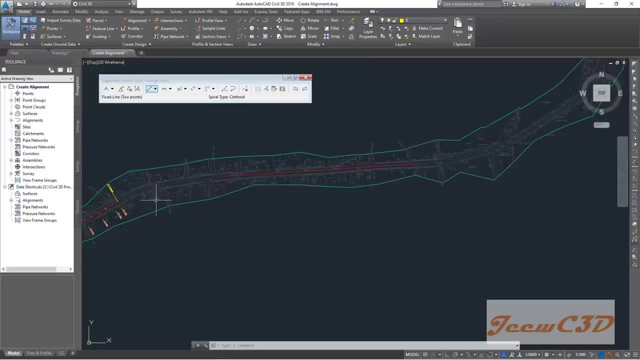 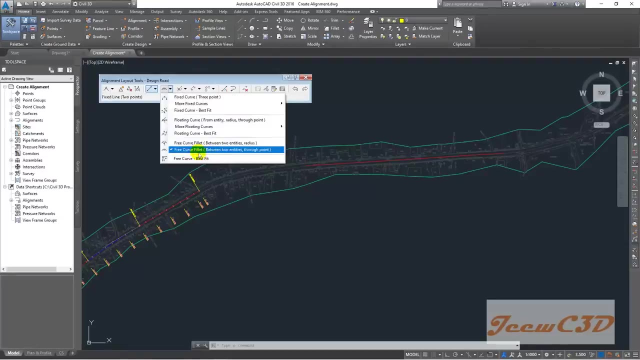 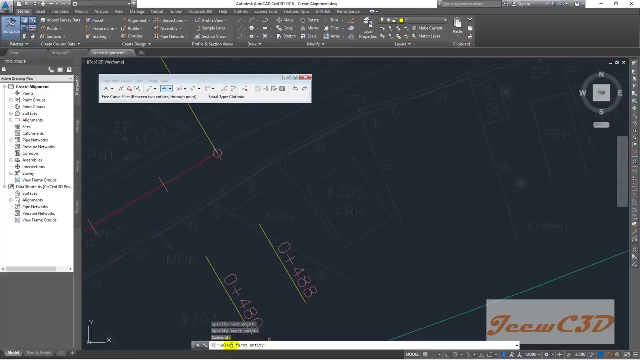 the changes are not continuing at to this point because this area is discontinuous. So that one is okay. We have to add a new curve here. Again, I go to curve option fill, curve, fillet between two entities, two points Then I. it is asking in the command line: 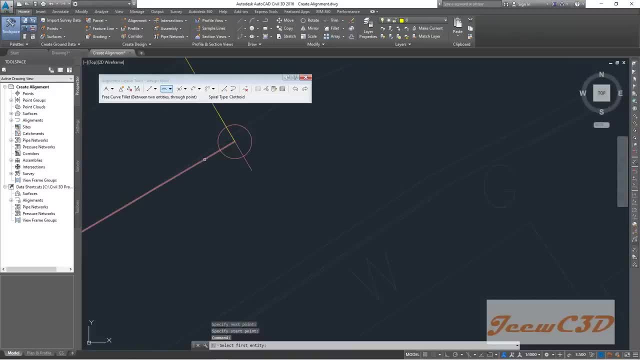 select first entity. I select this red color line. Click that red color line. Then it is asking the next entity. I will select this Red color line. Then it is asking a place where my curve goes, So I can choose a place. 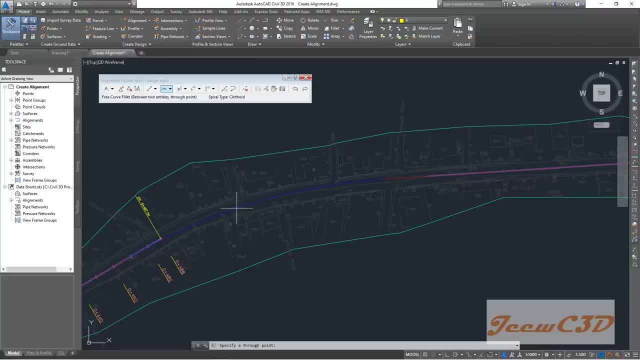 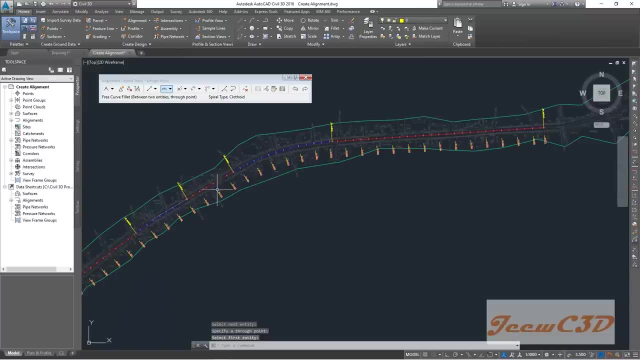 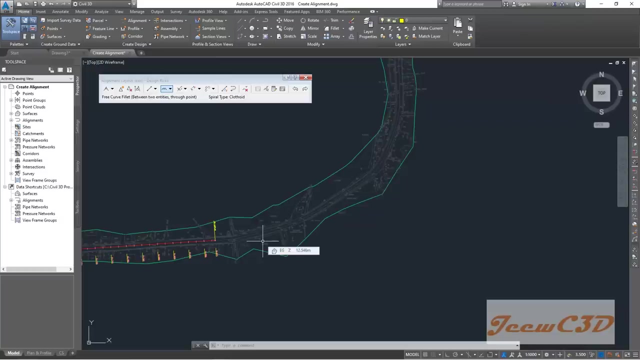 where my curve supposed to go. So that's where I am picking somewhere here. Now, up to this point I have created some part of my alignment. Then I will see the red color line. Now I will tell again: the red color line, That's a big curve within this area. 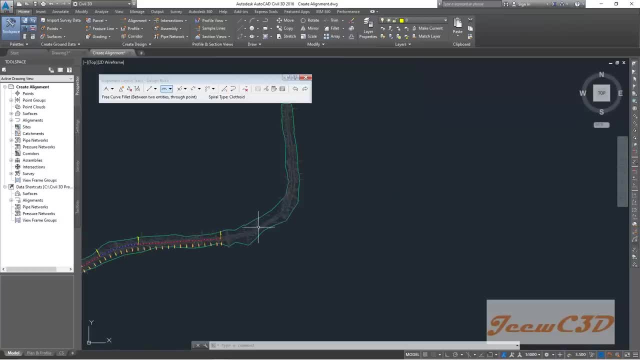 Yeah, I have to be more careful now because I don't know whether I can cover it with a one curve radius or whether I have to use a compound curve. So this time I will do different approach rather than getting a new state here and connecting this one. what? 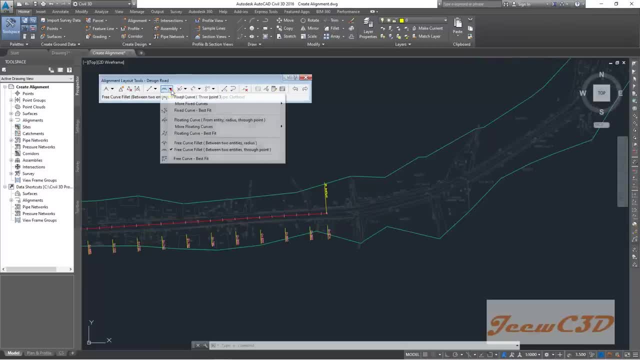 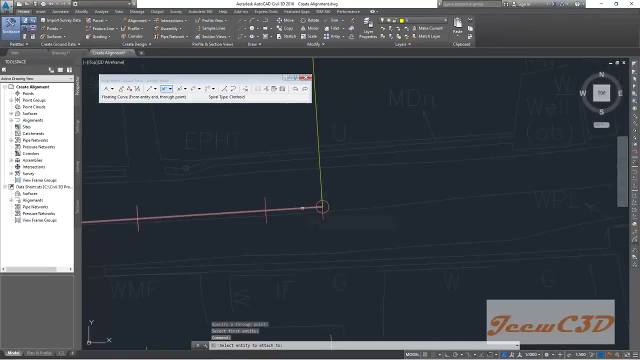 I do is I go here and I use this option. floating curves, more floating curves from entity end through point. I click here, then it is asking select entity to attach to. this is the entity where we are going to attach the new curve. I click here, then I so you. 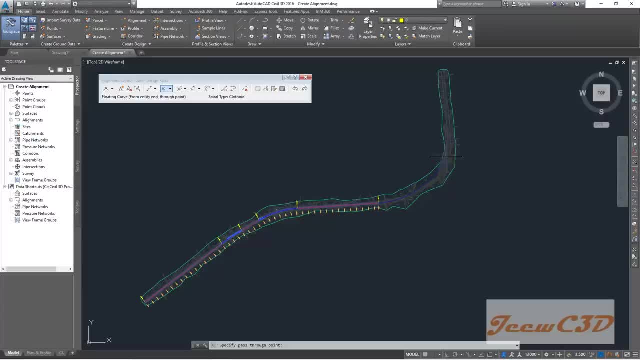 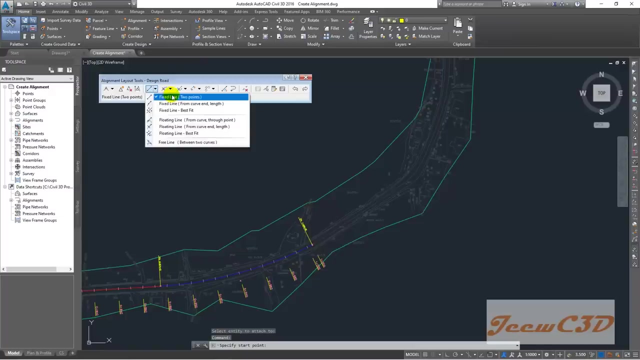 can see. I can't go in the same curve with one radius so I have to stop somewhere here. let us say I will stop somewhere here, then I go with a straight. looks like a straight is there, so I use this now. I can't use 6 lines, 2 points, because it is end of a. 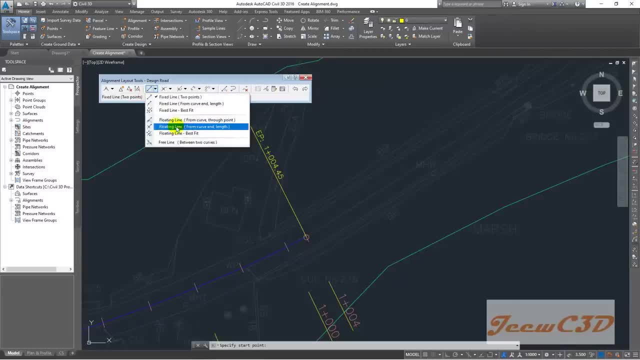 curves I have to use floating lines, tail lines where I am annealing, you have to use uis, a sink line. just start there. think of the 잘ertr happiness of growing from curve through point. then there is no, nothing at the start, then there is nothing at the 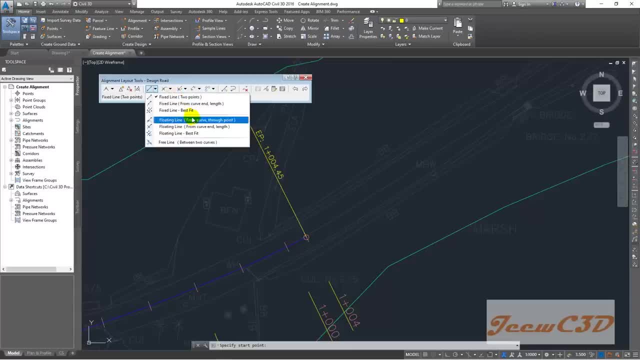 start of an entity you can use fixed entity. if there is something at the start or something at the end, you have to use floating entity. especially if you have something at the start of the entity, you have to go for floating entity. since we have a curve at the start, you have to go to floating line option. you can see. 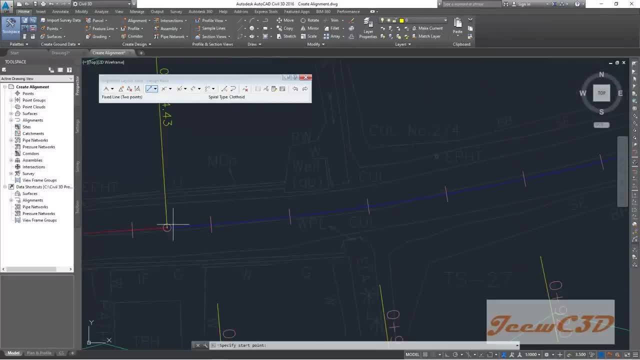 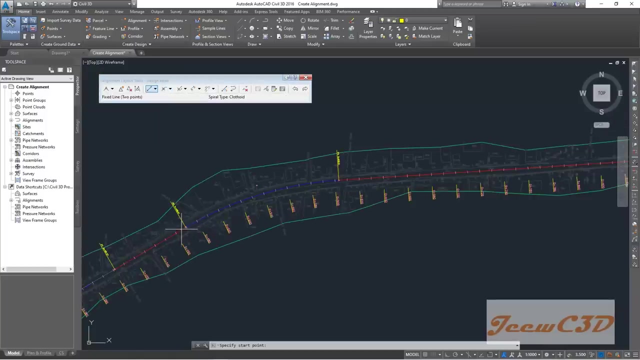 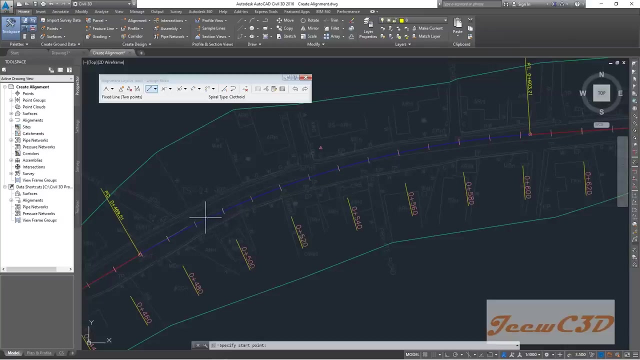 remember here I went to at this point I went to floating curve option because I had a straight- sorry, I had a straight here in this. I used floating free curve fillet option because I had entity, both sides of this alignment. entity because that means when I draw. 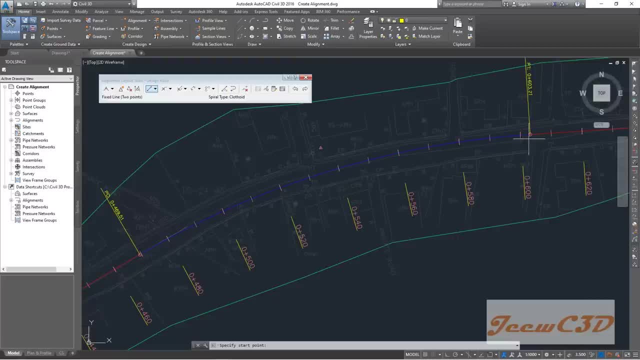 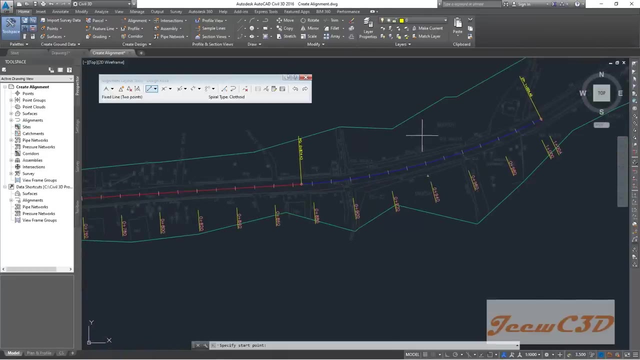 this curve. I had this straight at the start. I have this take and then I go with free curve. that means you have to concwand at both sides for floating curve also tonight. you have consent at one side. here you have what was wanting. Halloween Bay 14. 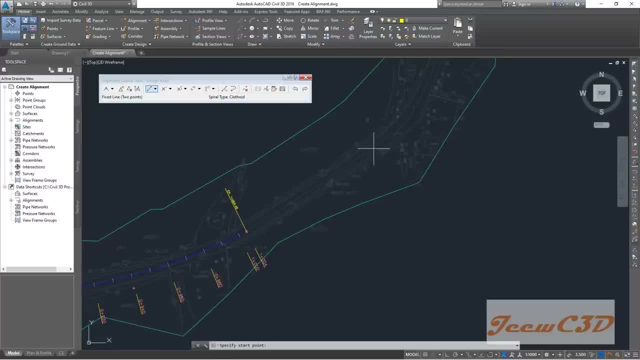 14, 14, a constraint. at the starting side and the end side we don't have this constraint, so I go here floating curve from through point. then it is asking: select the entity to attach to. so I select this one. then it is asking: what is your endpoint? so I will be selecting somewhere here, so it is hard to select. 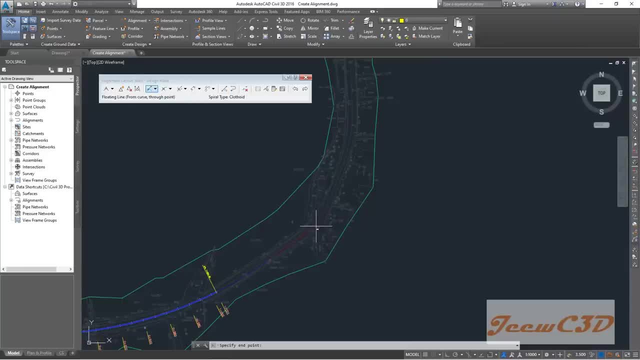 because of the curve type. sometimes it may have to go outside the curve. let us stop somewhere here, like we are getting a very sharp curve. then again I will go with the floating curve option, or otherwise. you, I can use this first. I can use this straight section. you, I can create this straight. 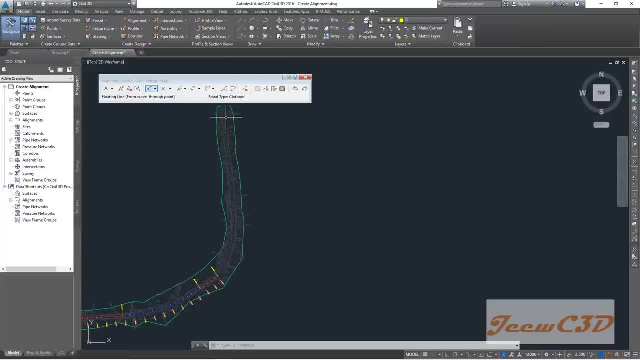 section, since I am creating it from here to here. I don't have any constraint. so I So I can go with the 6 line 2 point option. I click here and I click somewhere here at the end, Then press enter. Now my end is okay. Now I have to have a free curve here. Free curve, select here. 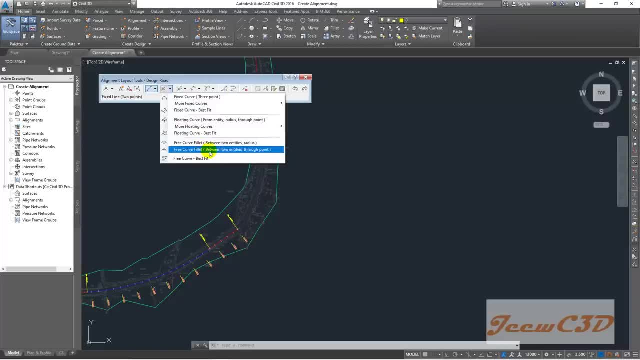 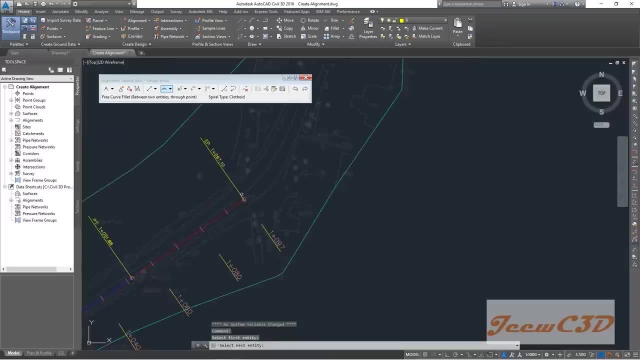 Then I go here, Go free, curve, select between two entities, 2 point. I click, select this one as my first entity And select this one as my second entity And I have my curve somewhere here. like this It is not readily following the 15 row center line. 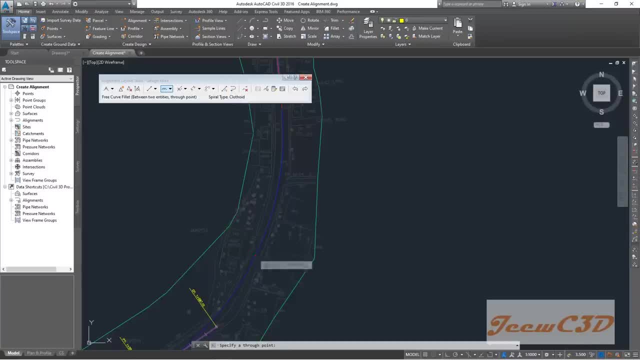 So I will make it as much as possible. So you can see here I have a very sharp, I have a compound curve here, Turning at the same direction And with a small straight in between. So I will try to modify this in the coming video. 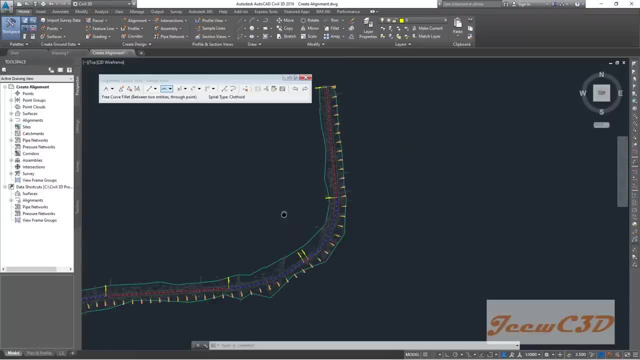 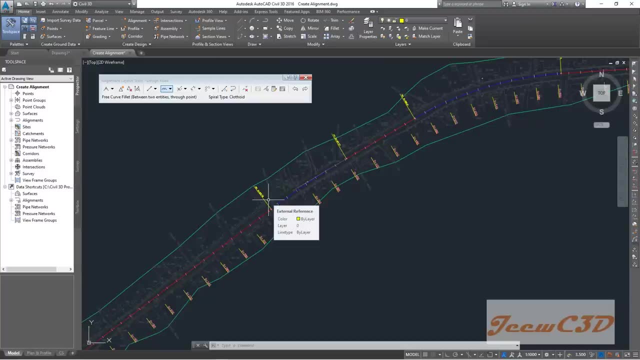 So I will try to modify this in the coming video. So I will try to modify this in the coming video. So up to now, we have created an alignment. Actually, this is a kind of trial alignment. We don't have followed any standard. 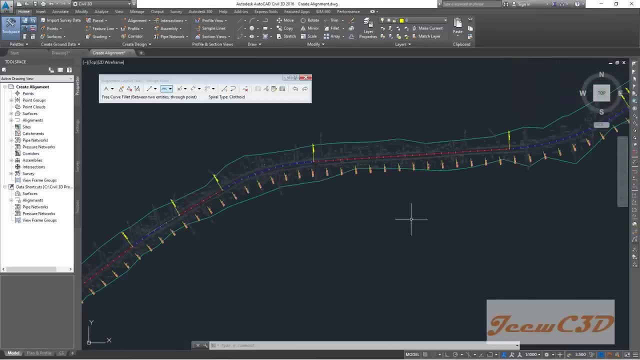 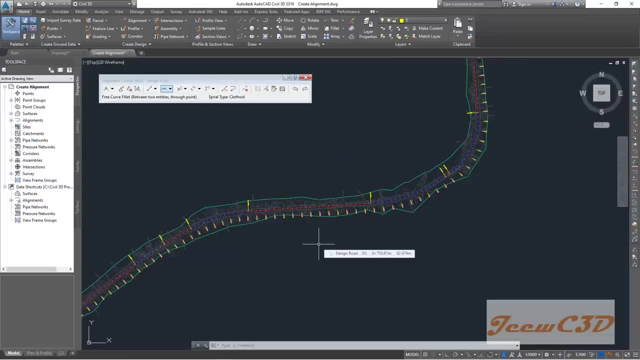 We just create the alignment according to the road. Now, in the next video, we will see how to modify the alignment according to the defined standards. In the previous video, I have told you how to create an alignment to match with this existing center line of the road. 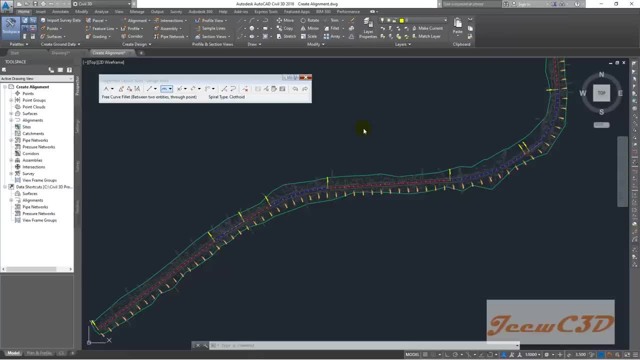 Now, in this video, what we are going to do is modifying the alignment according to the defined standards, and so you can do it first. you can, when you are designing the alignment, you can do the guideline part along with the design alignment part, but in this case i have 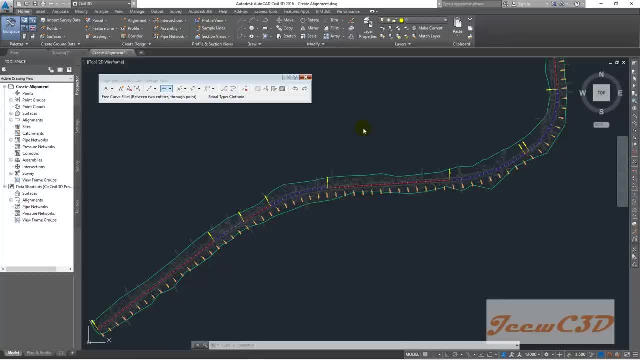 designed the alignment first and i am applying the guidelines at the next step so that you can understand the things clearly. but when you are getting that familiar with these things, you can apply the standards on as while you are designing the alignment at once. so before doing that, i will close this toolbar and i will close this drawing. 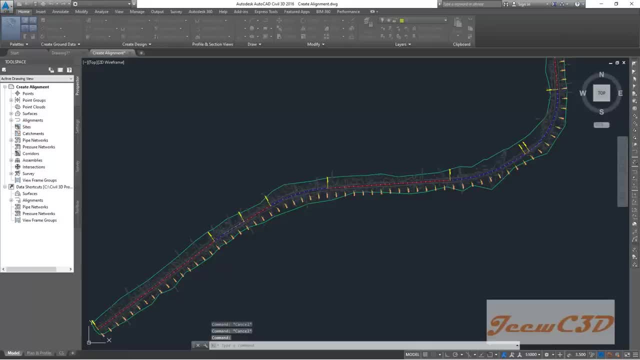 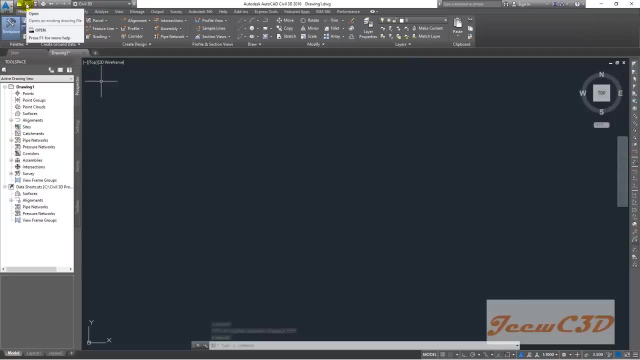 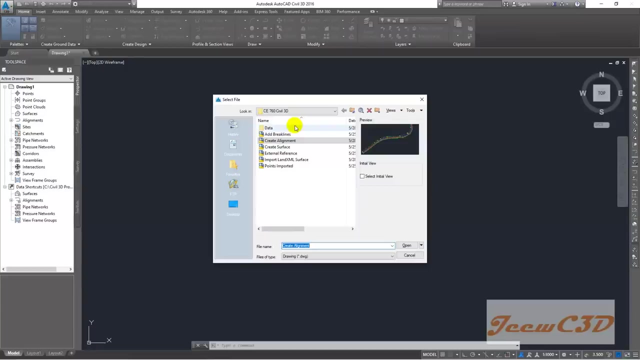 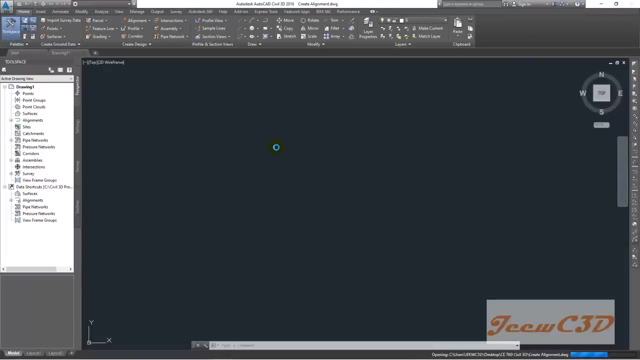 then i have to save the drawing. so i close the drawing, then i open it to open this. i can use it here or i else i can go to open option here. then i go to create alignment drawing and i will open it now in this video. what we are going to do is we are going to modify the alignment. 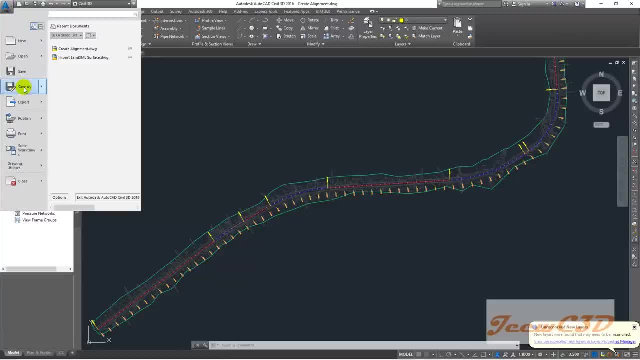 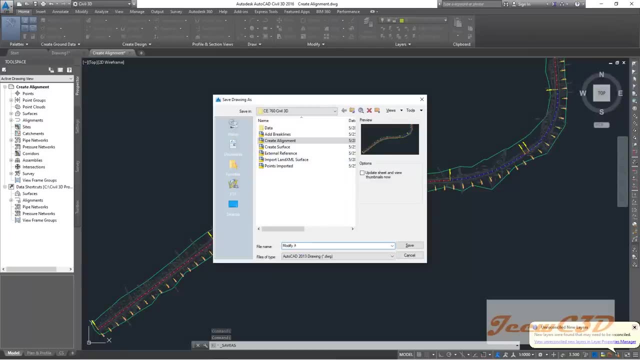 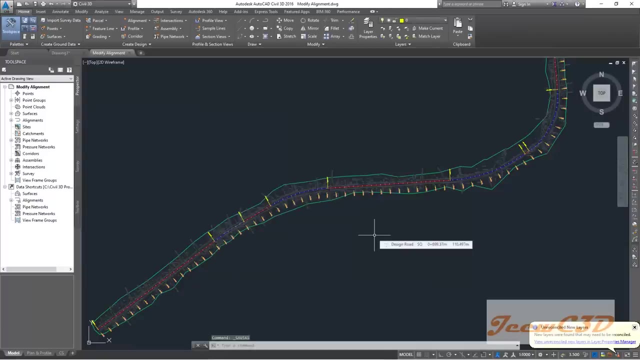 so i will save this drawing as: save this drawing as modified alignment. then i click save. so before modifying the alignment, you have to have idea what kind of the road you have you are going to design. so you already know you are going to design a two-lane, two-way road at a speed of 60 kilometers per hour. so i told you you are going to follow. 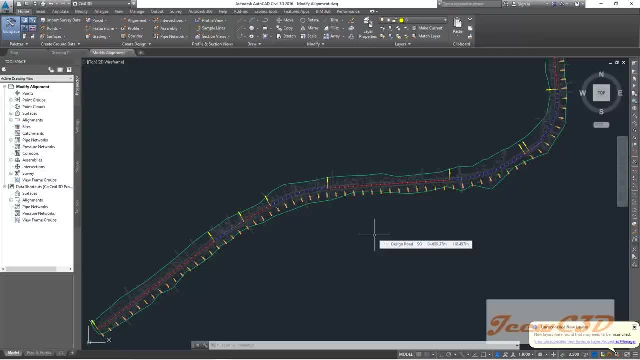 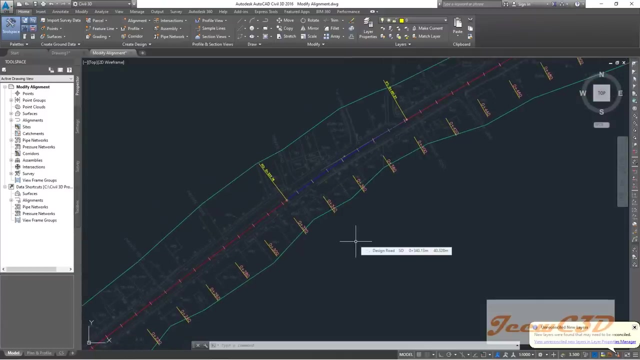 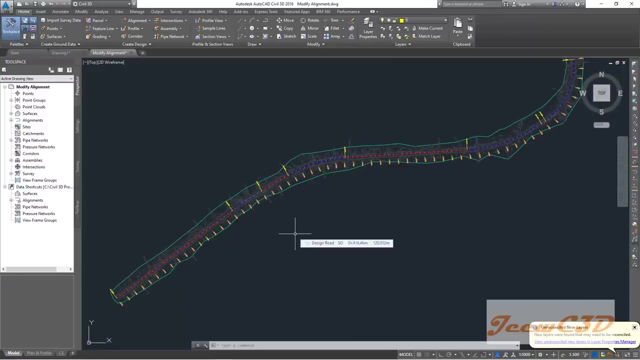 the rda design guidelines. so now, when you are following rda design guidelines, so what kind of data you need to create the alignment? now you have created the alignment without thinking any of that. you have just created the alignment, so now you need to draw the alignment, you need to define the alignment. 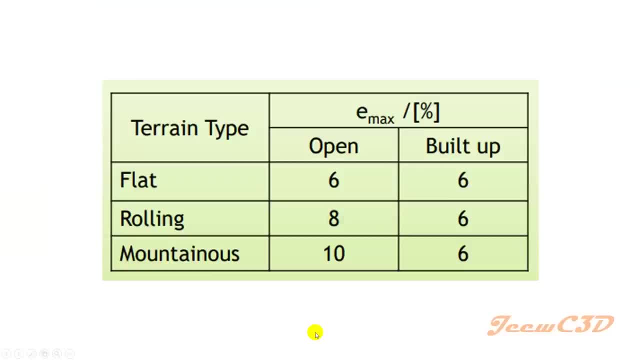 i told you that we are defining this road in a flat terrain. so, whether it is an open area or a built-up area, your super elevation- maximum super elevation- would be 6,. you can't go beyond 0.6% gain if it is an open area or a build-up area. 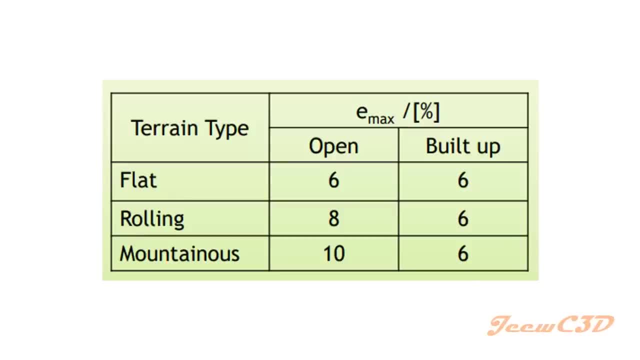 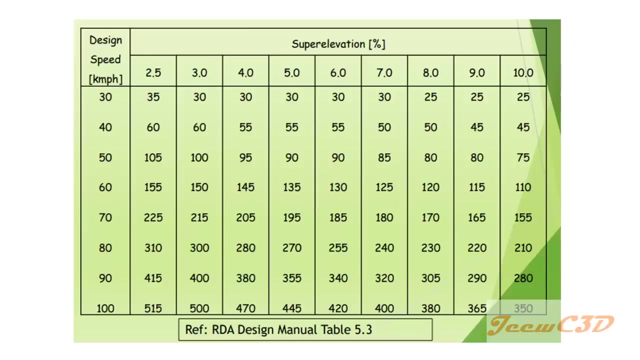 your super elevation, maximum super variation would be 6. you can't go 6.3%, gain super elevation in this road. So that thing has to be in your mind. Then the super elevation thing. So things we are doing at a maximum super elevation of 6 percent and we are designing the 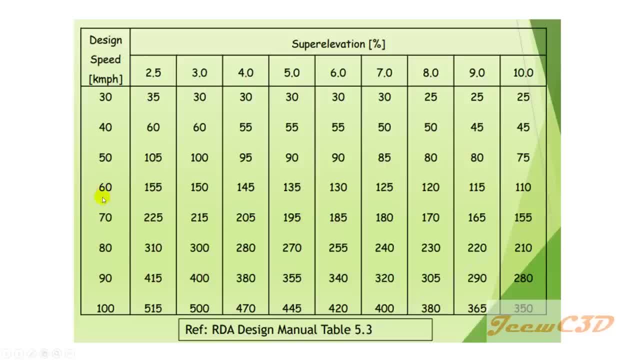 road for 60 kilometers per hour. This is the area you can work with 60 kilometers per hour up to 6 point super elevation. So you have to use a minimum radius of 130 and more than that to design your road. So if you use 130 radius at that point, 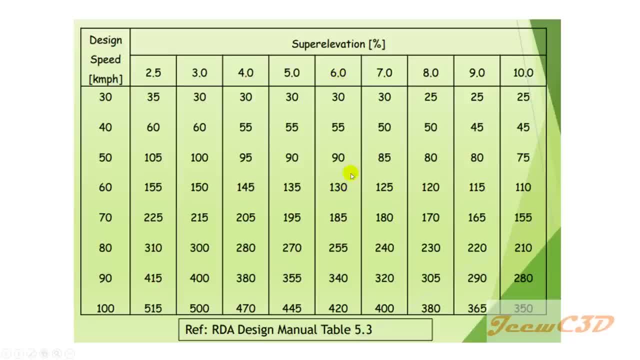 at that curve, your super elevation would be 6.. If your radius is 135 or greater than 135 and less than 145, your super elevation would be 5.. Likewise, you can go up to here. If the radius is more than 155, your super elevation would be 2.5. 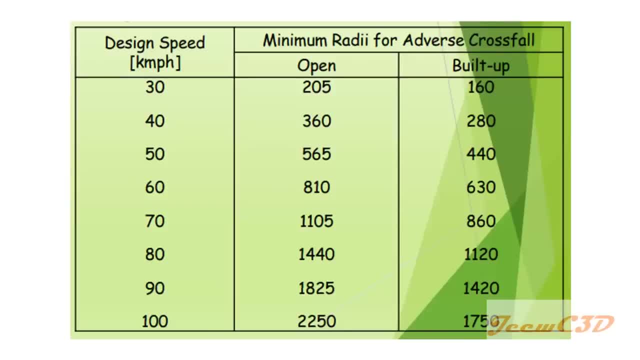 But if your radius is more than 810, let's say this is a build-up area. So if this is a built-up area, your adverse cross-fall would be at 460 kilometers per hour. The adversity you are at, the speed you are at, will be 613. So this is why the radius isивается more than 810.. Let us say this is a built-up area. it just means, If your radius is more than 810- let us say this is a built-up area- your adverse cross-fall is at 6364.. For 60 kilometers per hour- design speed, your adverse cross-fall will be 639.. 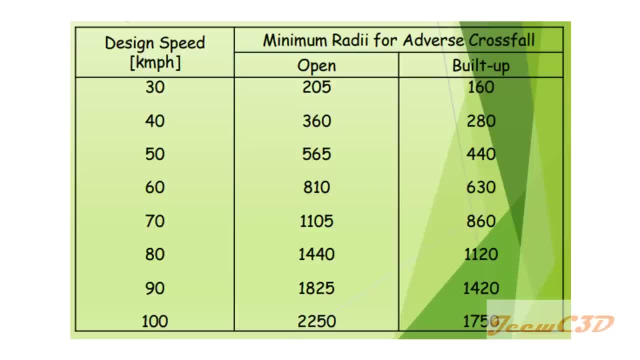 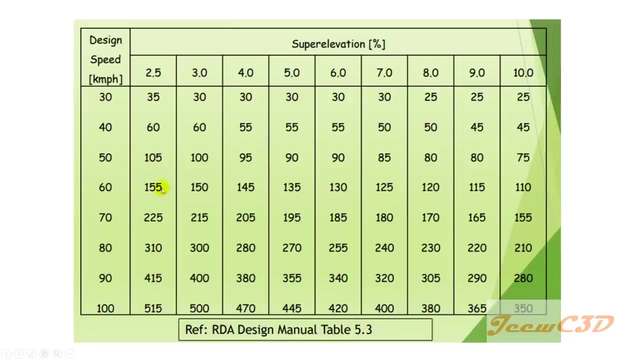 So when your curve radius increases more than 630, you will be having a normal crown for the road. That means you will not be having super elevated road. Your road will be like a normal crown road or normal super elevation road. So whenever the curve radius is greater than 155, your super elevation would be 2.5. 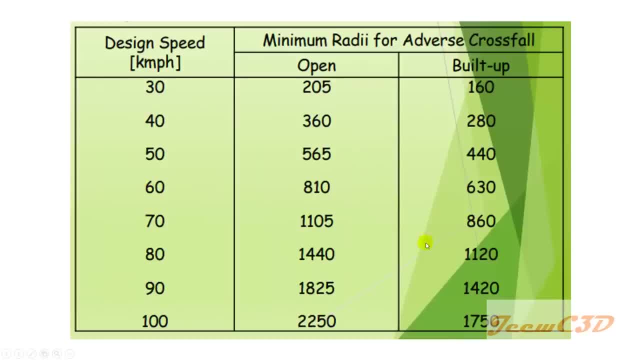 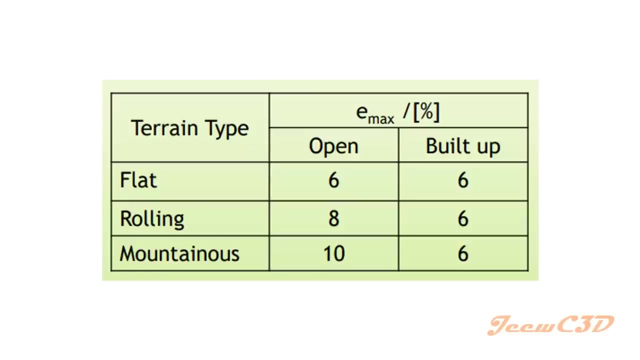 But if the curve radius is even greater than 630, your super elevation would be minus 2.5.. That means it will not be 2.5 super elevated, It will be at the normal cross-poll side. So those are the things you have to memorize, this maximum super elevation thing to know. you can go up to 6%. 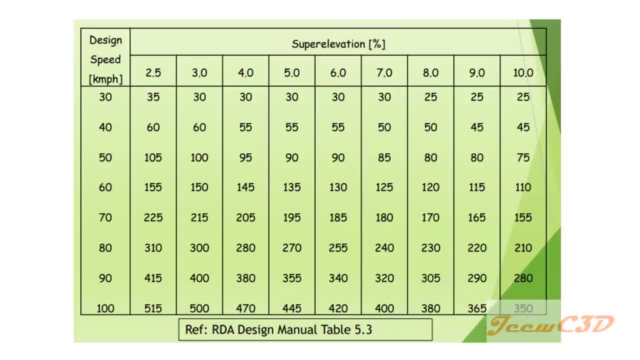 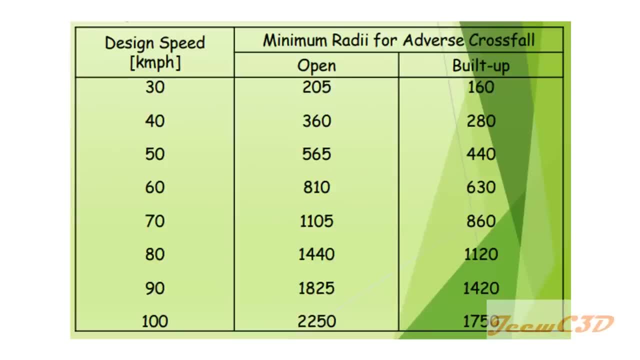 And this is just radius- minimum radius you can use for this super elevation. And this is just adverse cross-poll super elevation, adverse cross-poll radius for a built up area where you designed this road. So we will move on to the drawing and see how. 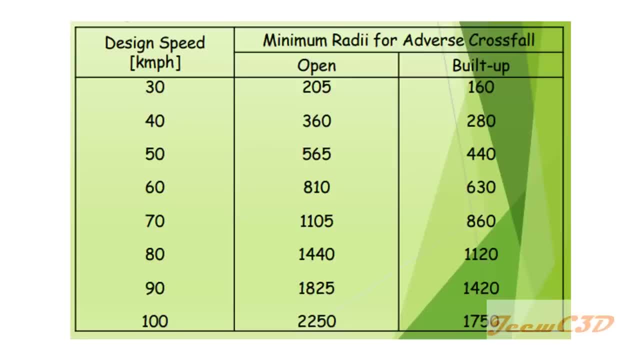 the things are there because we already have a created alignment. We don't know how we have created that alignment, Whether we have followed the RDA guidelines for 60 kilometers per hour or we haven't followed it. So we will check it now. 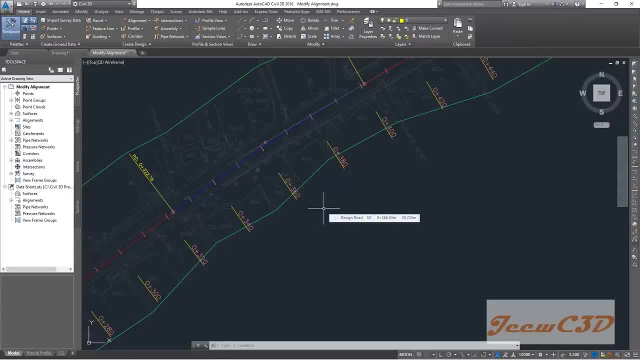 Now I have this alignment. Now I am going to edit this alignment So that I get the design alignment to be complied with the design guidelines. So to know these things, I have to know what are the radius values here. 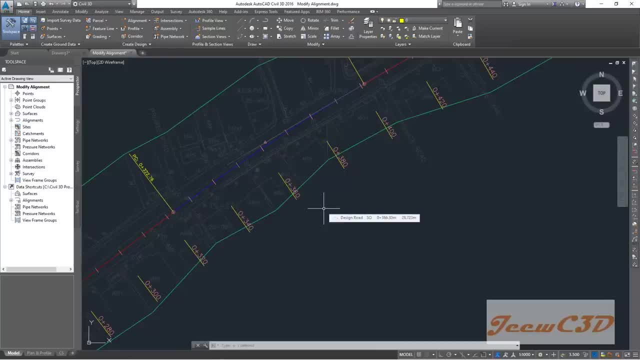 So, according to the guidelines, I have to use a minimum radius which is greater than 130 meters. So I can add that I will use a minimum radius which is greater than 130 meters, So I have to have a 60 kilometer per hour design road. 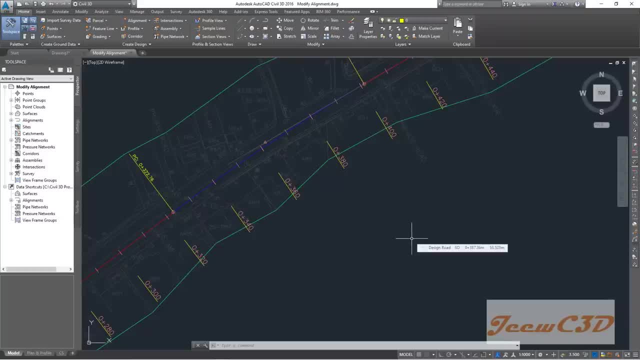 So we will see how we have design road up to this point using it without thinking of the guidelines. So now I am going to know what is the radius of this curve. So to do that, I click here, select the alignment. 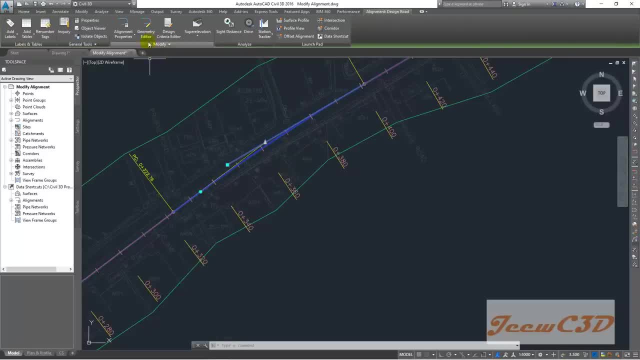 Then I go to here geometrics. I am going to submit here geometry editor and you will be getting this alignment layout tools, which was used to create this alignment initially. So when you are creating the alignment accidentally, if you have closed this one, you can get it back by selecting the alignment and go to geometry. 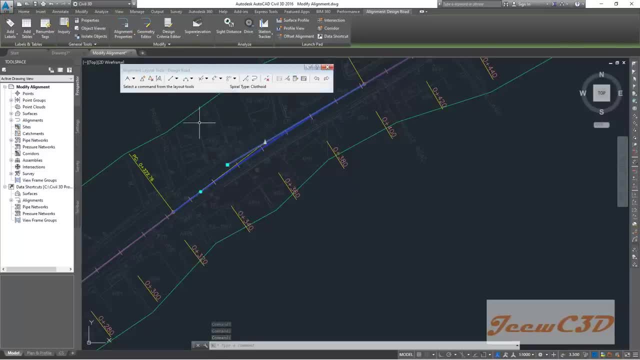 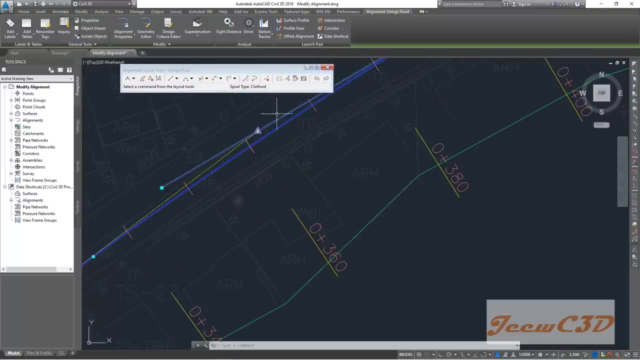 editor. So in case, if you see these, all things are grayed out so you can't select any of these. if that occurs, you have to close the drawing and reopen it. so it will be fine by that. So now I am going to set this curve radius. I click here this six subentity button A: 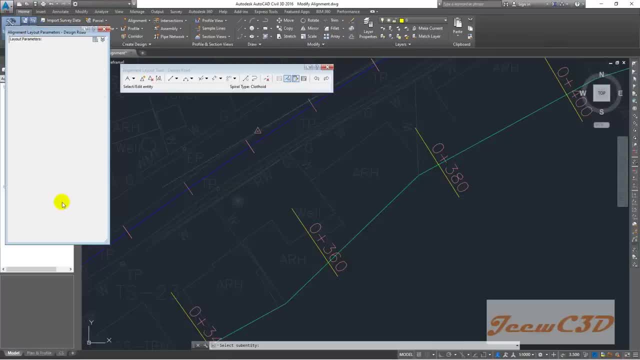 small window will be appearing on the side. Now I am going to select this curve. Select this curve, blue line, and you can see my radius is eight hundred and 60.201.. Since this is kind of an odd radius, I am going to change it. Also, I can see my. 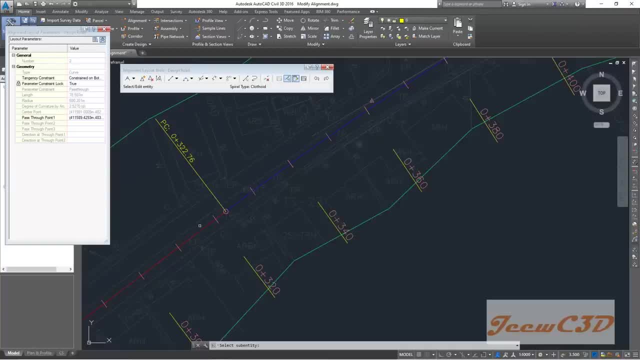 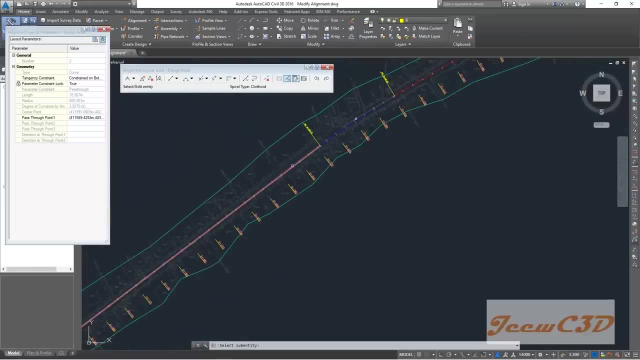 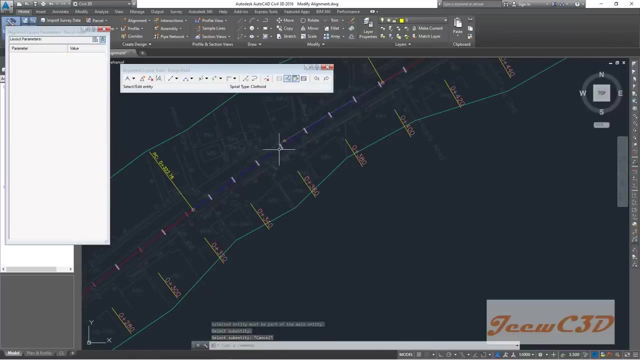 center line is too far, far from the alignment center line here. So I like to kind of change the alignment so that this part comes here. So to do that, I press shift, then to do that, I want to delete this curve, So I am doing. 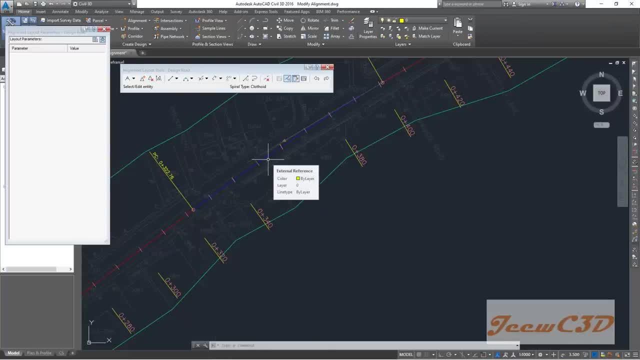 kind of modification to the alignment, So I don't I have to delete this curve, otherwise if I shift this thing my whole alignment could be shifted will be a problem. I will delete this curve first to disconnect this alignment from the alignment center line. So I am going 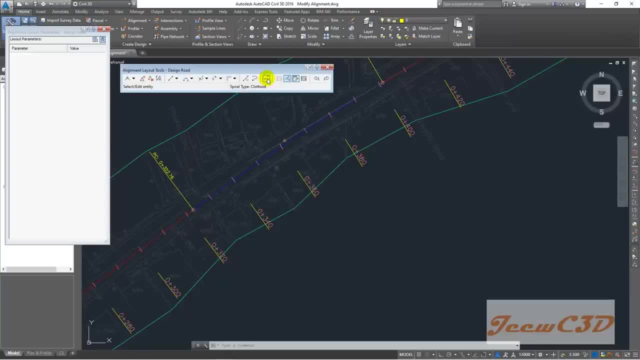 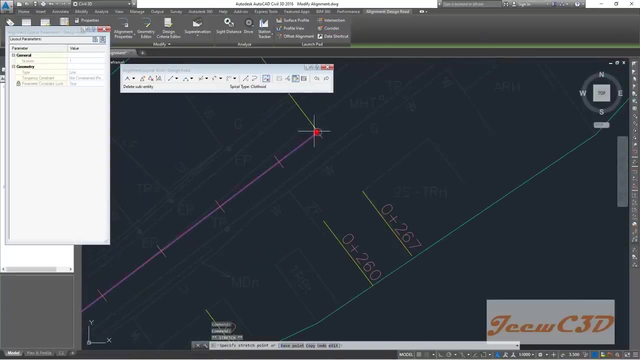 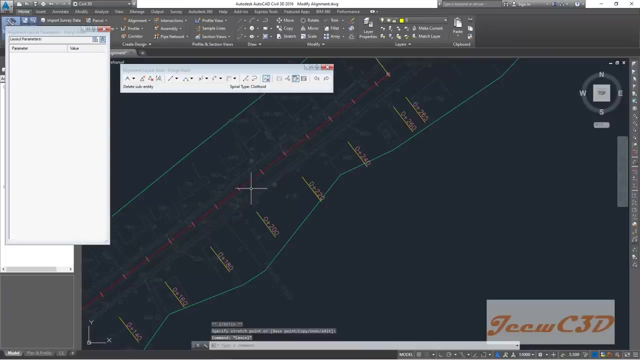 to change the alignment from here. To do that, I click here, Then I click this one, So my curve will be gone And I will shift this straight section or the tangent section from left here. So then I will be having a small depth here, but I think it is okay, since my 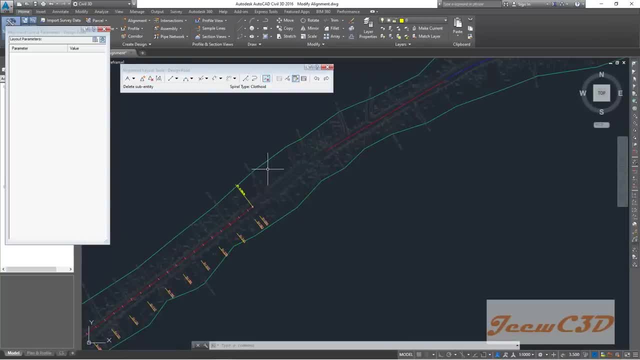 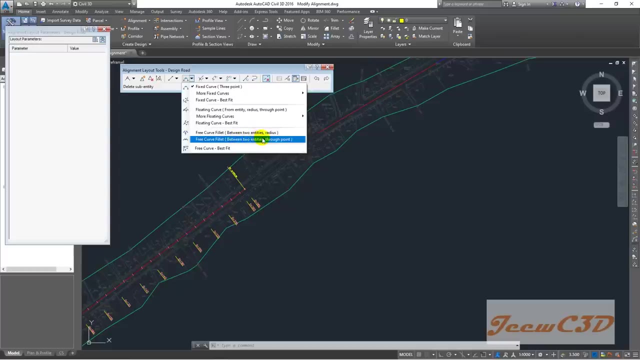 area is OK, So I don't have any issues with таких or anything. so I am going to change it Now. type t here. Our tangent tail plug is going to be placed. right click this point value and now I am created a new division, So I am going to add the vertical line here. bad. 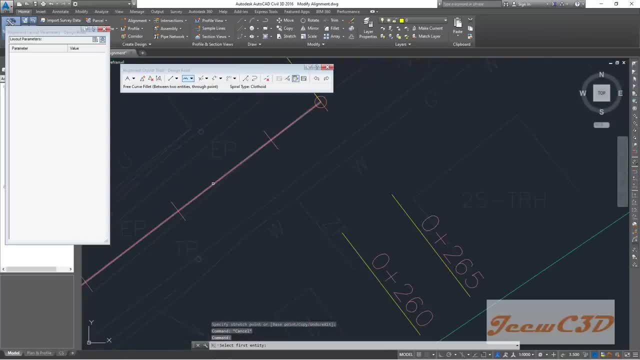 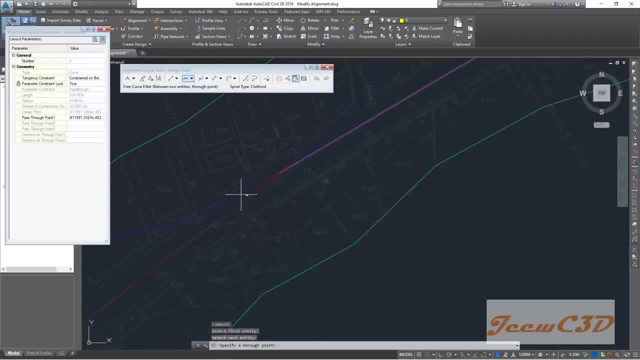 or the horizontal line, and the horizontal line is going to be graded a little bit more, So let's go ahead and create new division. You can see that I have added first and then twice: Yes, Yes, And I mark in the alignment. 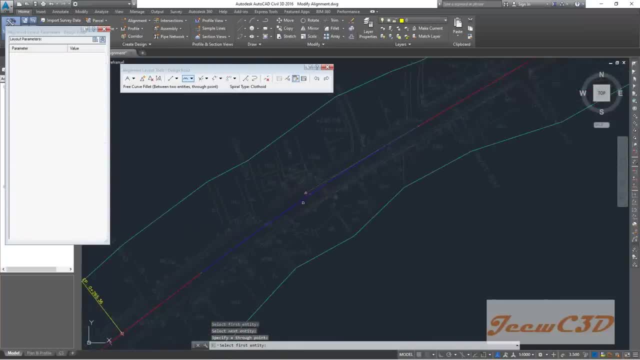 Right there here. Now I will just move towards to the center line. Just in case it is okay, I just center. Now again, I am going to use this 620 grader And select this curve. So now I see my radius is 600 and 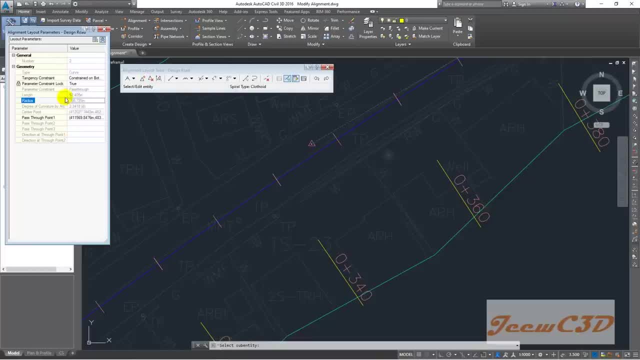 76 and you have so many other data for this curve. But I am worrying about the. what I worry is the radius. So I wish this radius to be some kind of rounded value. So what I do is I change this parameters constraint lock to false. 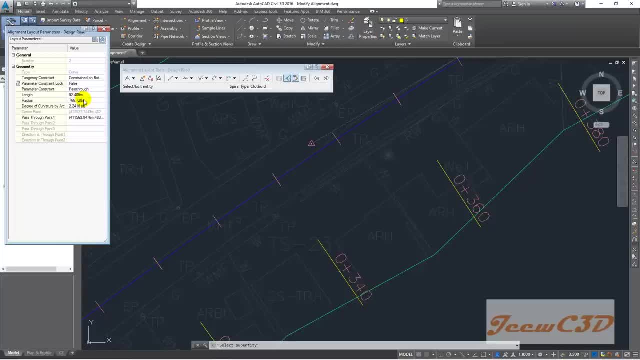 So then your radius will be activated to have some kind of edit. So I will change this radius to, let us say, 800 and see what happens. You can see, it is a slight change in the alignment, which is not a bigger thing to worry. 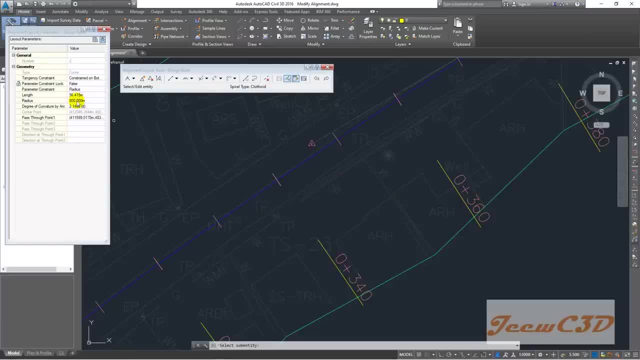 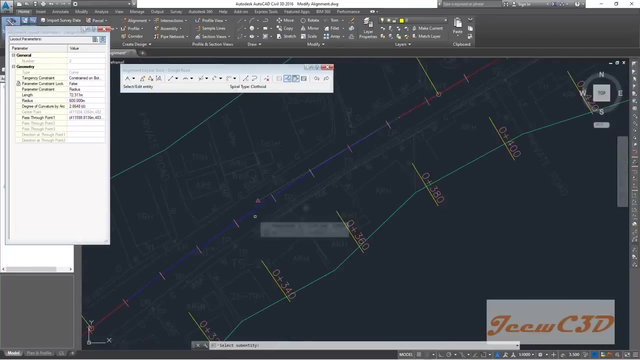 So I will keep it at 800.. So the beauty of the Civil 3D software is, once you apply the modification, it will show the results straight away. So if I type this as 600, it will show the results. So now you can see two things here. 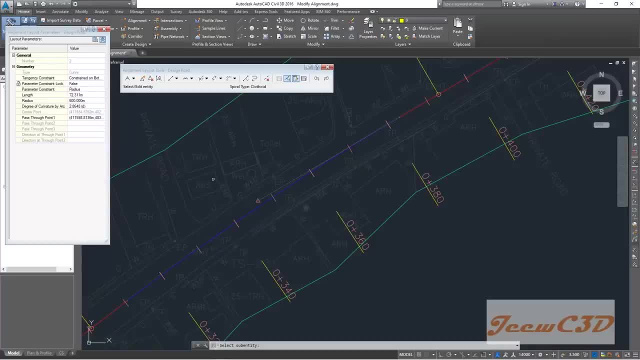 If you apply the 600, it will look like this. If you apply 700, it will look like this. So what option you go with? If you apply 600, you get this kind of a road. If you apply 700, you have a small shift here. 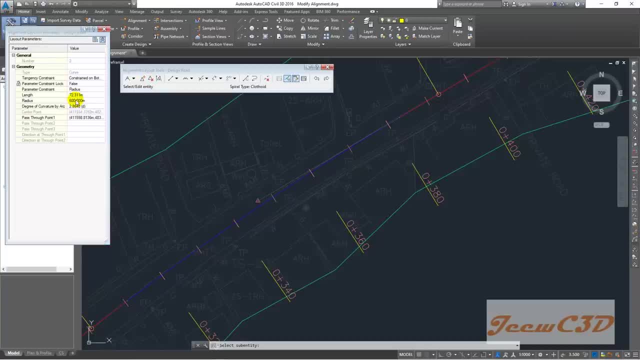 If you apply 600, you have a small shift here. it goes to the center line. But in this case what you have to memorize is the adverse cross fall. Your adverse cross fall would be 630.. So if you go more than 630, you can avoid super irrigation in this section. 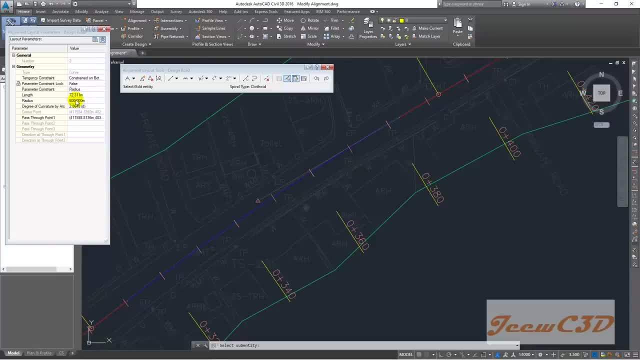 That means you can go with normal cross fall. So if you stick to 600 radius, you have to apply super irrigation. So this is a large radius curve. I can increase the radius, So I use 700.. Otherwise you can use any value greater than 630. 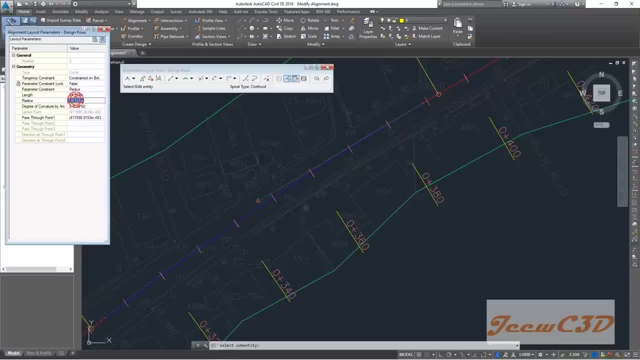 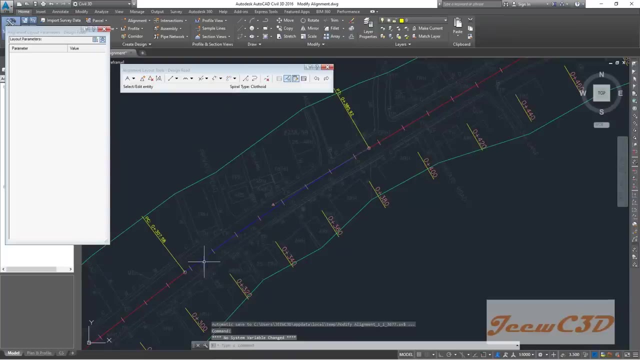 You can use 650 also. It actually needs to be 760.. So that may be very close to the existing center line. So that is that we are sticking to 650.. I press enter Now. this curve will generate. Now I am going to this curve. 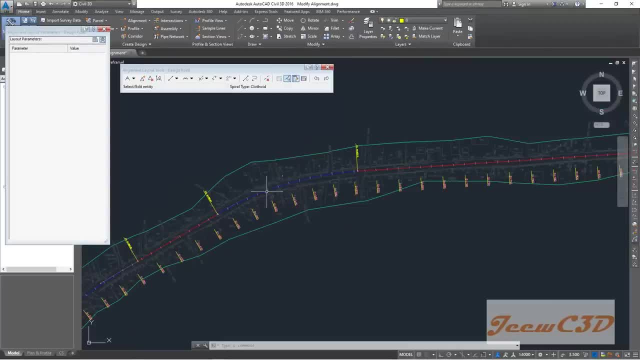 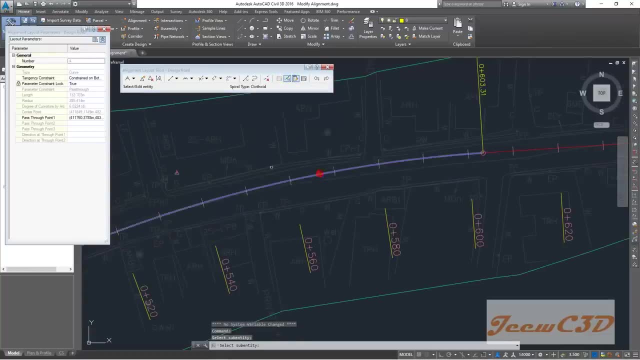 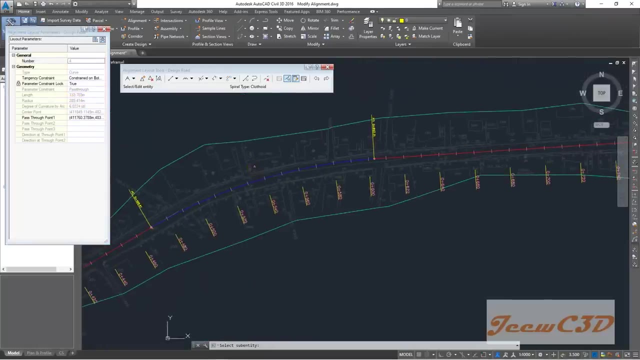 This one also have some modifications from the center line. But let us see what are the parameters. So I click here: fix up the interior heater, Select this one. My radius is 285.. So I wish to modify that radius. So here, and let us say we change it to 250.. 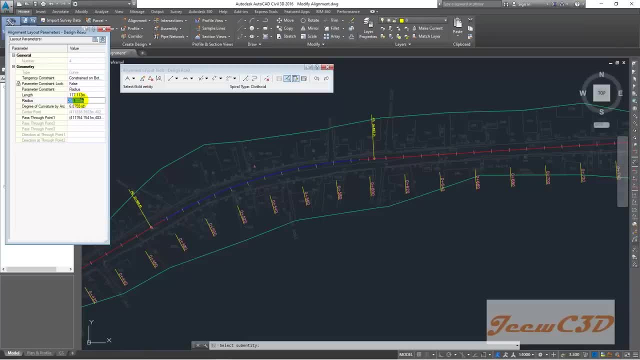 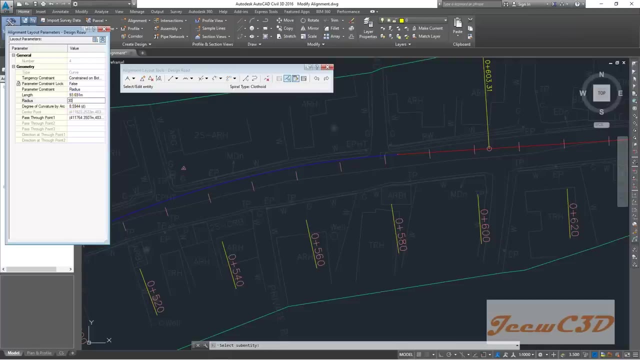 Otherwise you can change it to 200.. So when you are doing it, when you are lowering the radius, you can see this is going towards the houses. So I have to increase the radius of this. Let us see what is happening here. 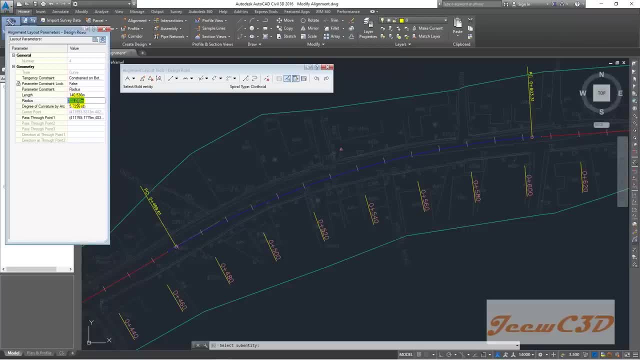 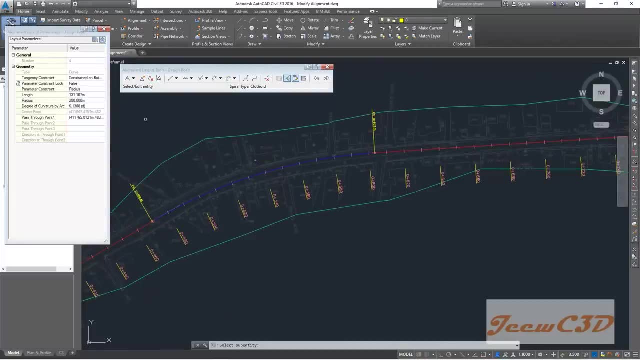 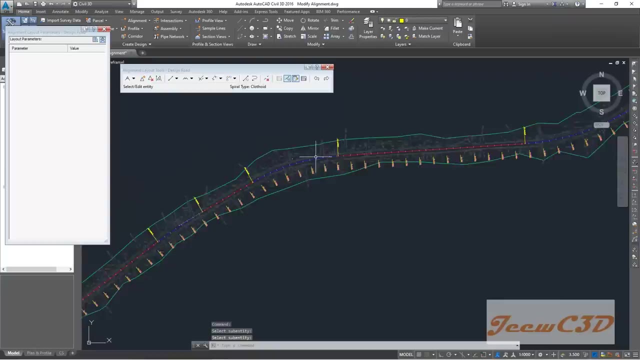 Now we find the 4k We use 280 may be much better road, So I will stick to 280 at this case And I press enter to complete that one. Here you have another two curves Here you can check what to do. 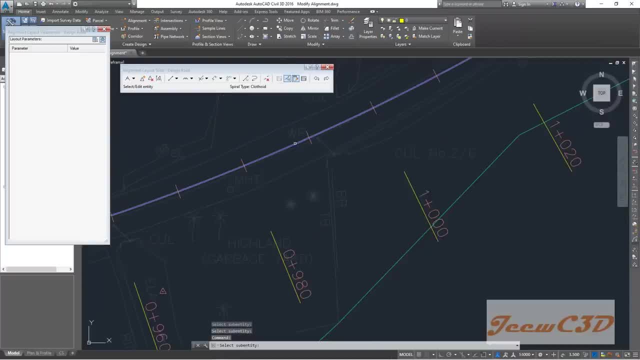 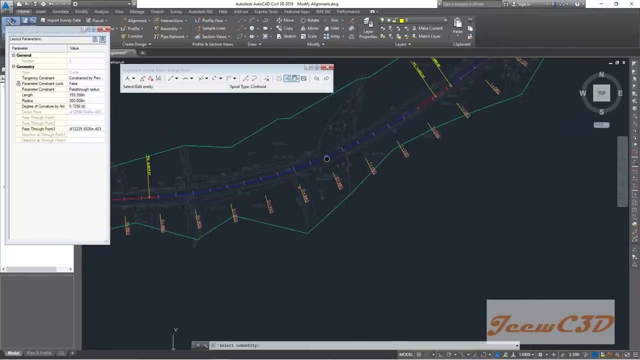 I click here and click this, So and you can see this radius is 323.. So I go to here and make it 4 and let us say it is 300.. Seems okay And we go to next curve. So, without going enter in. 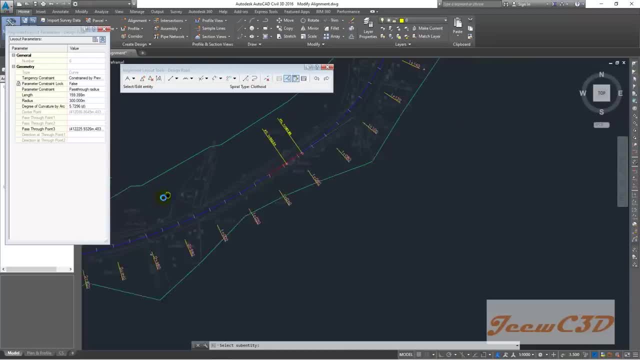 Or without pressing enter, You can straight away go to the next curve, Because it is asking select sub-emptity. So you can go to the next curve, which will be given the values here. So it is giving these values for us. 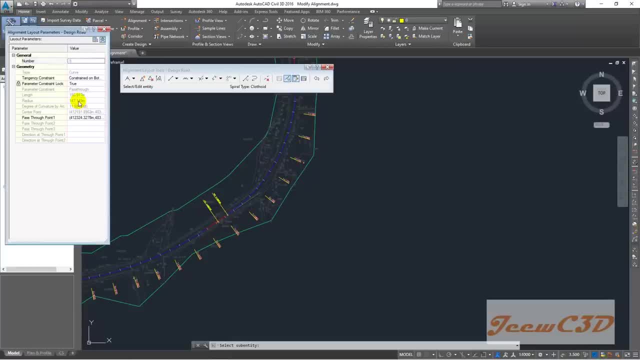 Now One thing I have to remember here: This radius Is 300. And this one is 147. So 300 means superelevation 2.5. Because any radius is any radius of a curve Which is greater than 155 meters and less than 630 would be 2.5 superelevation. 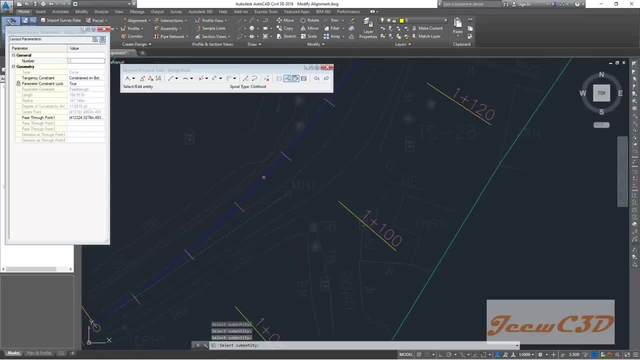 So currently this is 147. So It is less than 155.. So you have to apply a superelevation Greater than 2.5. maybe You have to look at that table and find what is the value. So instead of that, I will. 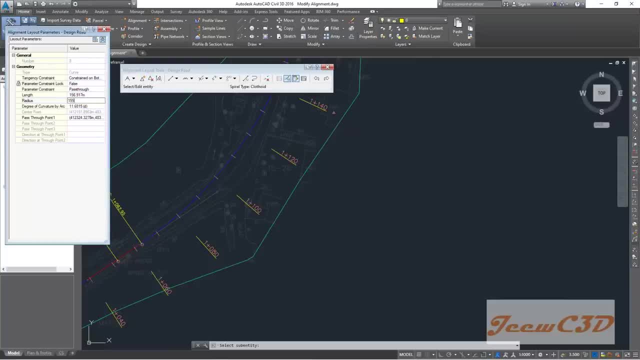 Increase this radius to 155 and see what happens. So you can see This is going A bit far away from the existing road. So I can't go that much. because it is going far away, I have to reduce the radius. Let us say I reduce the radius to: 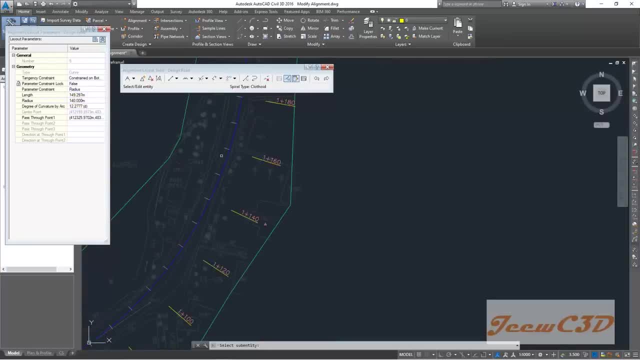 240.. You can see, in this area I have another problem because the road is shifting too much. So instead of doing that, I think I'm thinking of having another straight somewhere here and have two curves, Two separate curves. So to do that I will. 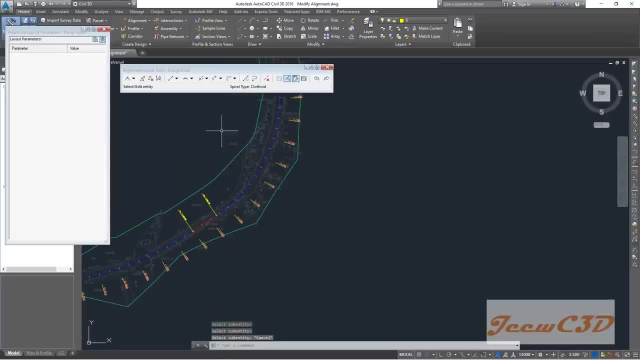 Press shift Button And I click here, Close this, Click here and delete this entity. That's the space. Let us say we have a small straight section here, So I do six line, two points, Then I create this straight section here. 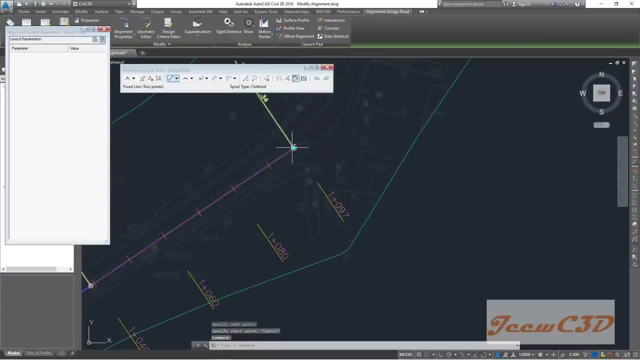 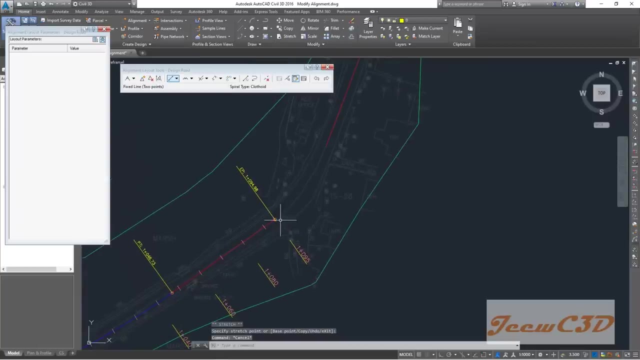 Then again I will modify this one also. I select this Red line and from this clip I can modify it. Then I go here, Go to free curve fillet option, Select this red line, Then select this other red line. 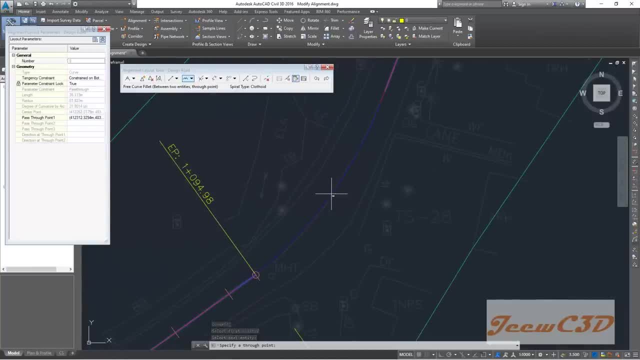 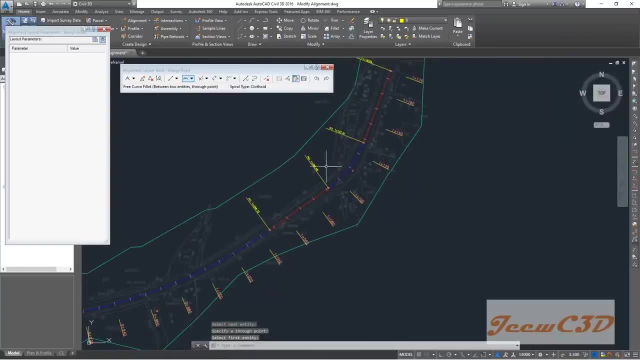 Then You can use this area- That's my curve- And enter: I am okay with that curve. Let us see What is the Curve radius. I'll click this 6.1. Then I click here: My radius is: 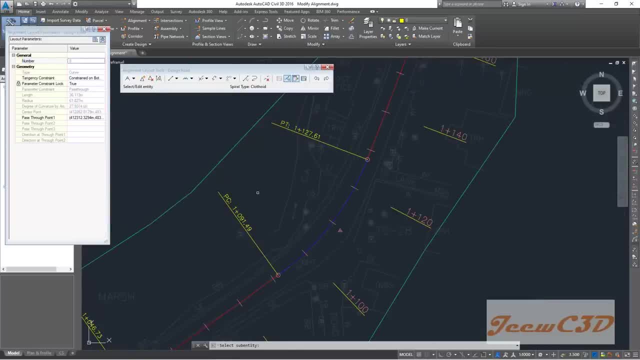 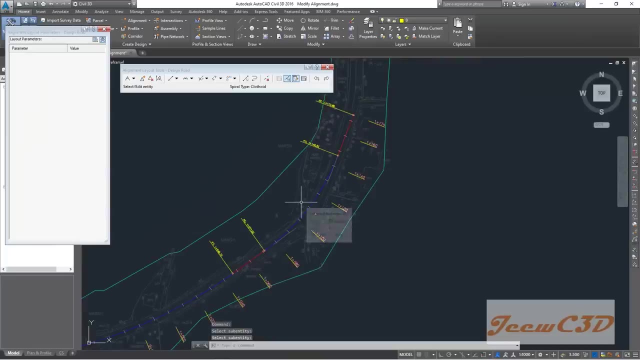 66 means a very low radius. Yeah, I cannot even use for 60 kilometers per hour speed, So I have to increase it. Let us say I choose 130.. So definitely I have to use this curve to go to 130.. 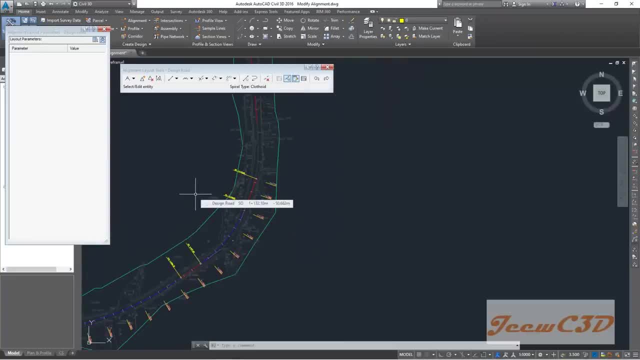 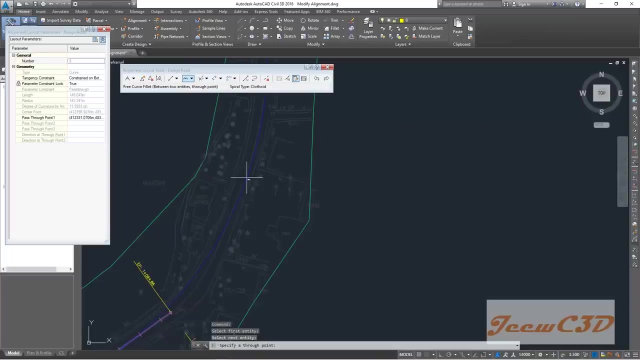 So there is no option for the moment. So instead, what I do is I create these two curves which I created, And I am going to follow this free curve, fillet, again to use this single curve, as which was earlier. Okay, So I will change the parameters here. 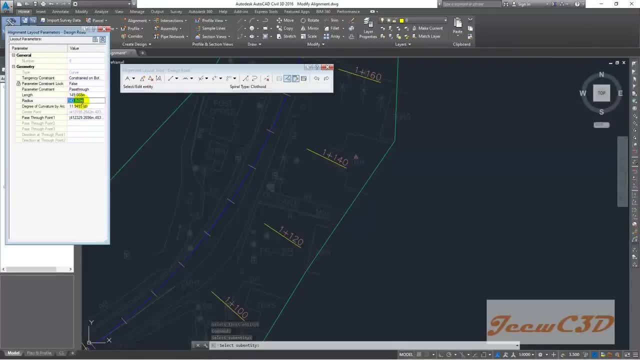 Suppose, Let us say, we change this value to 140.. Okay, 140 would be good because we have a house here. We don't have any office in this side. This is a very short interval, So let us say that kind of a. 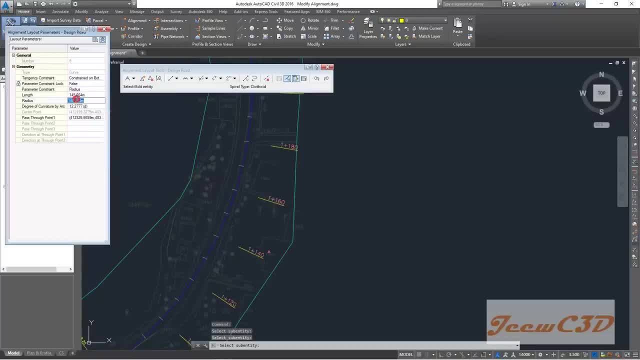 Good day, Otherwise you can prove 140.. Okay, So let us say that one is better, 145 is better. So I click enter to close the alignment. So we have Finalize the alignment. So you can Leave all the alignment entities at once by clicking here. 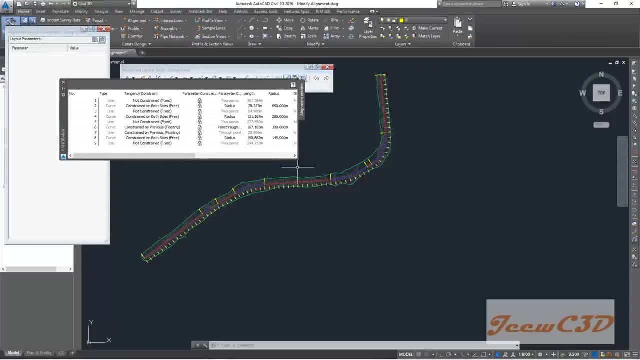 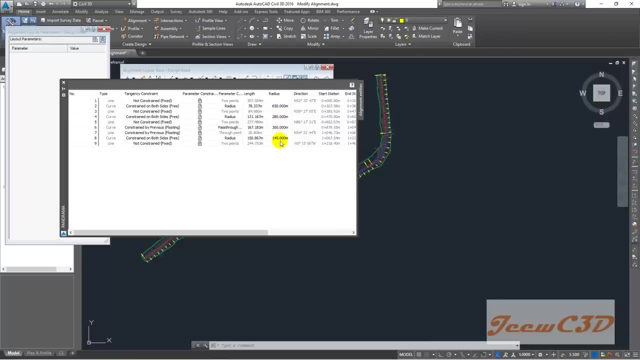 So Parameter Detail Alignment- Grid view will be appearing, So you can see all the The radius values we used and the length of these curves as well. So if there is an error you will see some kind of a warning sign here. 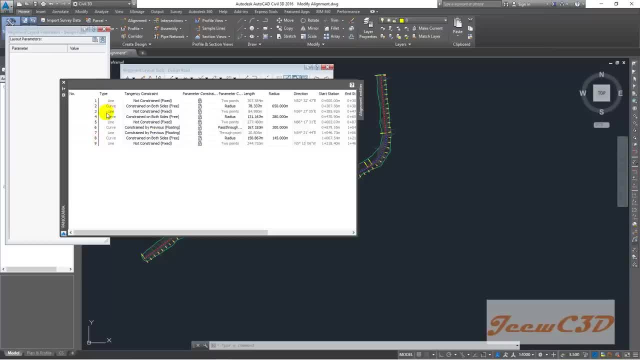 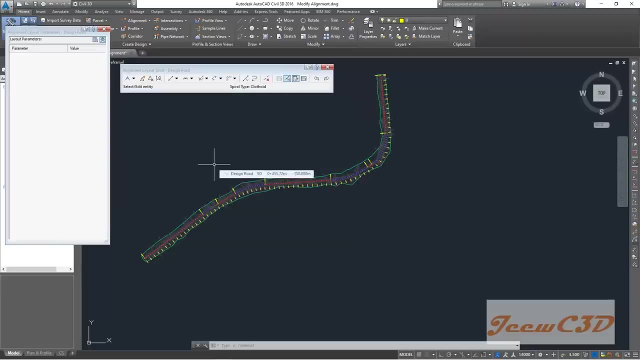 If you haven't done it correctly. Otherwise, if you have done it correctly, you will see This kind of alignment grid view. Here you have all the Data. So We have finished the modification and the alignment. However, what we are trying to do is to follow the existing centerline. 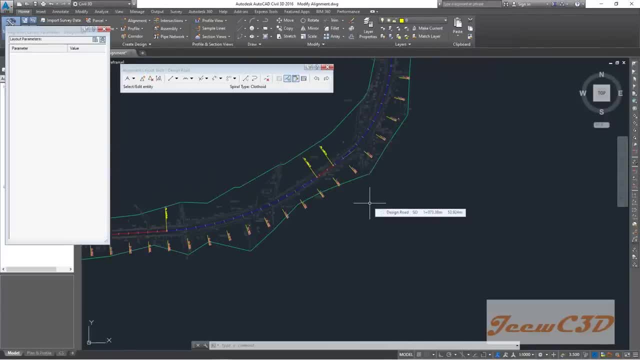 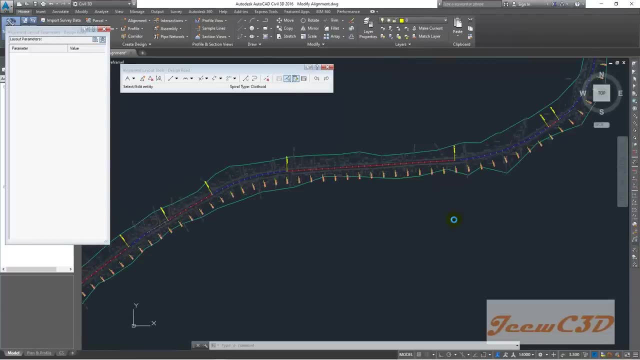 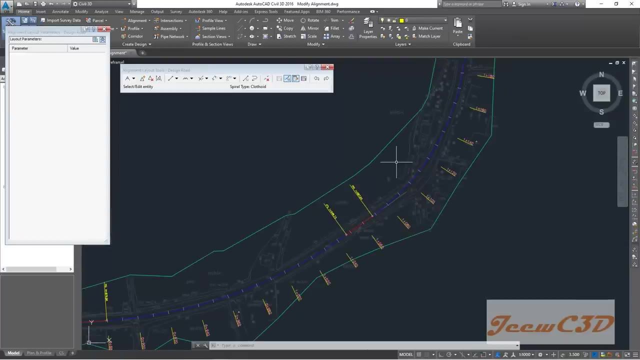 And there is a little bit of a hard time here because of this Compound curve, So we couldn't avoid this one. because we are going to avoid this one, Then it will create problems to the existing houses, So you have to be careful about that. 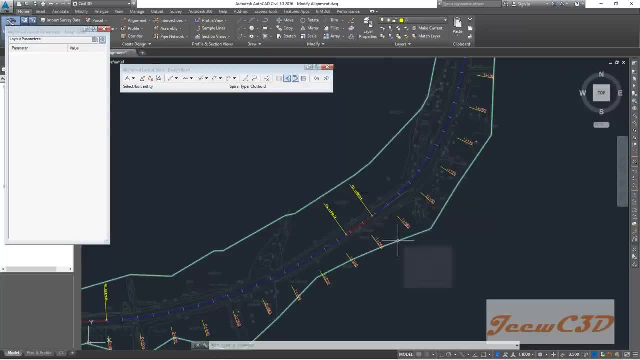 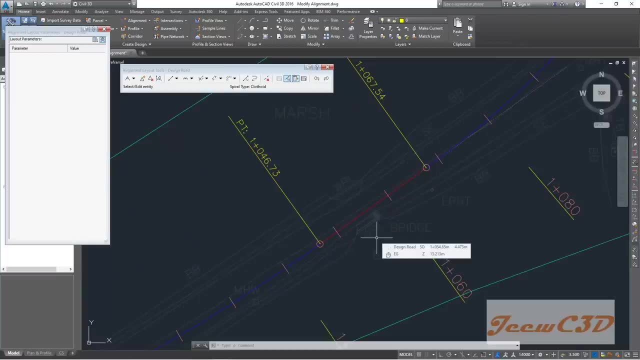 That is why we use this compound curve. Also, in this location we have a existing bridge, So that would be Better to have a straight here because There is a curve, The bridge, The construction of the bridge would be not easy. 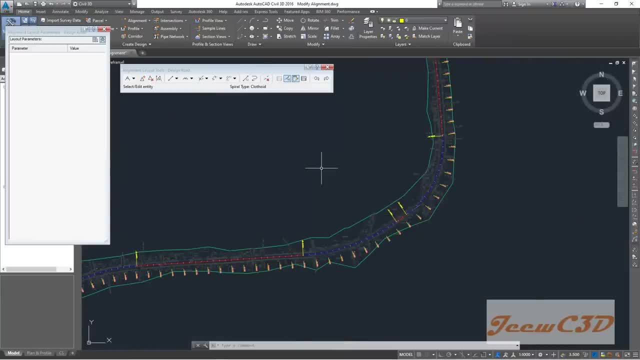 So So far we have finalized an alignment. In the next video we will see how to create the vertical alignment. Before that we will be learning how to create surface profiles and profile views. So Also we have to know how to apply super elevation. 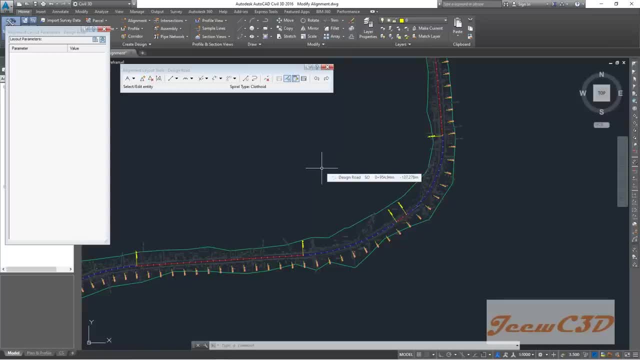 I will be telling that in a later video. In the next video, what we will be looking at is applying the creating the vertical alignment for the horizontal alignment. So far we have created the alignment and finalized it. Now we haven't saved the drawing yet. 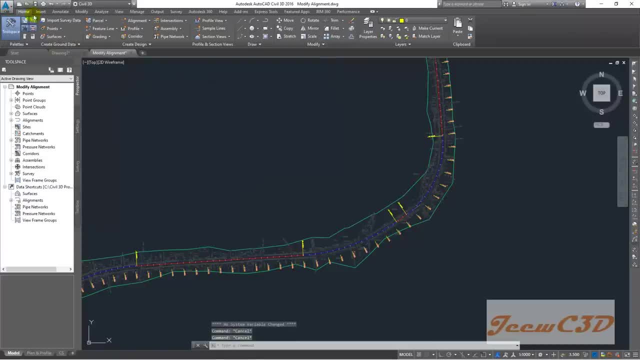 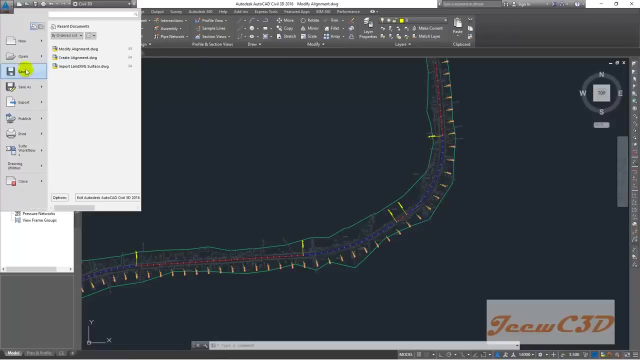 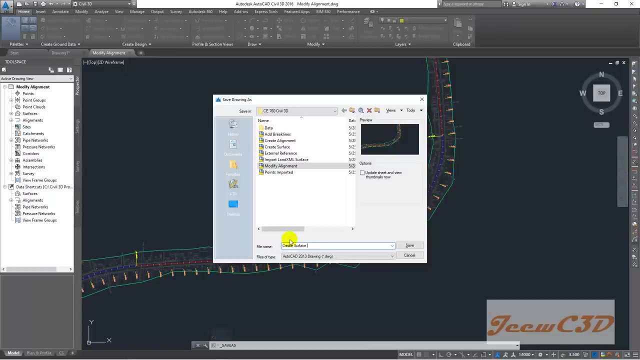 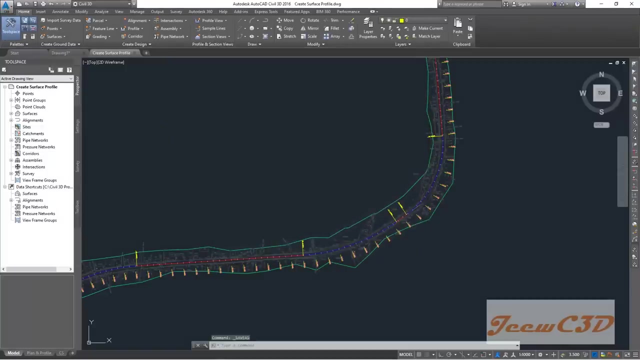 So I will close these things And will save the drawing from here Save, Then I will Save this drawing as Here Surface profile. Then I Now what I am doing is I am creating what is called. 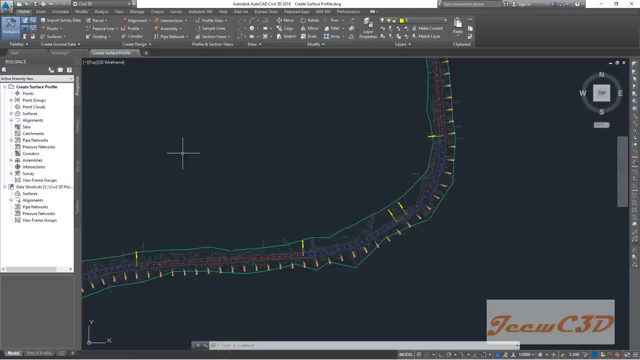 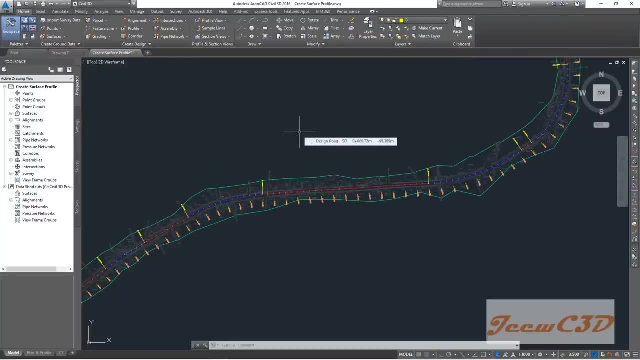 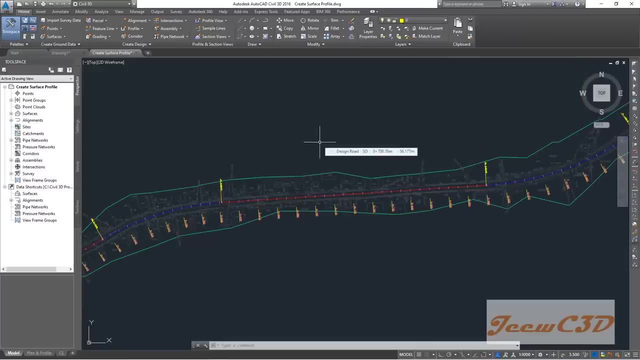 Surface profile Type. Now we have created alignment On the top of the surface. So You have the alignment, You have the surface. You don't have any connection between Alignment in alignment and surface. By creating surface profile means we are creating the 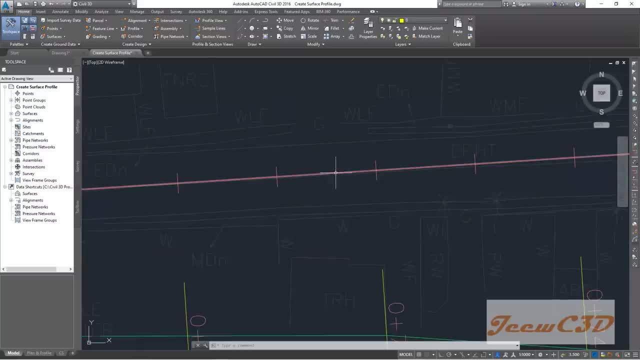 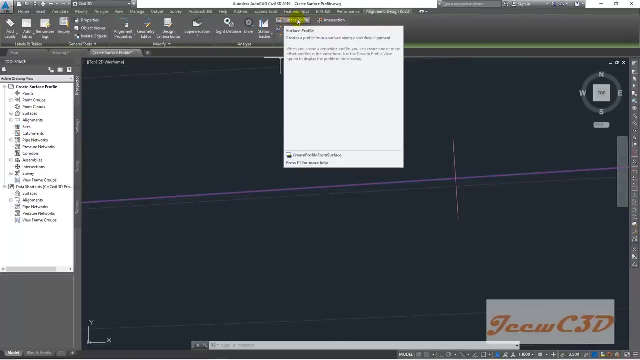 radiations of the surface just underneath this alignment. That means we are extracting radiations of the ground surface underneath this alignment. So to do that, we click this alignment and we click this alignment. Then, from the perspective- sorry, from the ribbon you have- 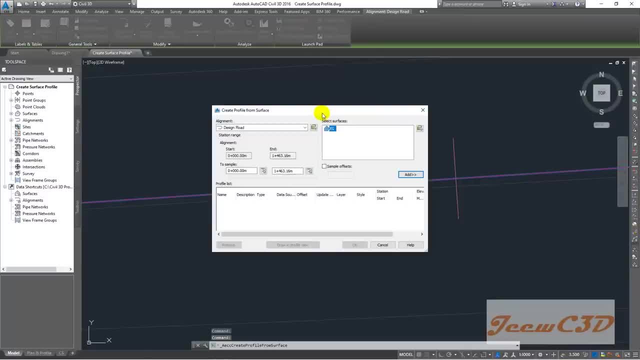 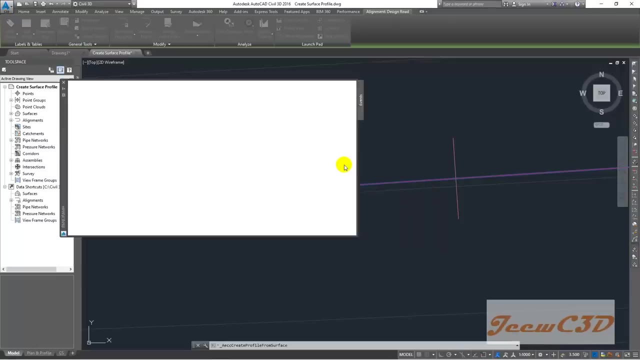 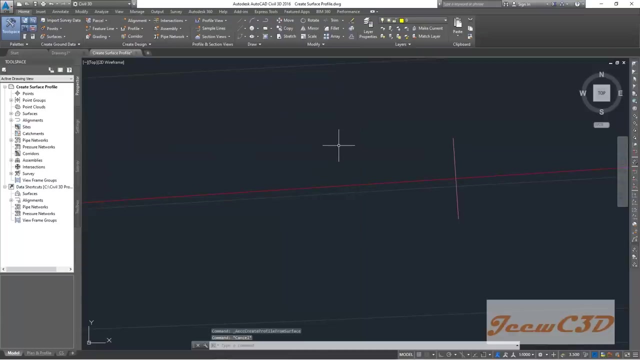 surface profile. You click here, Then it is asking for your alignment and the surface is here. You click. you click add here, Then it will show this. So your alignment would be given the radiations of the surface, but we can't see them. still We have. 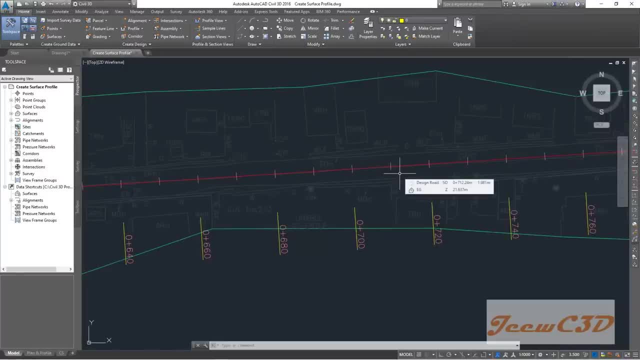 to create the profile to see these things. So in the next video, I will tell you how to create the profile view. So what we have done is created the surface profile. That means the radiation of the surface just underneath the alignment. Before that, I will ask you to save the drawing. 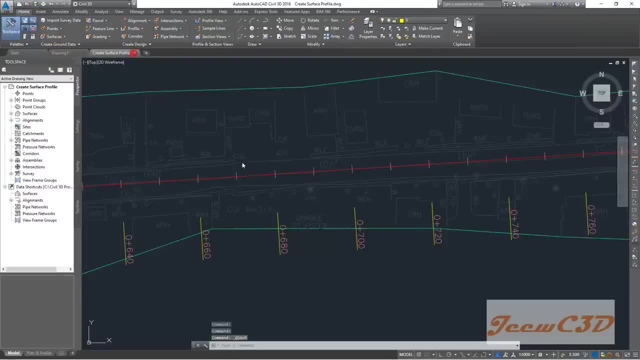 and let us close it. In this video we are going to create the profile view, So we will see what is the profile view- A profile view- moments later, So before that, we have to open the drawing we required to create the profile view. I am going to this application menu browser. 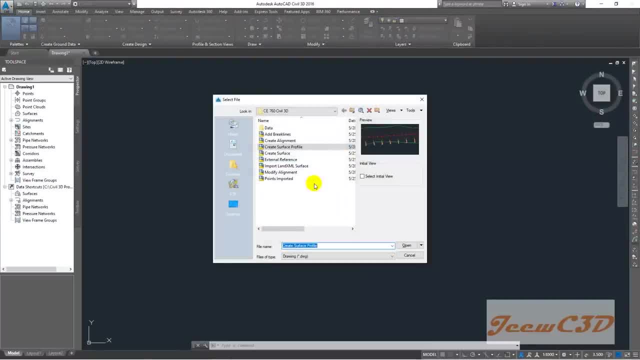 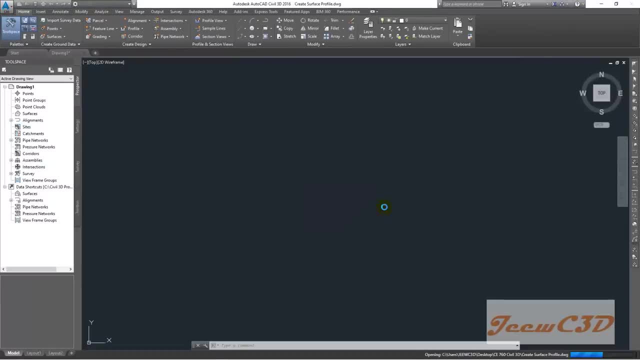 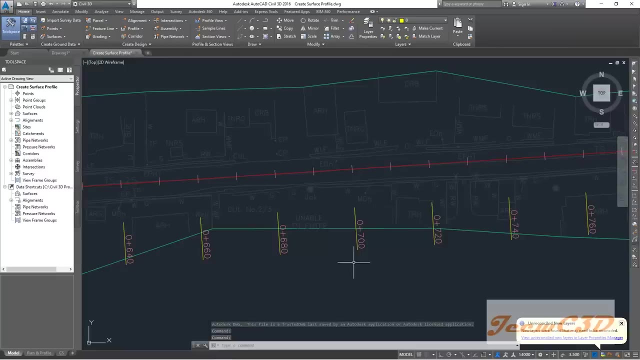 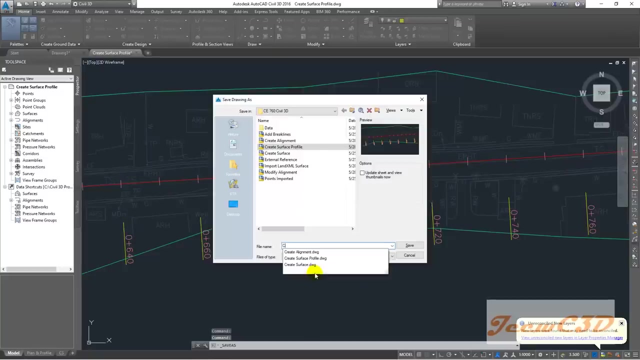 and go to open here, and I will select the last saved drawing, which is create surface profile. Click open Now. this is the drawing which we are creating. we created surface profile, So I will save this drawing as. save this drawing as create profile view. 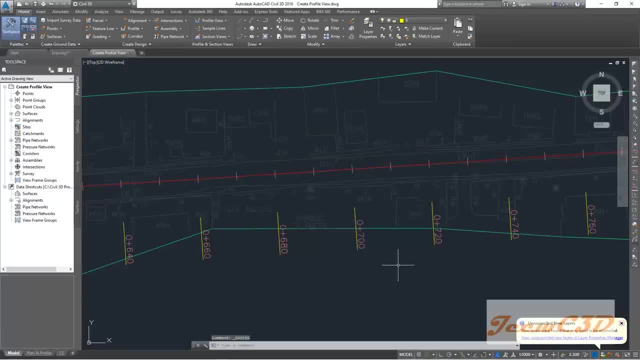 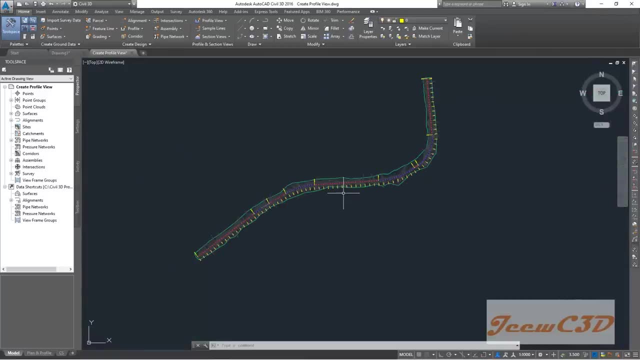 Let's click save Now. what I am going to do is create a longitudinal section along this trace. That means I have a curved road here, but I will mark the road stations on a straight line like this, and I will mark the elevations and draw a profile. That is what we are called. 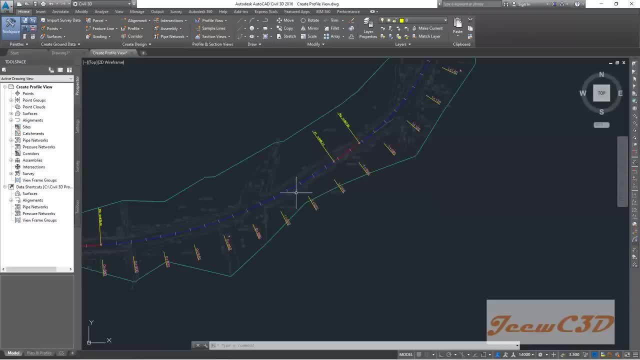 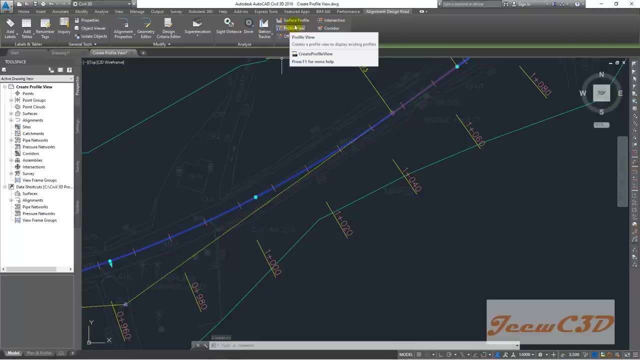 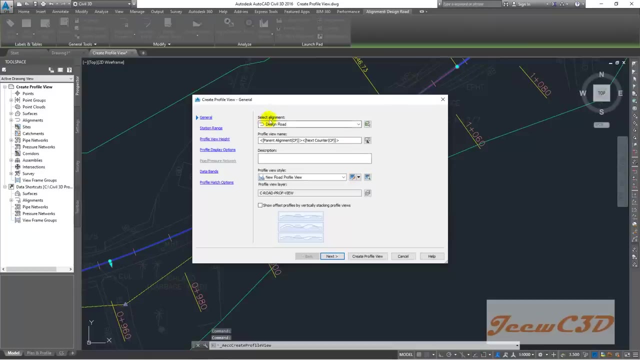 creating a profile view. To do that, I select the alignment. go to profile view from here, you will get this kind of figure. Go to profile view from here. you will get this kind of figure. Select profile view. Then it will give you the alignment name. 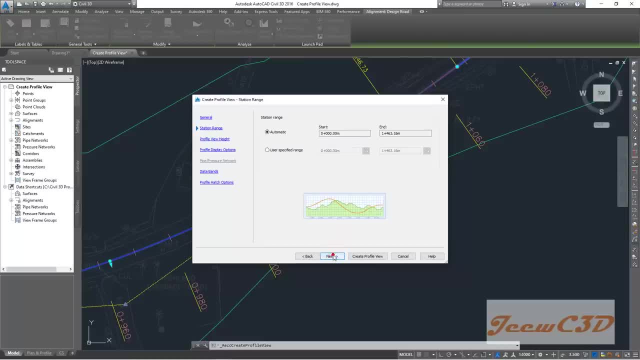 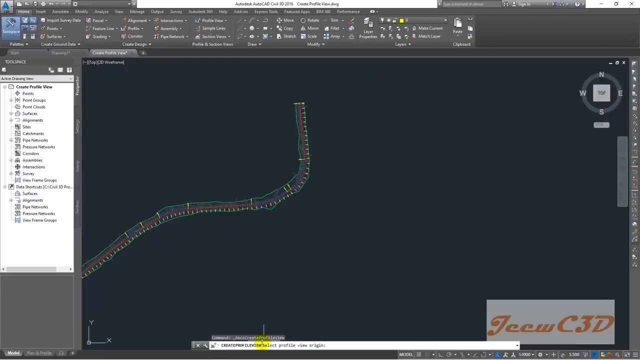 This kind of things will be appearing. You don't have to change anything, Just press next until you come to this point. and again you have to press next and click this create profile view button. And it is asking: Select a profile, the origin. That means it is asking for a place to place the 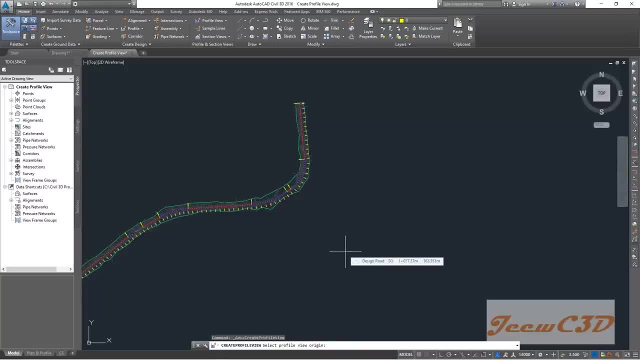 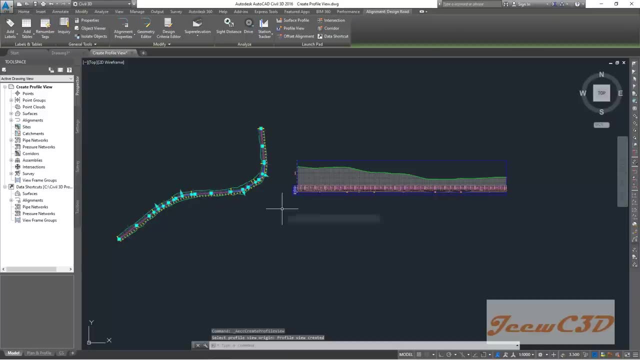 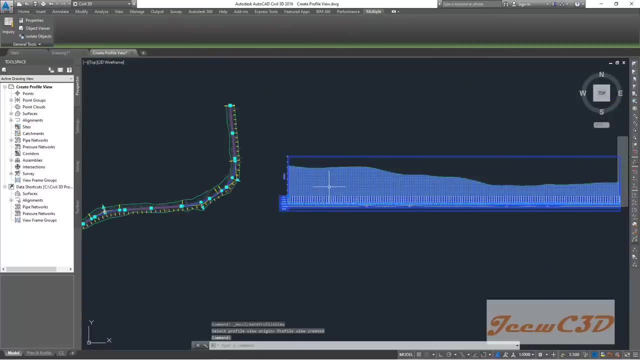 profile view From the right side somewhere here you click It will be. the profile view will be appearing like this. so if you don't like the location, you click this profile view. Sorry, if you see my ribbon it says small tree. we will keep that as as a view and don't need this page. 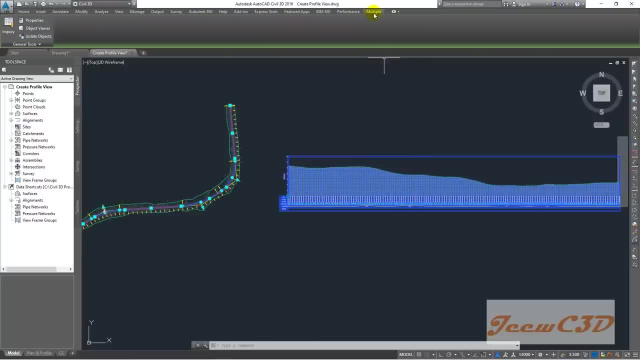 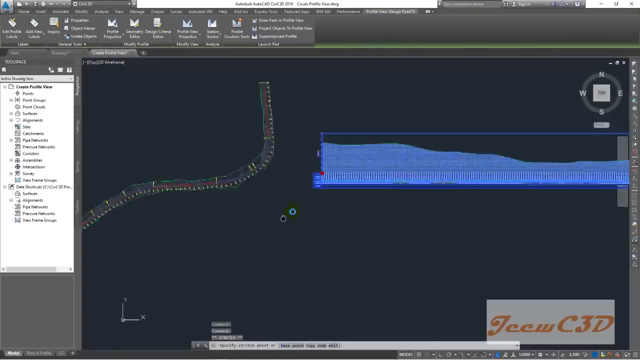 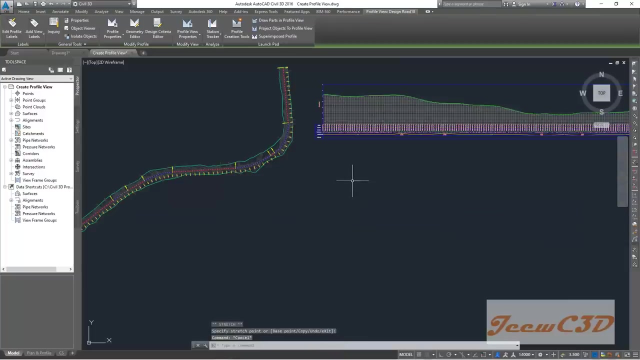 option we will click after that. that means you have selected my profile view and alignment both. so I have to press k8 and again select the profile view. then I can move it from this grip here I can move. you have the grip here. yeah, you can move it if you don't like the place it was located, so you. 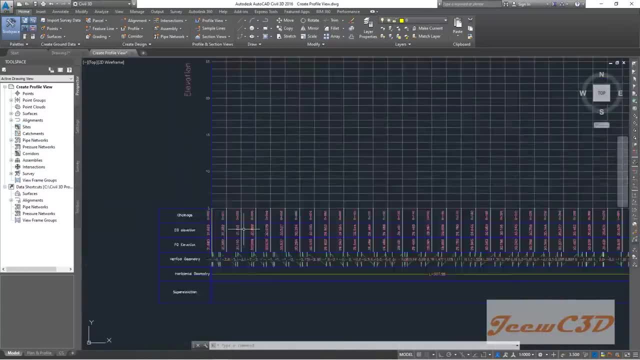 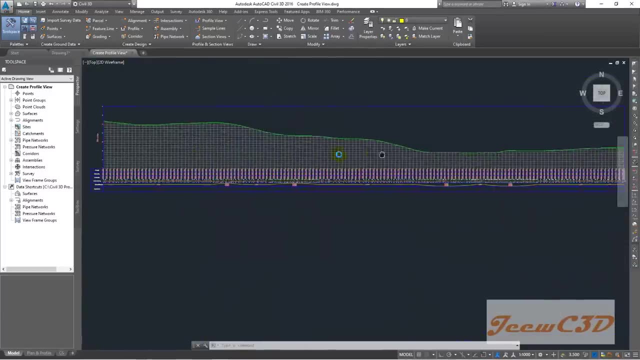 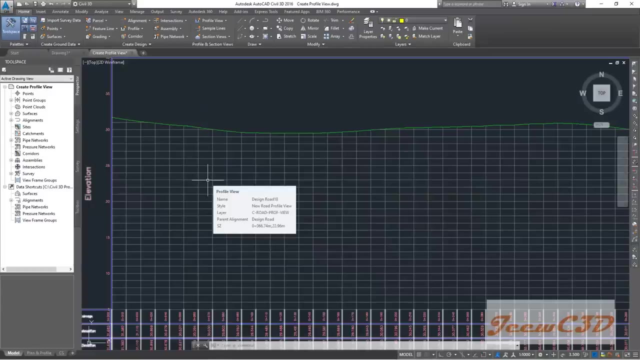 can see at station 0 this elevation, station 10 this elevation, because these are marked at 10 meter intervals. so you can see kind of a smooth throat here, but it is not smooth at all. we getting this kind of a smooth throat because we followed the existing centerline. 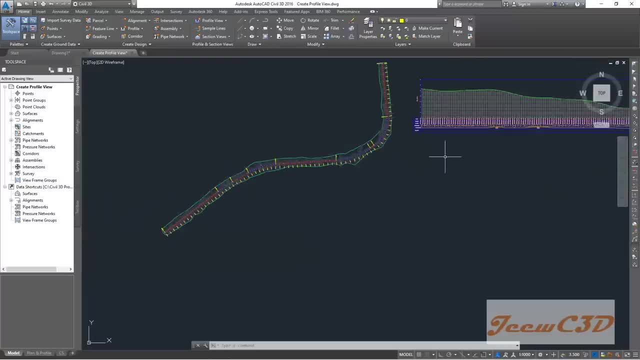 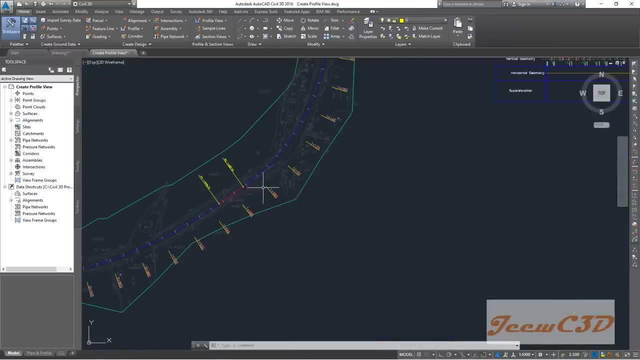 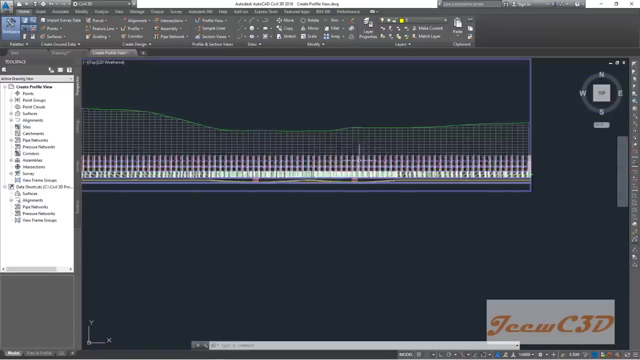 because existing centerline is kind of a smooth throat. that is why we are getting some kind of a smooth throat, smooth section, smooth road section here. so if you think of a place somewhere here, 1 plus 100 or 1 plus 110, somewhere here, you may be having kind of a odd shape. let us see whether 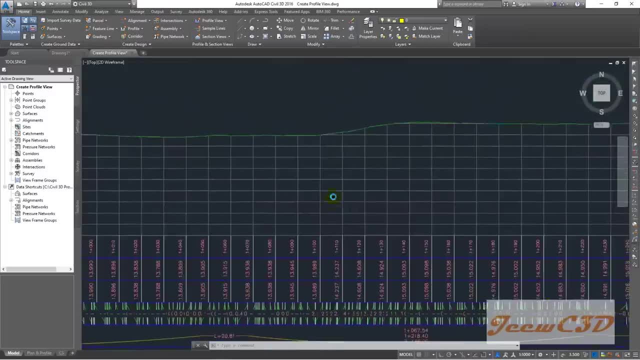 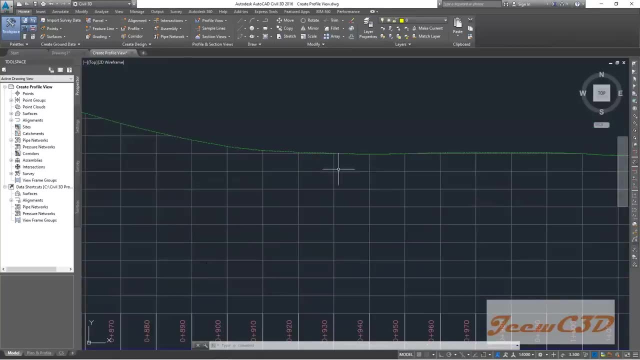 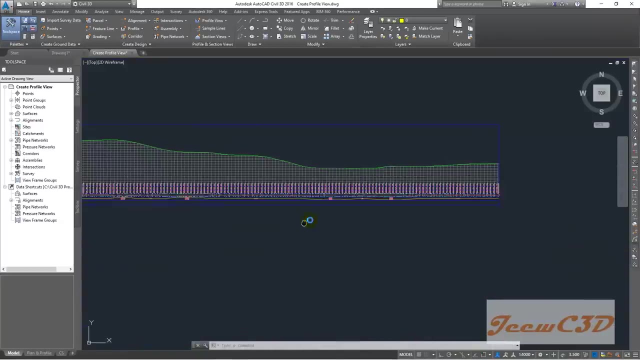 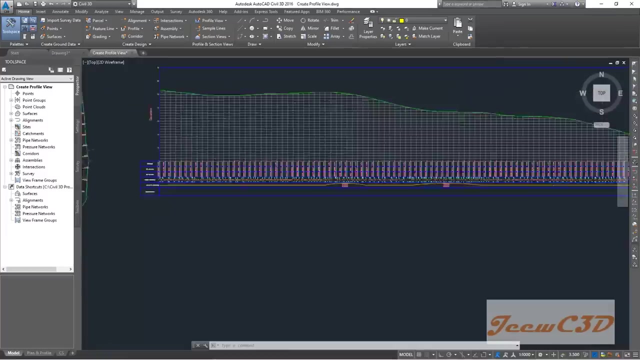 it is happening. yeah, you see, some kind of odd shape is happening here. so also you can see some places there may be odd shapes because the alignment is going outside. so that is how to create a profile view. you have the elevations of the alignment in a profile grid. 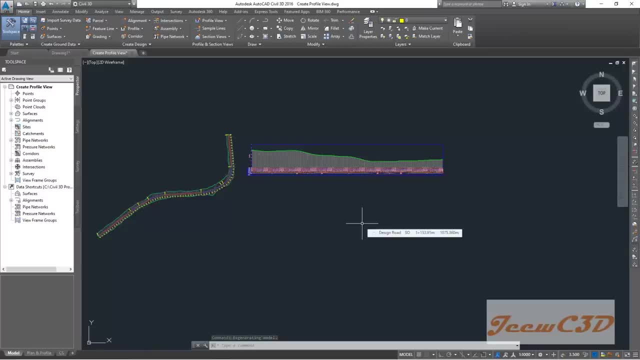 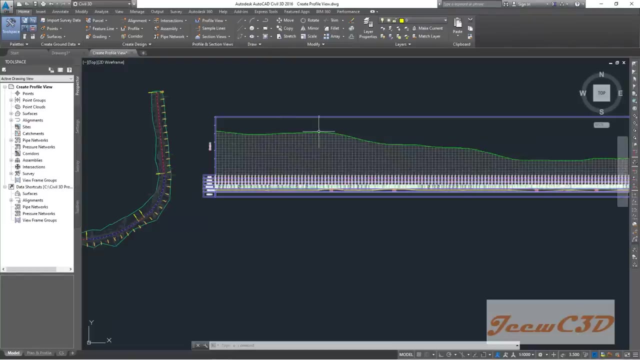 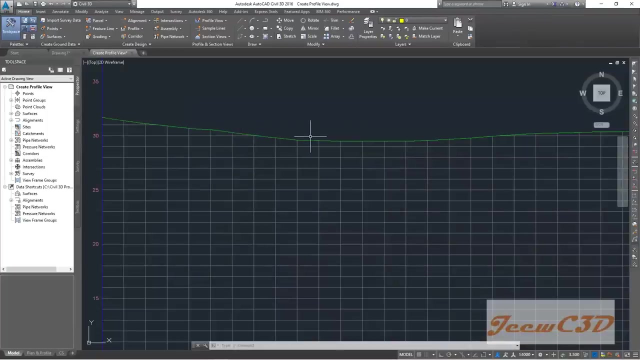 so by that you can get a clear idea of the elevations of your road, existing elevations of your road. In the next video we will be designing a new road on top of this profile view. that means we are creating a new profile. we have the surface profile here. surface profile means: 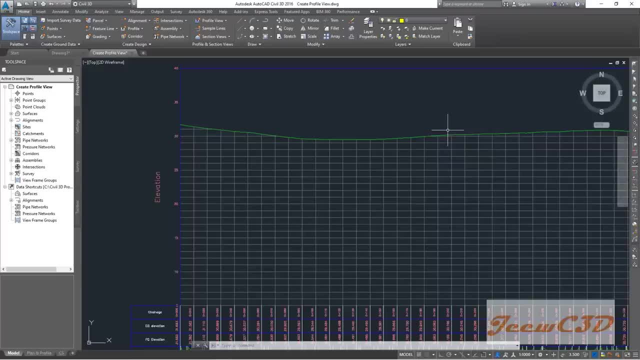 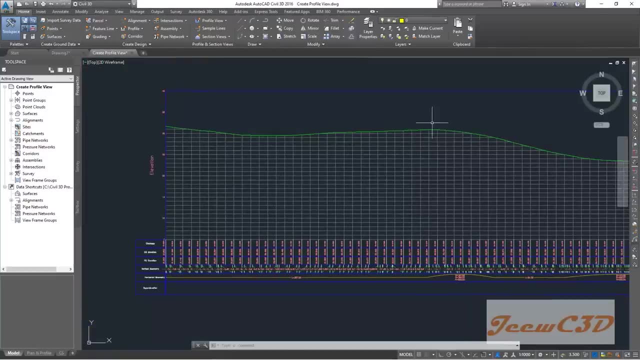 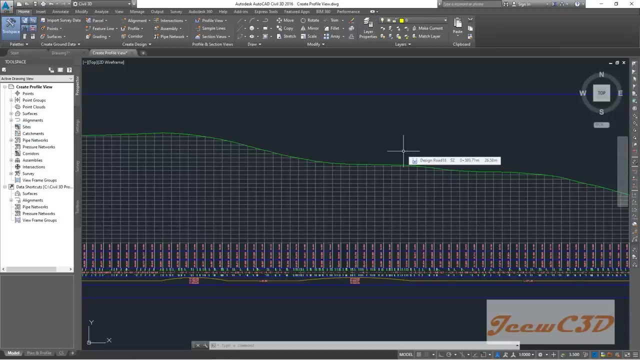 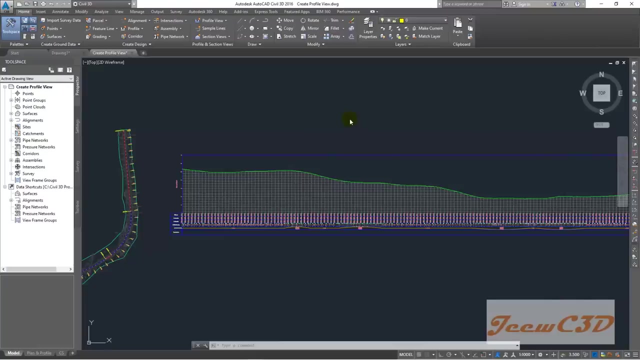 the elevations of the existing alignment in that ground. so we will create a new ground or new surface to follow this existing surface. So in the next video we will look how to do that. in the previous video we learn how to create the profile view. in this video we are going to create a new vertical alignment. 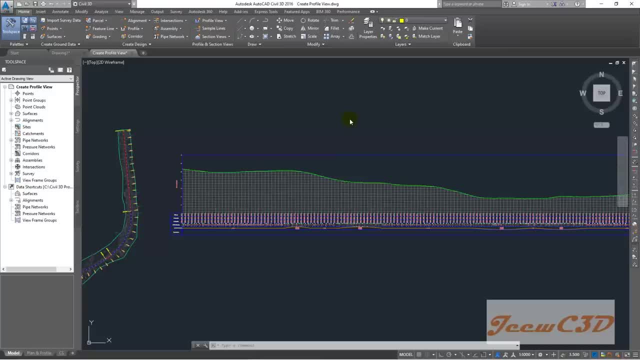 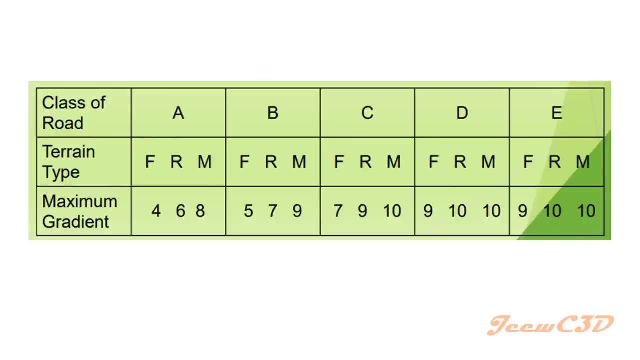 to our road. so before that, we need to know what are the guidelines we have to follow to design the profile. So we will look at that now. since you know, road is a two lane, two way road and it is on a flat terrain, we will assume that this is a b class road. yeah, you can go the gradients. 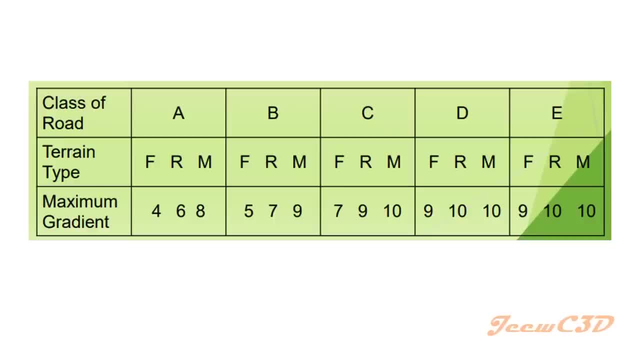 or the slope of the road up to five percent. So we will look at that now. Since your road is a two lane, two way road and it is on a flat terrain, we will assume that this is a b class road, So you can use gradients of two, five percent. so that is one kind of maximum, one kind of 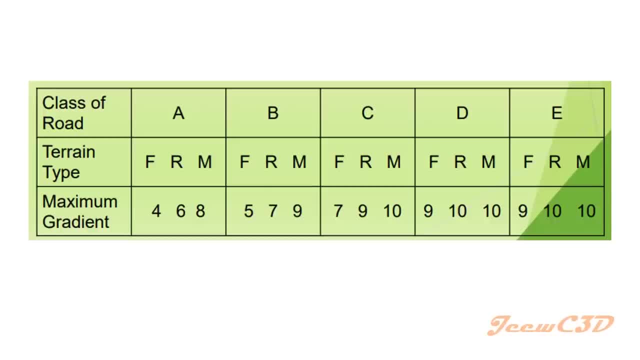 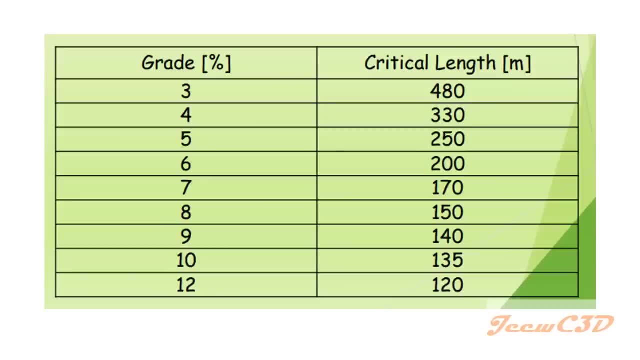 constraint you have to maintain in this road. The maximum you want you to know is five percent, then then you are going with that gradients. you have to follow the critical length. so if you are going with Three degree gradient, but maximum gradient, three degree gradient, 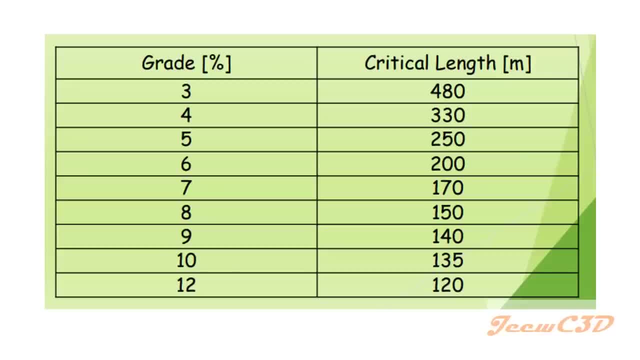 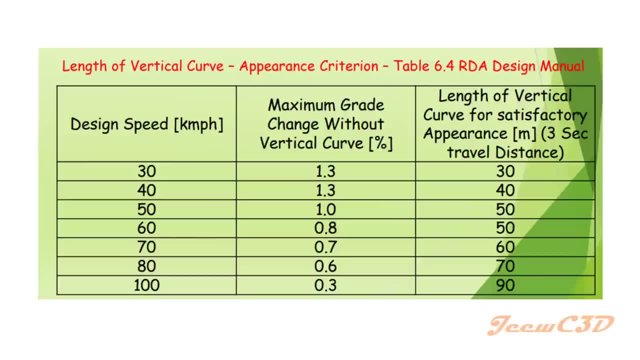 length you can go is 408. likewise, then, you have to follow the curve length. for appearance criteria, since we are using the design speed of 60 kilometers per hour, you have to follow the length of the vertical curve, which is 50 meters. so you have to use the length of the vertical curve of 50 meters or higher to get the 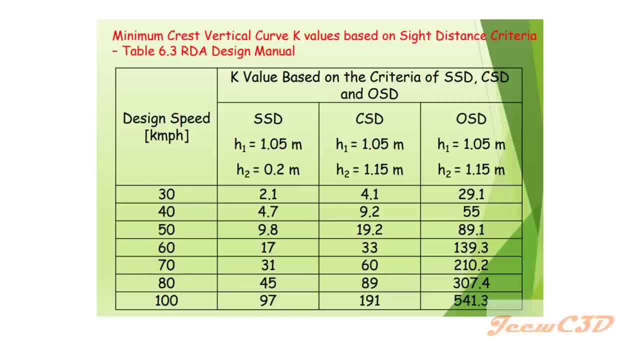 appearance criteria. so for a crest curve you have to use the side distance criteria to be satisfied. so if you are, since we are designing the road for 60 kilometers per hour, side distance should be 17 in terms of the K value. for crest curves that means: 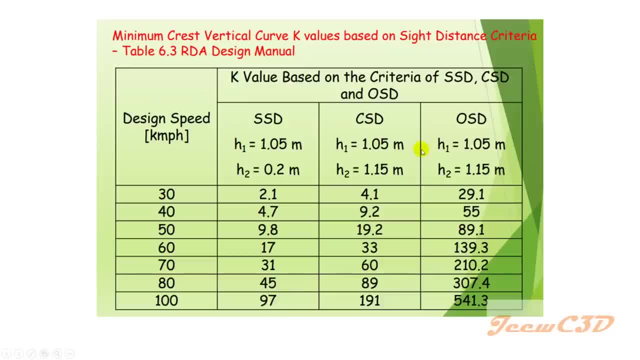 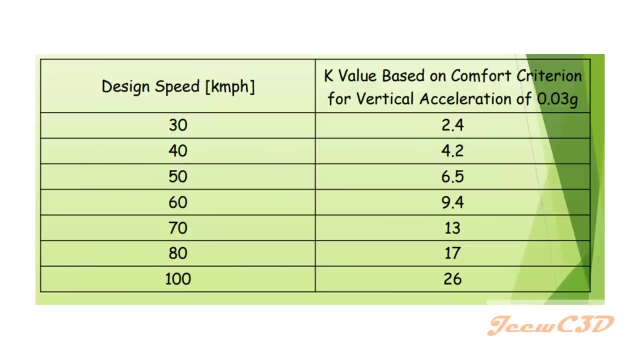 curves like this, vertical curves like this. so we are looking only at this SSD or stopping side distance criteria. so your K value should be greater than 17. then for crest value, you have the comfort criteria. that K values. you have the comfort criteria. you are so great K value should be mine. 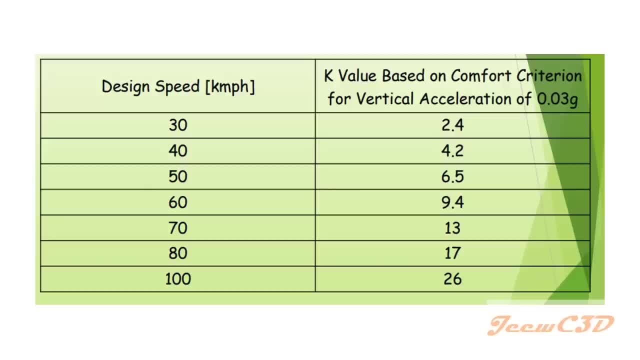 so great K value should be mine point four. so when you are comparing nine- point four- and senator, whether you have to go with 17 OSEOWOU whole day 시간, 섭 m понимаю that curve will not satisfy SSBE 5. 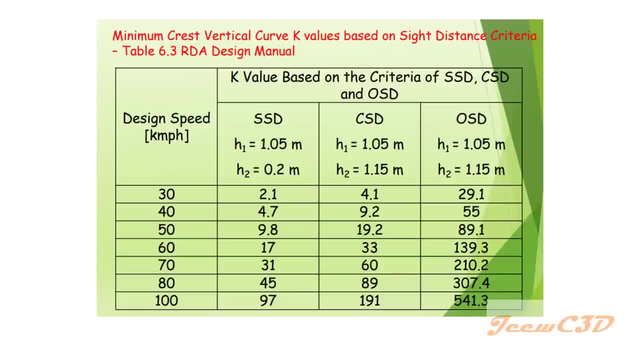 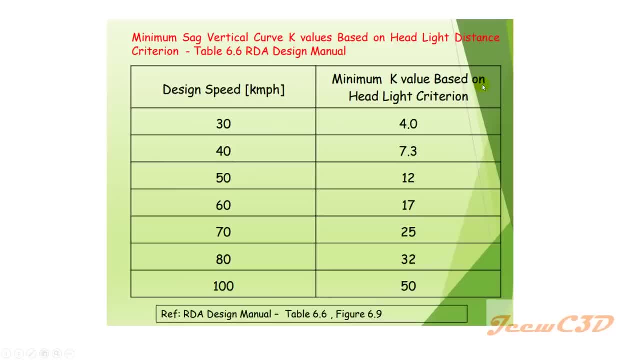 when 3757, if you go with 9.4, if that code will not satisfy SSD criteria, so in that code will not satisfy SSD criteria. so in any case, when use any of these values, well, 0, sec, 10, 13, you satisfy the SSD criteria. you will automatically satisfy the comfort criteria. so if you are using 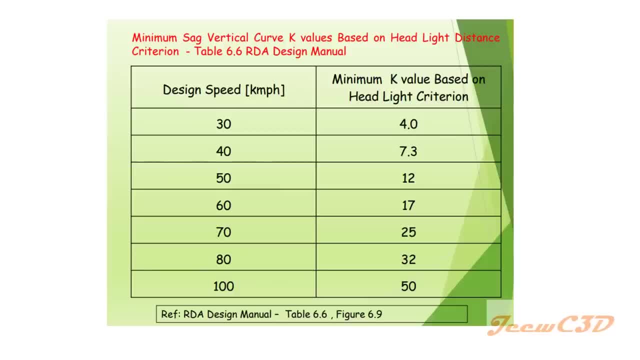 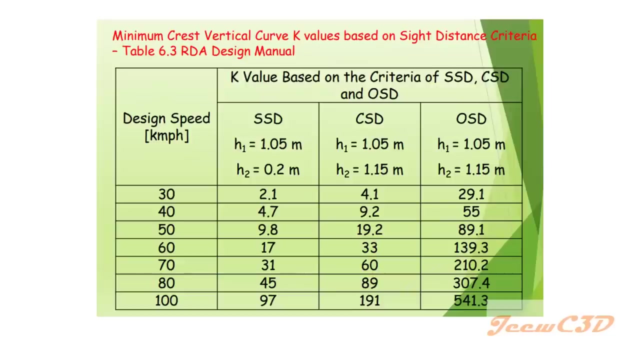 side vertical curves you have to satisfy the headlight side distance criteria, which is 17, so you have to use 17 for a sub vertical curve for 60 kilometers per hour design speed. so as well, you have to follow the SSD criteria. that one is also 17 for the side curve because 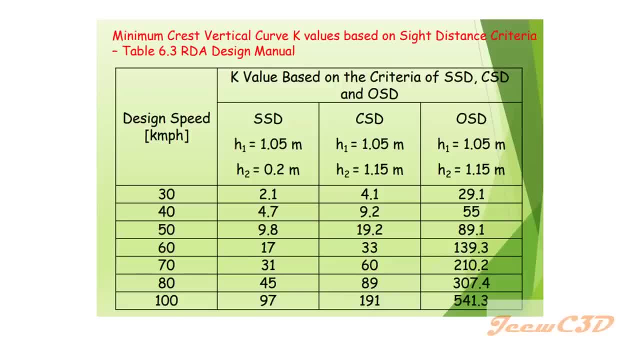 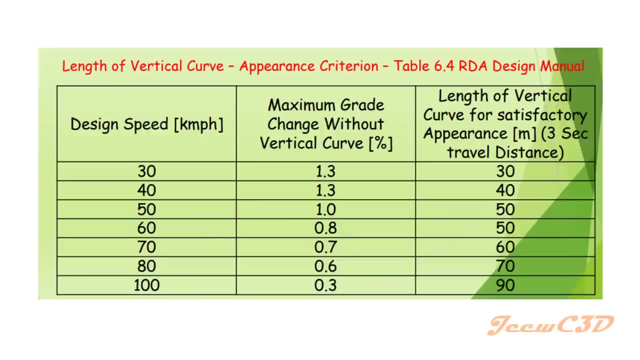 i told you we use headlight and SSD criteria as same in the picture. however, for the side curves you have to satisfy the appearance criteria also, so in that case you have to follow this one again. you have to have a curve length or vertical curve length of 50 meter or greater to satisfy the 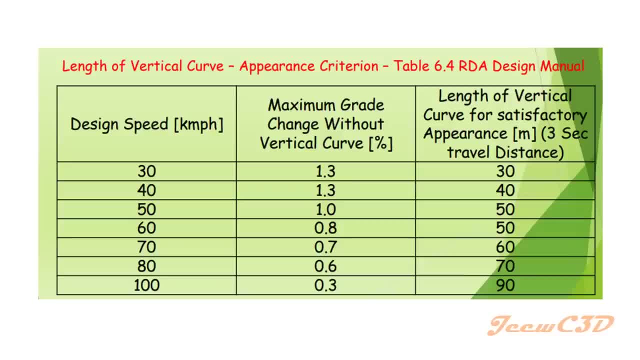 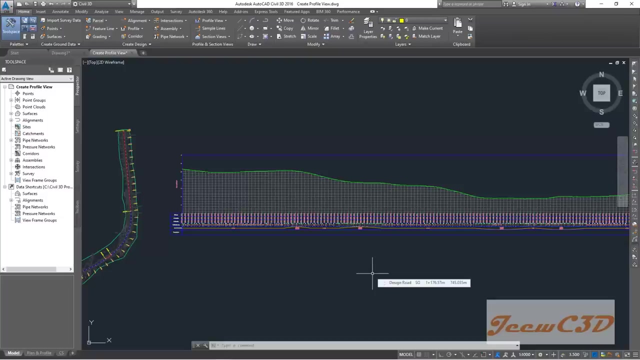 vertical curve length criteria for 60 kilometers per hour. so that is the kind of design criteria we have to remember when designing this. for example, alignment for this particular road. this is a way how to design this road. so now we know what are the criteria we have to follow to design this road. so with that in mind, we will start. 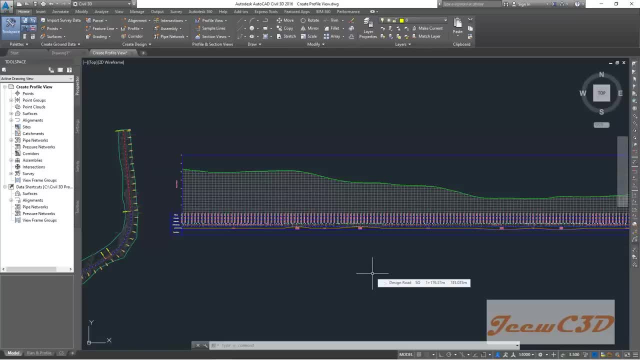 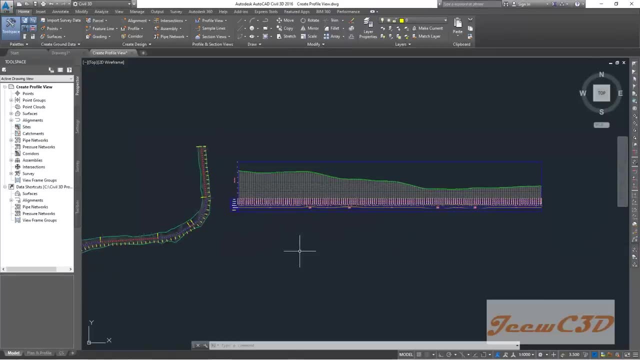 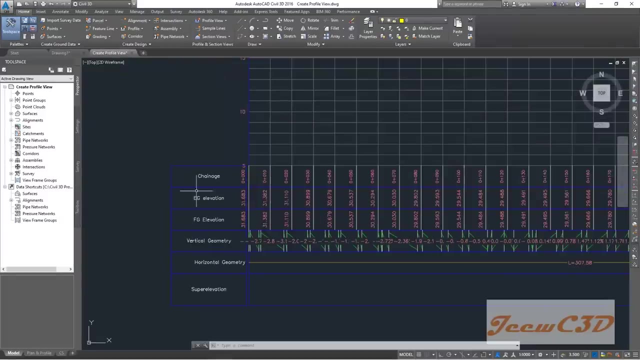 designing this vertical alignment. so before that, we will talk about something new in this profile view which i've forgot to tell earlier in this tell in the last video. you have some bands here: chain edge- EG elevation, FG elevation- vertical geometry- Horsham region. 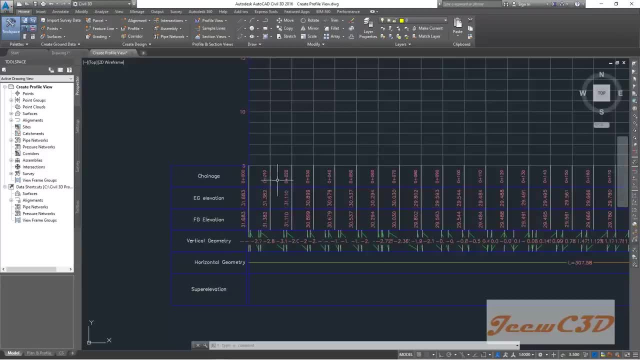 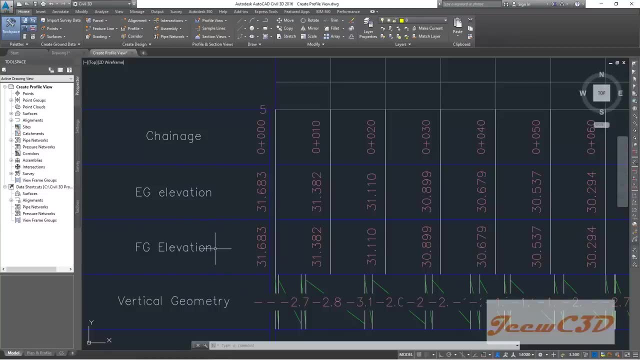 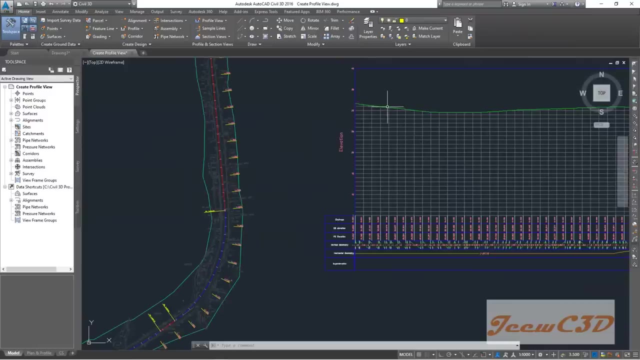 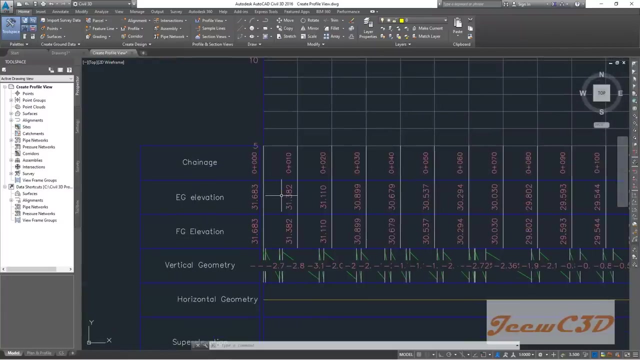 and super elevation Chain. edge means the length or station of the road. EG elevation is the existing ground elevation. FG elevation is the finished ground elevation. You can see both these elevations are same because only we have existing ground model, existing ground profile, So it will give both elevations as same. So once we design the vertical 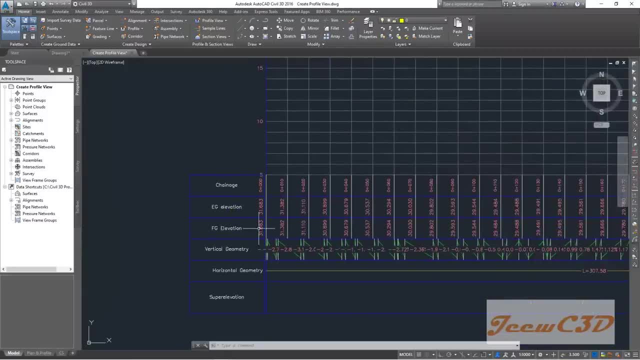 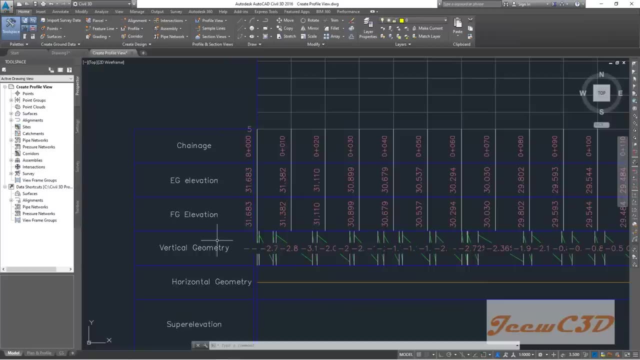 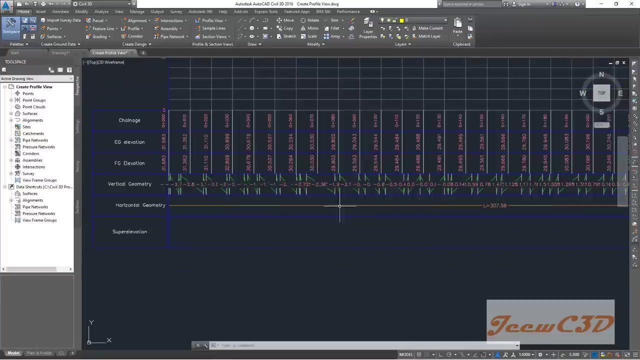 alignment here you can apply that vertical alignment to this FG elevation band so that these values getting something different than this one- So this vertical geometry will also be changed- can also be changed once you apply this vertical alignment criteria here. So here, this horizontal geometry, you can see we have the straights, then you have the. 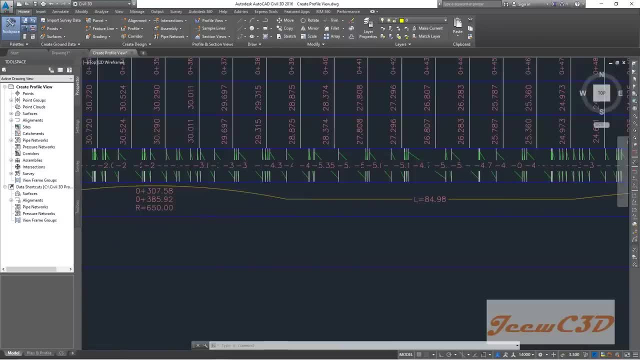 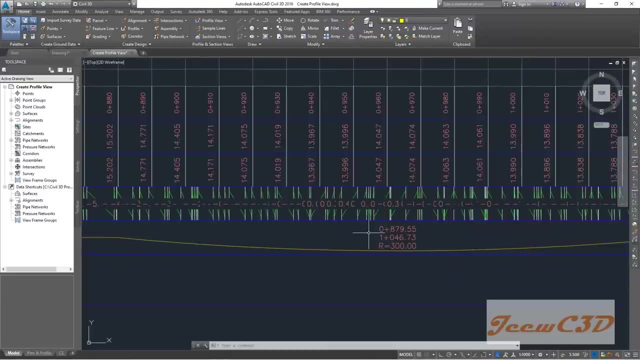 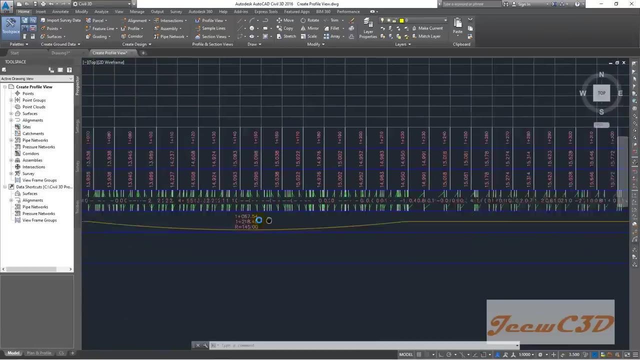 curve criteria: 650 curve we used And again we have a straight, then again you have a 180 curve. Again you have this 300 and this 145 curves which we had earlier when designing the curve. So it is a summary of the horizontal alignment in this band. 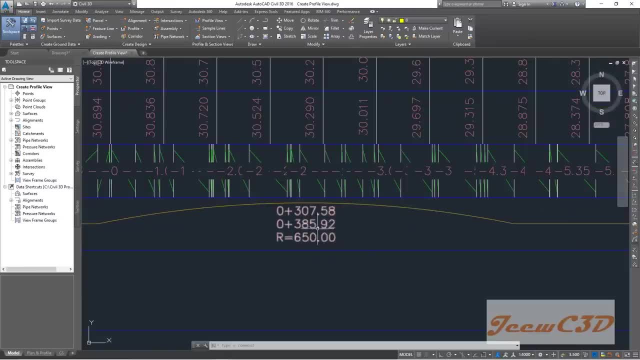 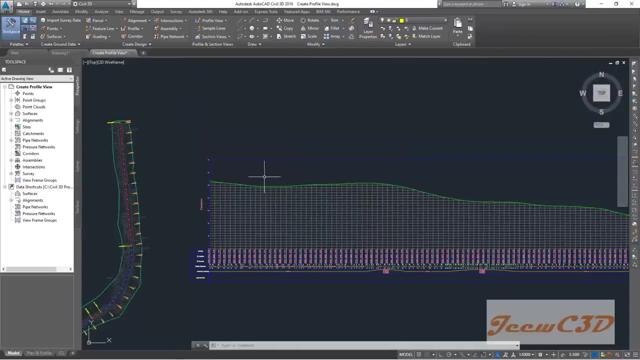 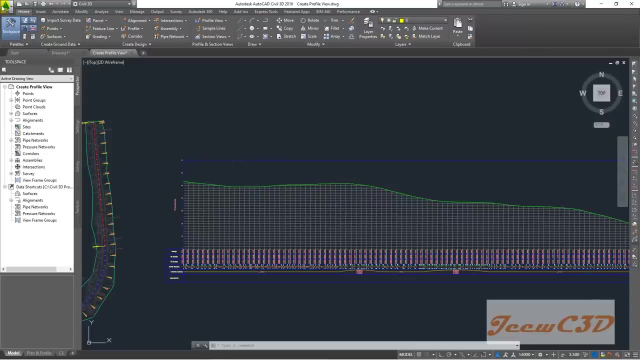 Again, it shows where the curve starts and where the curve ends. This is the starting station, this is the ending station, likewise. So, with that in mind, we will start drawing the vertical alignment. Before that, I will save this drawing as first I will save this. 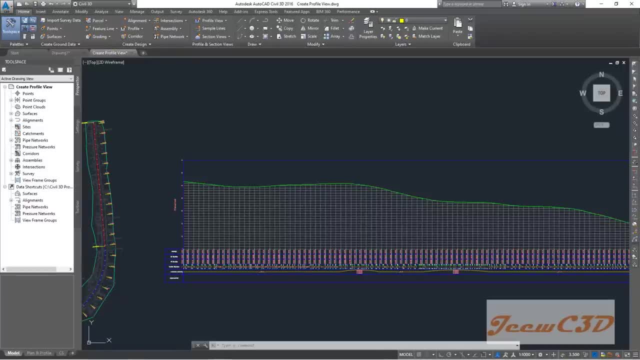 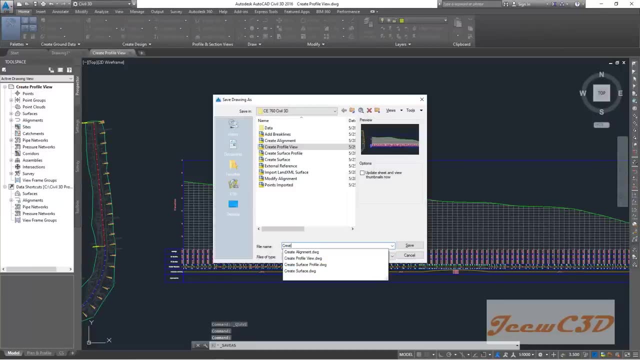 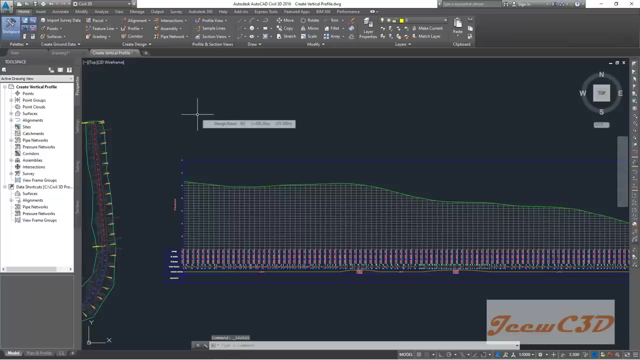 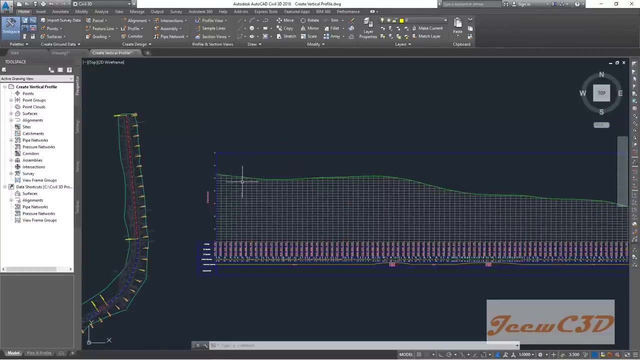 drawing and then I will save this drawing as create vertical alignment. So this is create vertical profile. Okay, save. So this drawing will be continuing with over dash: create vertical profile. Now what I am going to do is select this grey lines. 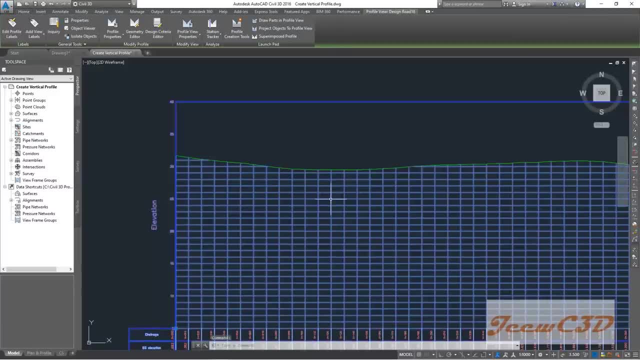 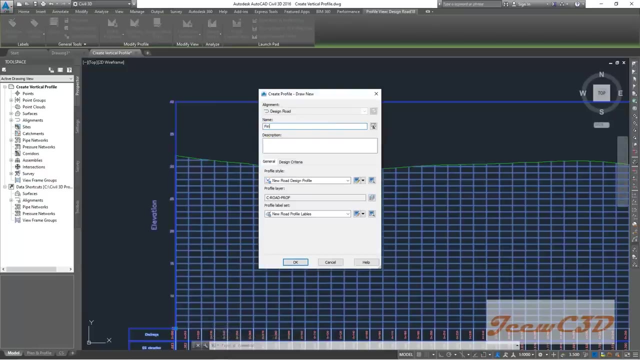 here. So over the profile will be get selected In here. I use this profile creation tools, this option. So let us say our profile name is finish found, So you can have a description here if you want. Otherwise I will make these. 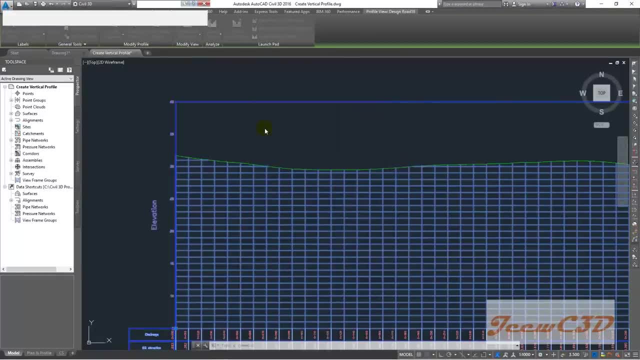 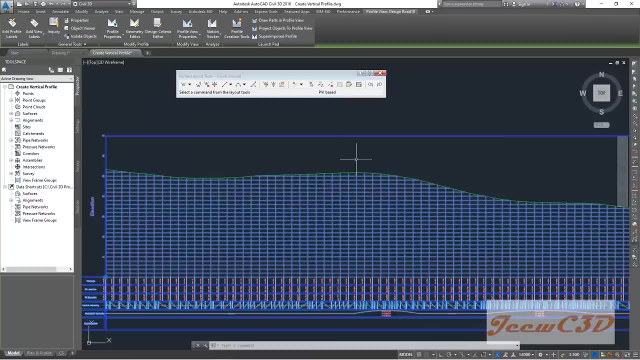 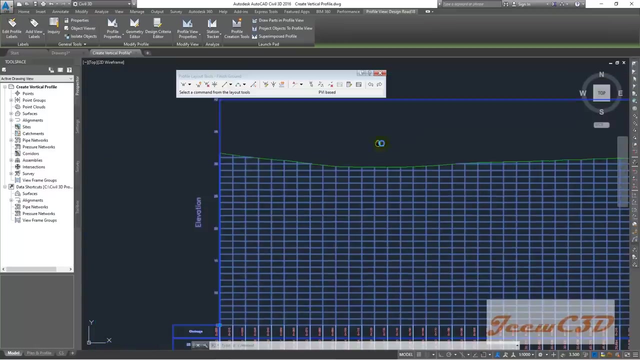 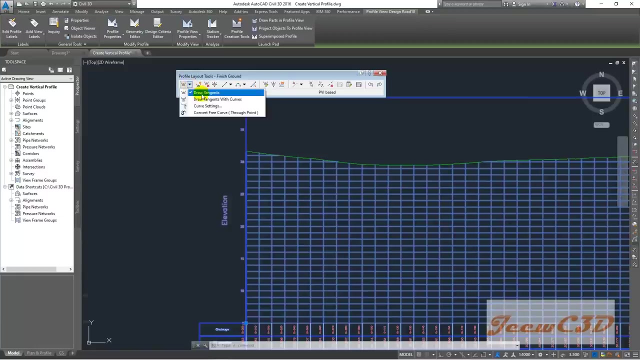 values default and click OK. Then I have code. You have this code. You have this toolbar, like we had in alignment. Now I am going to draw this vertical alignment on top of this horizontal alignment, So you have to use this tool here and go to draw tangents. 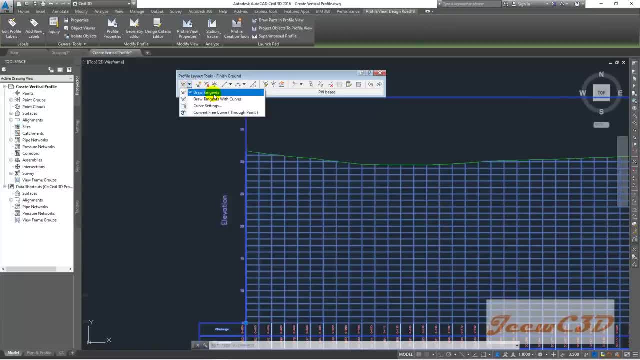 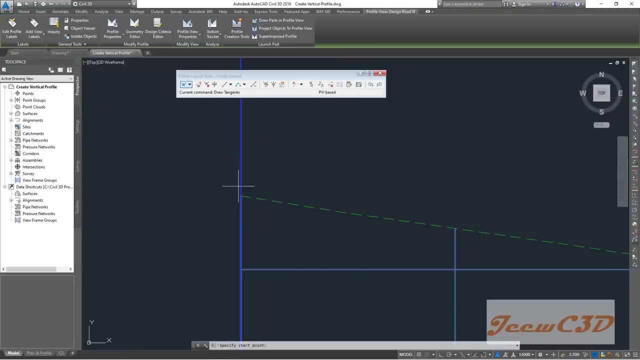 So we, first we will only draw the tangents And then next we will add the curves. So I come here, So I have to find the end point of this. end point means this zero station I have. I do not know whether, if I click somewhere here, whether I will get the end point. 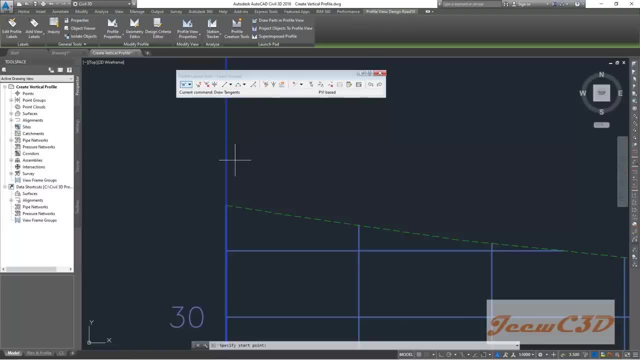 So to do that, what I do is I press shift key on my keyboard, then right click Okay And select nearest, Then it will let you find this edge of this blue line where the starting station is. I will start somewhere above the small amount, above the ground. 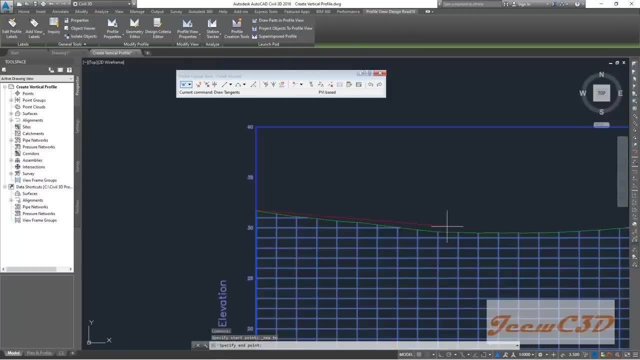 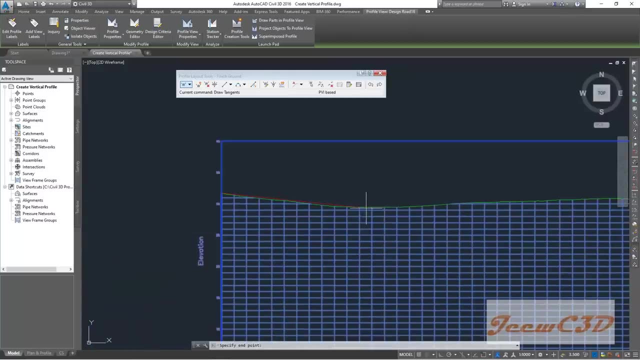 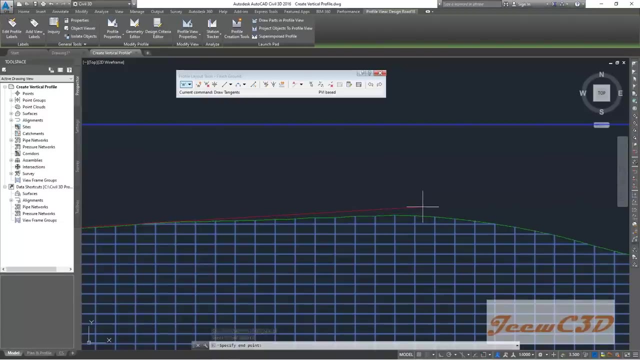 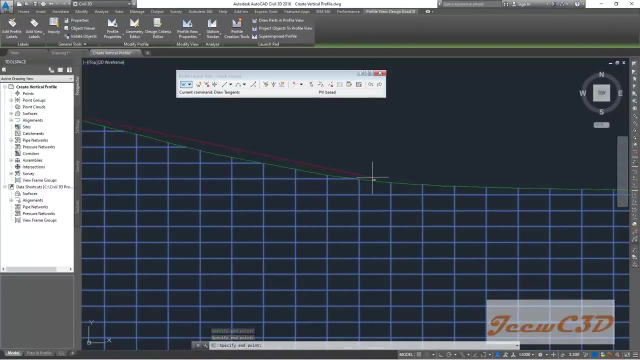 Then I draw this one: We have a sag here, So I will make a sag here. Then again, we have a crest here, So I will have a crest here somewhere like this: Again, I have a sag here. 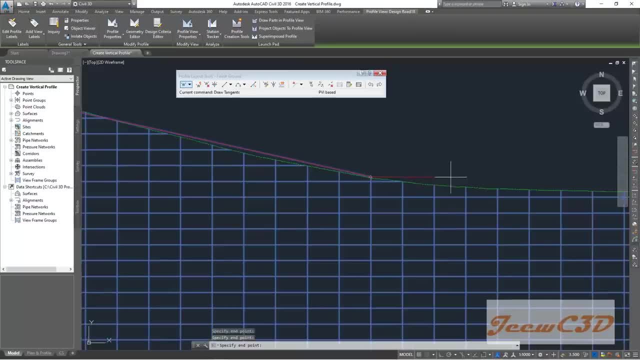 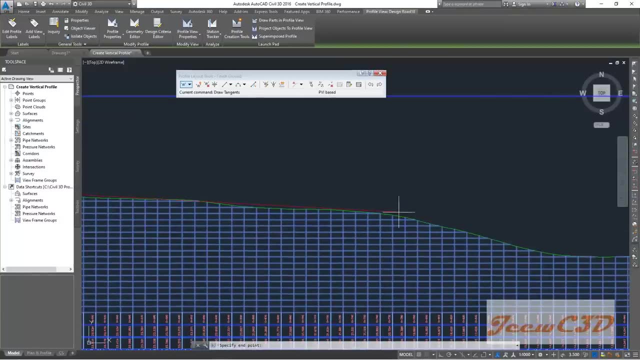 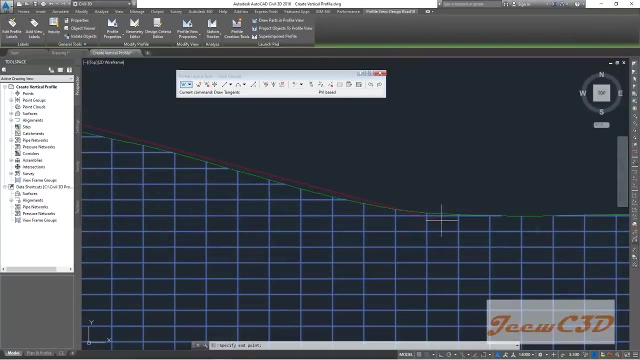 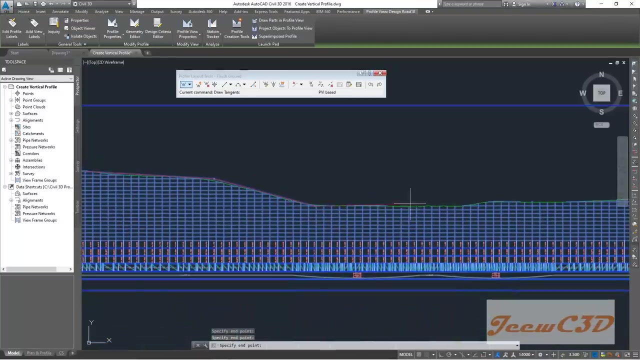 So I will have a small part section here And come up to this point somewhere here. And again I have this sag. Now we place somewhere here, Let us see, And now we have another small curve up somewhere here. 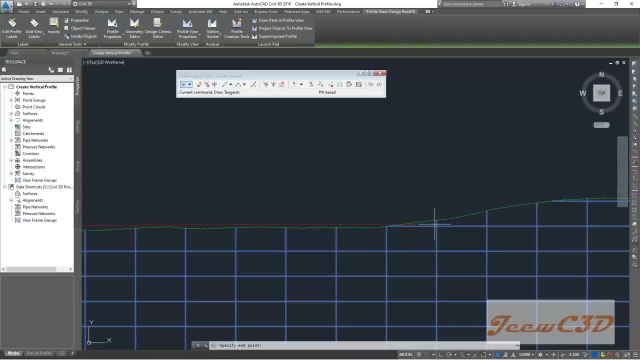 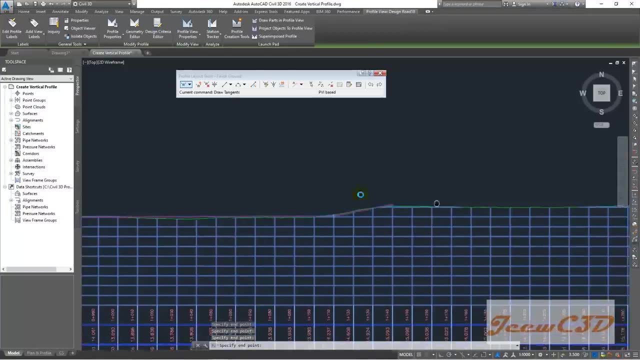 And again, I have this sag here And come up to this point somewhere here. And again I have this sag here And come up to this point somewhere here. We will have it somewhere here, like this. So I am just drawing the follow the ground. 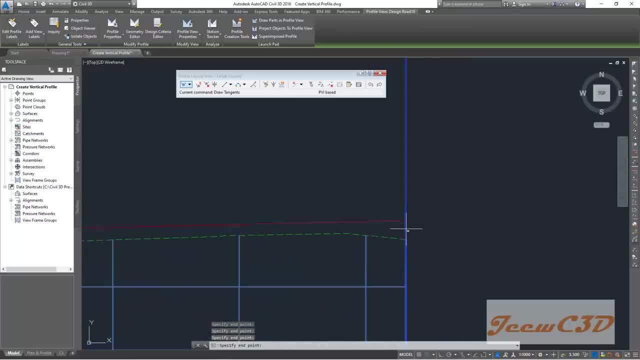 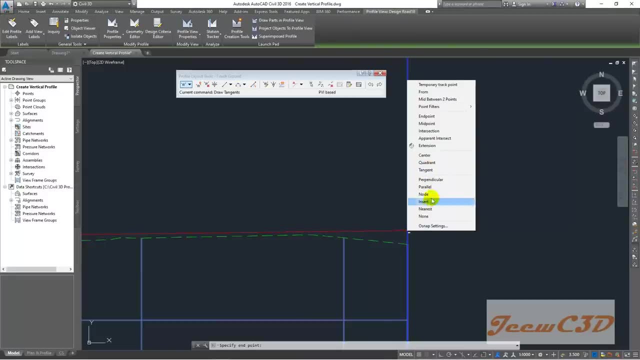 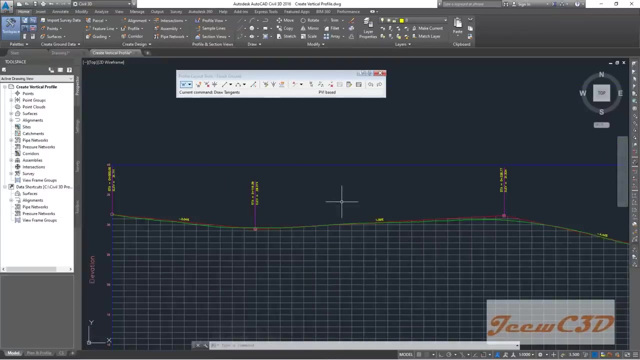 Somewhere here is stop And close it Again. I press this shift key And right click, Go to nearest when I catch the end point and I will finish my row. then press skip. you will see I have created the vertical profile. but in this thing you have to follow a lot of things. you have to 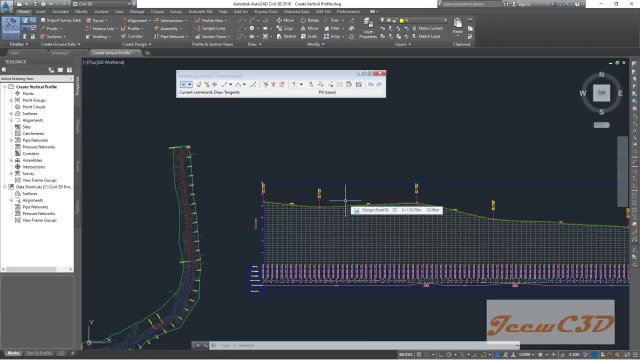 check the vertical horizontal coordination. but you don't have that much of time to take all these things, but I am giving you this small idea about how to create the alignment. so if you are designing the alignment in a project, you have to think of all these factors particularly. 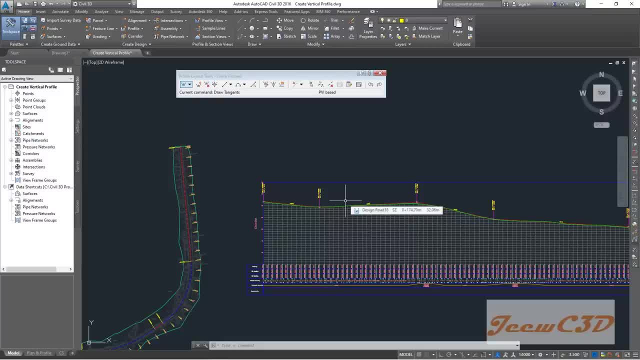 there is a dropping boundaryção and you have to check those profile like that, those locations. and if you are use in a cut section, you ensure that it will not create access problems to the nearby houses. also, if you are using high field locations, it should not cause access problems to other nearby houses because of the 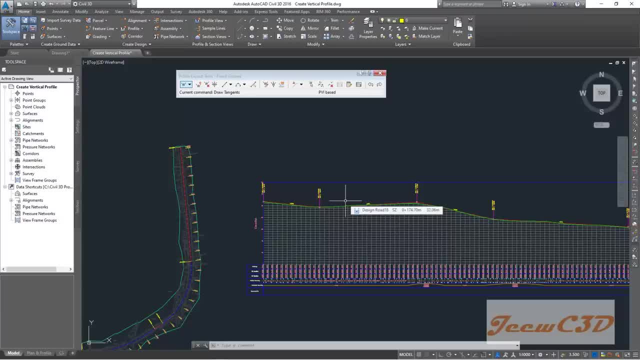 road and when you are having cutting sections, you have to ensure that you don't have forwards or flood issues when that profile is there, when you are lowering the profile, and also you have to put the flood values when you are designing the alignment if there is some flooding. 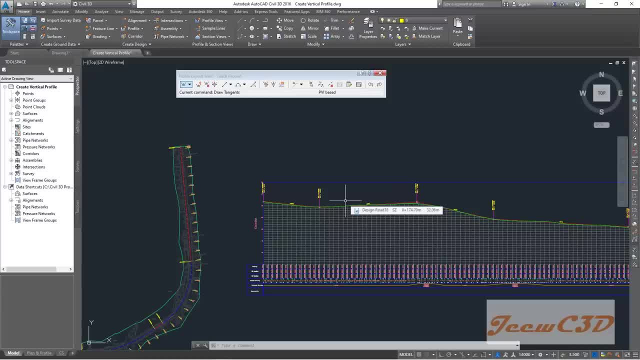 at some location you have to design your profile so that it is your road is going at a higher location than the flood. so those things you have to consider when you are designing the profile. what we have done here is just having the profile to give you an idea how to create the profile. 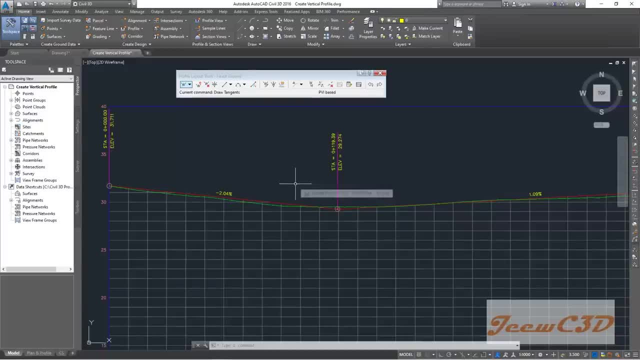 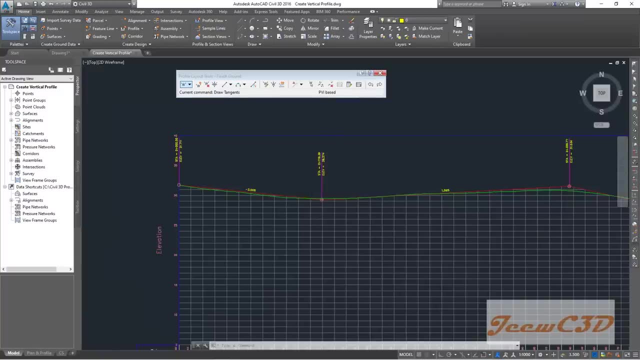 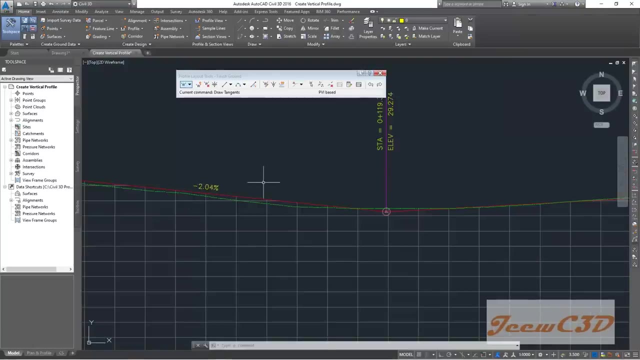 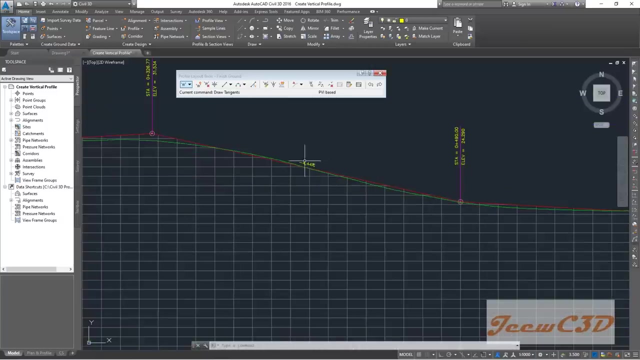 so creating tangents, how we are going to create the alignment, create the curves. before that, we will look at the tangents how they looks like. you can see, this is for 2.0 percent gradient, 1.09 gradient, 4 plus gradient, because you can go up to five percent and one point, one, four, five point. 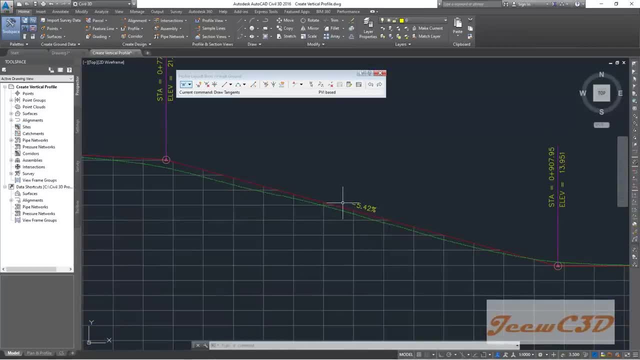 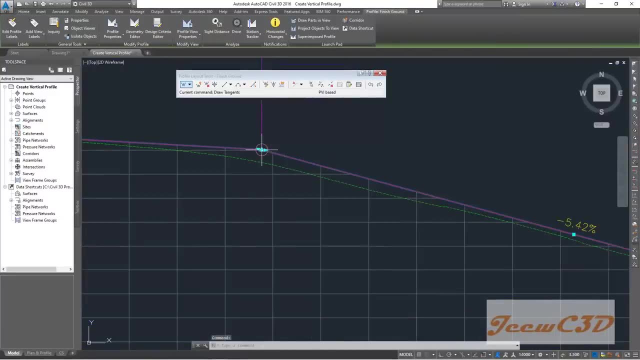 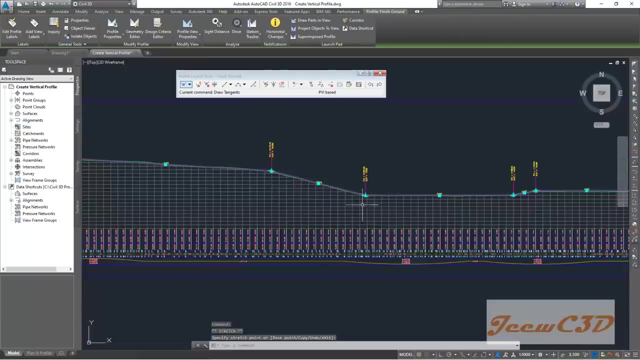 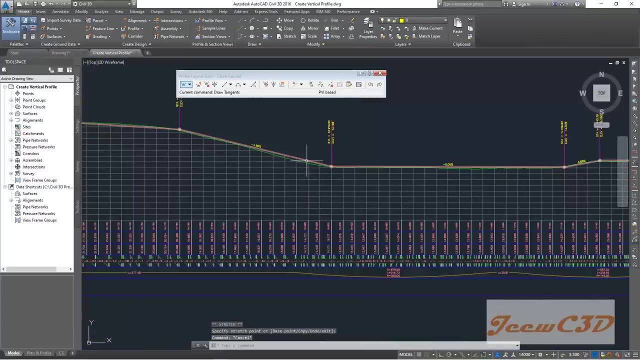 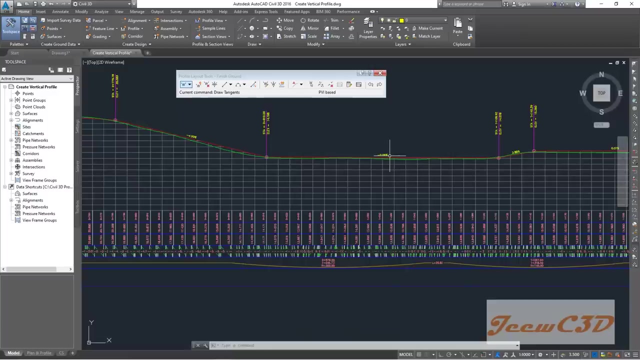 4,2. you can't use this value. I have to change this value so I can lower this one and raise this side so that I get something less than 5,. now there is a problem here. this specific gradient is 0.06,. you can't use that gradient because you should have minus 0.3% gradient. 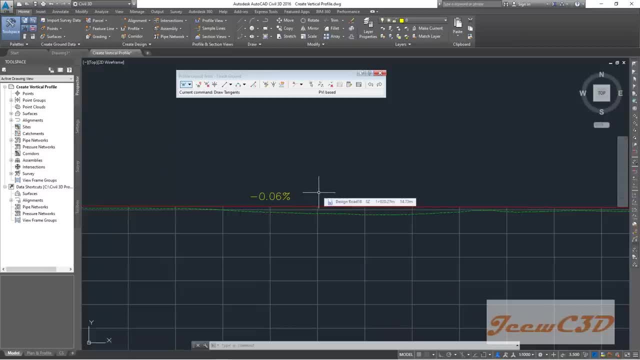 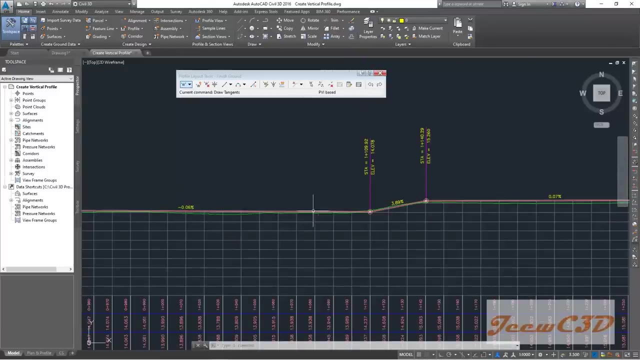 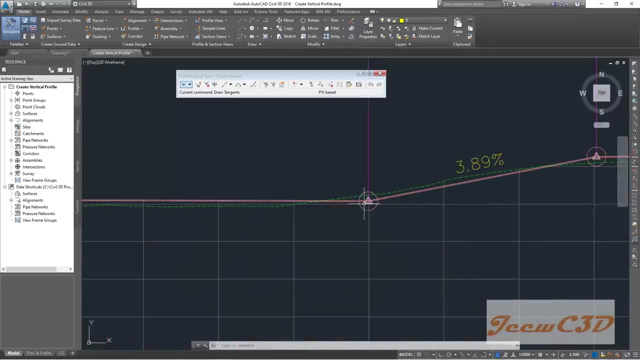 atleast. why not minus actually 0.3% gradient atleast to satisfy the next purposes? so what we do here is I have to increase this gradient instead, what I will do is I will delete this PVI point, point of vertical intersection, so that this: 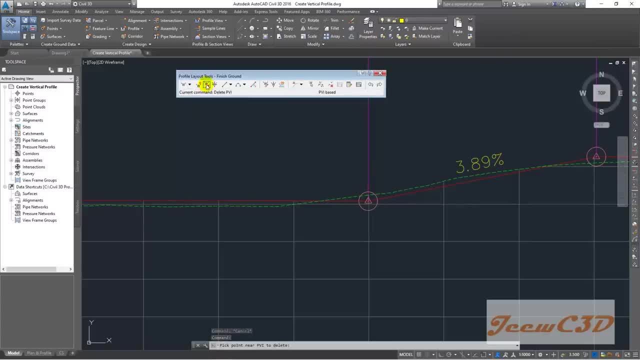 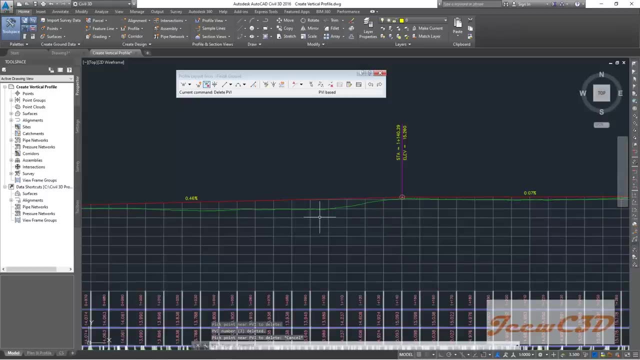 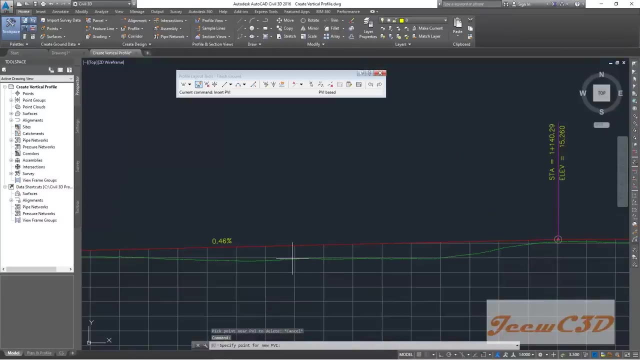 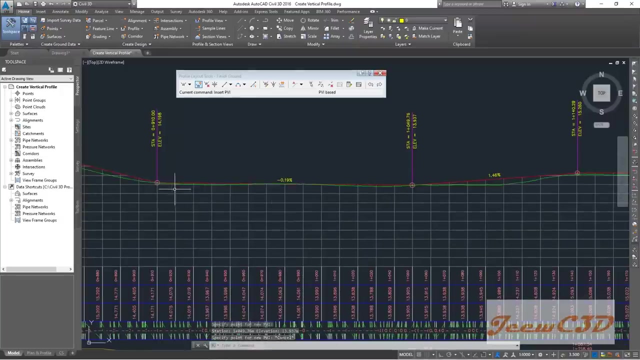 gradient increases From here I click delete PVI, then I click here. so it had some problems. it had created some problems for us. so I have a PVI again somewhere here. let us say, I apply a PVI somewhere here. still I have the problem. so I can. 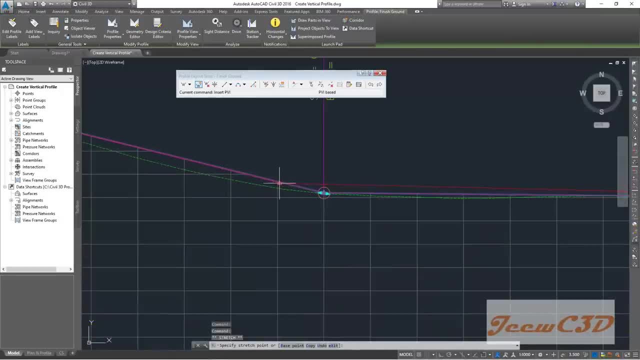 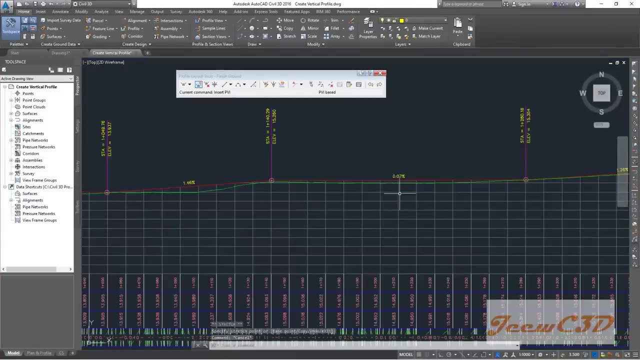 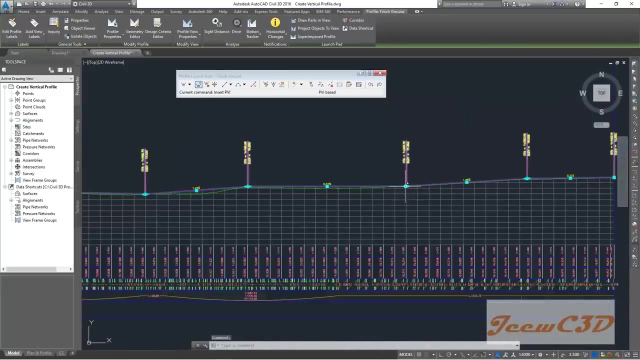 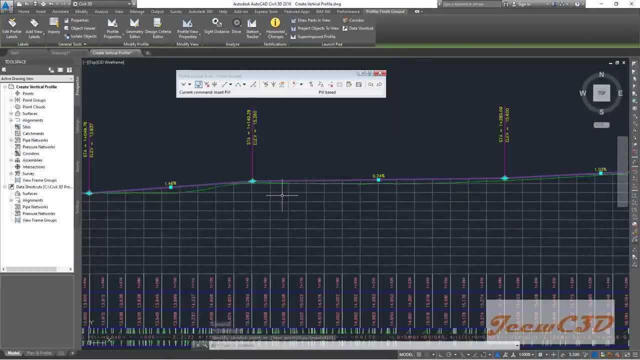 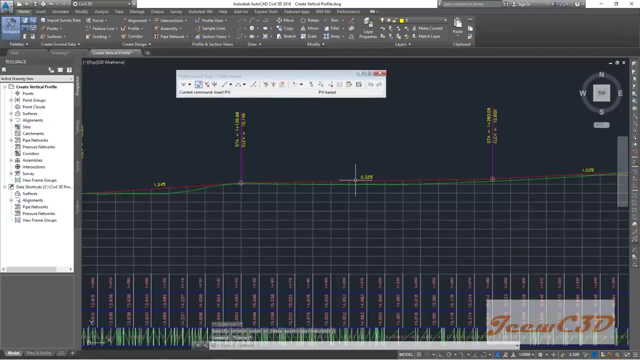 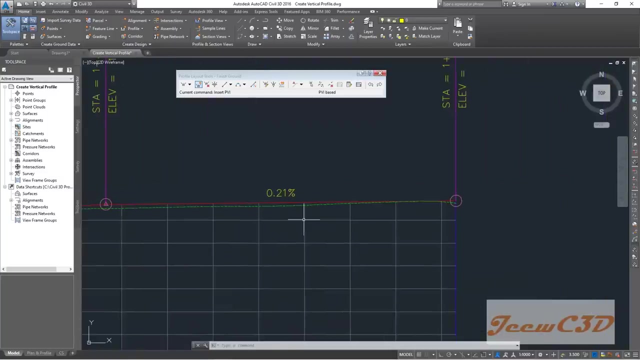 raise this one a bit, then it looks like okay. again we have a problem here. so I will raise this profile and see what happens and I can go over somewhere here and just doing some modifications. I have to redo these modifications later also, and again I have this 0.21 percentage, so I 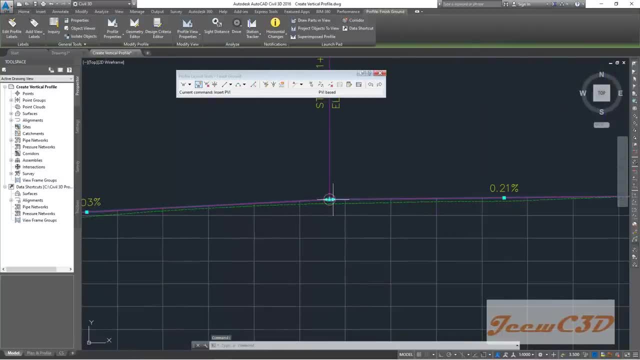 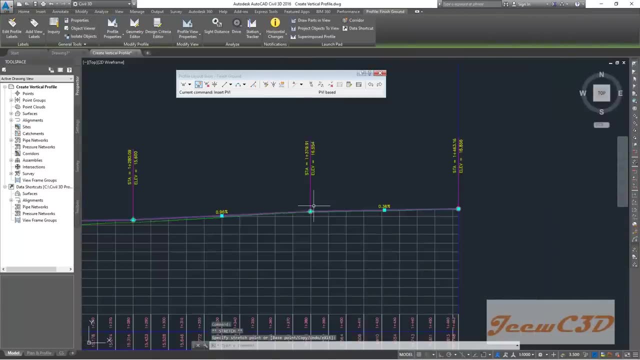 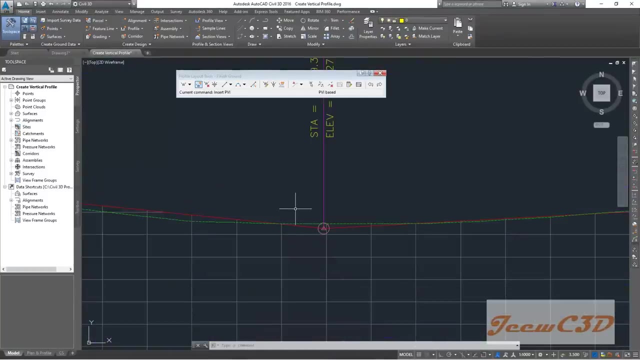 will change. this side seems right, ok right now. let us see the next one. seems like ok for the moment. so now I am going to apply the create the vertical curves. so your minimum curve length should be 50 meters to satisfy the appearance criteria. so once, 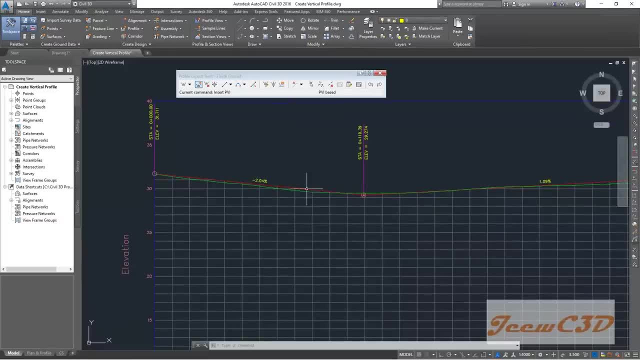 I place the curves- vertical curves here- between two tangents. I will use the curve length option and I will use something like 50 or 60 as my curve length. so to do that I am going here: profile layout tool. this option then free, more free vertical curves. free vertical parabola. 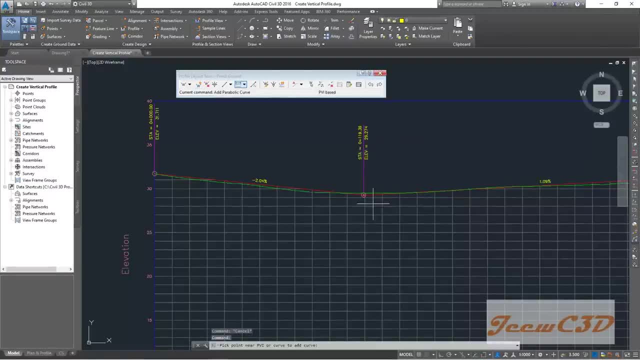 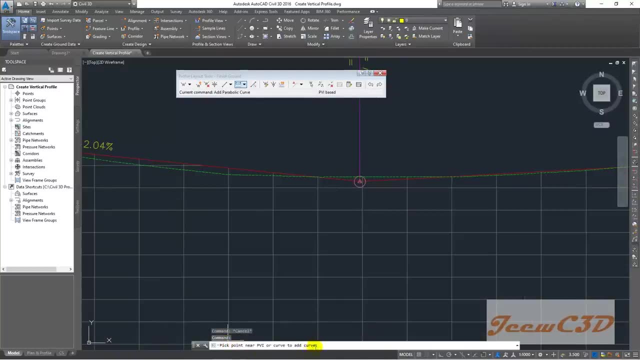 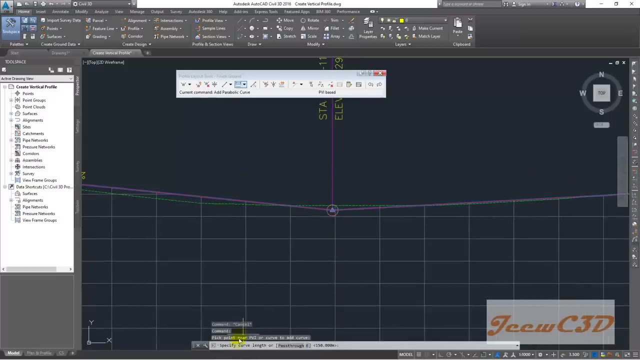 pvi based. I click that one. then I click here. it is asking: pick point near pvi to add curve, where I am want to add a curve here. so i click this pvi. it is asking: specify the curve length. let us say, since my minimum curve length is 50, i will type in: instead of 50 i will type 60. 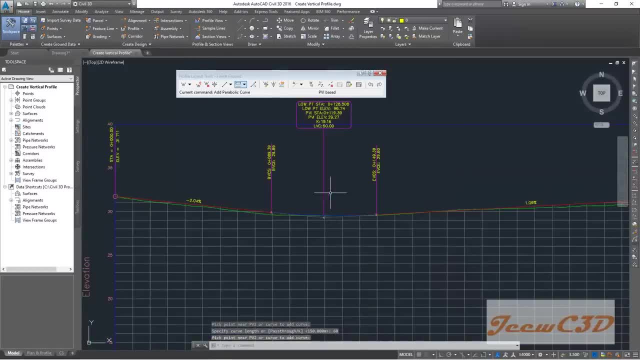 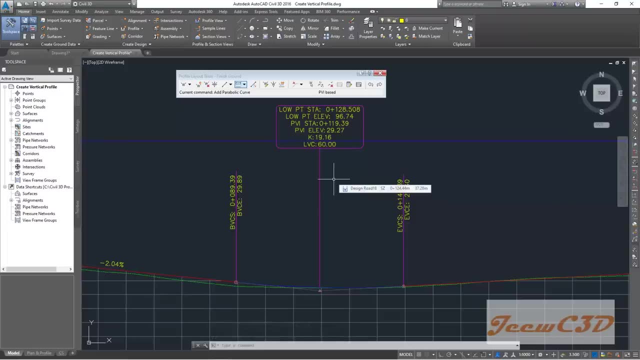 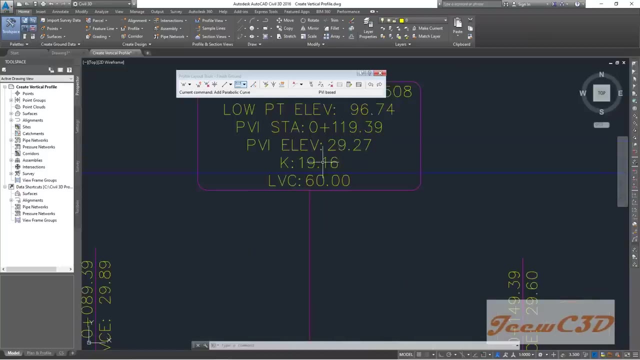 then press enter and i will see the value. so at least i should have 17 to satisfy k k value for stopping side distance criteria. in this table it gives my k value as 19.16. so that means my k value is okay. so this curve is okay then i am going to this point. 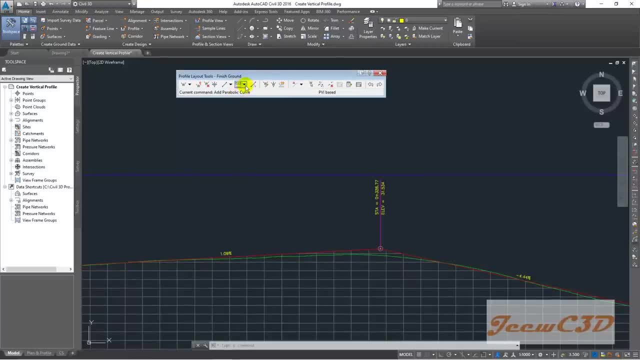 so, since our last option is this one, you don't have to go to here and click this one. instead, you can just click this one. it will activate the last option, what we did. so i am picking this point again. i am giving my curve length at 60. 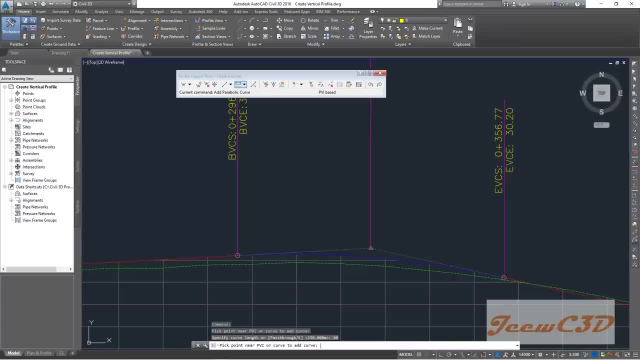 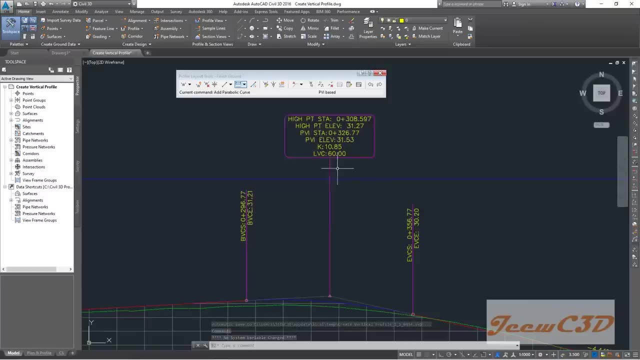 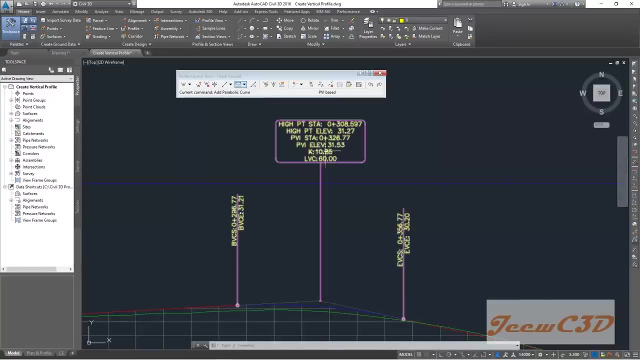 and i press enter and see whether that satisfy the criteria. oh, that is a problem because it will not satisfy the site distance criteria. i have to have at least seven. So what I do is I click here, pick subentity, edit, select pvi option. then this kind of 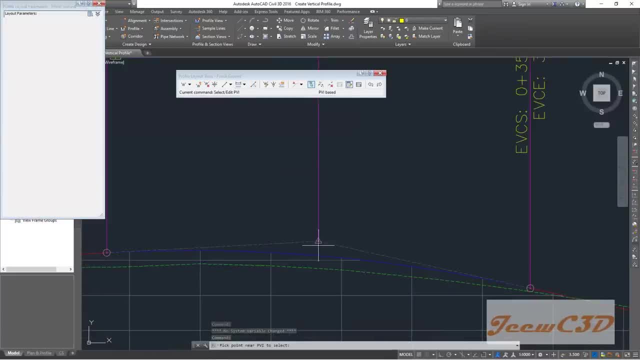 a window will be appearing. I select this pvi's. I click somewhere here. it is asking to point me a pvi to select. I select this one. so what will I do? I do increase the curve length. let us say I increase into 70, so my k value is 12, now finish. let us say: 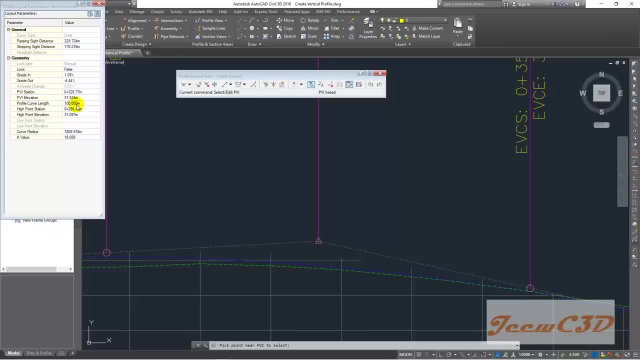 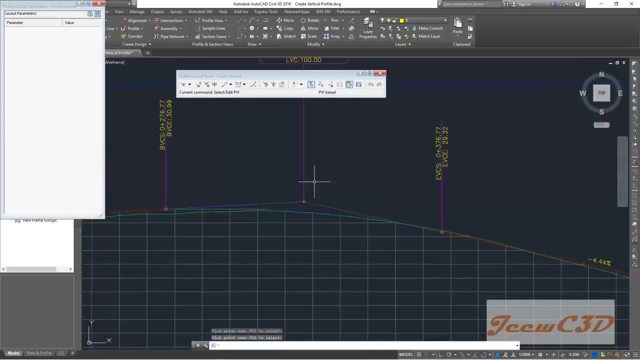 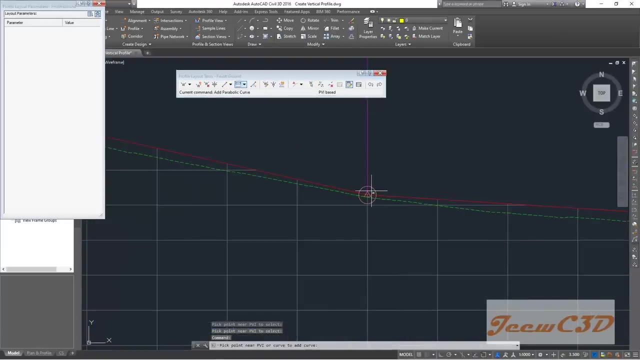 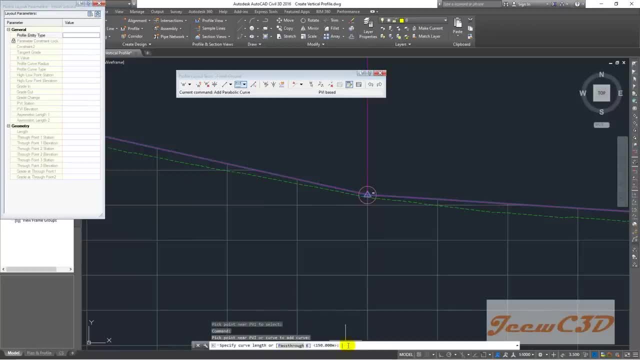 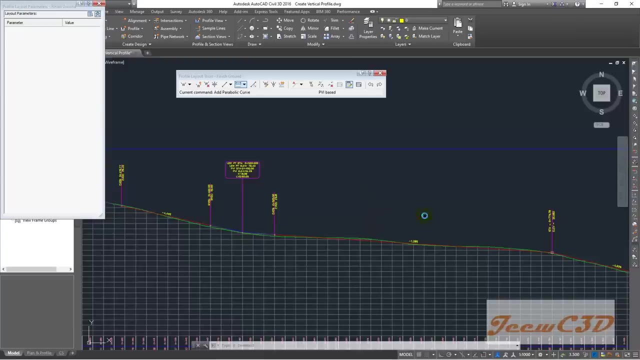 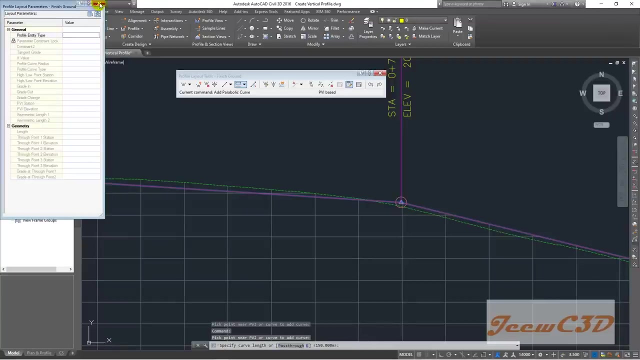 so I type my curve length as 60, as usual, then press enter. it is ok, because this k value is greater than 80,. again, I come to here and press here and my. so if it is, if this one is bothering you, you can close this one. then I type here: curve length: 60,. 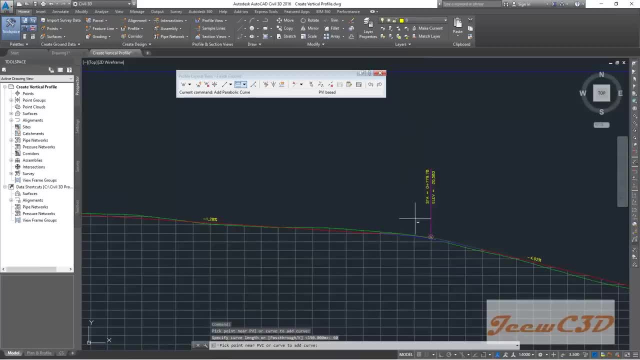 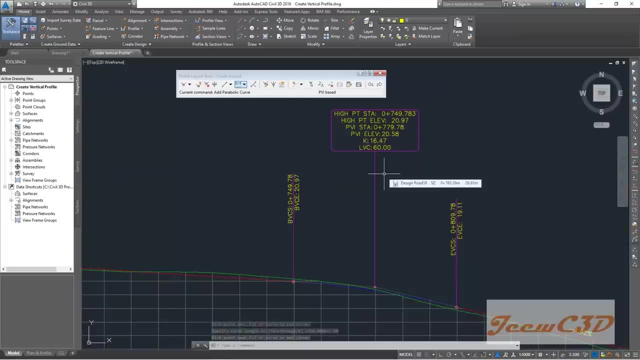 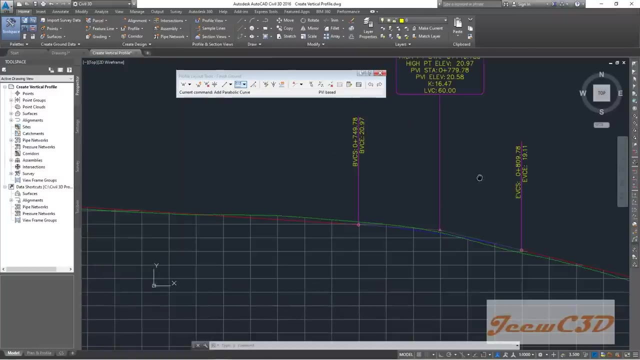 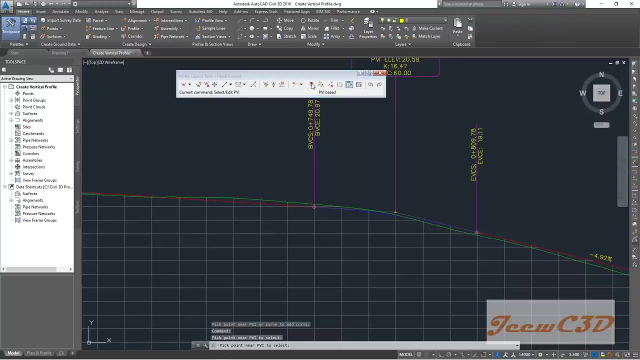 as 60. So when I press enter this one, I need a small modification, because this K value is just less than 17. So I have to increase a little amount of prevalence. So I click here to select PVI, but I don't get that window here, So in: 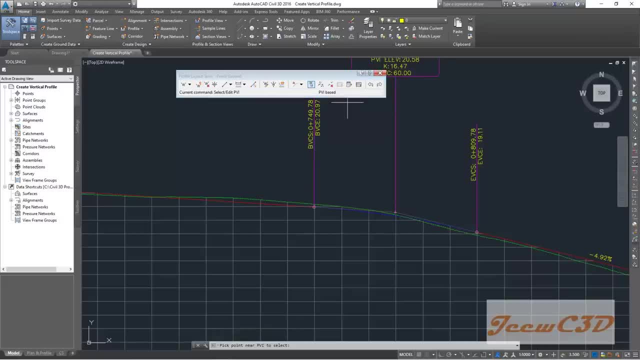 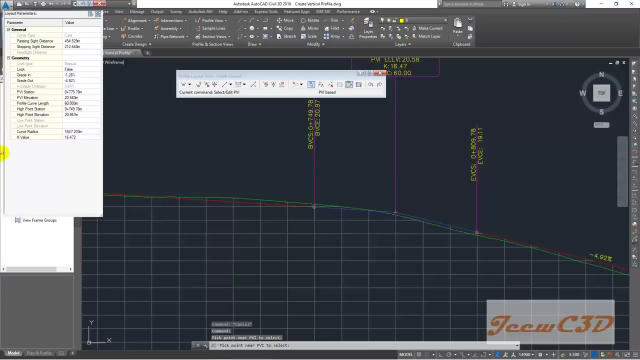 that case you have to click it here one and again, So you have to click two times. Then you select this PVI button and here select. here You will be getting this small window. Type the value as 70.. The same that your K value is now satisfied, I am. 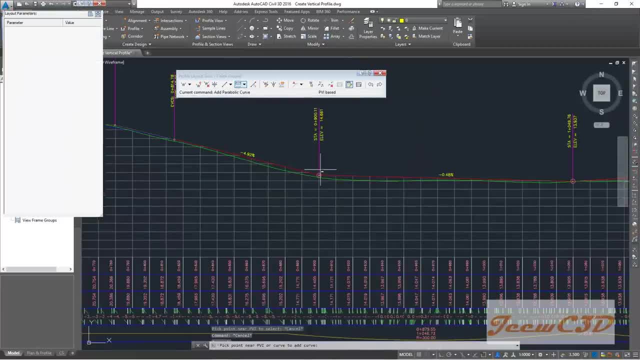 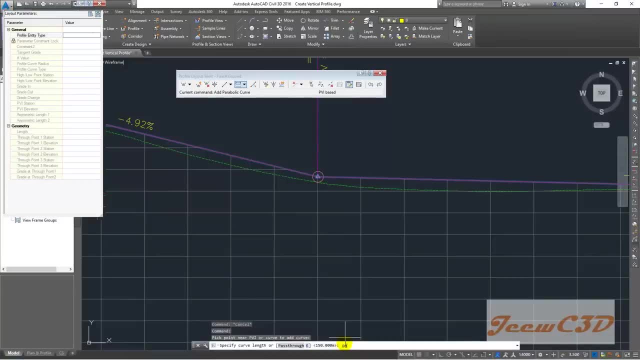 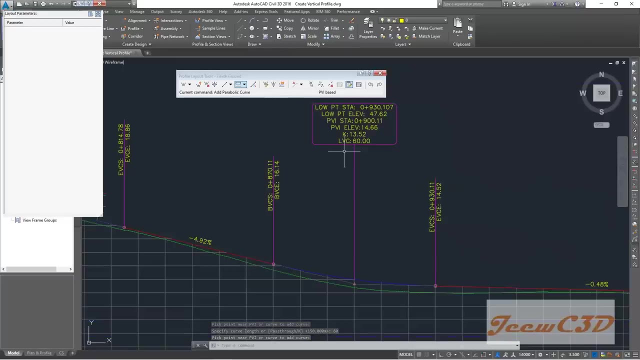 coming this point, the curve will be here. my curve will be 60,. press enter. we will see: still it is not satisfied. I have to increase the variance. I increase my variance up to 70 and see, still it is not ok. now, instead of increasing the curve length, you can decrease the variance. 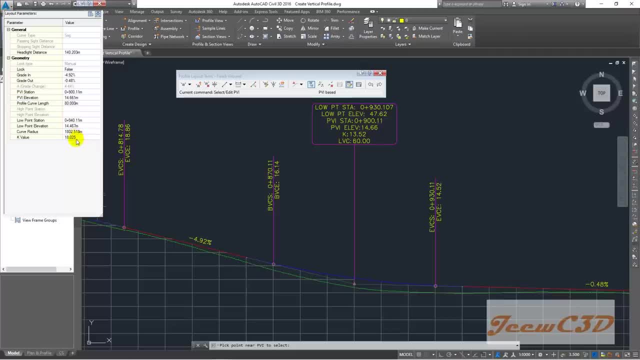 and see what happens. also because if you decrease or increase the variance, these values will be changed. for example, let us say this grayed out, we can change it to minus 0.5, so you will see the p-value changes. so instead of increasing the value, you can. 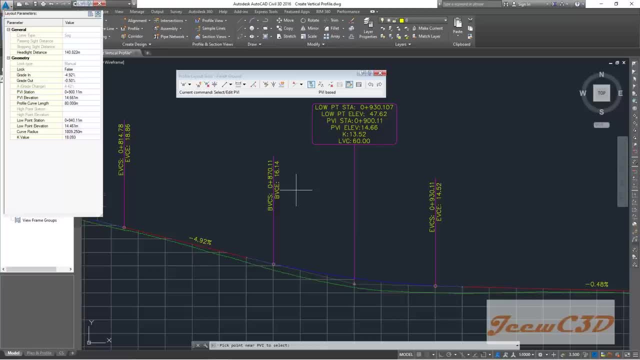 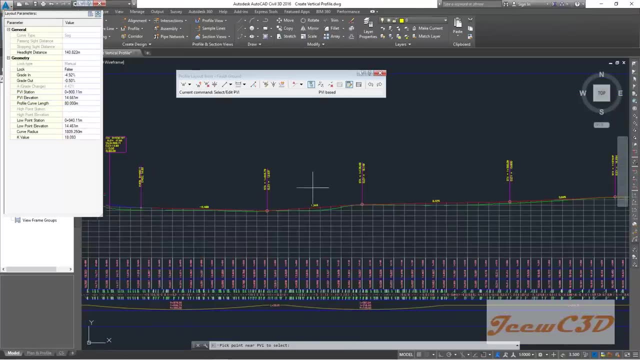 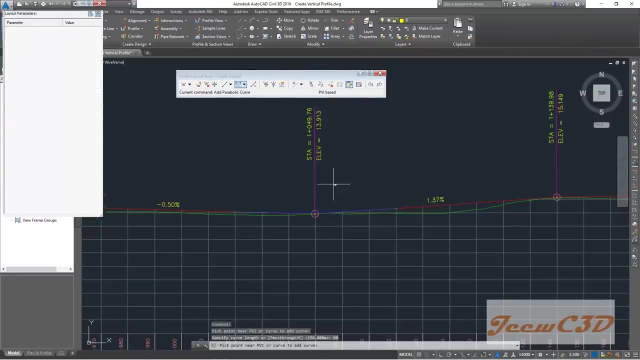 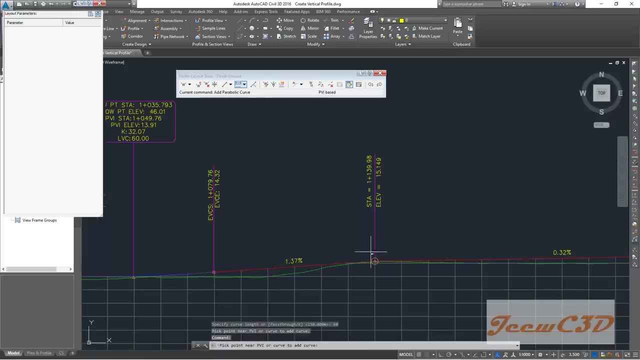 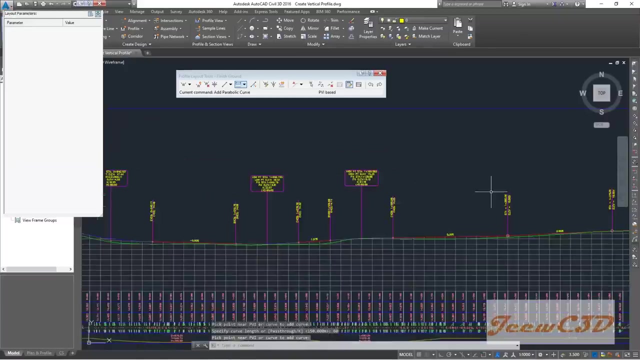 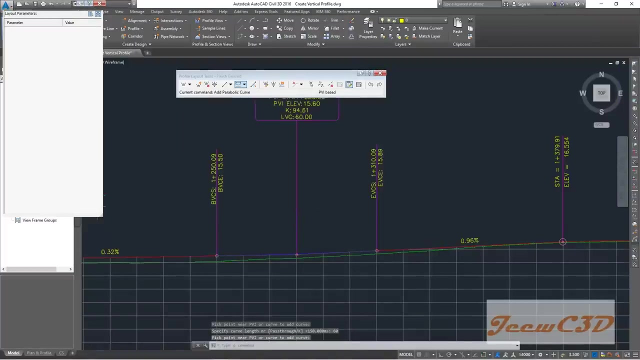 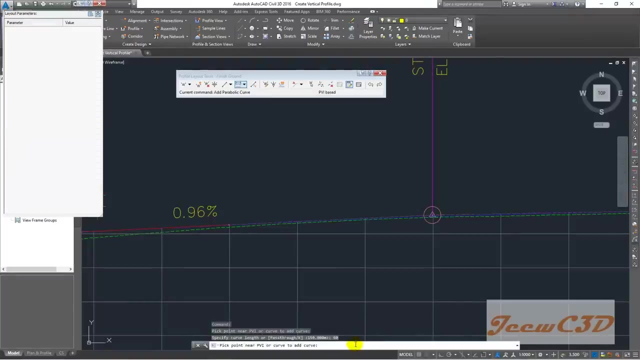 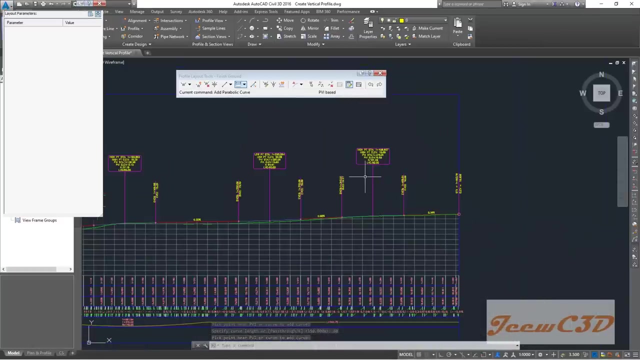 change it to minus 0.5, so instead of always changing the curve length, you can change the variance also. so we have few curves left. I will click, go through them seems ok, and here again ok. everything is more than 17,, which is the critical k-value for this design. 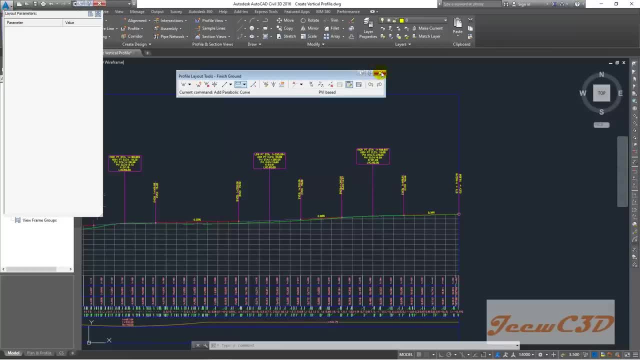 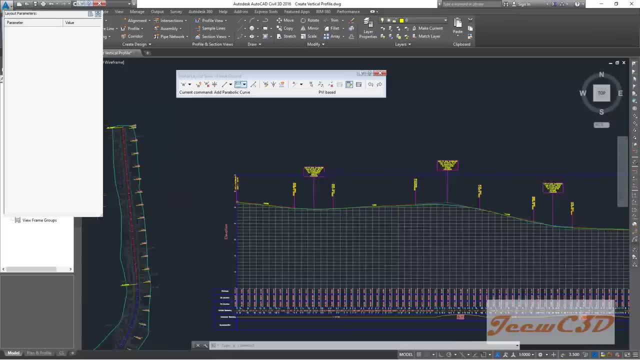 the first one we will change again. now I am in the front of the table. this is the 1.2, so you can see that. that about 3%. now when I am changing the value, it becomes. 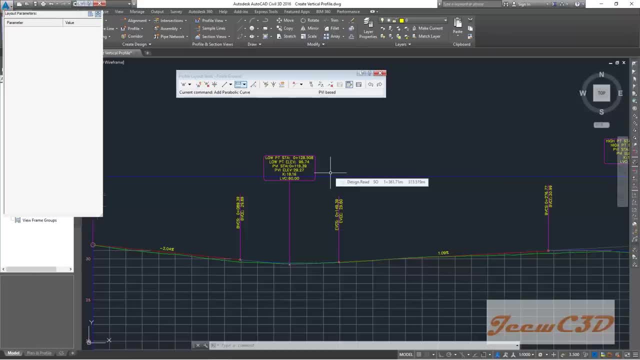 0.5,. now that increases to 0.5,. now let me add another value to it, which is 0.5, and after that we change it to 0.26,. ok, so the effect is done. so far, we have created the. 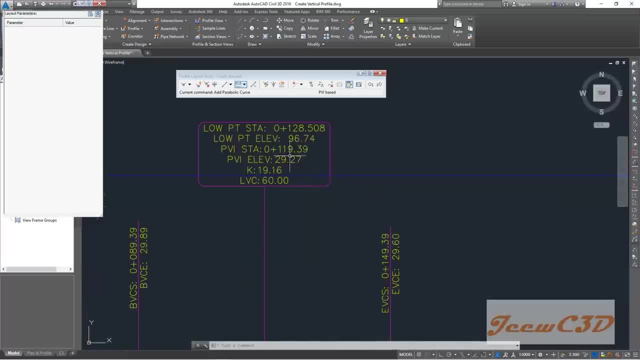 profile of the code. now we have checked everything, but you can do one more thing if you like. you can round off the ratios. instead of having this 918.39,, you can change it to 120, like that. so the find these 4 contacts and see it used to work on the. 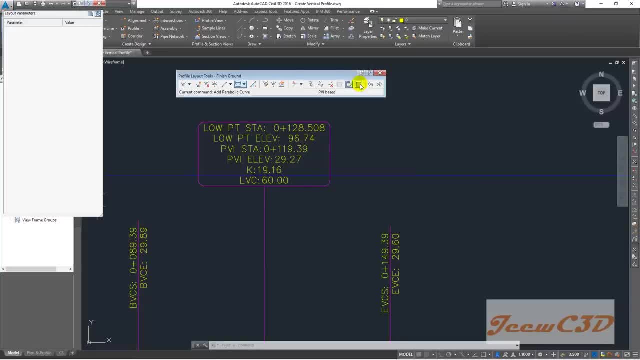 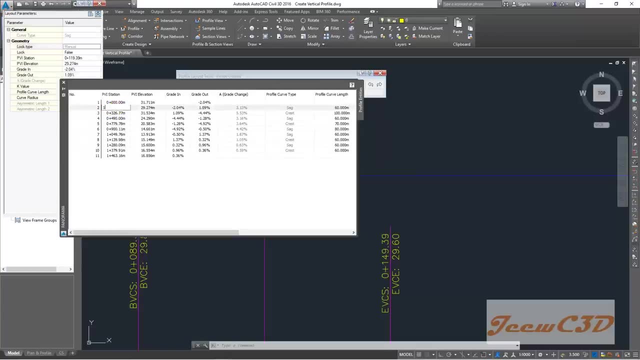 the easiest way to do is you have to click here papaya, good view. so you type the teenagers here 120 instead of this 26. we will type 330, here 490. let's just type it again: this one is 780. this one is 900. 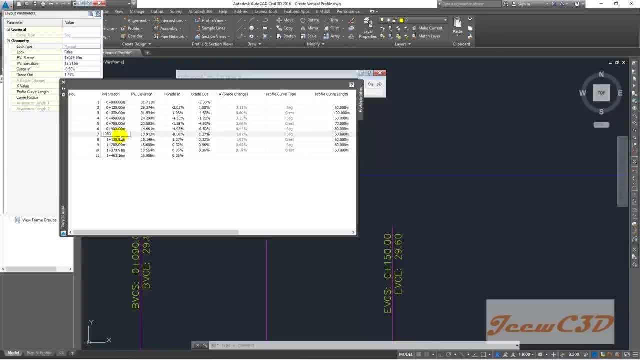 this is 1050, this is 1140, this is 1280, this is 1380 and final one: you can't change because that is the end of the alignment. so this is this and you can't change it. you have to be exact with that. so you can't change this one in the middle. you can change these. 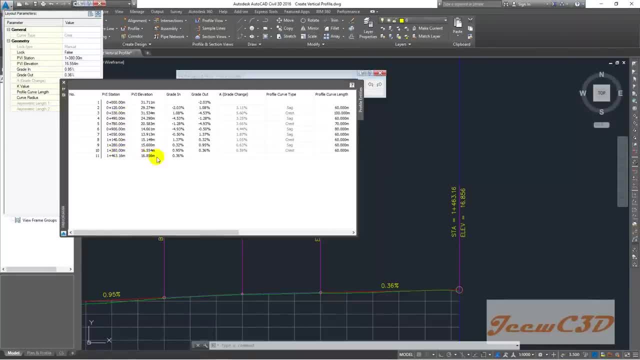 values. once you have changed the values, you have to check the gradients- they will be appearing here- whether they are less than 0.3, and also the k values. once you are changing the station, sometimes this k values may be just shifted to a value less than 17 in this case. so you have to check the. 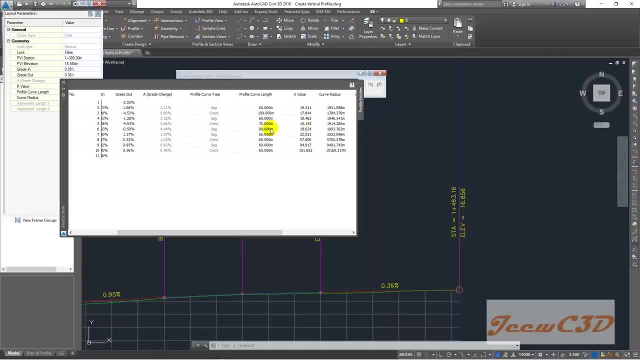 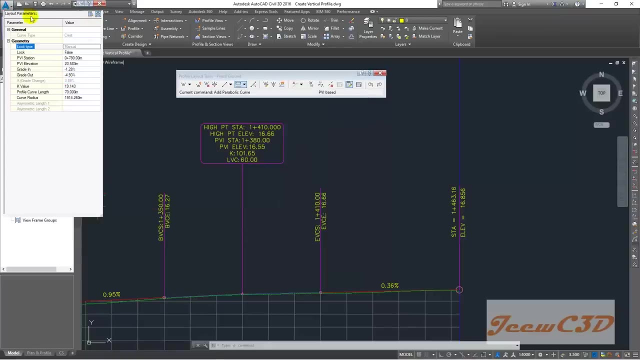 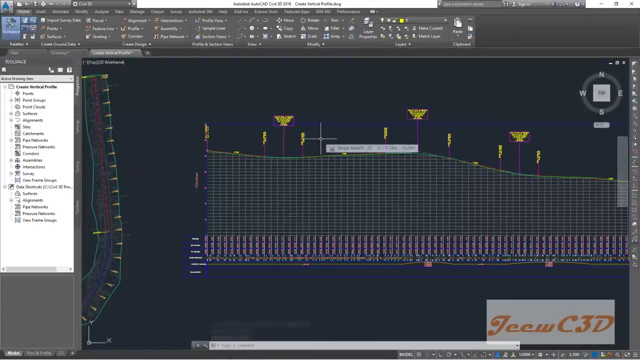 values here. also, if there is a change, you can increase the turbulence from here and check whether the value satisfy this criteria. so i will close that one and i will close this one as well. this i will request it from here. so that is how to create vertical alignment. 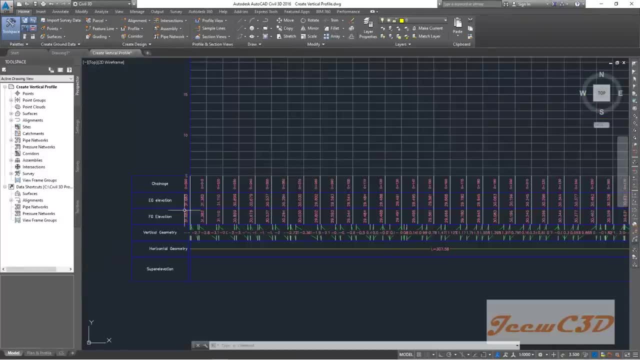 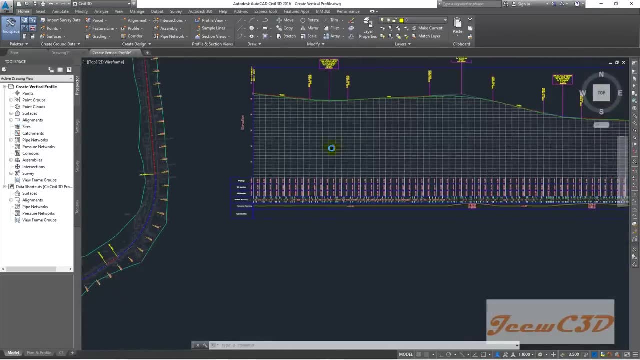 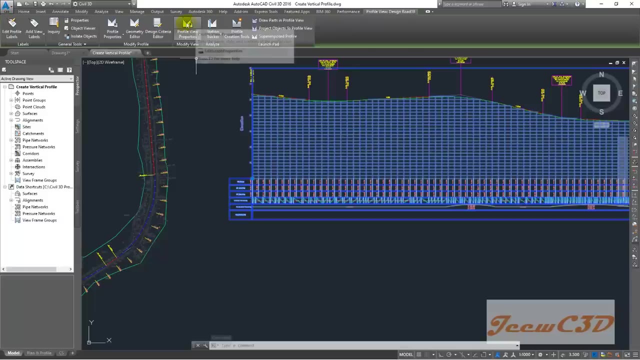 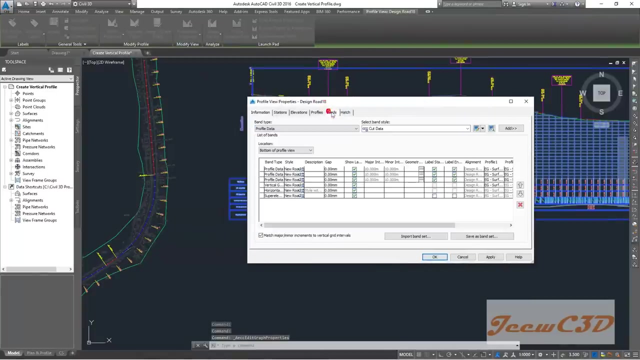 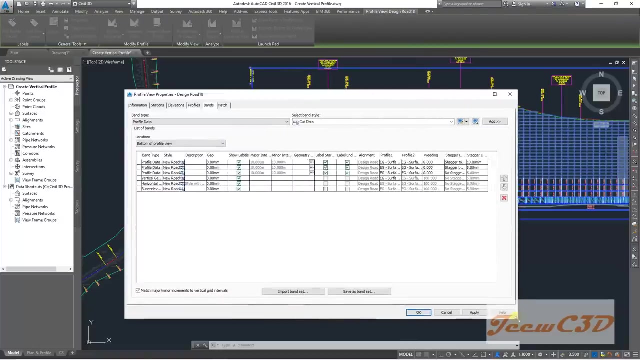 and also i will tell you how to modify this band now, because we have a vertical profile here. to change this band data. i click this profile view, then i go to profile properties from here, then i am going to bands tab and if you can't see this profile, you can expand it here. 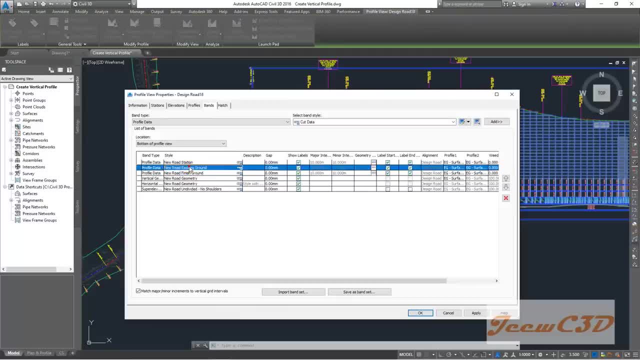 so you can see. for existing ground you will get eg surface. it is okay because existing ground data is getting from eg and new road finish done. you have to take it from your finish ground here. you created chest moments earlier. you have to set two options here so i put a profile one and another way. so you have to saw your existing data now. here you will create at least moments actually moving. so that you pay attention to 23. Jayah. so i hope you guys did not off, like and comment on the video until the end. see you later 2016. see you later. say bye, bye I entonces. um, and thank you guys. oh, and thank. 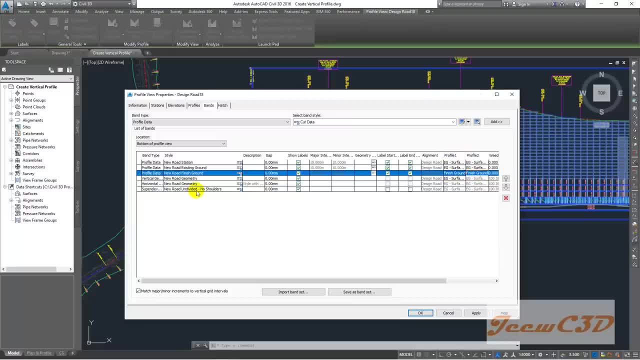 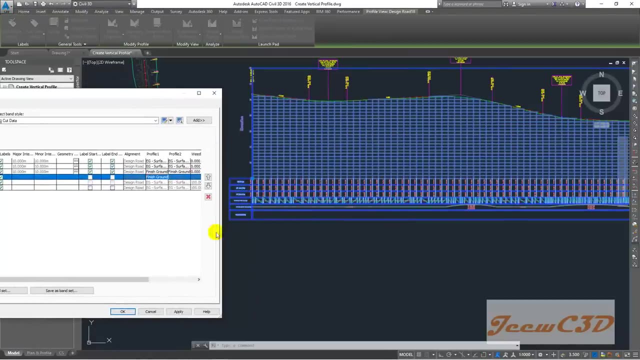 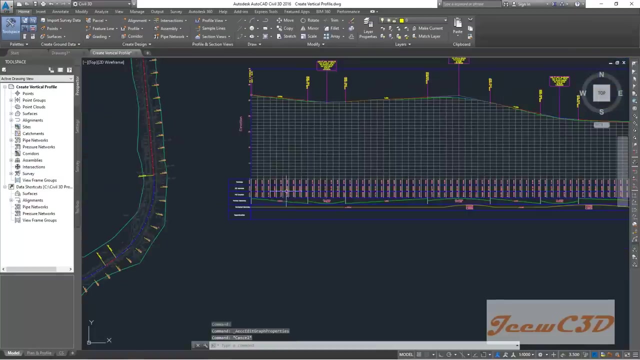 you profile to finish down and vertical geometry also. so vertical geometry- here we have to set it to finish down. so these changes will be applied to this finish down and this vertical geometry location. so we see these are changing while i click. ok, we see here. now what happens here is: 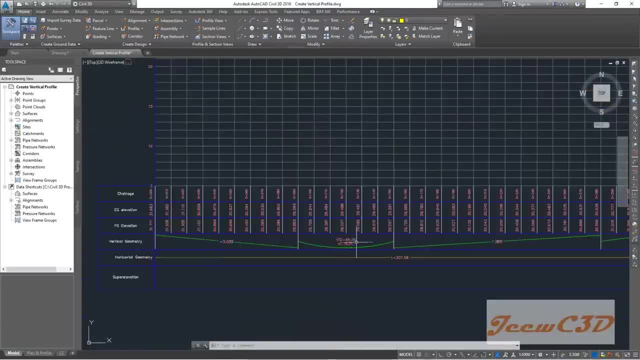 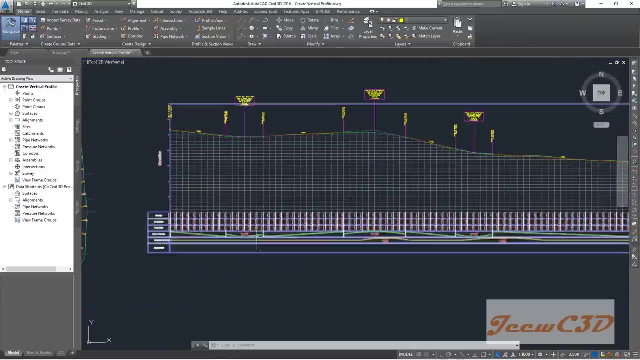 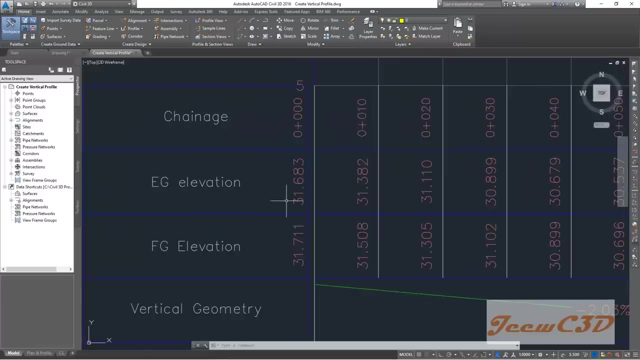 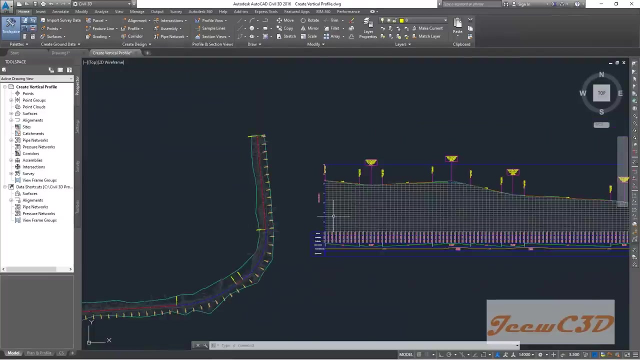 this profile is drawn here like a summary. you can see the gradient and k value and turbulence. so we have less data than here, but still you can get a good idea. then you can see. now the eg elevation and fg elevation have changed because we have changed profiles for eg elevations. it will take 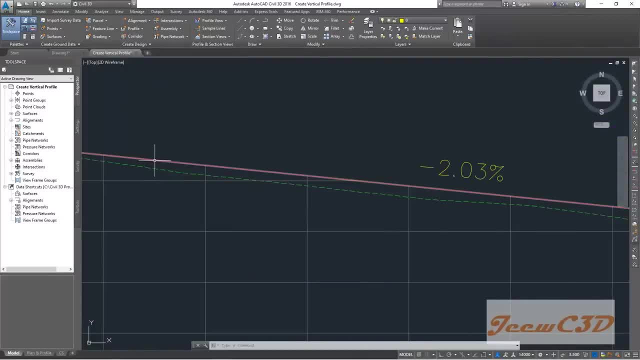 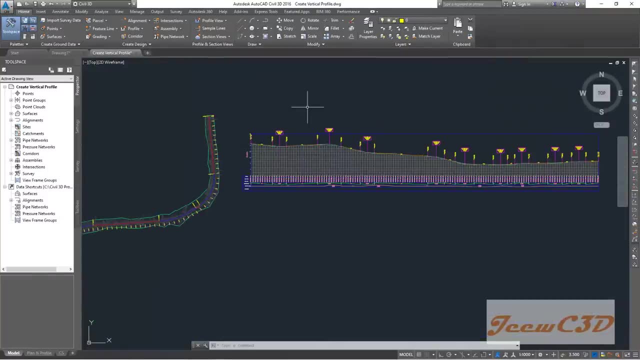 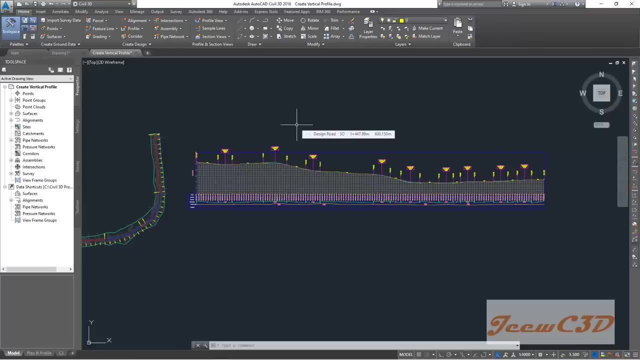 elevations from this one for fg elevation. it will change stations from this one which is the profile we created for fg. so so far we have created alignment for horizontal alignment and we have created a vertical alignment and we have set up the vertical profile view there to get the clear view of the 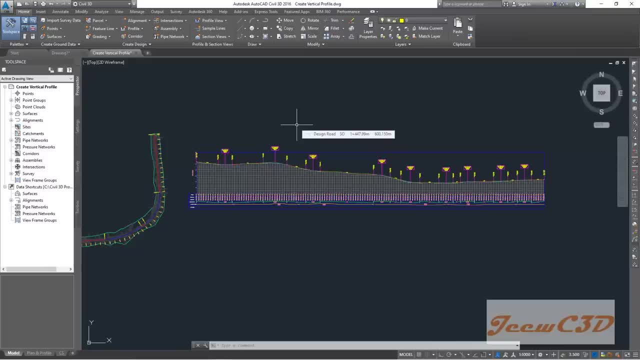 data in the alignment as well as the profile. in the next video we will be looking at how to apply super elevation to this alignment and then we will create the corridor and the first sections in the coming videos. so before that, i will save this drawing and close this drawing. save it and 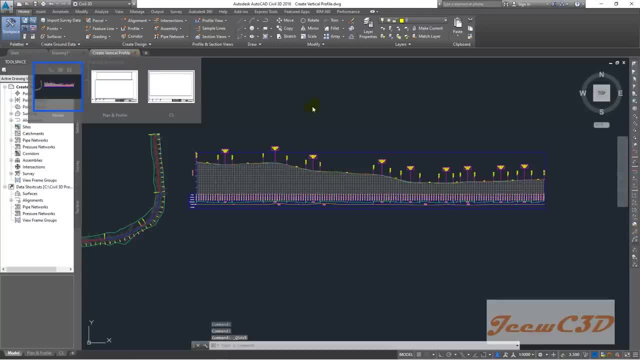 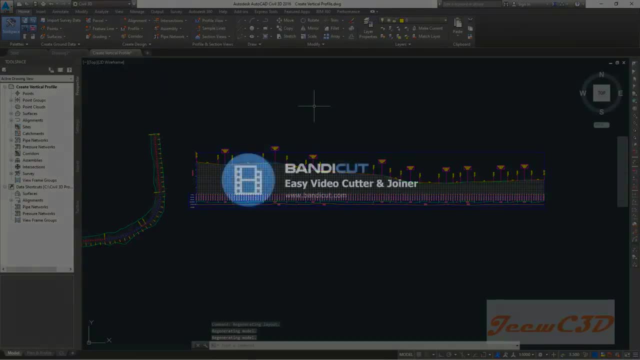 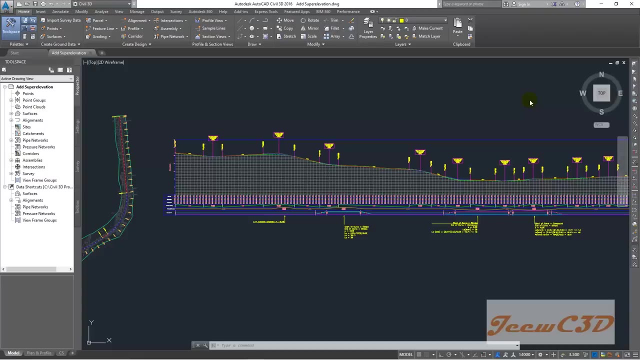 close it, so i have resource. in the previous video we learned how to import super energisation and create the super elevation diagram, so in this video what we are going to do is creating the assemblies or super elevation or otherwise, the typical sections for your robot design. so i hope you have saved this drawing by. 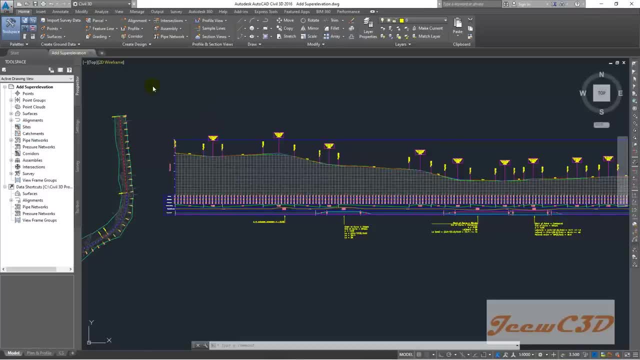 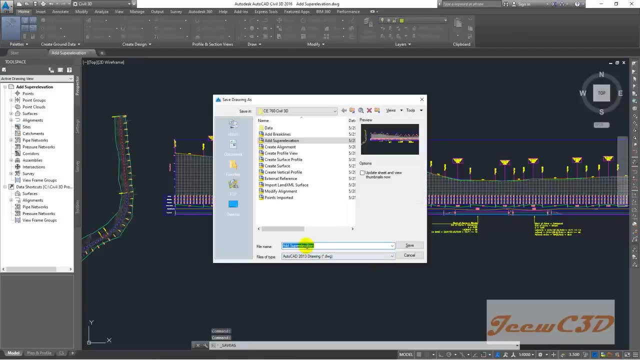 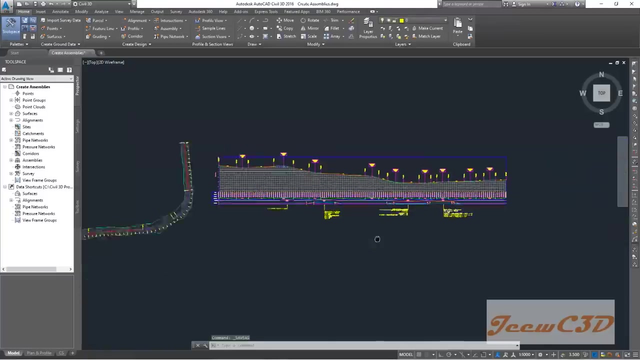 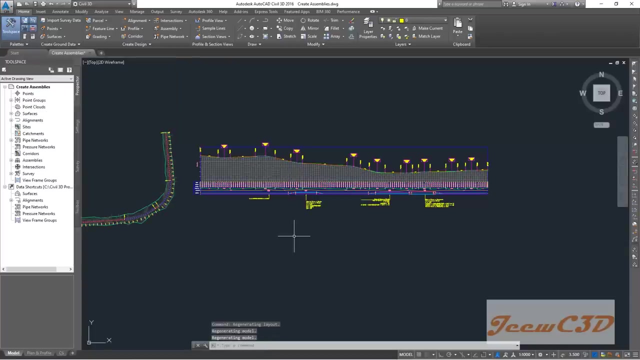 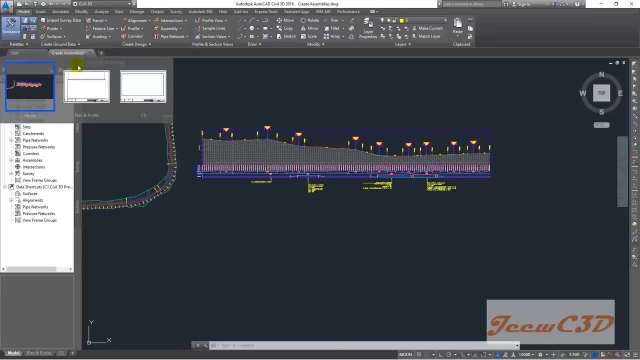 now. so i will rename this, rename this drawing by save as the drawing as p8 assemblies- create assemblies and then click save. now i have a new file which we hold with the name of create assemblies. so if something, if you move the cursor here, something additional, something you may be, 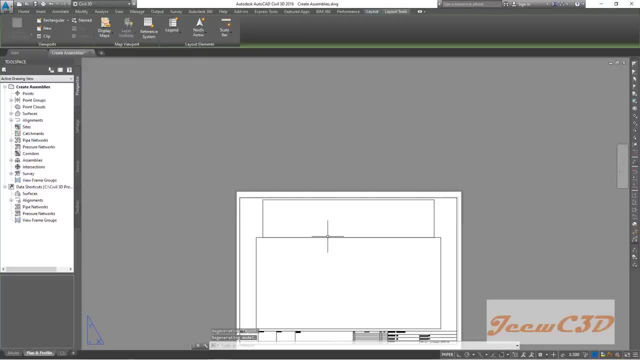 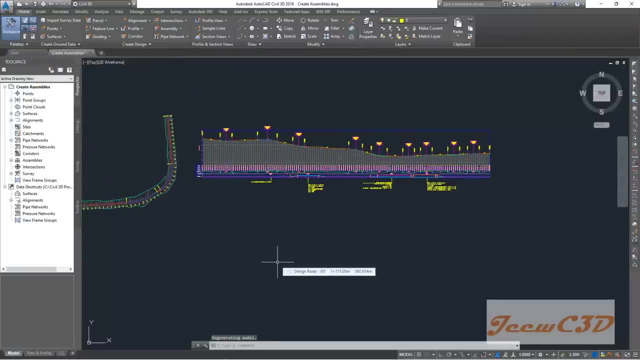 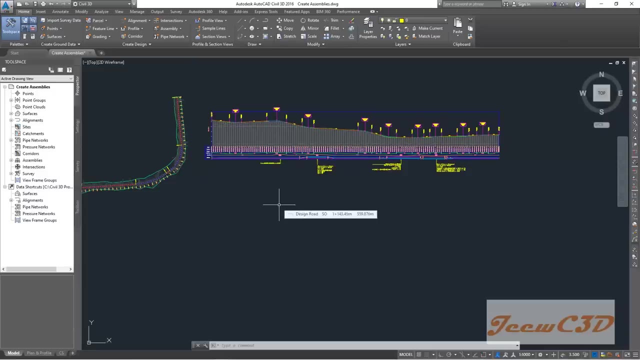 shifted to another, so you can click here again and go to module one, so you will be getting back to the normal view. so that is something additional. so before create the assemblies of the typical cross sections, i have to tell you what kind of regions we are creating in this word project. so 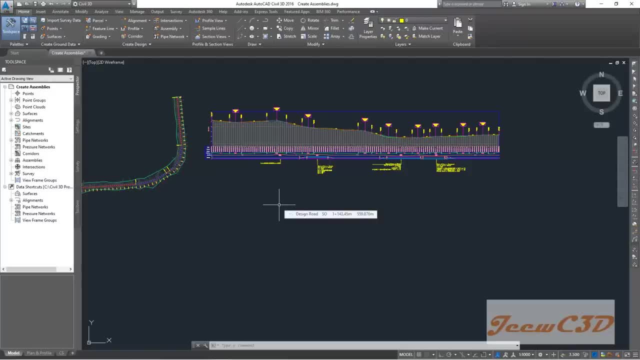 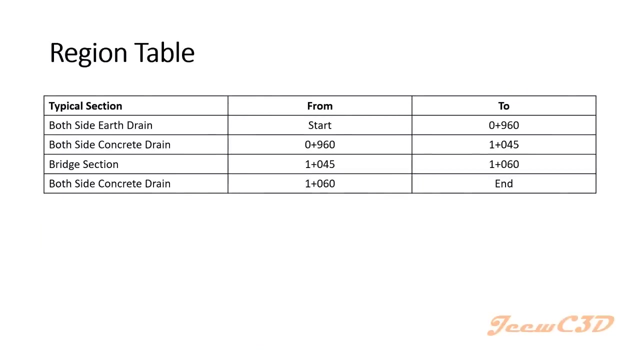 let us say we have identified several regions in this road project and how they are going to be created. so now i will show you what are the regions we are going to create inside this road project. so this is our region table, so the road project. so you have the robot with earth drains from start to. 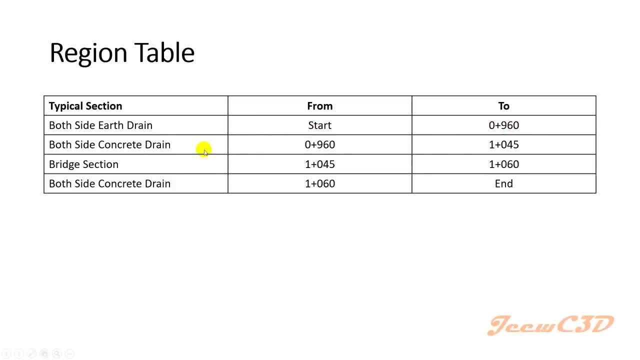 station 960.. Then from 960 to 1045, you have both side concrete drains. In 1045 to 1060, you have a bridge section And finally from 1062, you have again concrete drains to the road. 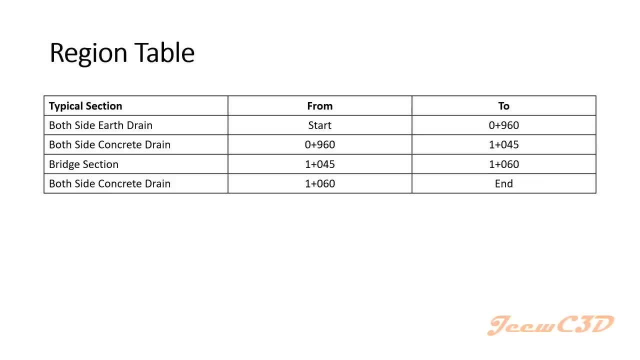 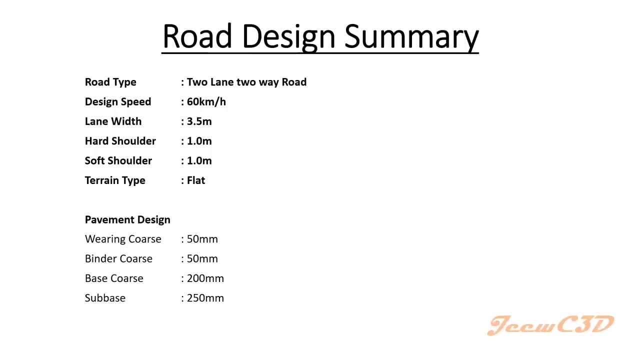 So we have to create the three typical cross sections for this project. That means both side drain, both side concrete drain and the bridge section. You have to create three typical sections. At the start of the design summary I told you in your payment design: 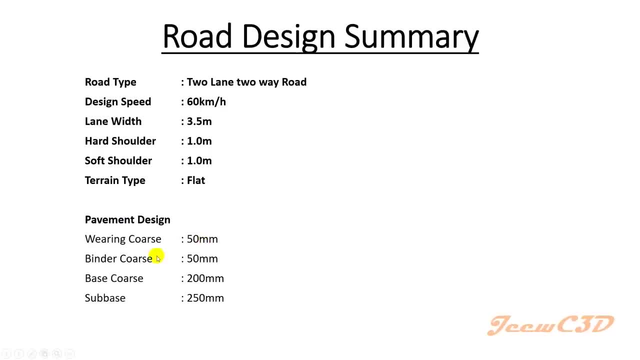 you will be having these: Pairing cost 50, binder cost 50, base cost 200 and surface cost 200 and 50.. For the bridge section, we will assume we only have pairing cost 50 and binder cost 50 millimeters. 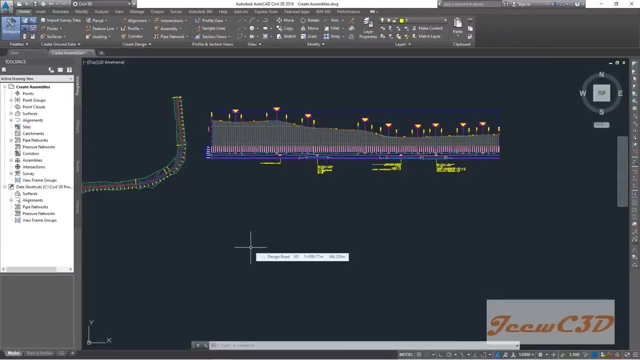 Now I am going to create an assembly, or otherwise. we call it the typical section For the road. if you are familiar with road projects, you will know what are typical cross sections. So what we are going to do is we create a typical cross section for this road project. 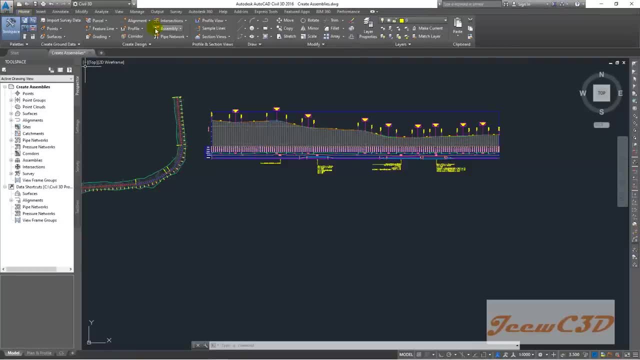 To do that you go to home tab, then go to assembly. here click the drop down, go to create assembly And type assembly The name here. both side drain same. you don't change anything if you can type some descriptions here instead- I am not typing here, I will click okay. then it is asking: specify assembly baseline location. it is asking for a location. 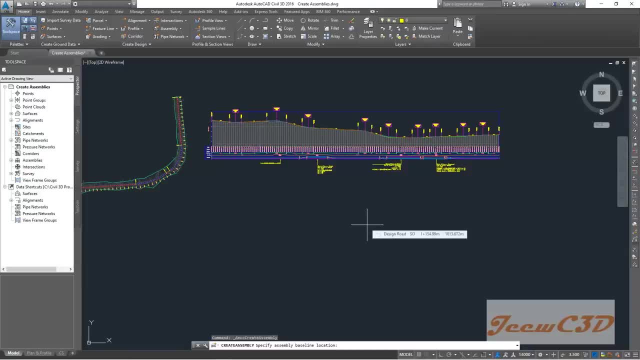 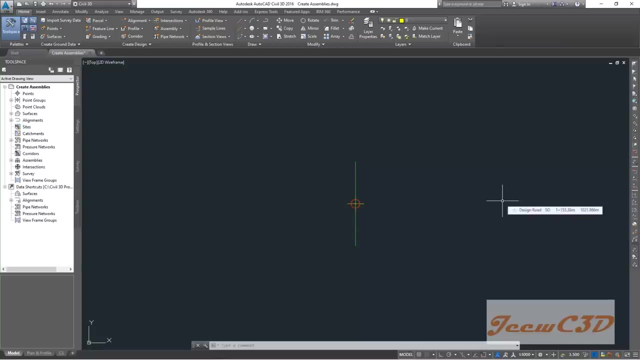 To paste assembly. you click somewhere here you will see this kind of a green vertical mark may be appearing on your screen once the assembly is created, But still it is only a vertical line, So to be a cross section you have to add parts to either side of this. So you can remember, you have a lane width of 3.5, 3.5 lane width, 1 meter half shoulder, 1 meter half shoulder and other drains and cut and pick sections. So I am going to add a lane to this assembly. 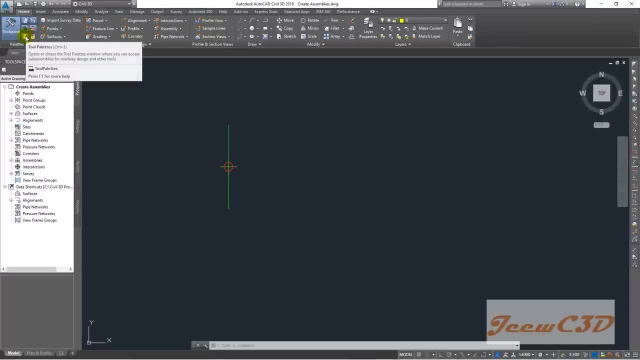 To do that you have to go here to poly tool palettes. Then can make this larger if you need. So if you are not getting this thing first, I have to go to this lanes tab here, then I click this lanes super elevation AUR. 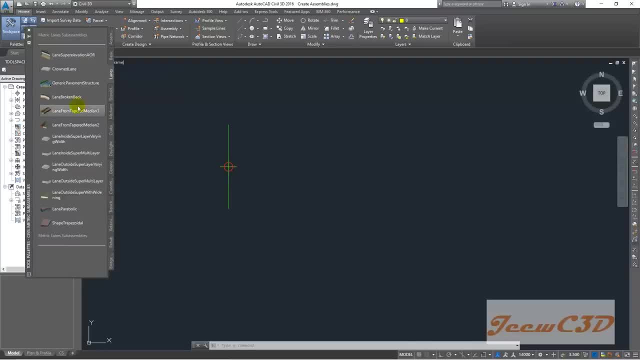 But if you are not seeing any of these in your tool palette, what you have to do is you have to close the drawing and go to your desktop. instead of double clicking your CV3D matrix equation icon to open it, you right click the software matrix icon and run it as administrative. 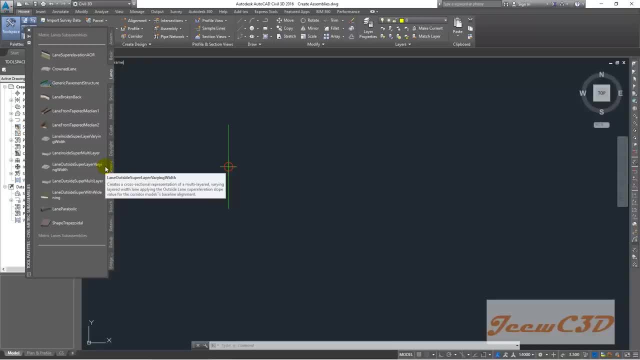 so after that you open the drawing from that administrative open software. that means you in the desktop. you right click the CV3D icon and run it as administrative. so that is how you make it appear if this one is not visible to you. so now i am on this lanes tab. i click Rhodes Super Elevation AOR. 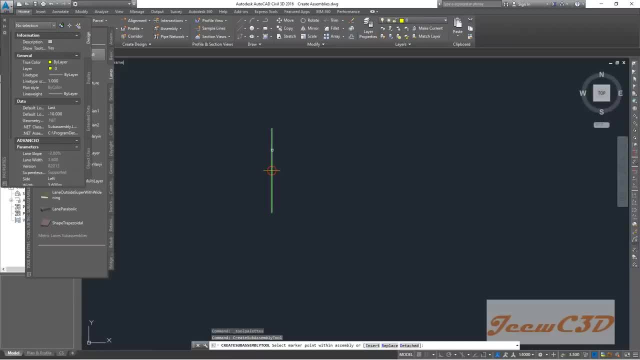 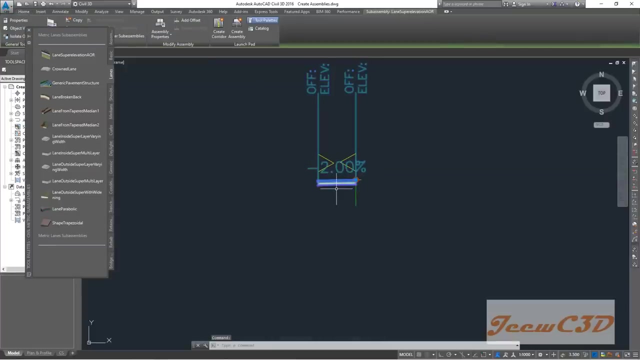 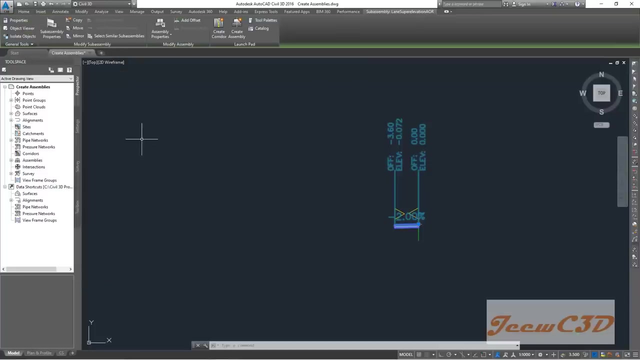 then i click new. click here, so it applied to my left side. so again i click here to select the sub assembly. we call it a sub assembly. i will close this for moment. so my lane is attached, but i don't know what are the data inside this. to view this data, i select this one so i escape. to deselect it. then i select. 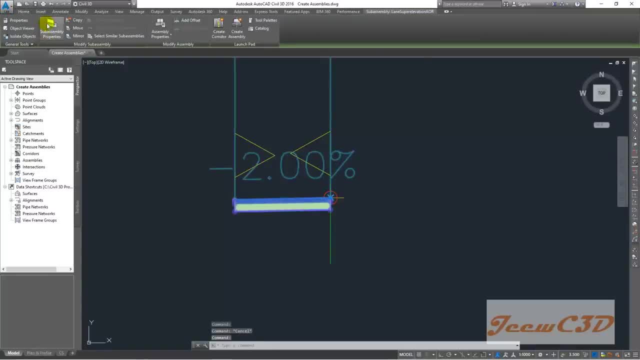 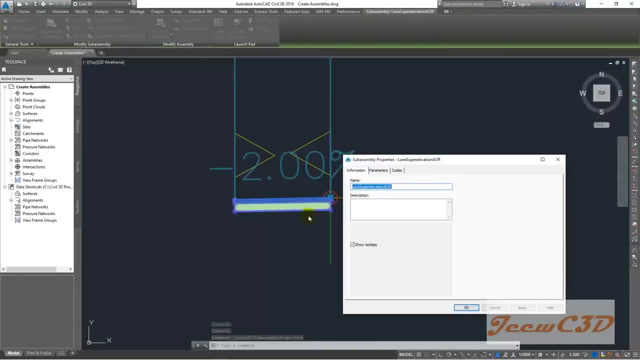 it by clicking here. then i from here i go to sub assembly properties. so my this part would be the left plane. i type it as left plane and my parameters could be side left, which should be 3.5. super elevation could be minus 2.5. default, my pair, one that could be varying course depth, that. 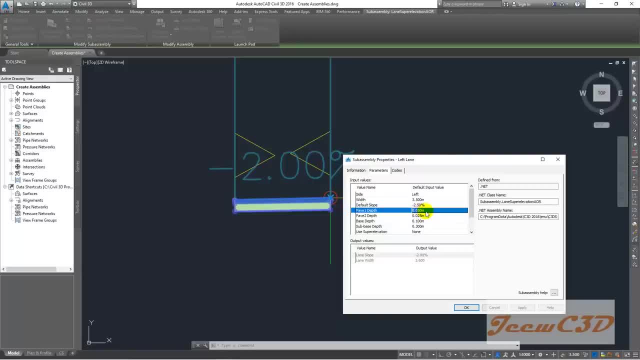 is 0.05 for millimeters- 50 millimeters, but in terms of meters it is 0.05. tail 2 is the bind, the course, and base depth is 0.2 and sub base depth will be 0.25 for use. super elevation option: we have to select. 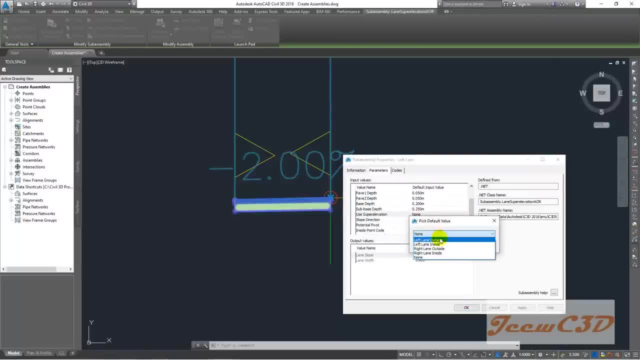 repeat here and select. since you are at the left plane, you have to select left plane outside. so if you can remember when one, when we fill up the excel sheet to import super elevation, we filled only two columns, that is, left outside lane and right outside lane. so we are telling civil td to get. 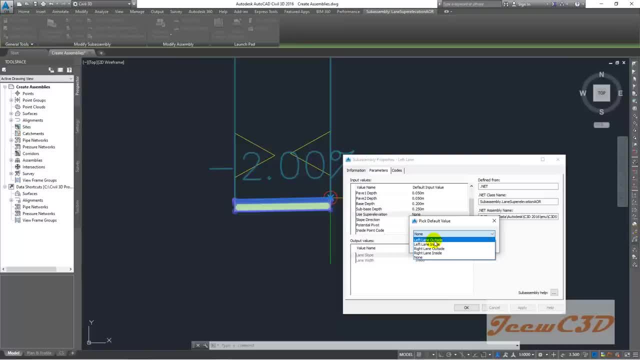 the super elevation values from the left outside plane. so here we have to set it to left outside plane. then you have to set this potential pivot to no and then this inside pointer would be problem and outside point port you say none. just type those values and click. 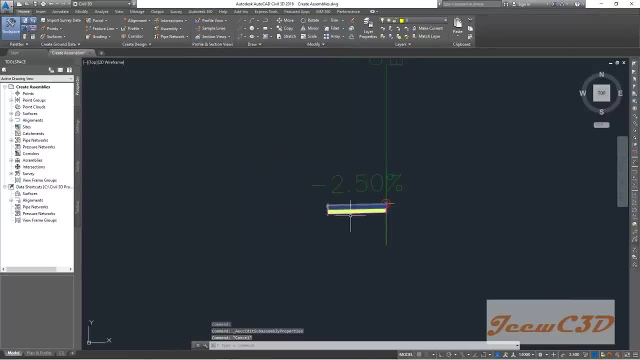 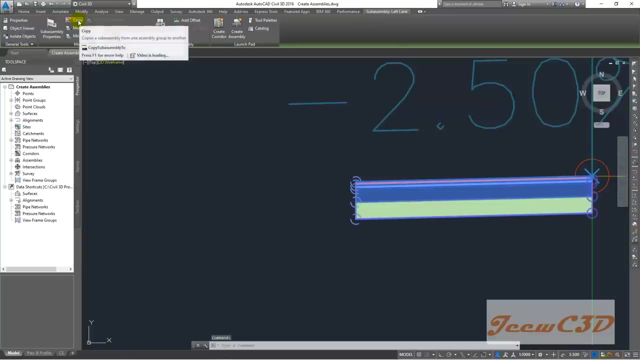 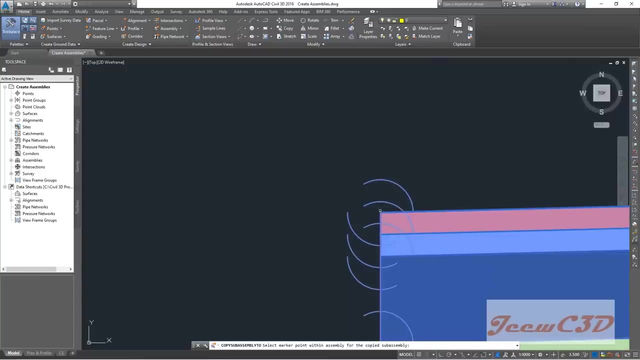 okay, so you will be getting this one, so your hearts holder would be same as this one, because you have the same layer. only difference would be the width. so what we do is we will copy this to this edge, so we select it. we copy it from here and we select this top circle to catch this edge. 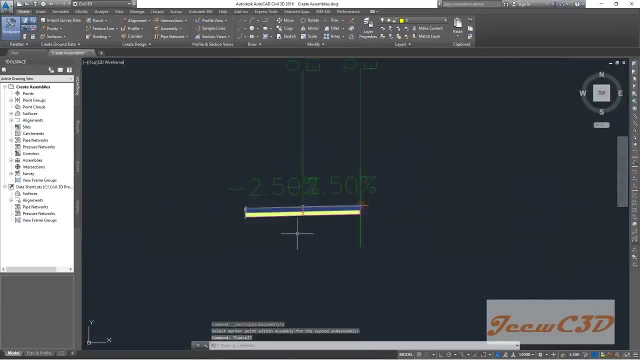 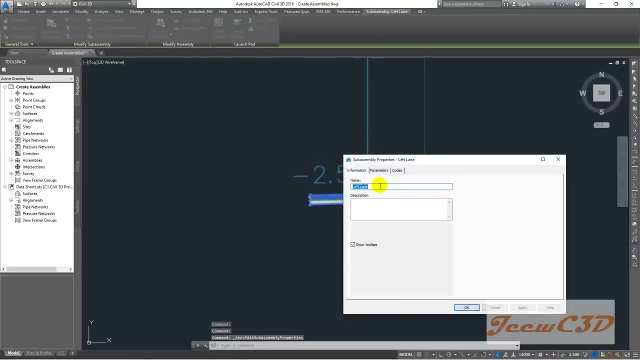 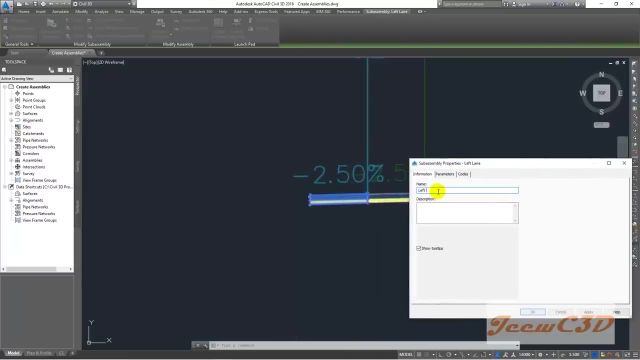 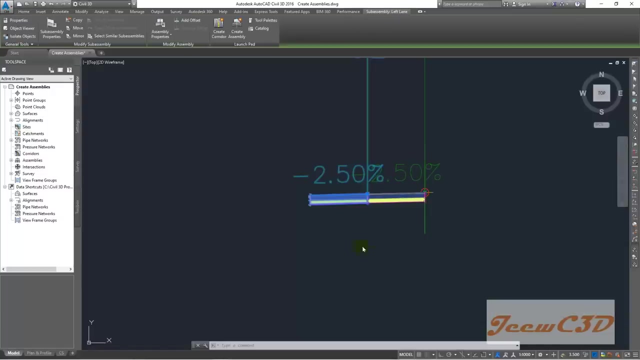 so it will be attached to this edge. then I select this one and go to sub-assembly properties and this time my this part would be left part shoulder, not the plane. I will type left part shoulder, so other parameters would be same as the plane. so I put them as it is. so far we have 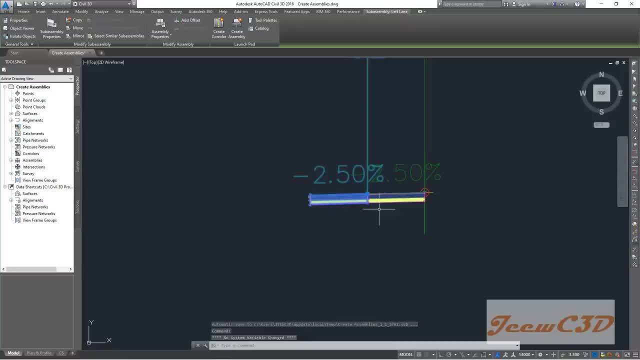 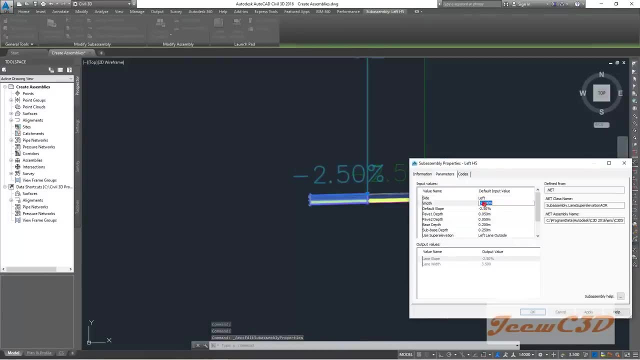 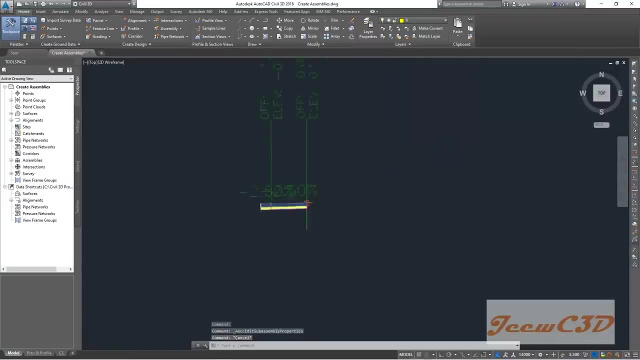 anyway, I have to do something. some change there. I select it again and go to sub-assembly properties and go to parameters, because the width should be 1 meter. that one is okay now. so if you think this is too complicated, this labels are too complicated, you can change the scale somewhere about 100%. 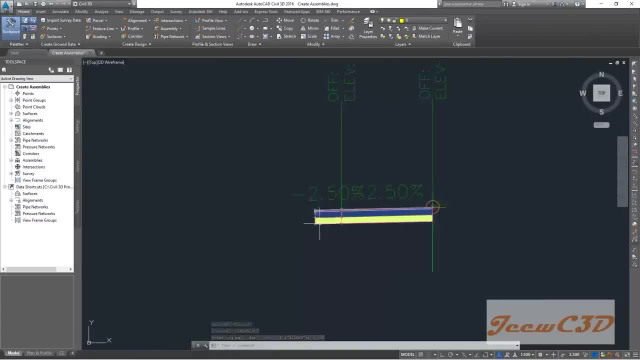 so I will change it to 100% so that you can see them clearly. now what I have to do is I have to mark the soft shoulder baby one meter. so what we do is we see the marks of shoulder and say in line instead of and each layers, we mark it as in line. because we will be doing a filling in this мест which we already marked last now, so don't skip till 6: 1m of max. as we mark this one layer to gr ot the every layer It certificated that 1 measurement will be marked. 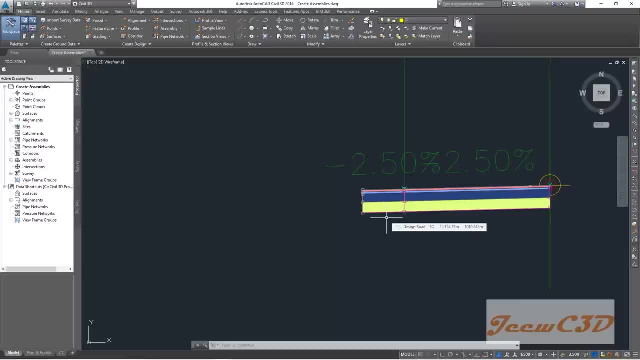 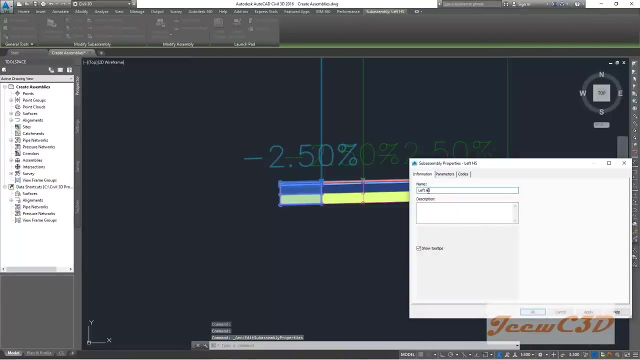 that location. so if you need, you can use some kind of a layer, but i will use. i will use a thin layer or a single line to represent the shoulder here. so i select this one, then i copy it from here and go to here. so i have copied this to the left side so i have to change the parameters. that should be left soft. 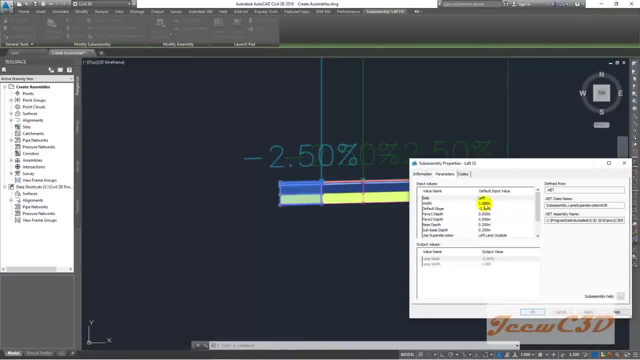 shoulder left ss and now, which could be one meter. but what i do is i change all the layers to zero, and here i would know super elevation applied here and default super elevation of the default slope of the surface is usually minus four. so i have set those parameters and you will be not having any. 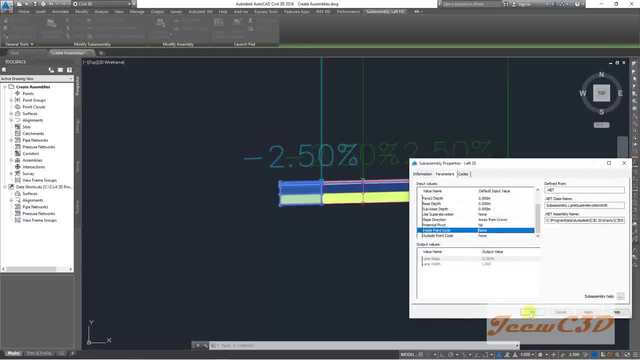 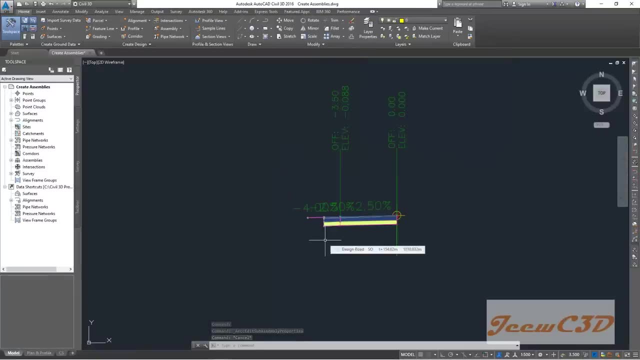 point codes in this section, so i click okay. so far we have created the plane part shoulder and the soft shoulder. so there are several ways to create these things. instead of using the lane assembly here, you can use shoulder assemblies as well. so, if you do, when you get more experience you can use them, but as a practice i am going with. 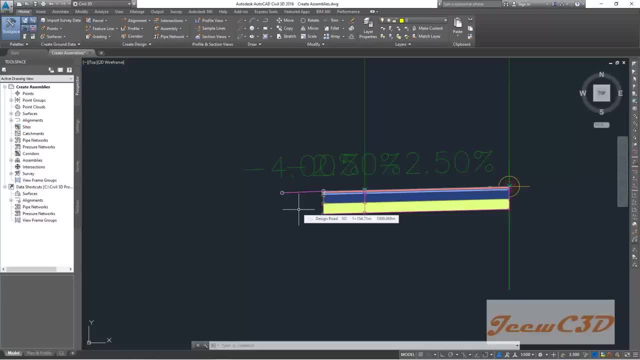 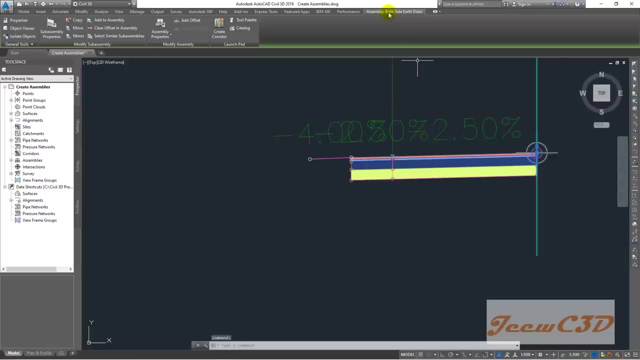 as for the practice, i am only going with one assembly so you that you can get the easy idea. then what we are talking here is: if i click here, you can see both side the earth plane assembly. so what i am having is a earth drain assembly. so, if you can remember, usually we have earth drains at the end of 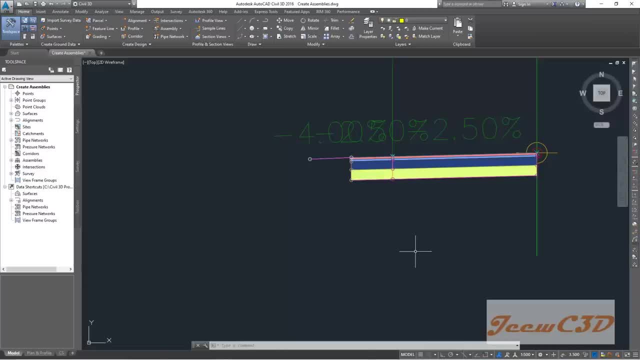 the field section or especially at the cut section. if you have a cut section where you have some kind of a cutting situation, at the end of that cut situation you will be having an earth drain. so i will mark the earth drain here. but i will think, i will think so. i will make sure that this earth drain will be there only if there. 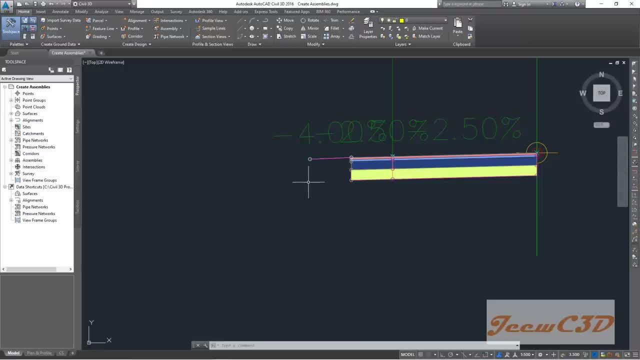 is a cut section. only if there is a cut section you will be having a drain, otherwise you will be having a fill only. so i will describe it sometime just in a few minutes. so so if you want to get the earth drain assembly, you have to go to 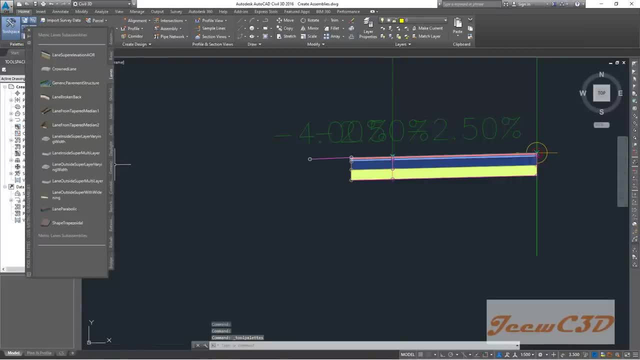 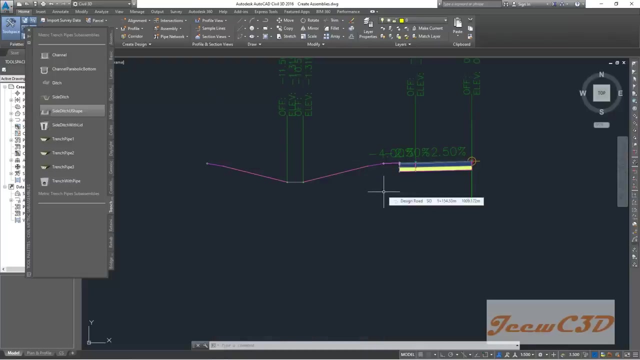 tool palettes. then you go to trench and then you go to ditch assembly and you click it here. so you will now see some kind of a long section assembly is appeared. so this is called the ditch. but you, this is a very large assembly, so we have to modify the parameters. 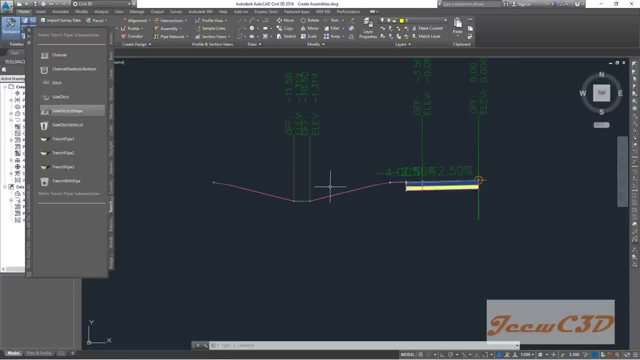 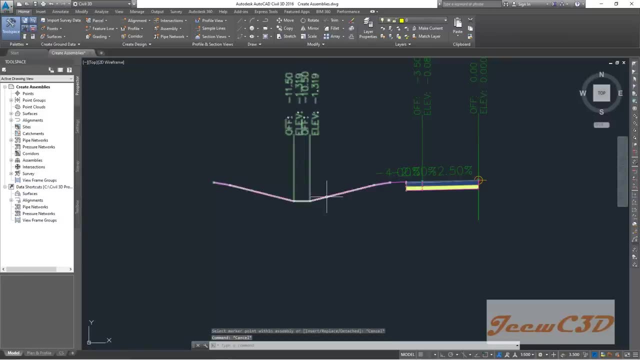 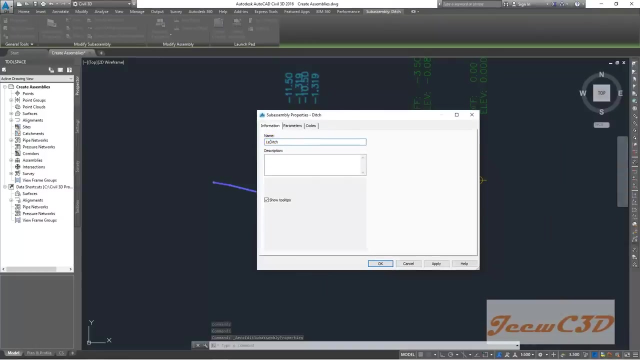 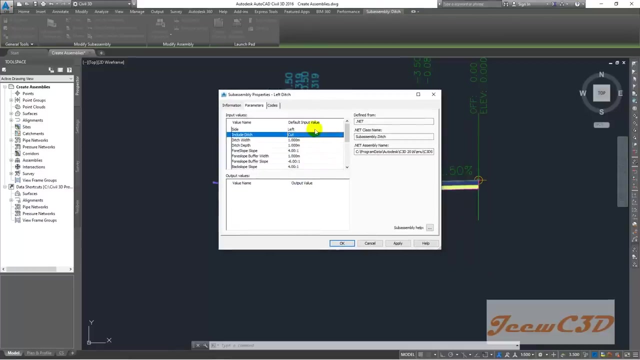 to get the required drain from here. so to do that i will modify this. So I click this one and I go to subassembly properties, so I will type the name as fditch and so it will be applied. only include ditch only will be at third section and I have 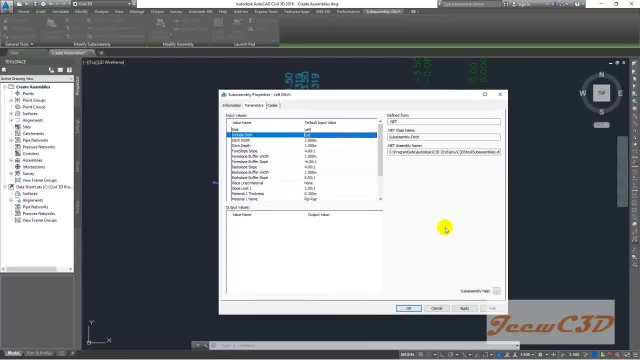 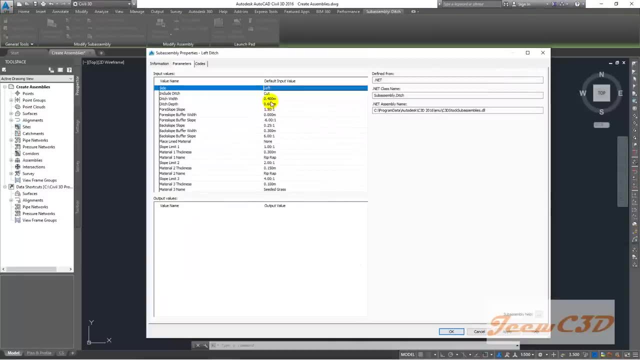 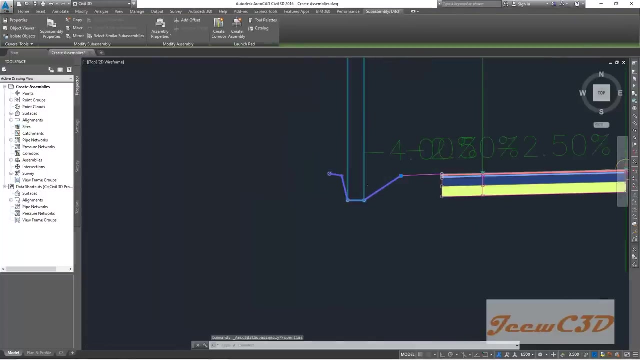 to fill more. fill some more parameters here. so once you fill out all the parameters, it will be looking like this: you can fill out these parameters in your assembly also, so I will click ok now. so it will be looking like this: the drain will be looking like: 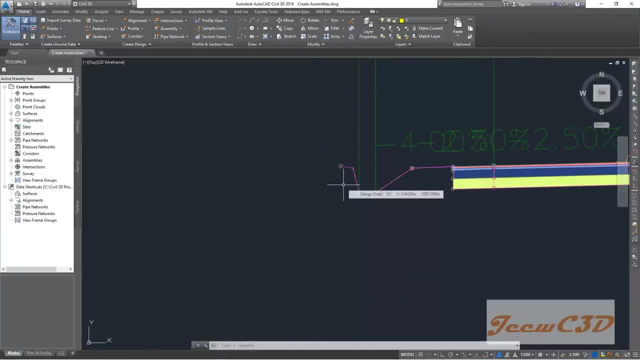 this. So if there is a drain, it will be looking like this: Then, after the drain, you have to add the cut and fill. If there is a cut, it will be going like this. if there is a fill, it will be going like: 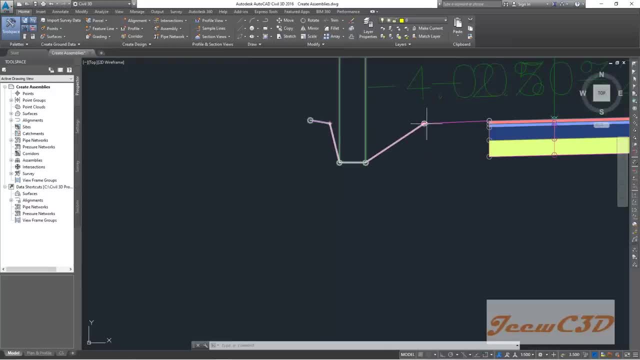 this. Actually, it will be not going from here. it will be going from here because we say this ditch will be included only if there is a cut section. So to add the cut and fill, we call it the daylight. 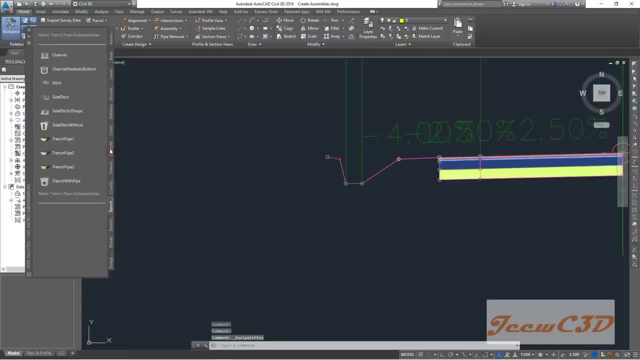 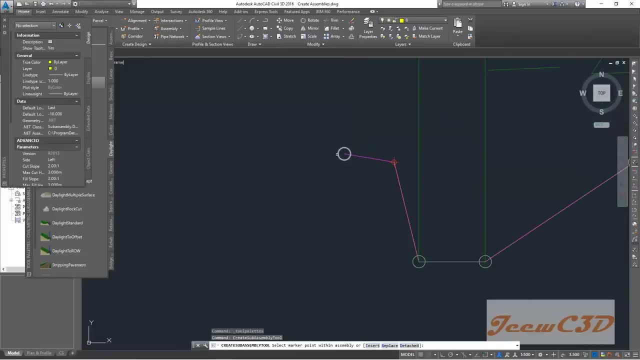 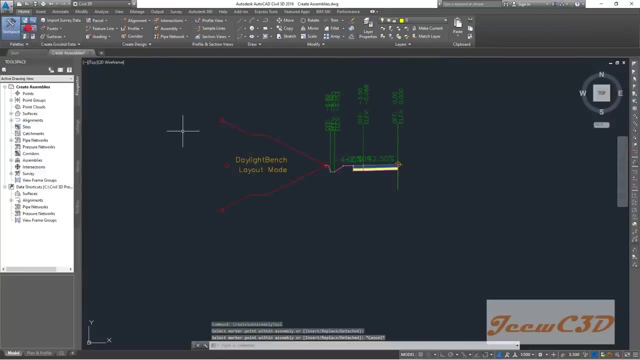 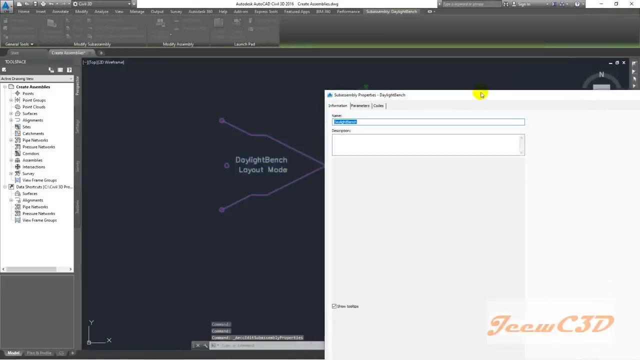 So we have to go here. then you go to daylight, then you go to daylight bench. ok, you click this point so you will be getting a daylight bench assembly. so I close these things and I change the parameters of the assembly so it should be left at the daylight bench. 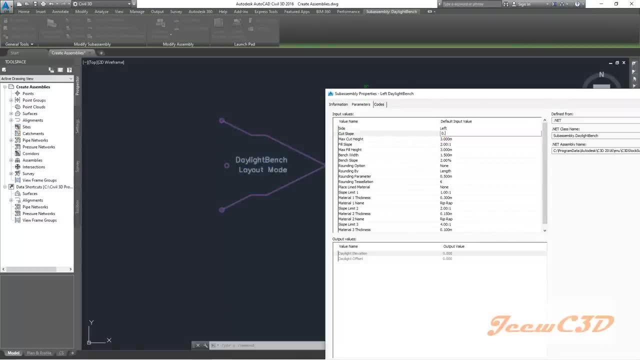 and this cut slope would be 0.25 to 1,. next height height would be 4 meters. this slope would be 1.5 to 1, next height cut height would be 4 meters. bench would, let us say: 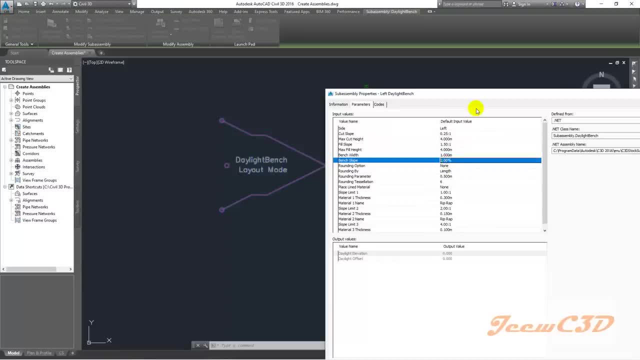 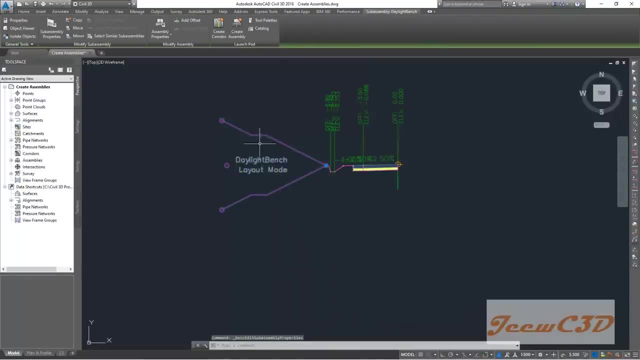 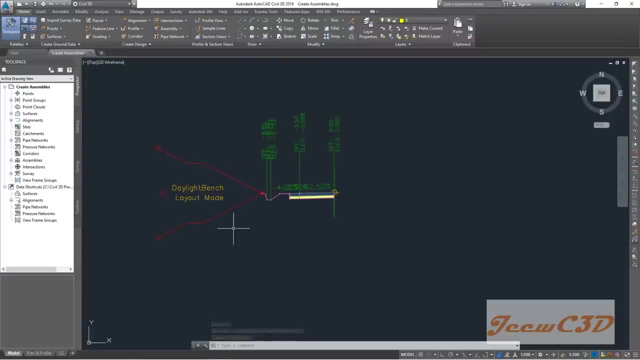 1 meter bench slope: 2%. so these are the values we have to type in and then press ok. so you will not be seeing any change here. But the changes are readily modified into the assembly. So then you have to fill the right side, same as we did for the left side. 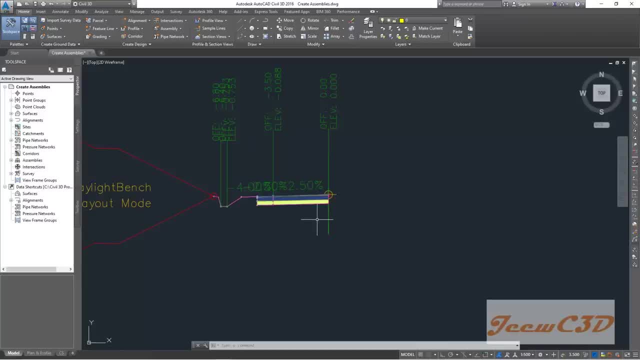 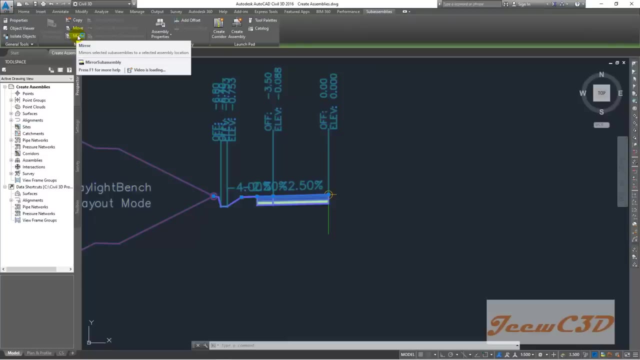 Instead, what we do is we select all the assemblies from left to right, right to left, like this: Without this green one, we have to select these things only Then we click mirror. here, when it is asking what is the mirror assembly, we click somewhere. 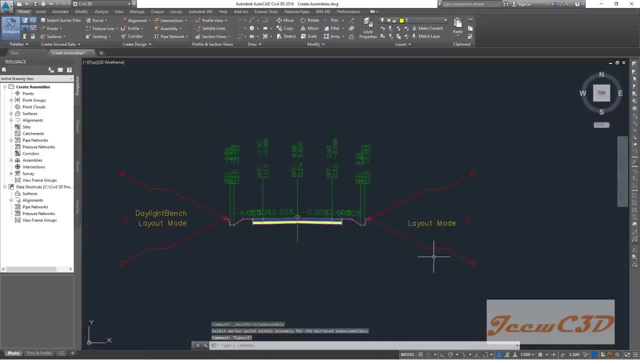 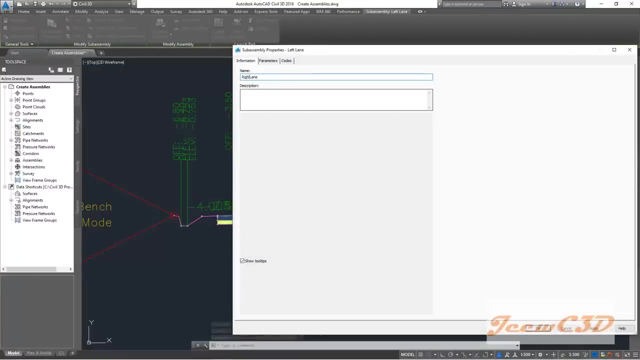 here. you will see it will reflect to the other side. but you have to do some changes because if you click this one, you go and it is not left lane, it is right lane Again. this would be super elevation at the right lane outside. 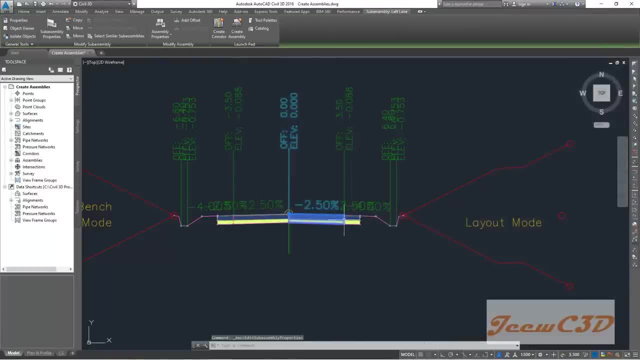 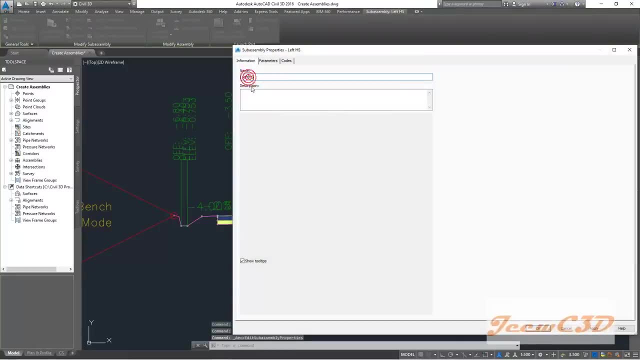 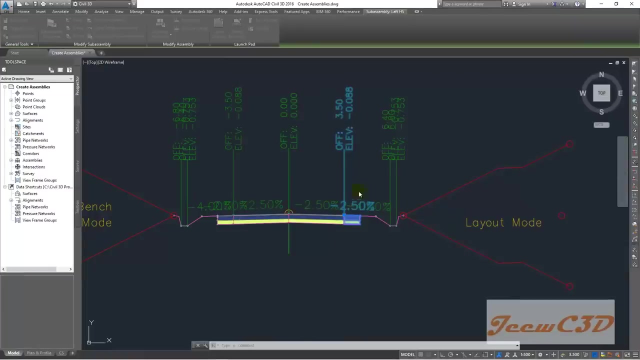 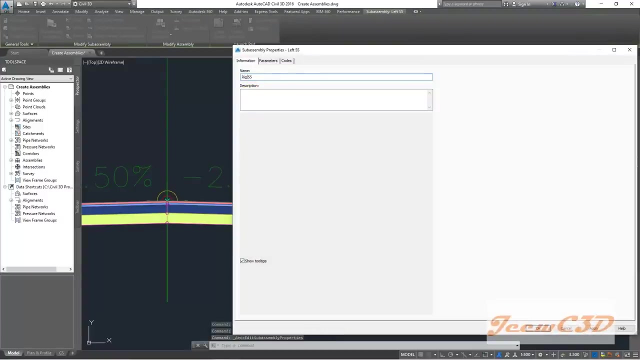 Click ok and I press k and then I go to hard shoulder, which would be right hard shoulder, and these are the values and this would be right lane outside. Press ok. so this one would be right. soft shoulder values would be changed in the soft shoulder. 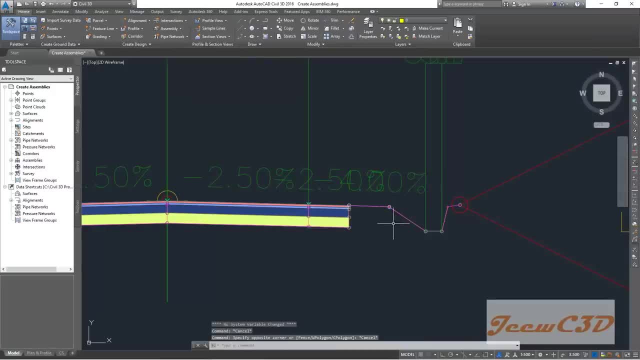 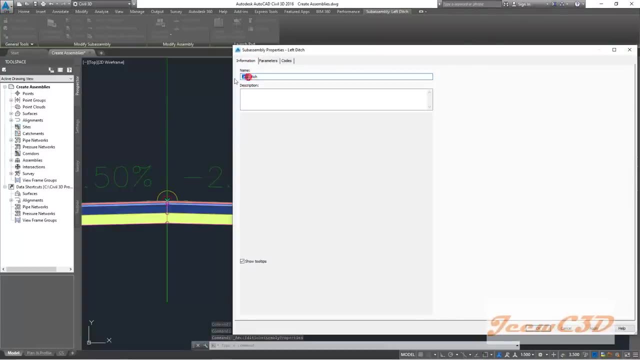 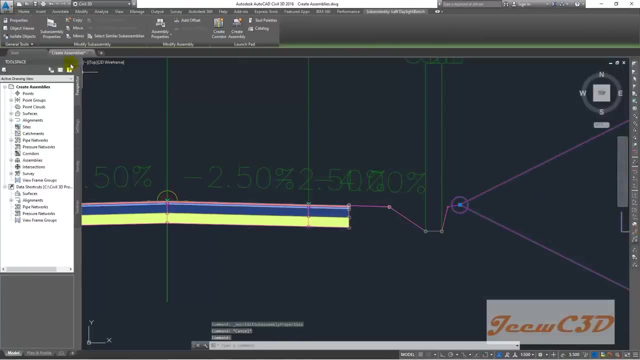 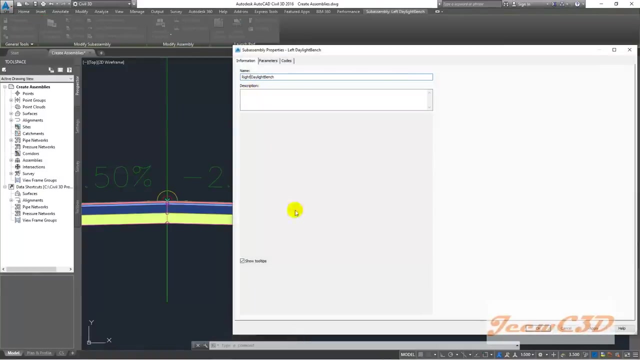 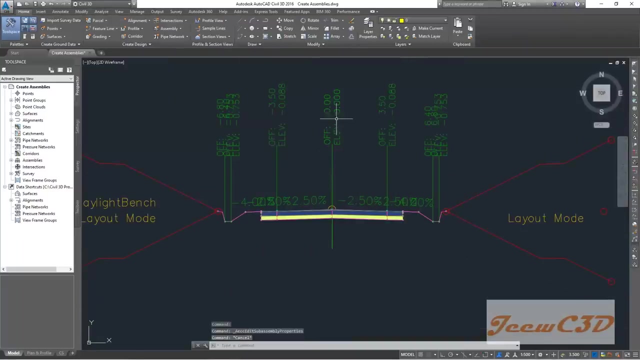 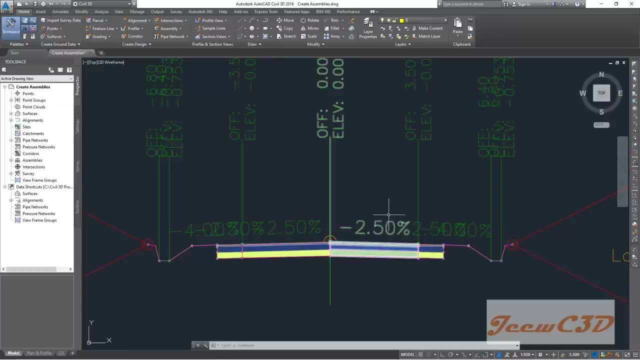 and this would be right side And finally this would be right daylight pinch. So we have created the first assembly here. you can see these are the representation, assuming that this is zero elevation. so if we apply super elevation here, minus 2.5,. 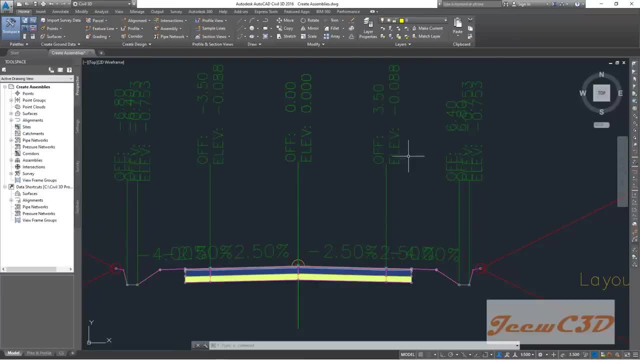 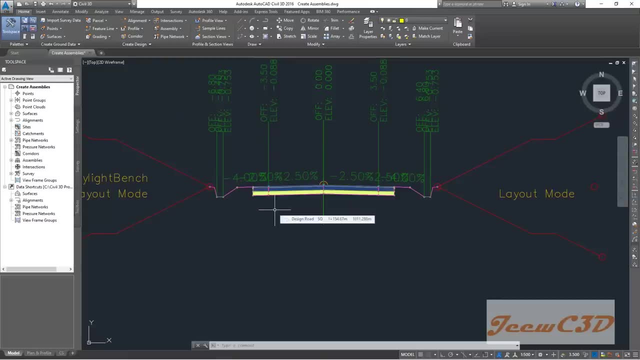 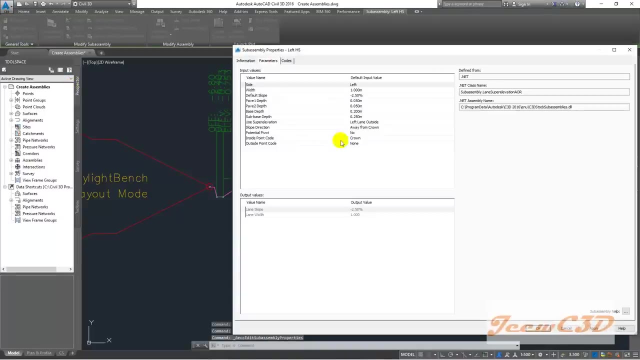 with the width of 0.5.. Ok, With width of 3.5, you get these values. So I have to tell you one thing. I forgot to tell that thing earlier. In this sub-assembly you have to go to sub-assembly properties and you have to change the point. 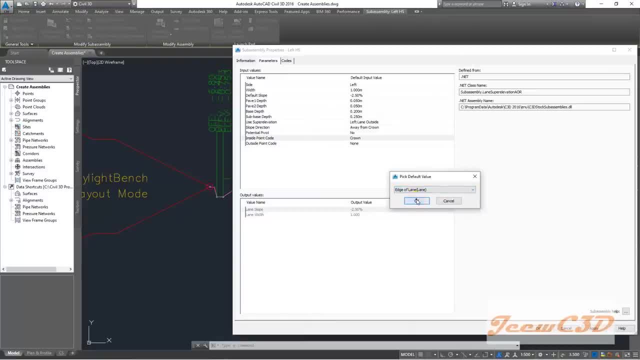 port from edge of lane to inside point port and adjust payment ETW to outside point port. So this was this part also. you have to do it: Lane and ETW. So that is the change you have to do. 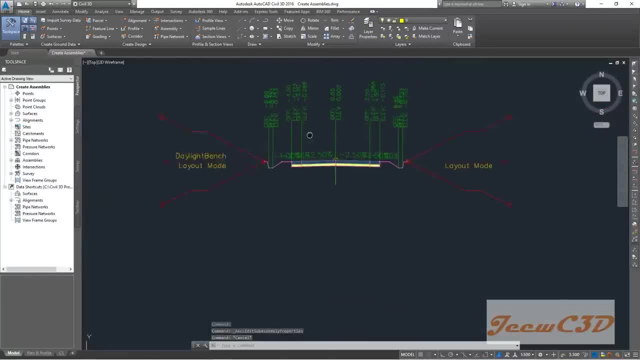 So once you do that change, you will see this label appearing in that location. So we have now completed the earth drain part in the next session. In the next session we will create the bridge assembly and the concrete drain assembly. In this session we will be creating the other two assemblies, meaning the, that is, the. 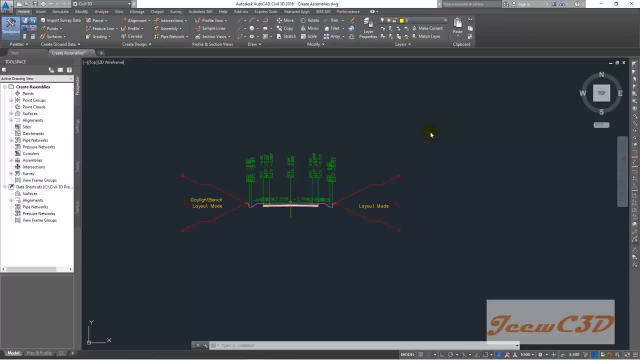 assembly with concrete drain and the bridge assembly. So we are still continuing the last loading. So to create new assembly, I go to home tab, Then go to assembly and create assembly And this time it should be both side concrete drain. 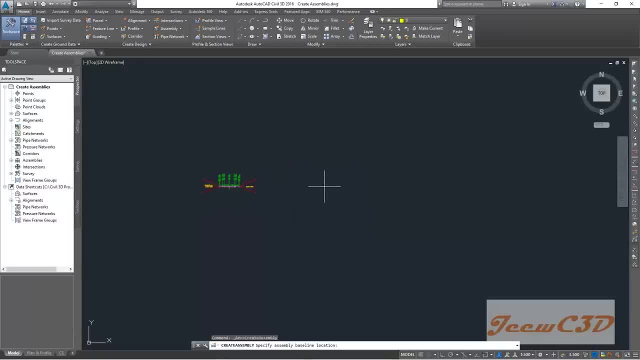 And I click ok, So I will be clicking that somewhere here. Create the assembly. So in the concrete drain assembly also you will be having all these three sections Lane: hard shoulder and soft shoulder. So what I can do is I can copy these things to this assembly, except this drain part, earth drain part and daylight part. 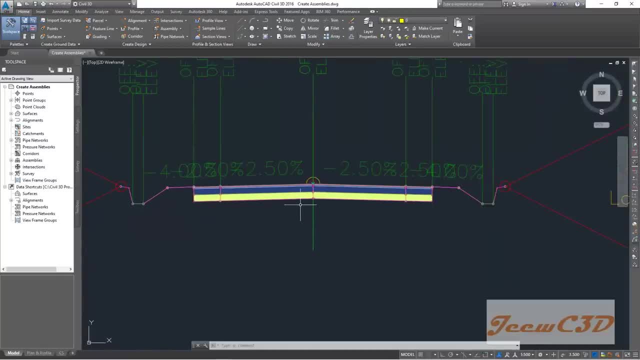 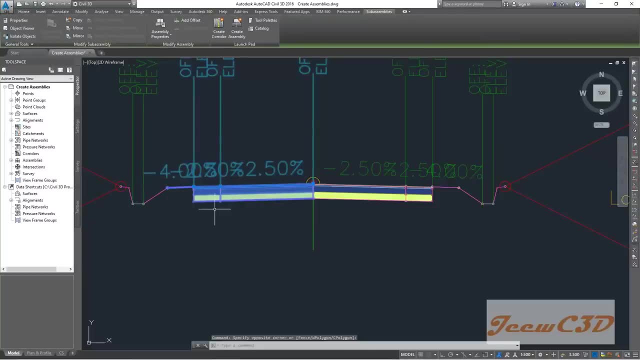 So what I do is I select, put my cursor somewhere here, Then I select these three, only These three, only So you can select one by one. So like this: I press A, I select this one, then this one and then this one. 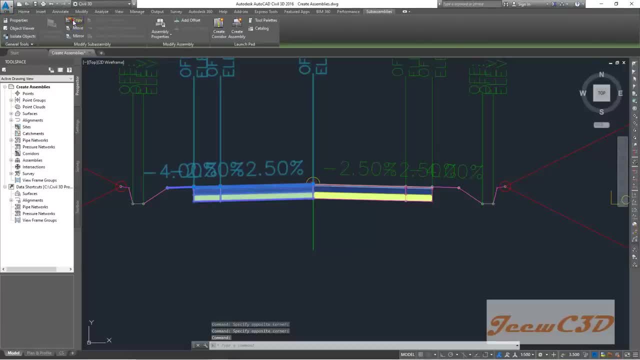 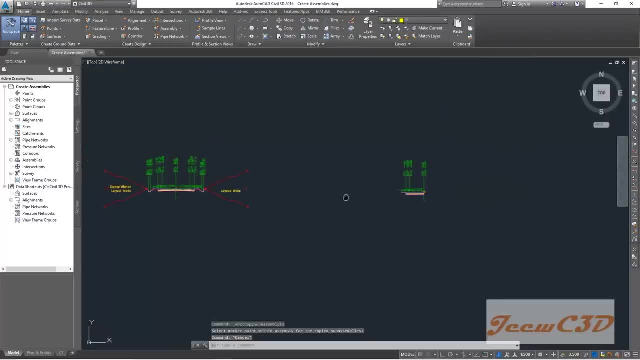 Like this: you can select in your copy And go here. So by this method you don't have to change any name, So anything, because they are already there, as in the sub-assembly here. So then I copy the right side. 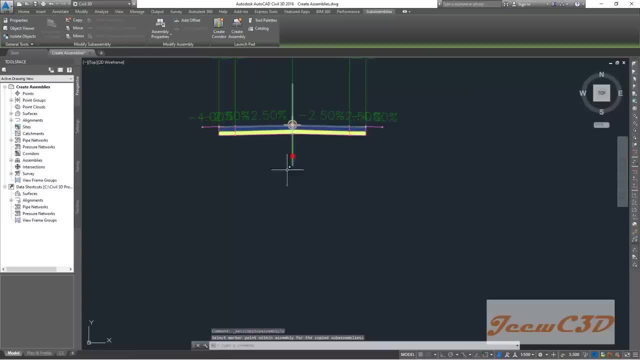 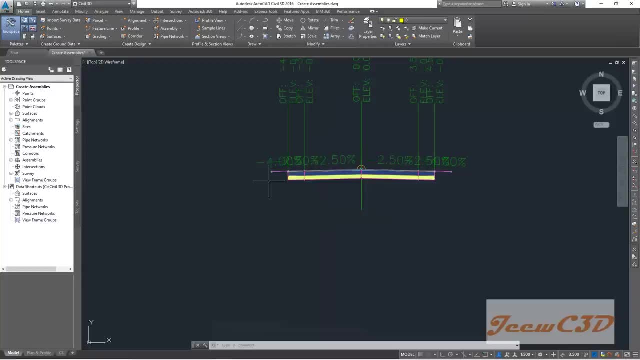 Right side here. Just click here. Right side will be copied. Now what I am going to do next is I am setting the concrete drain here. To do that, I will go here To Eucalyptus, Then I go to French tab. 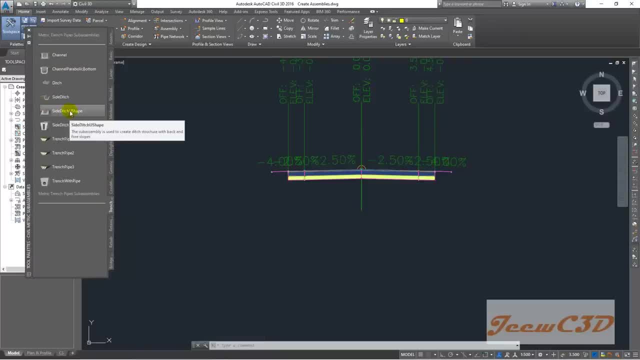 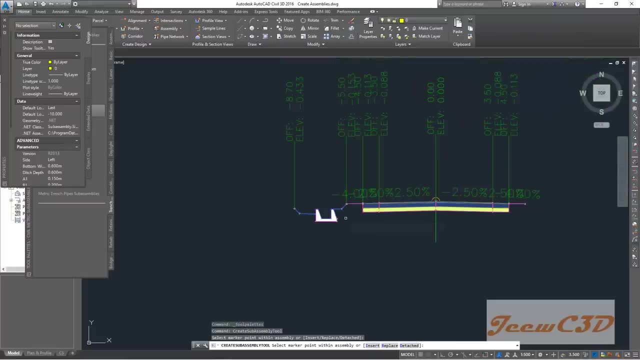 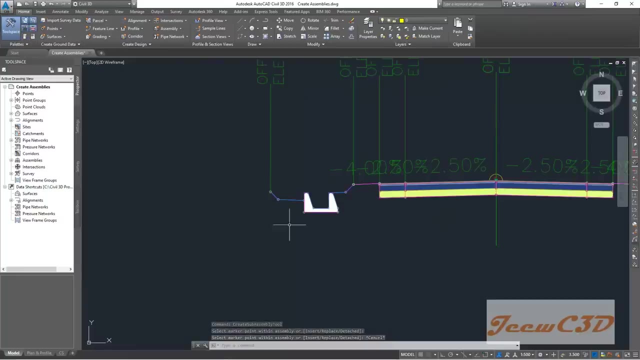 Here. Then I go to side dish, Go to shape, So I will attach it to the left side first. So this is the decoy. Same to be equal. I press A And I close this one. Then I have to do some modification to this. 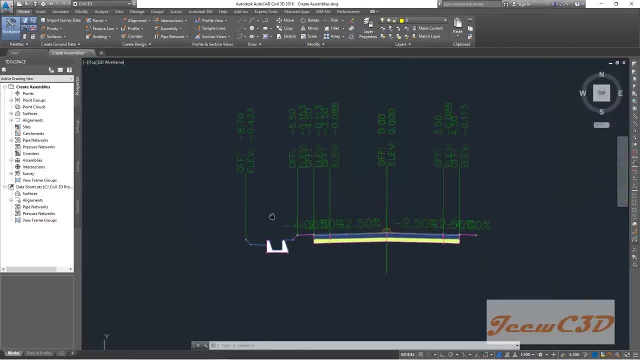 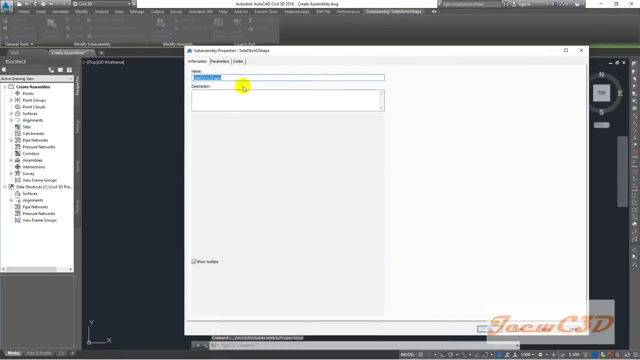 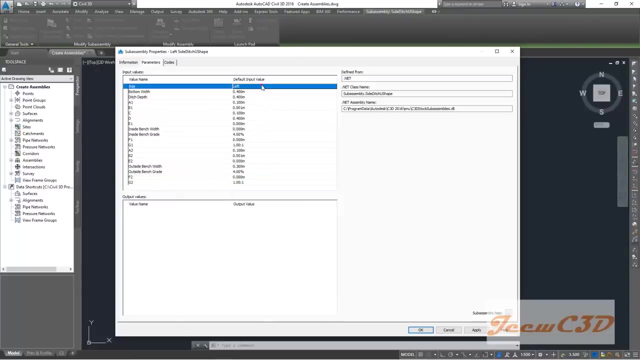 To get the required drain. So I click here, Then I go to the same properties, Then this is the left side dish user And I have to change this parameters. So I will change this parameters now. So you want to fill out all these sections? 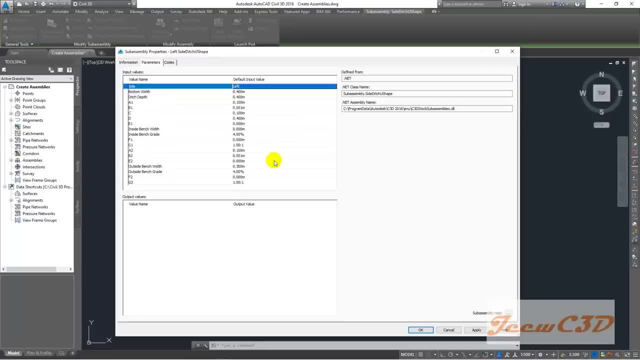 You can fill these values. You can fill these values. I have used this 1 mm values Because I can't use 0. It will give you an error. Instead, you have to have very small value. I have put 1 mm to show you the value. 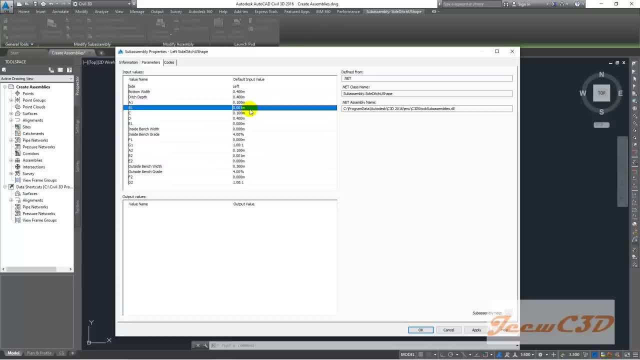 So you can even put a value such as 0.00001.. To get something close to 0. But you can't type exact 0. Because it will give you an error. So if you need to know more about assembly, 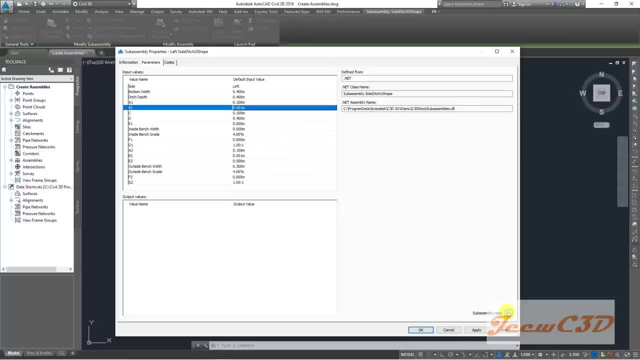 You can click help here So it will show you all the help related to this assembly, So you can get the help from any assembly you work with From here as well as from here, So sometimes it may not be working with you. 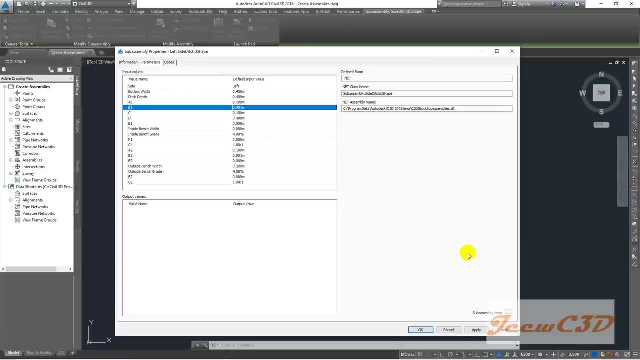 If the help files are not installed in your computer. So in that case you can go online and search for the help files, Or else you can download the help file. So since we have completed this part, I will click OK. 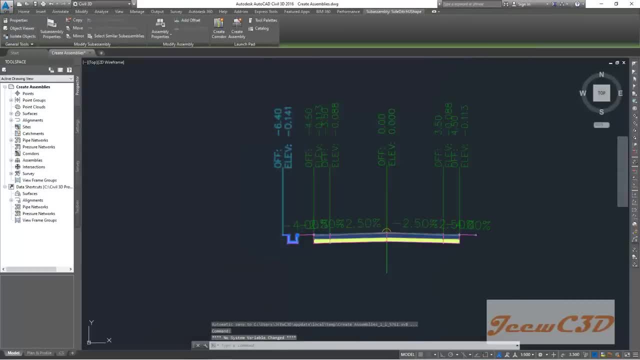 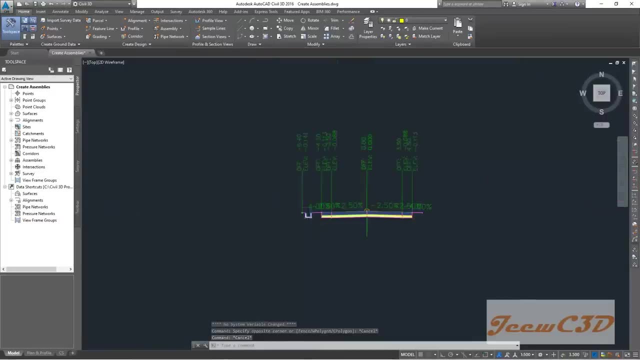 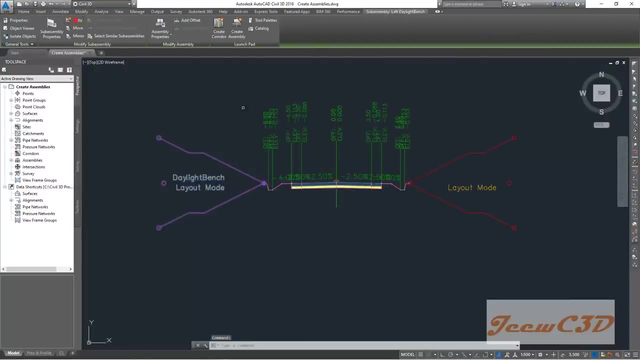 So you will see this kind of a drain appears here. Then what I do is I am going to have the lay light part at the end, So I will copy it from here. Copy and click here to set it to here. 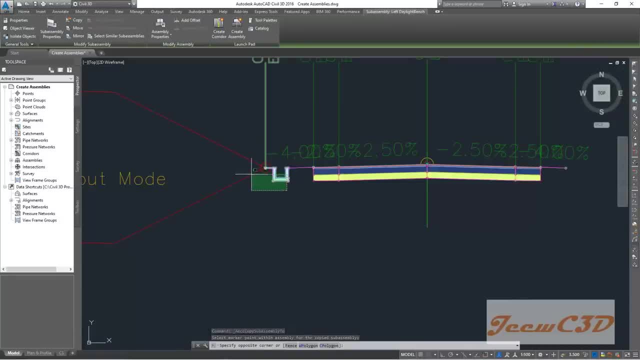 Now what I am going to do is I will mirror this. Actually, I will mirror this one only. So I click this one, Then click mirror. So if you don't see mirror here, That means let us say if you click something. 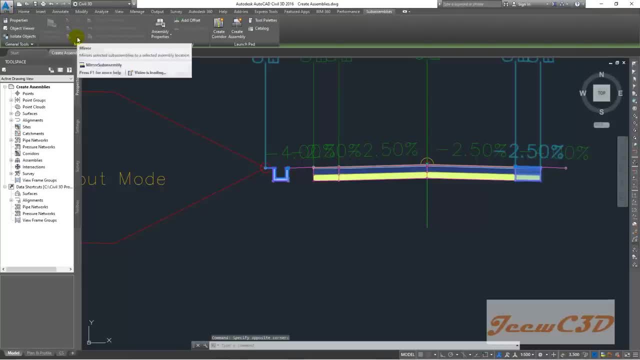 Something else this side, So mirror will be disappear. In that case you have to press K And click it again. So I press mirror And I will mirror it to this side, But I have to change the name. 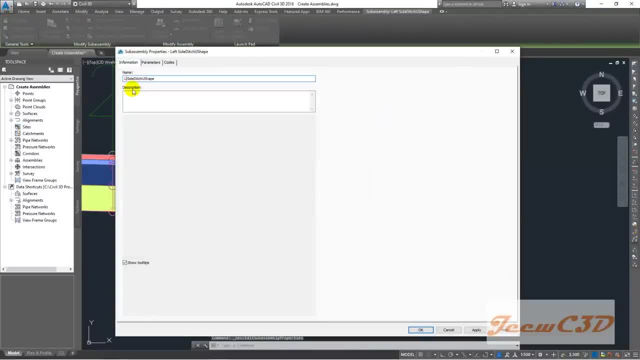 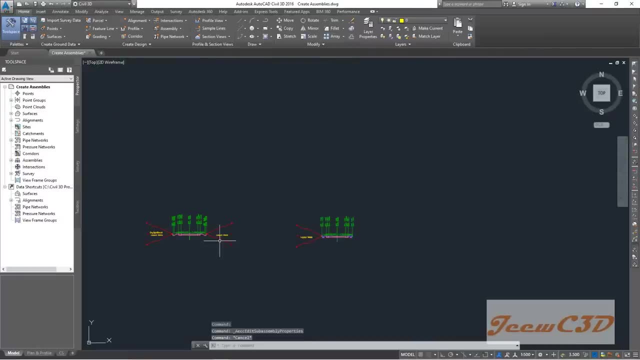 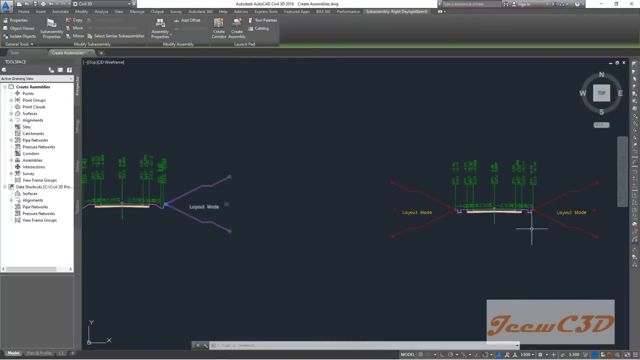 Go here And change the name as right. I will click this way. Then I copy the Lay light assembly from here To this point. So I copied it from here, And if I mirror it from this point I have to change the name. 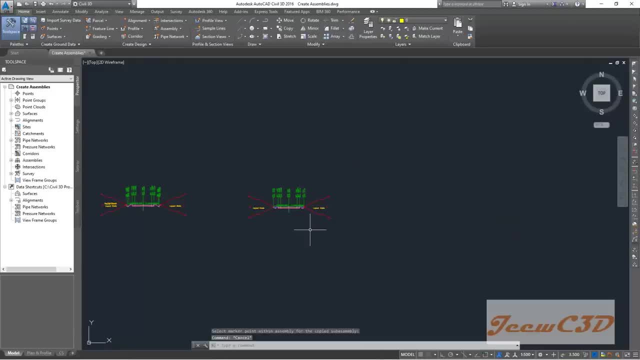 If I copy it from here, I don't have to change the name. So now what is left is Only the bridge assembly. So I will do the bridge assembly in a separate way. So what I do is I click copy here. 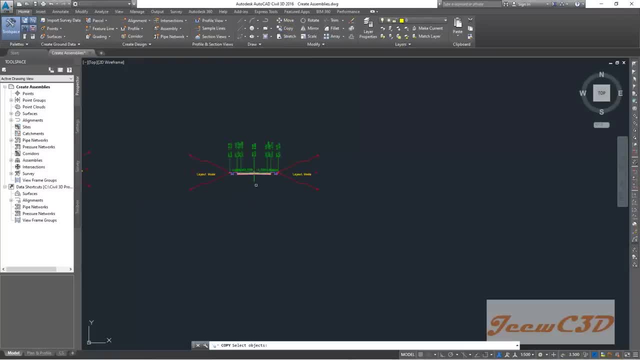 I click copy here, Then I select this assembly, Then press enter. It is asking for a base point. I select this, Select somewhere here at the bottom, Then I paste here That second point. I will paste it here. 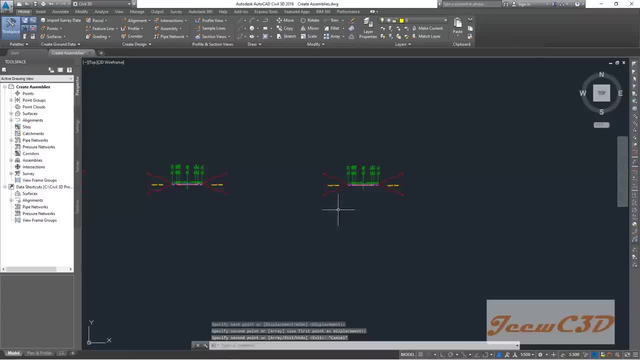 Then press enter. Otherwise you can select all these things by click, copy and do the paste, And it will do the same thing. Now I have done it. So now what I am going to do is I am having a bridge assembly. 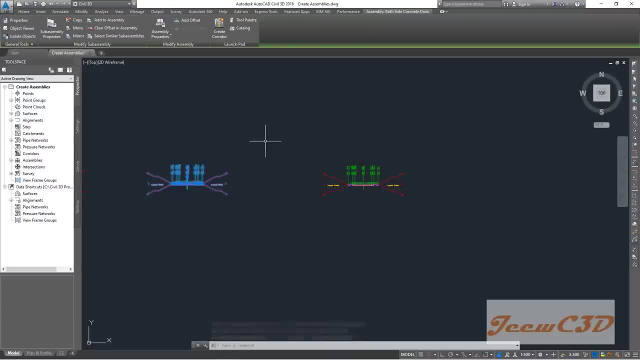 So I don't need these things for bridge part and clip, So I will get these two by just pressing delete. So like this, I have done two parts And the last is a bridge assembly. Please don't forget to give like and subscribe to this channel. 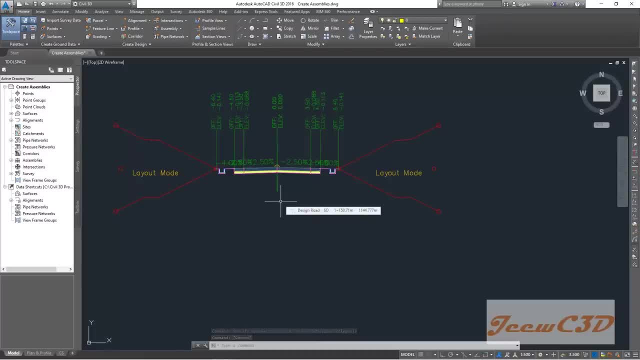 And I will see you in my next video. Bye-bye, Thank you. Bye-bye, Bye, Bye, Bye, Bye-bye, Bye, Bye, Bye, Bye, Bye. I am just pressing delete button after click on it. 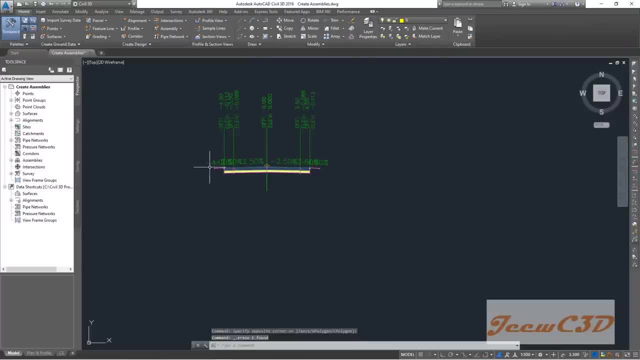 I will not be having no change for it. so let us say I have this for footwork, these 1 meter sections, so depending on the big section, we may have some kind of a larger value. so we have to use those values from the typical constructions. 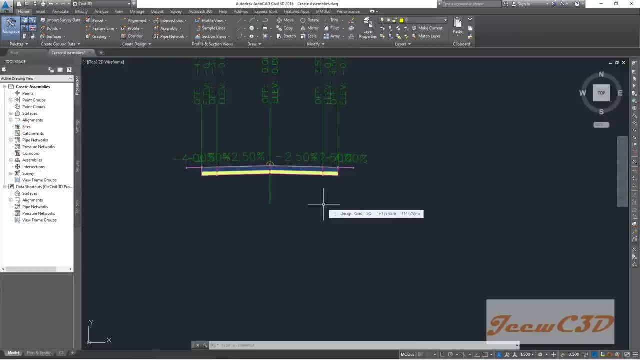 from the big engineers. but I will keep straight to the current values. now in this we don't have ABC or the base post or sub base in a big section, so we have to remove those layers. so I will tell you a quick way to remove those layers. 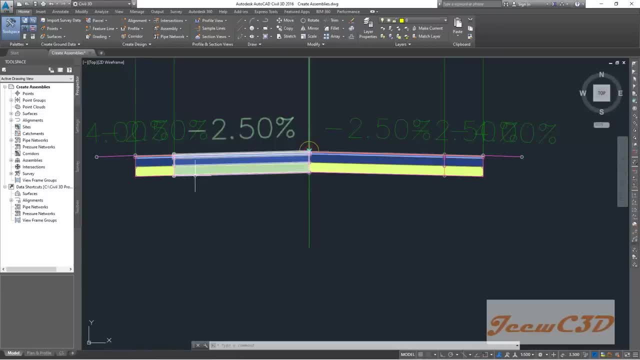 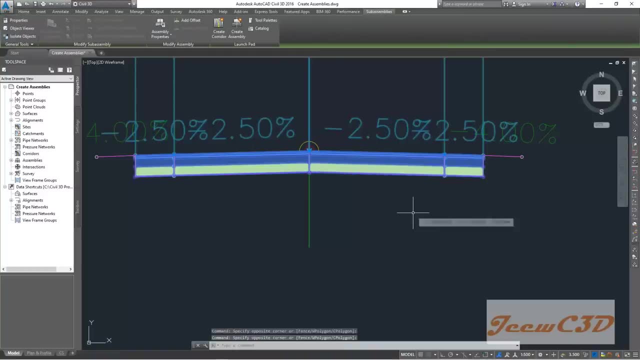 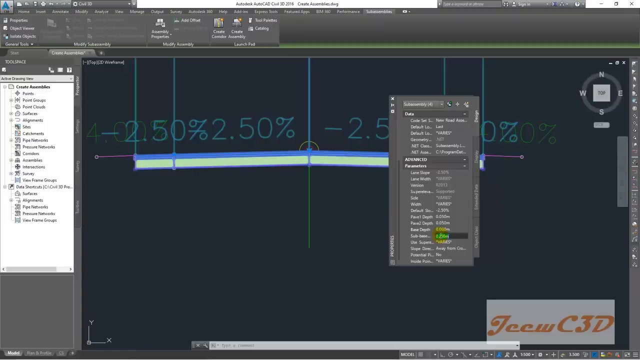 if you see all these sections you have same layers. what I do is I select all of them like this and write to go to properties. then from here I drag it to here, from here I change it. 0 and 0 those two layers, I make them 0. 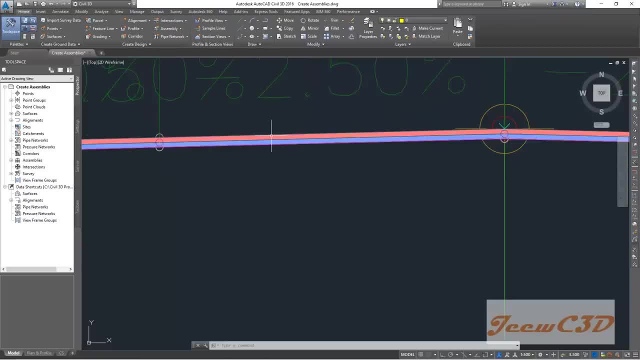 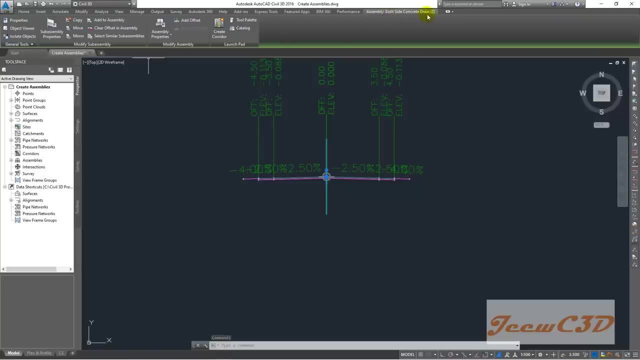 then I press close and we only have a varicose of 50 mm and binder of 50 mm, but still I have to change this name of the assembly. so I click here because my name is both side concrete drain 2, so I have to change it to boot assembly. 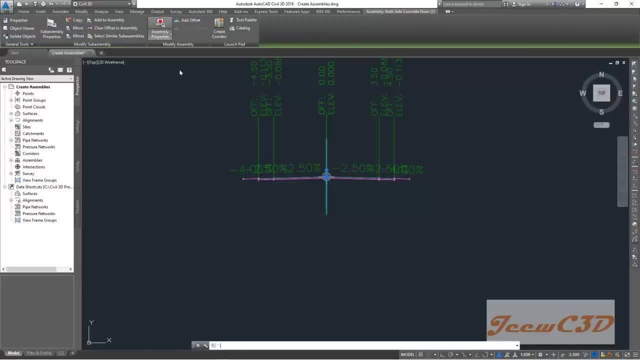 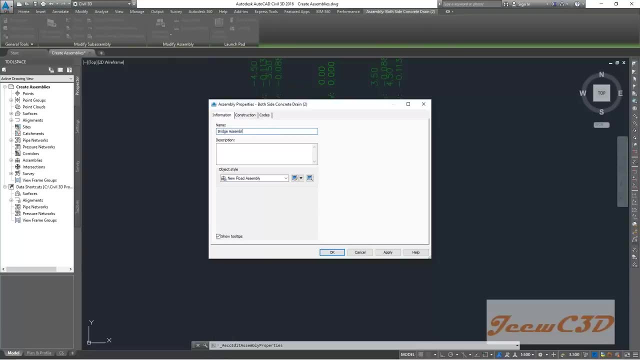 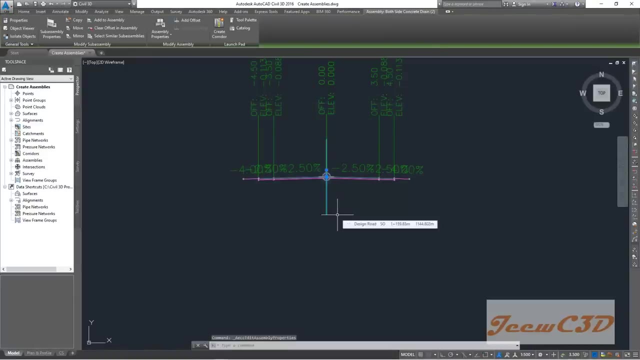 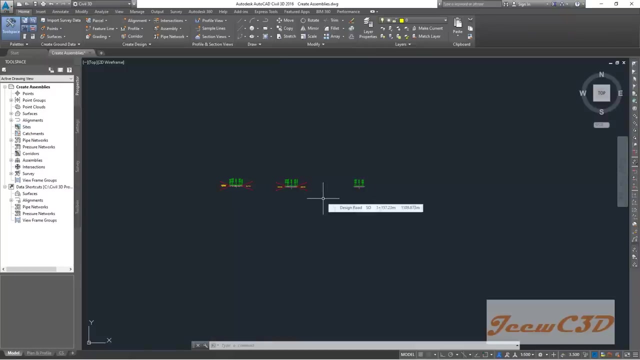 I select it here, go to assembly properties and I change the name as switch assembly and click ok. so then I press k to deselect that one. so far we have created all the sub, all the assemblies, all the typical cross sections. that means the drains, concrete drains and 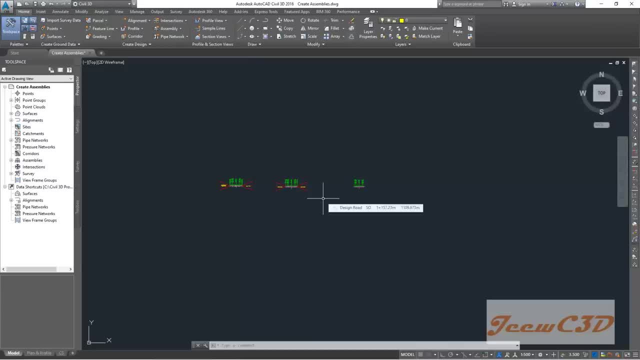 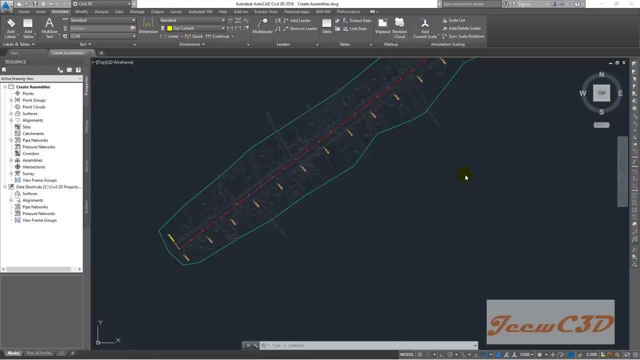 with sections. in the next video we will be looking at how to create the corridor for the road section road trace via design. in this section we are going to create the layout of the road before creating the corridor. this can be done even at the start of the 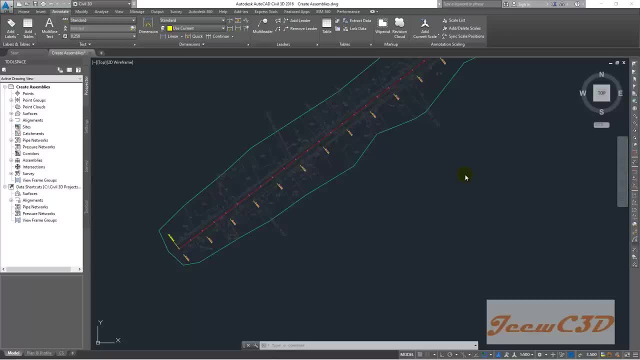 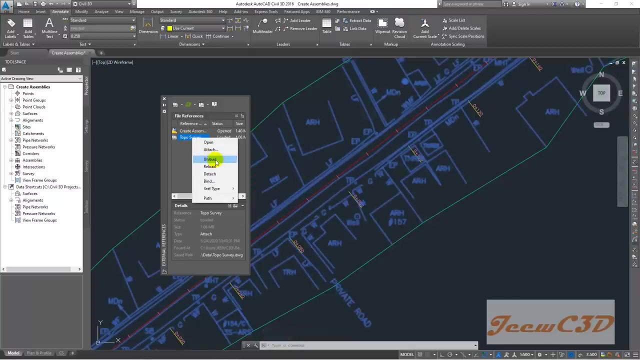 alignment even after creating the alignment. but I will do it at this moment before creating the corridor. to do that, first I will unload this xref. to do that, I type xref in my command line, then I select this topo survey and click unload. so it will be. 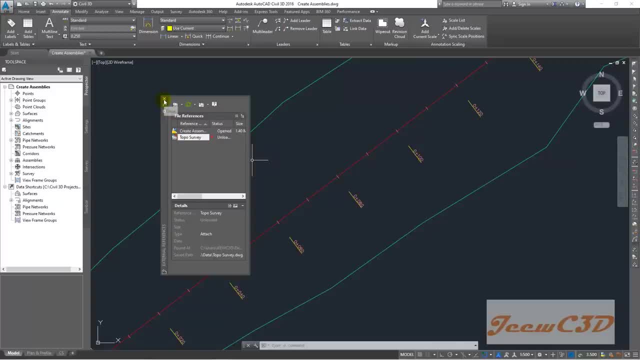 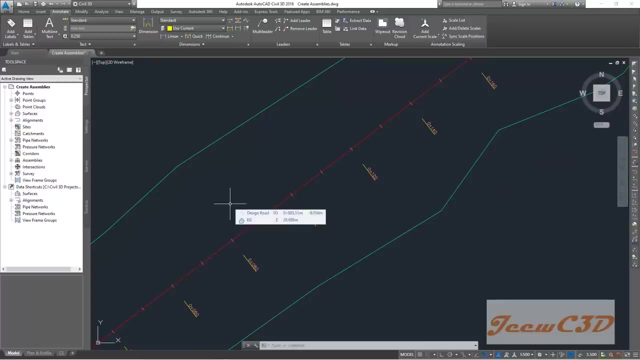 deselected for moment, then I click close. now I will do something called offsetting the road section to get the alignment. that means we are creating the plain edges, hard shoulder edges and soft shoulder edges to represent the layout of the road. before that, I will change my scale. 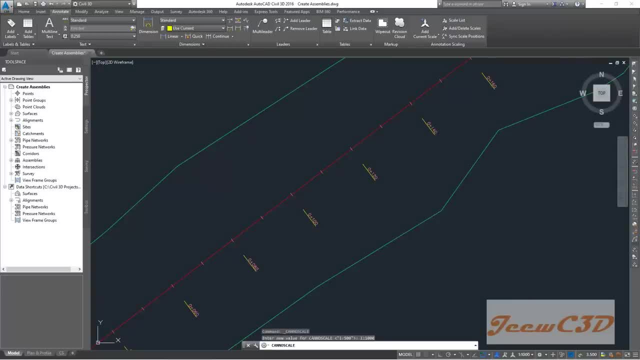 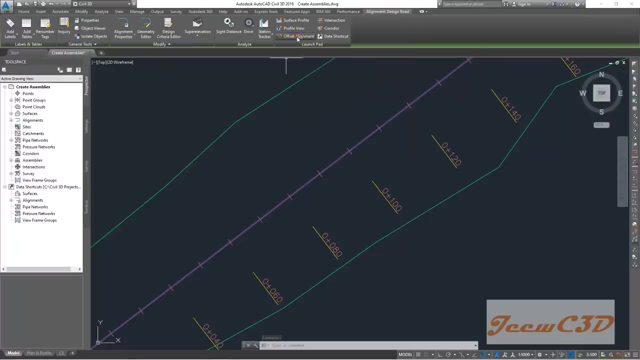 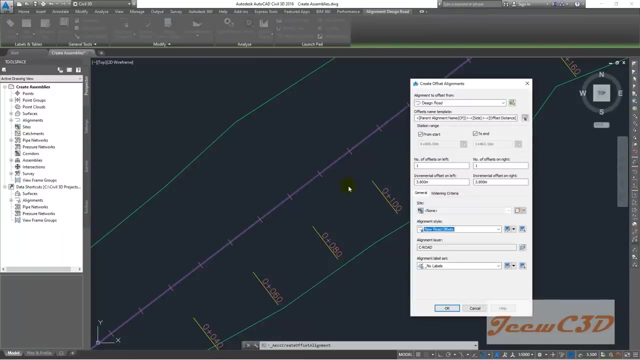 to 1000 so that I can get a bigger view of the window. to get the offset alignment, I will select my alignment then from here, select offset alignment. so we have 3.5 lane either side of the road. so here our lane is from start. 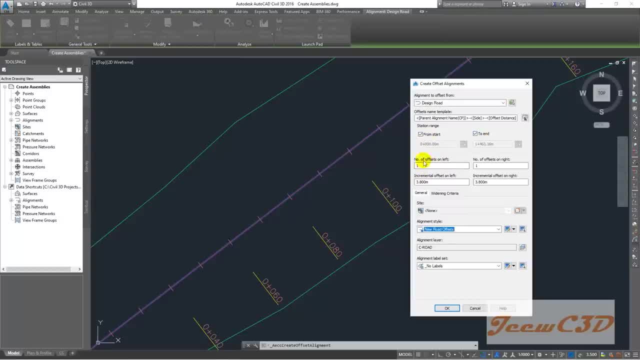 to end. so we have one lane to the left, one lane to the right and lane width is 3.5 and the other lane is this also 3.5 and the alignment style would be in road offset. alignment style means how this alignment looks like. 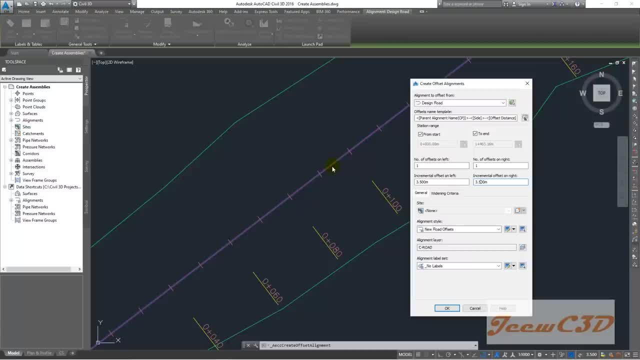 so in this alignment it is looking like red and blue. you can see straights are in red and curves are in blue, and this is the style we are going to use for the offset alignment. we will see how this looks like once we press ok, so I 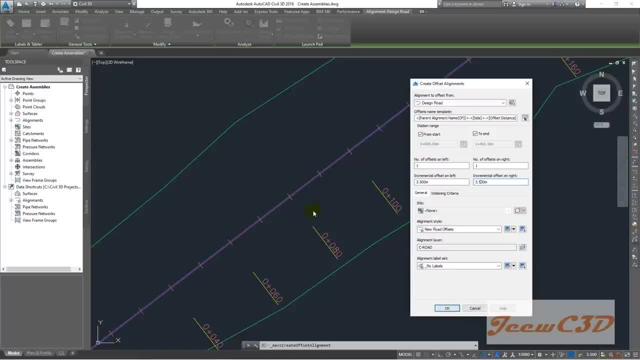 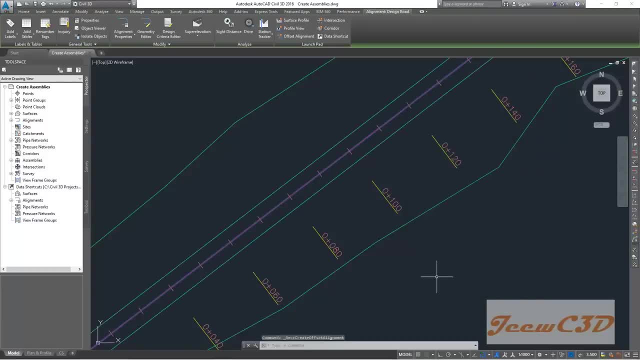 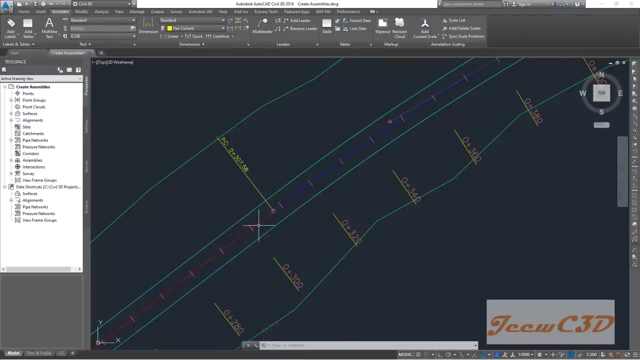 press ok. so then it will create two offset alignments at 3.5 distance from my center line. so you will see it was now created, even though this has. this has two colors- red for straight and blue for curves- but this offset alignment has only one color. 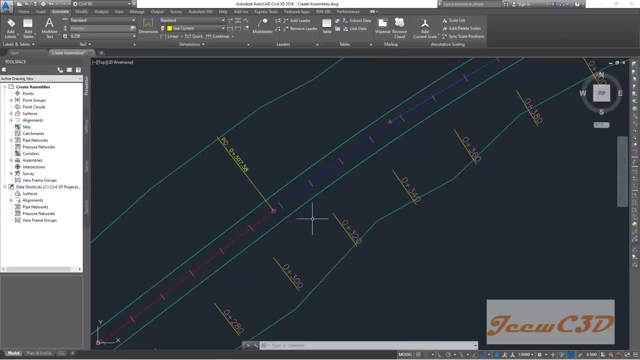 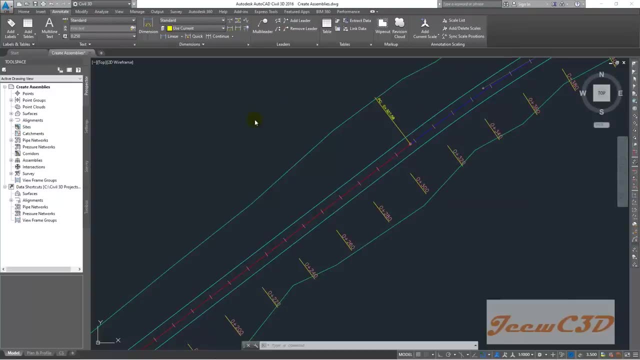 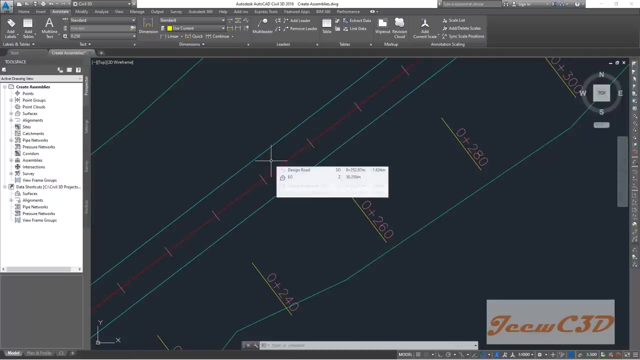 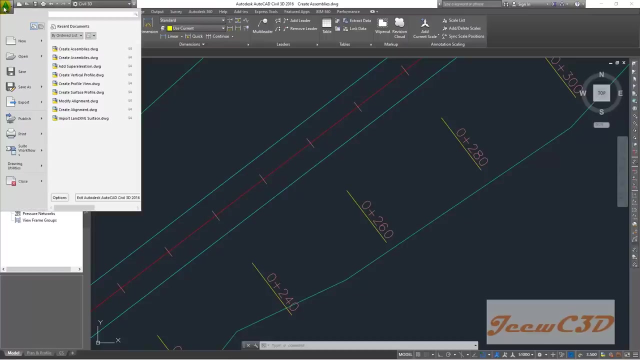 so you can see how it is set. now we are going to add the half shoulder to this offset alignment, so before doing that, I have to tell you this is we are still doing. I will rename it as actually I will save it as: create layout of road. 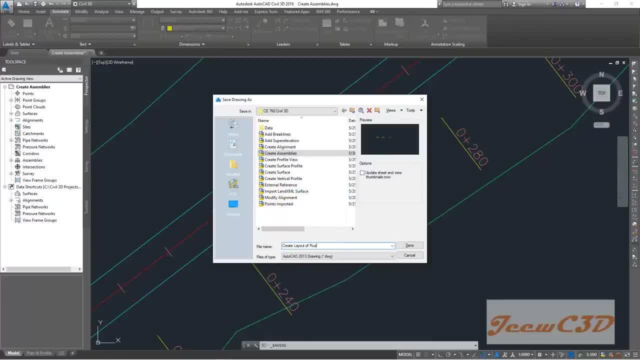 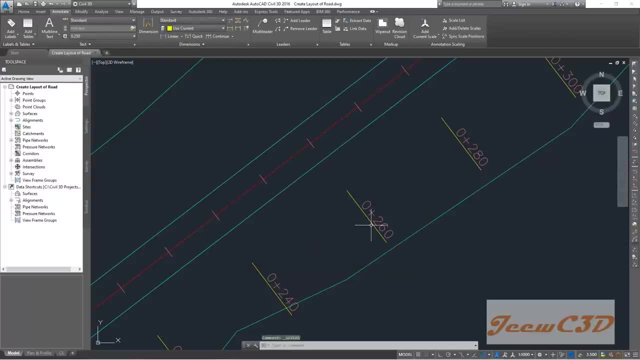 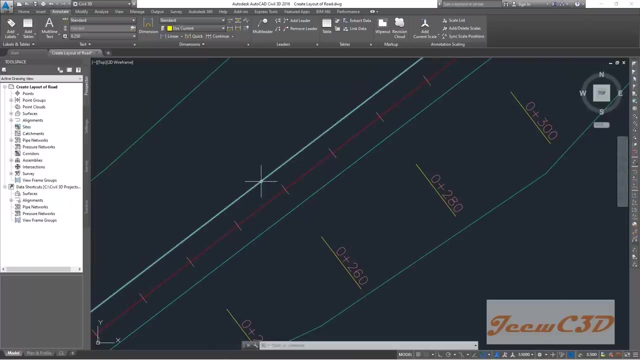 so click save. so we are going to continue this drawing with a separate name, just only different. then I am going to have the half shoulder, one meter from the plane edge. so I click a plane edge offset assembly, then I go to offset, offset alignment, then I go to. 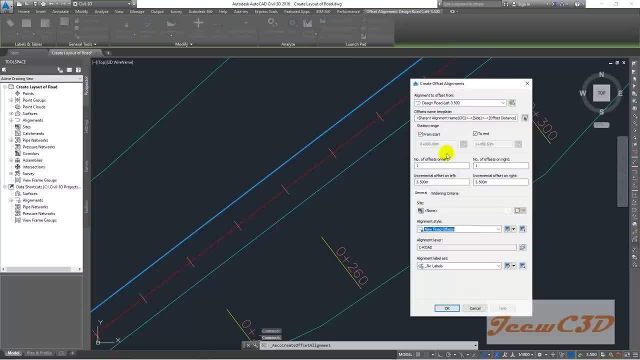 offset alignment here from the ribbon. so this time we will have the offset alignment to the left side only because if I come into the right side it is the plane inside the right edge. so I will have the left side and it is one meter and we will stick. 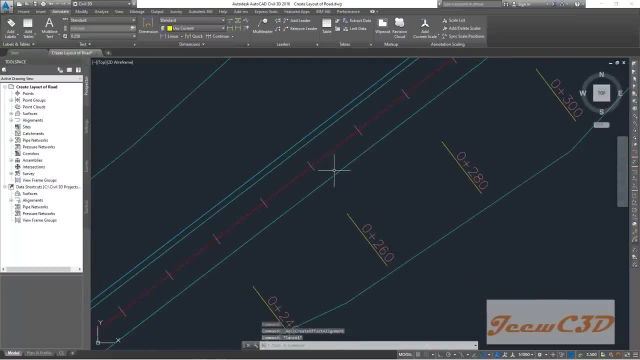 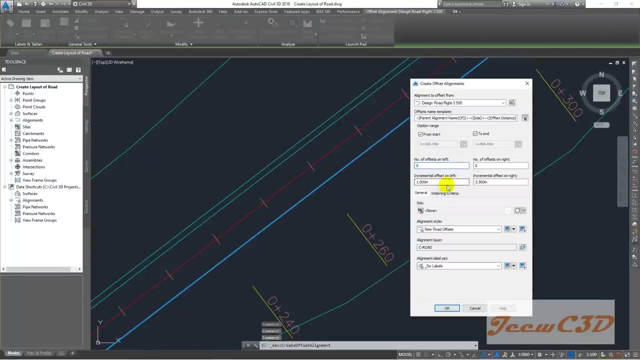 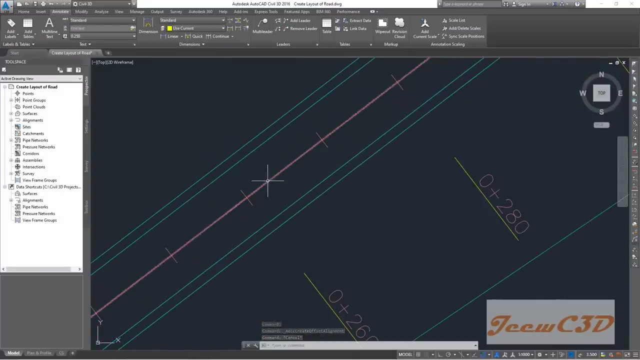 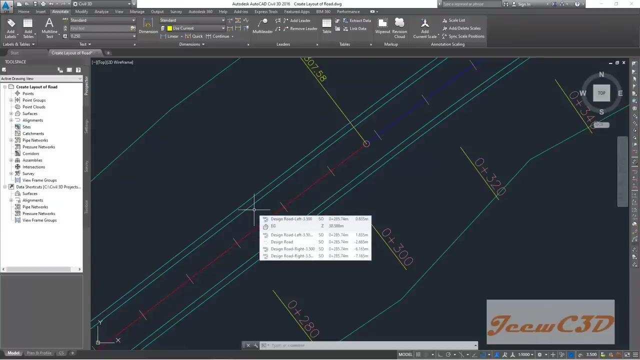 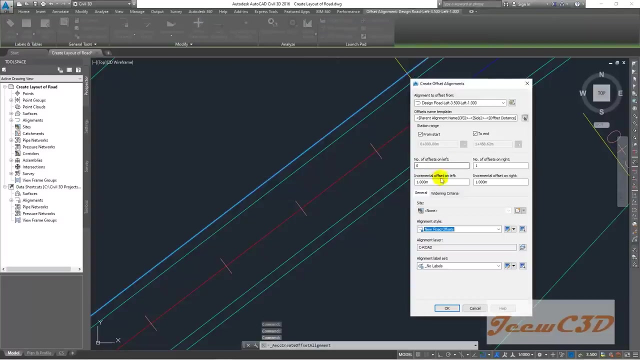 with the new road offset tile. so you get that. then for the right side also. you do that from here. then now you have two lengths and two half shoulders. then before then I have to mark the top shoulder, which is also one meter. it would be one meter. 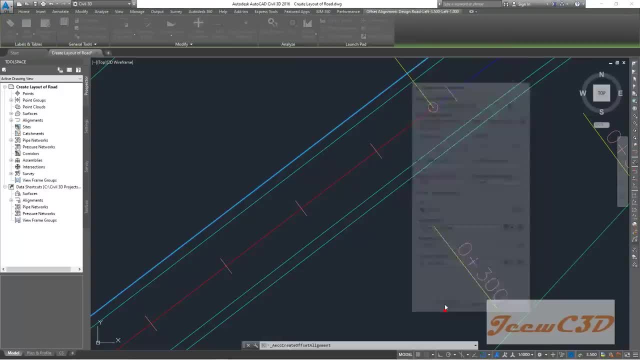 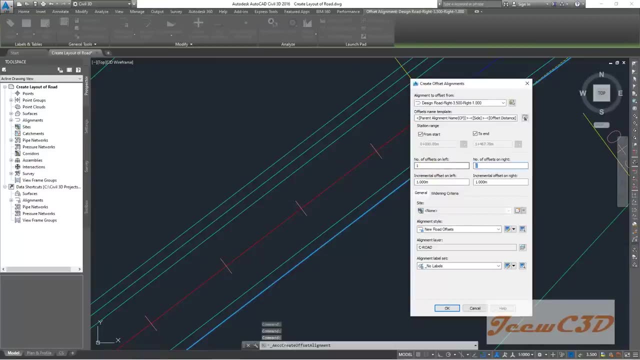 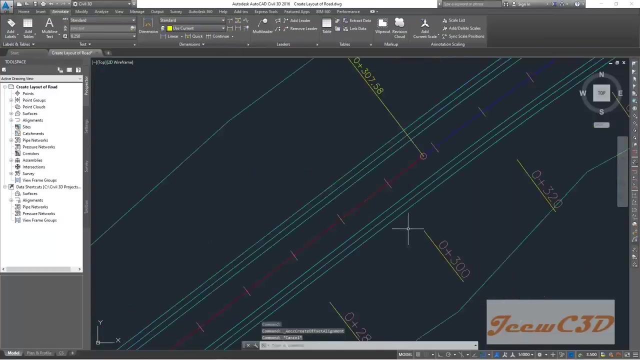 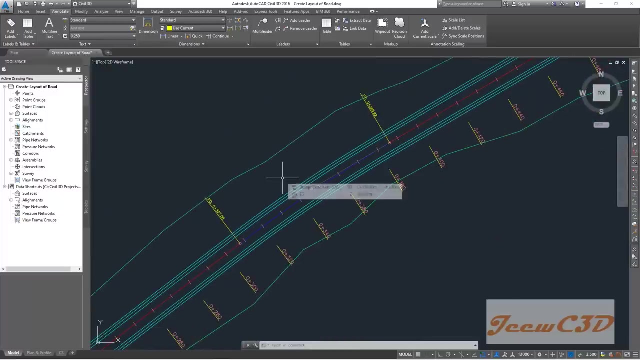 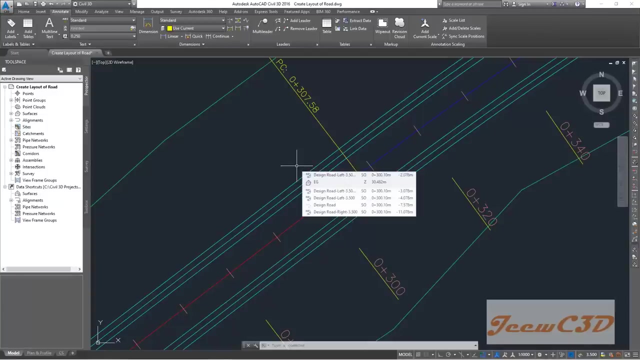 from this. so I click this one. so I'm going to the right side now and multitask one meter. so if you need, you can have separate tiles to this line here. for the moment I will stick to one, one, one. one one one two, three, four, five. 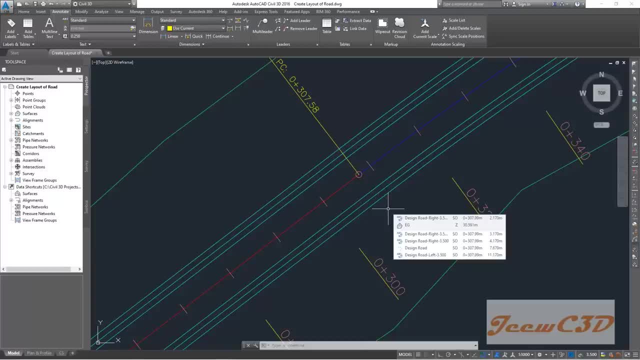 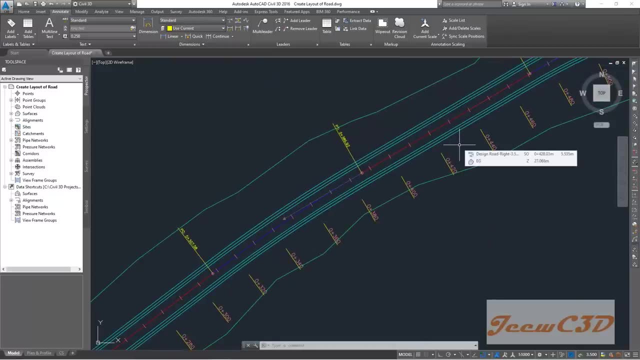 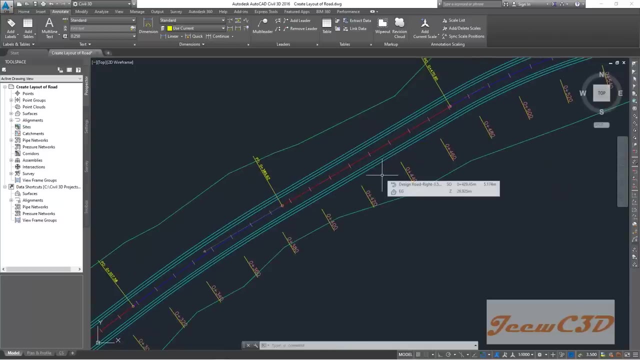 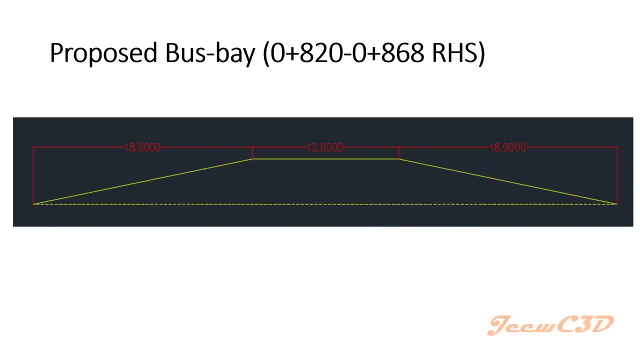 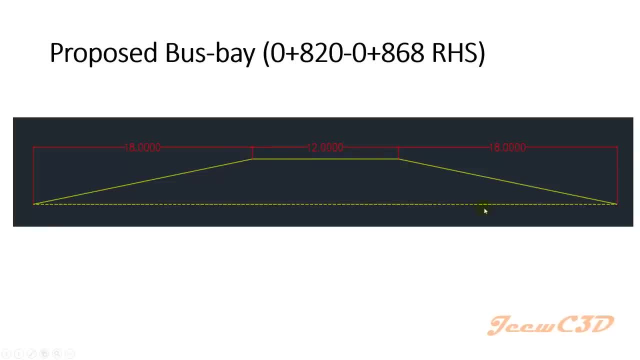 into the hard shoulder, which should be hard shoulder with 18 meter. so this height would be 3 meter. so this width should be 3 meter. so the bus day would be 3 meter in width. so altogether we have 48 meter long bus day. we have to model that inside the plane arrangement. 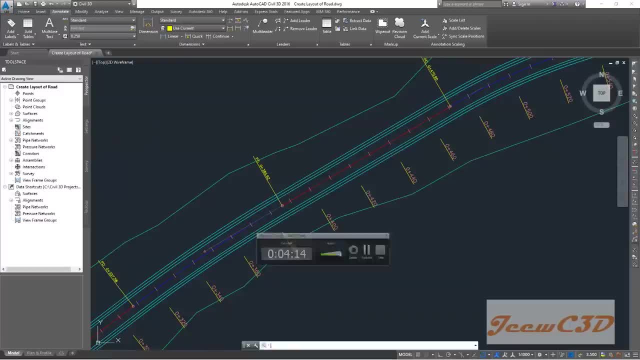 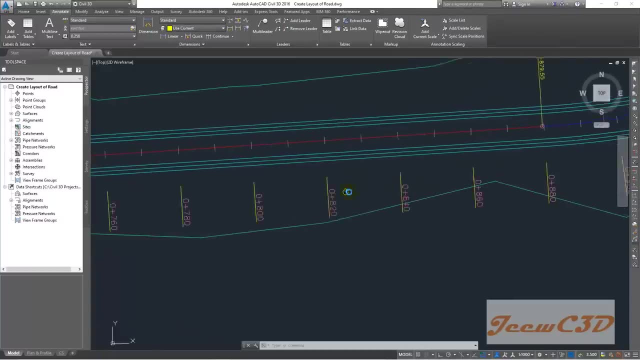 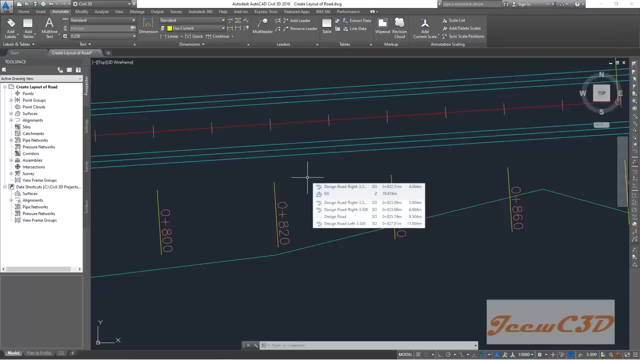 so we will see how to model that now. now we are going to find 820 point in the drawing. this is where we have 820. then what i am going to do is i am widening my hard shoulder so that i get the bus day. so this: 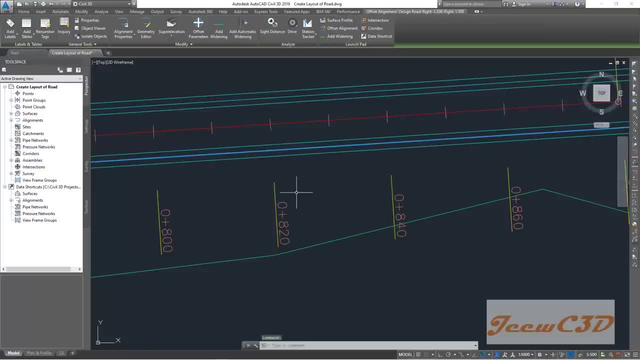 is how to do it. just click this hard shoulder before it is. the bus day is at the right side. my plane is just increasing to this height, so this height be the right height and by selecting the hard shoulder can i go and widen it. This one. 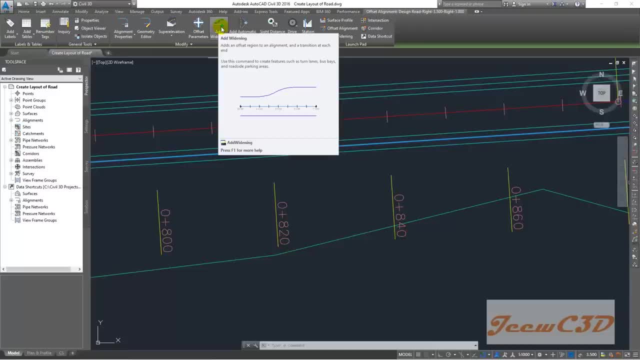 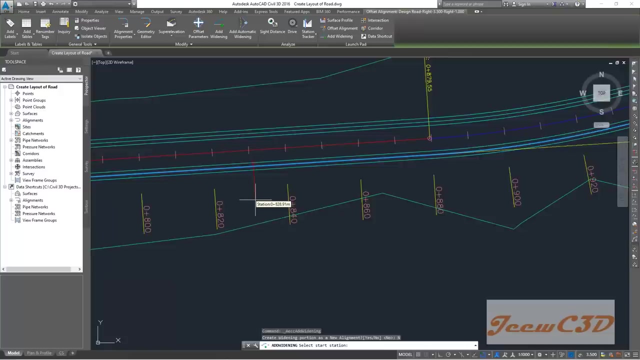 Suppose at the bus day the plane would be widened, so i will select here. then It is asking on the command line create widening portion of an alignment. It will say no. You click No. Then it is asking: is the start station? so it will be started. so the full whitening, that means the full width of the 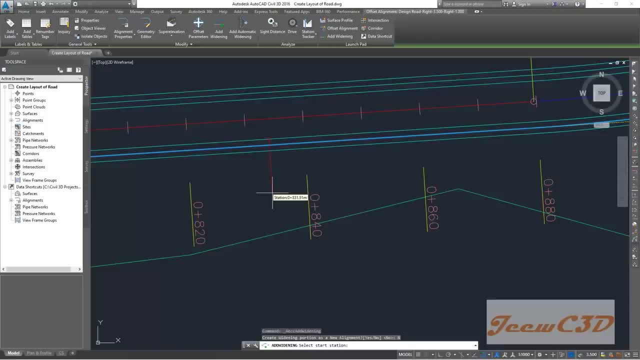 whitening will be started after 18 meters. that means from 820. after 18 meters means 838, so i type 838 here. so that is they are my full width start and then it will be end at 12 meters. that means 850. so then it is asking: what is the widening of it? 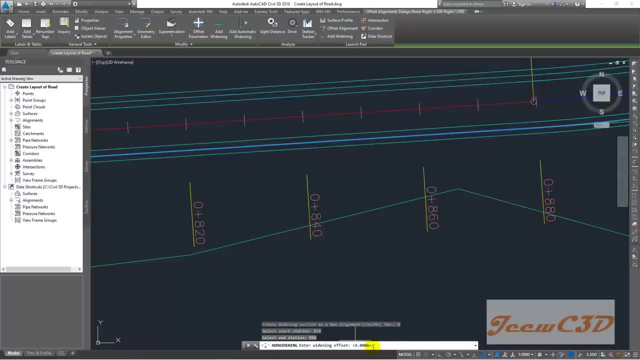 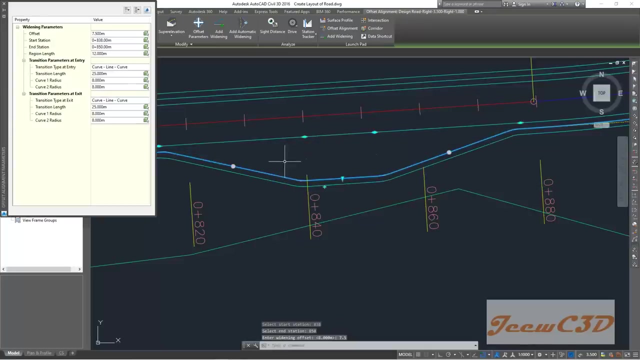 so this time the rising offset would be how much from the center line? after this point we have three points plus one, four point five. another three meter means seven point five. so we have to mark the width from the center line. so we will see how it gets widened. actually i have done some. 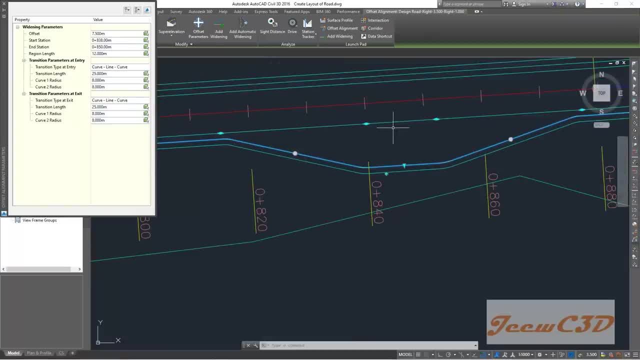 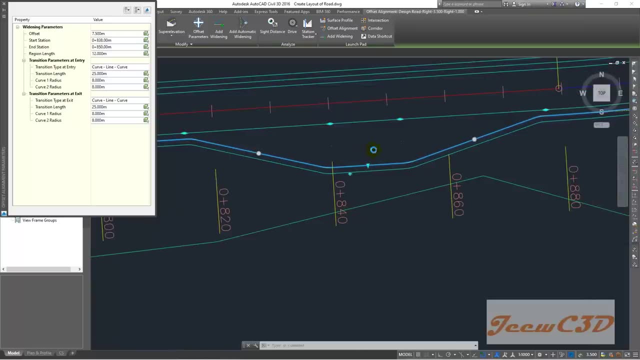 something wrong here, because it has widened from the center line, not the center line, since it has widened from the main- uh, this one- so i have to change it. this should be three meters. sorry about that, i just forgot how it went, so this should be three meters now. 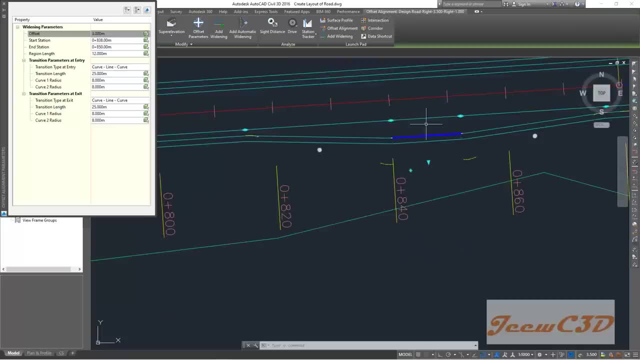 so you can see this has been widened for three meters. now i will assume we have so in the layout we have. we saw we have a linear transition of 18 meters, so i will select this entry as a linear, so i change this value here we can remember. 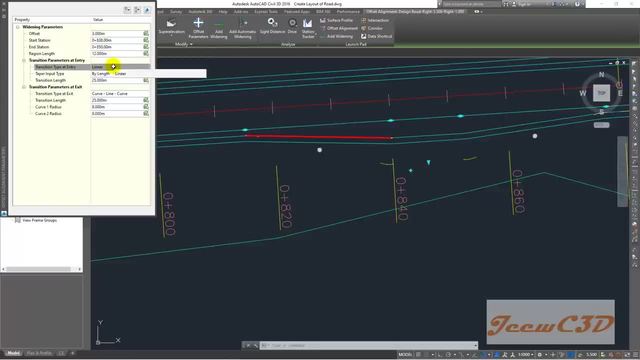 to three meters and i have a linear transition at the start and linear transition at the end and the function length would be 18 meters both sides. and you can see when you change this length my start and end stations are changing. so my start station was 838. 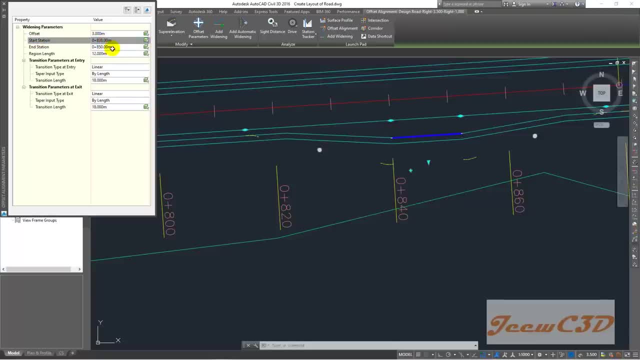 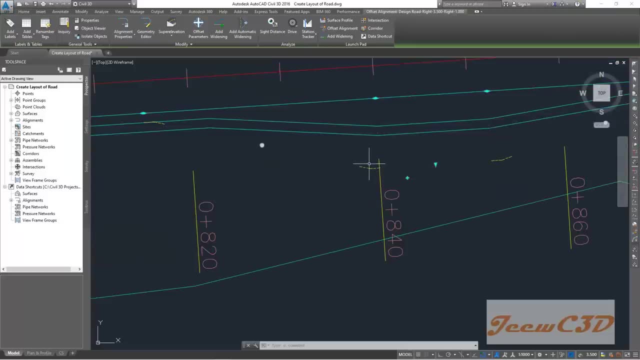 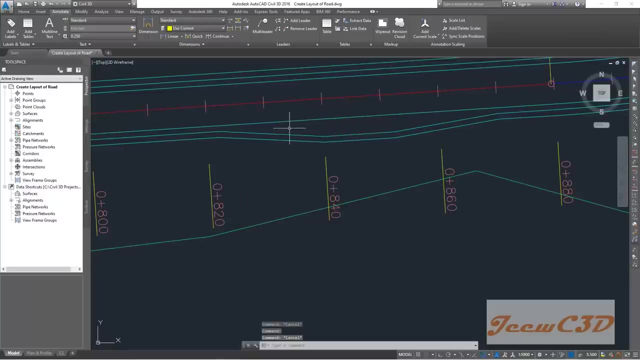 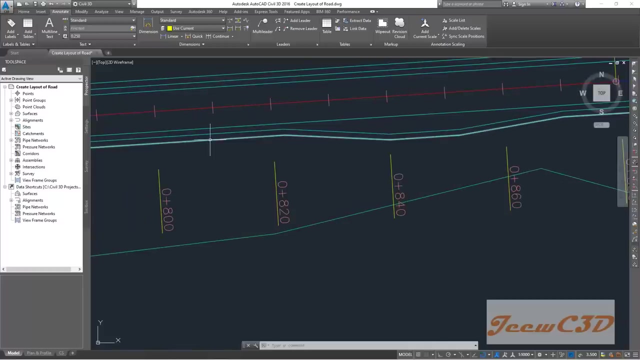 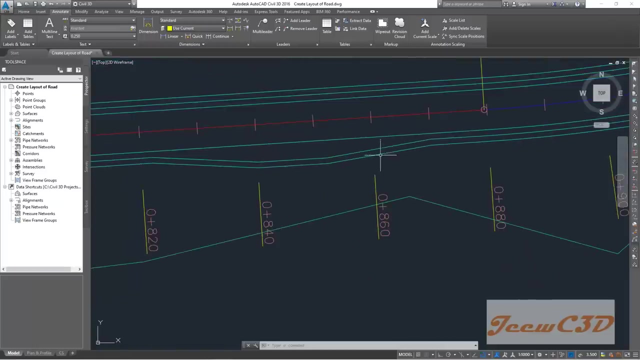 and my end station was 850.. now that data, okay, i click close. so now you can see i got k. you can see i have widened the heart shoulder. you can see, when you widen the heart shoulder, your top shoulder, which is going outside, automatically stays with the heart shoulder with a one meter gap. that is called the dynamic with the. 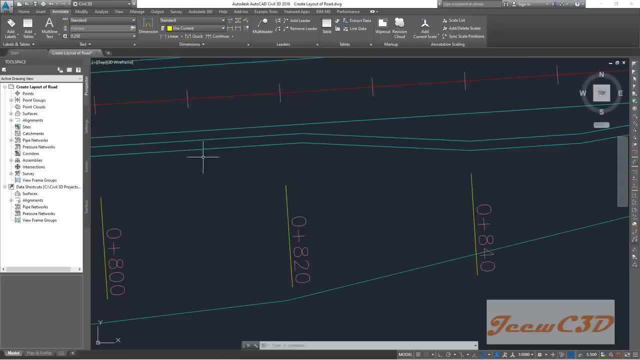 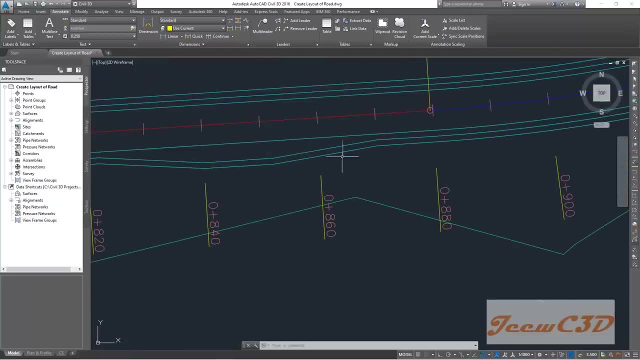 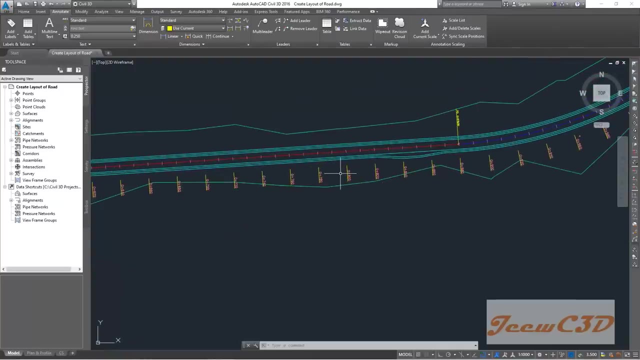 behavior of civil pd. once we updated one thing, it will automatically update the other related location also. so now we have completed creating the layout of the code. in the next video we will be going to create the corridor of the road. we have created the layout of the road up to this part. now we haven't saved the 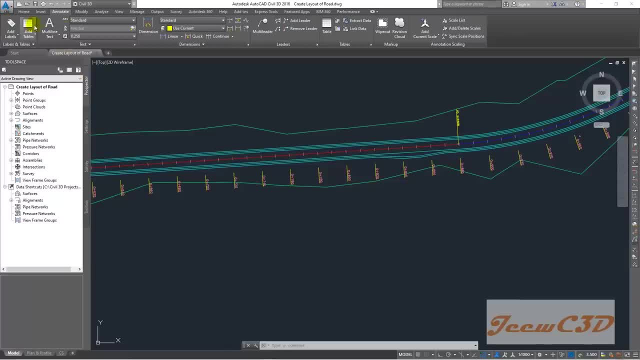 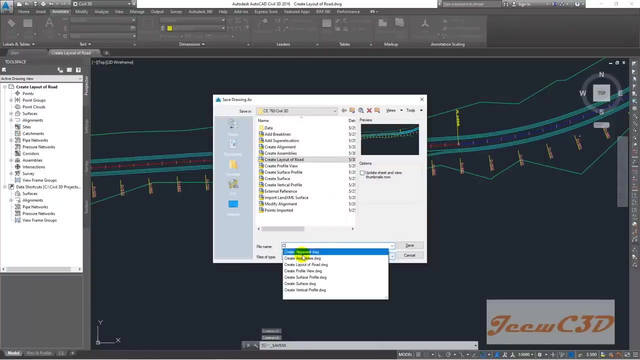 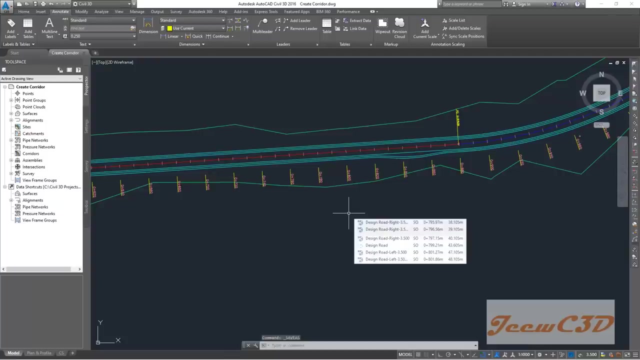 drawing i have. i will save the drawing. now i click here to save the drawing, then what i do is i will create this drawing with the save as with the name of create corridor. um, now we are going to create something called a corridor. that is the 3d model of the finished 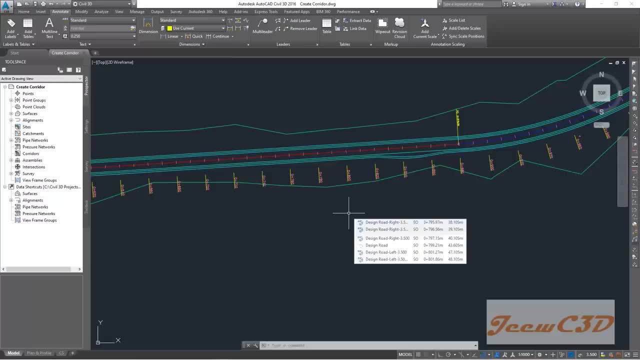 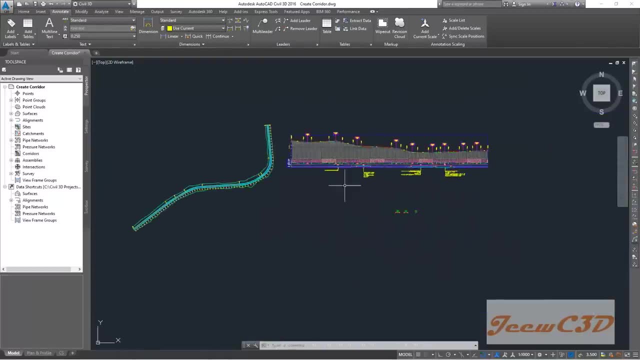 round what we are working so far. we have created the horizontal alignment here, we have created the vertical alignment here and we have created the assemblies here. so, using all these three parts, we will be creating a 3d model of the new road we are going to construct. so 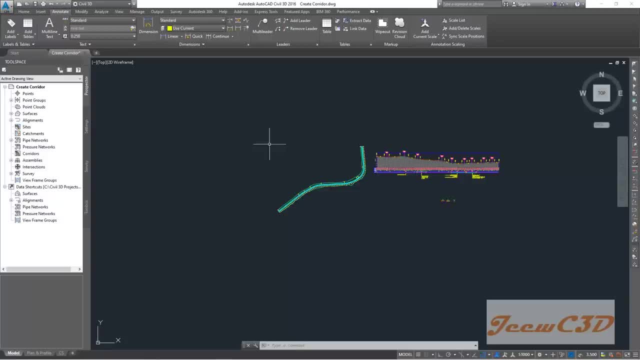 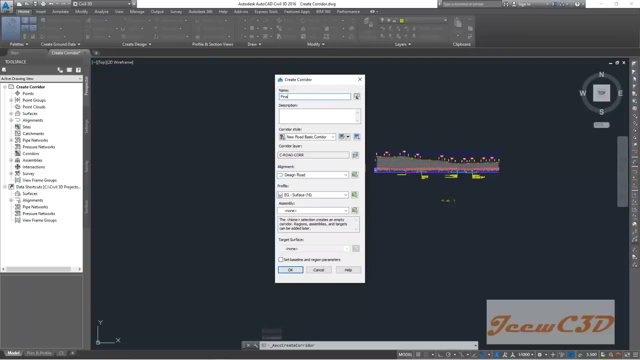 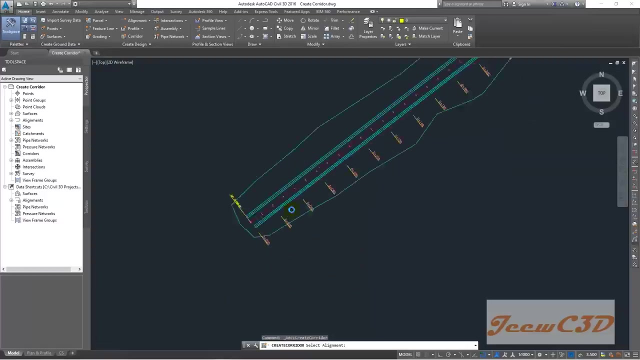 that is called creating a corridor. to do that, I go to home tab, then I go to corridor, then I name the corridor as final corridor. then my alignment would be my design road alignment, which is the alignment of the centerline. you can select the alignment from this button. also, if you have so many alignments you can use. 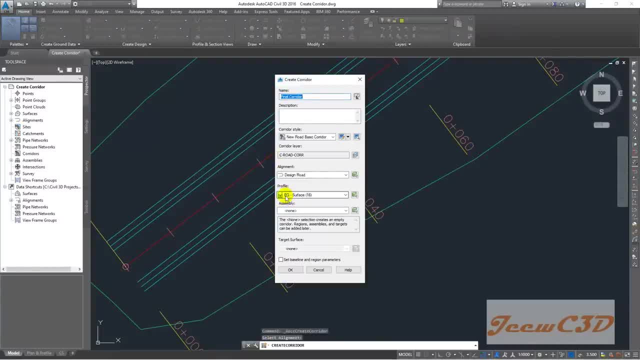 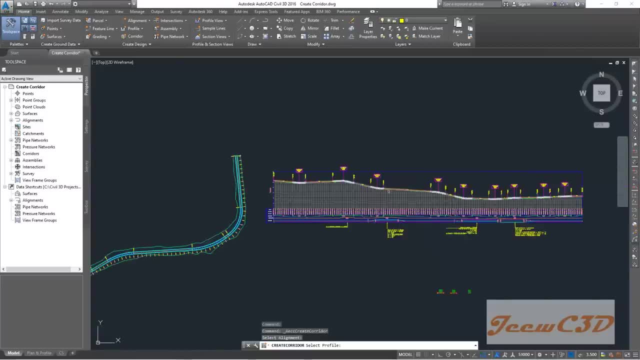 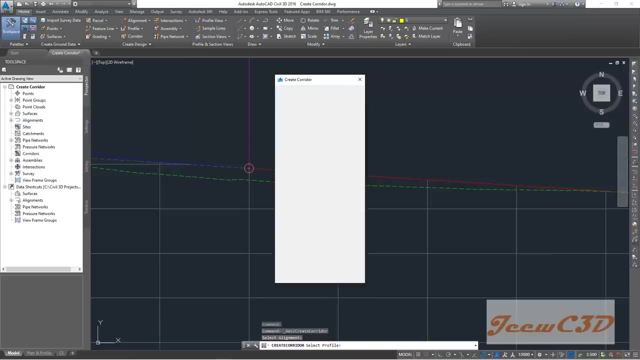 that button to select the correct alignment, and your profile would be. I will select it from here. you have to select this red and blue one. that is the design profile. so it is the finish ground. you can use this drop down to find it also. then I will create the. 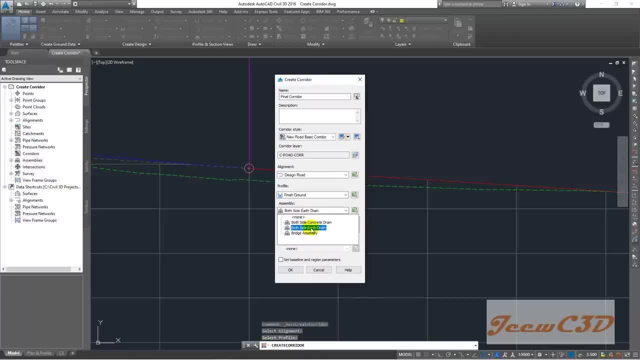 assembly. I will create the whole road for this road drain assembly and then I create the target surface as PG. so that means when we are having a field situation, a field stops at the ground. so target surface means when the field condition is applied, when the field is. 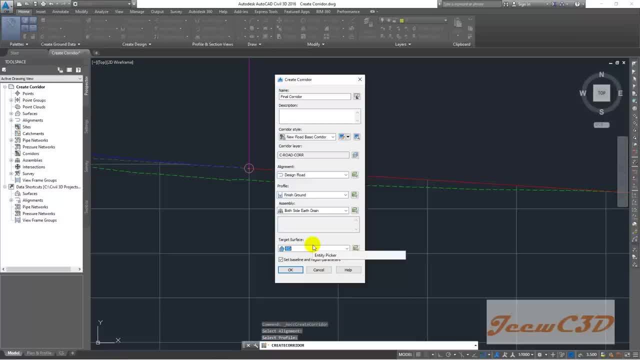 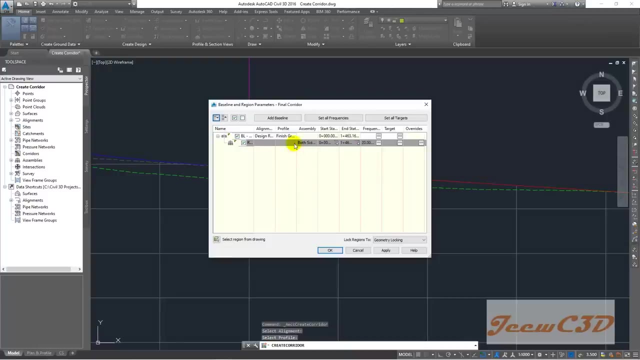 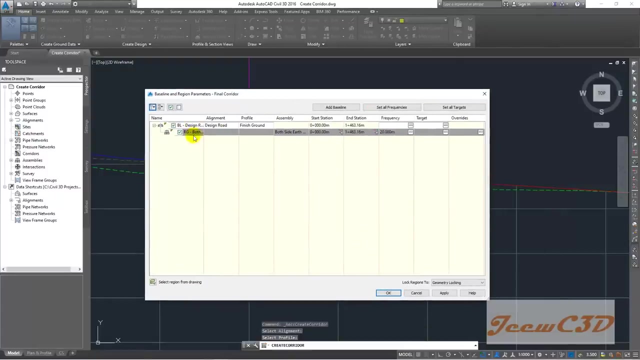 coming, it will be going down up to the existing ground. this target surface is given to touch the FG surface, existing ground for the assembly. so i click ok now. now, if i expand it a little bit more, we can please see clearly: this is the name of the corridor region. this is the alignment, this is the profile. 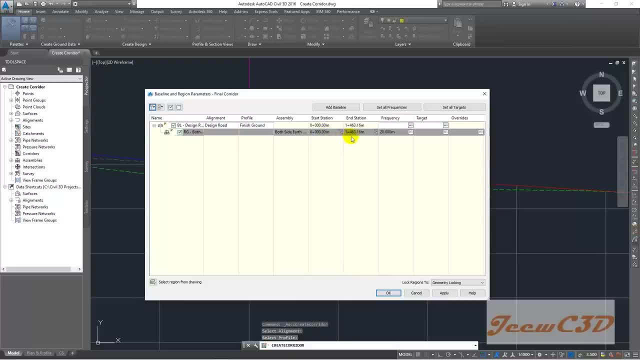 we give and this is the assembly and this is, uh, the start station and station, then the frequency. so i will give some more detail after creating the corridor. at the moment, i will click ok to create the corridor and i click rebuild to create my relation. you will see. 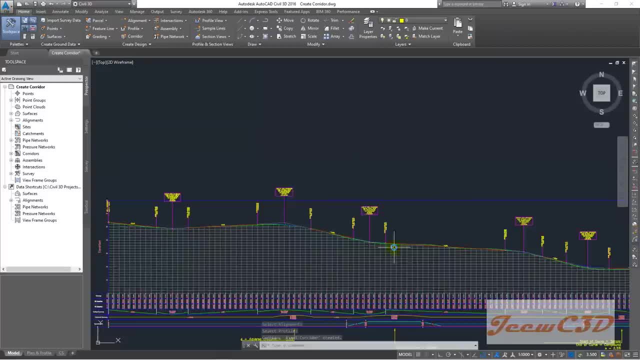 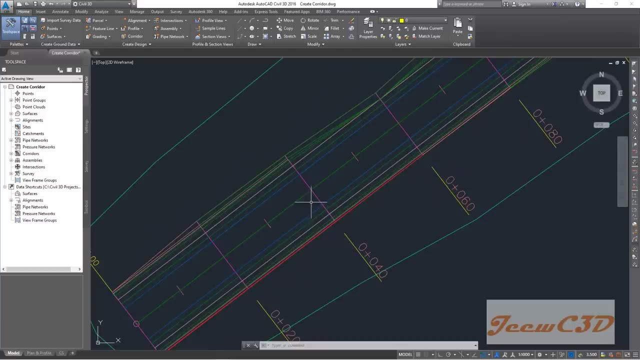 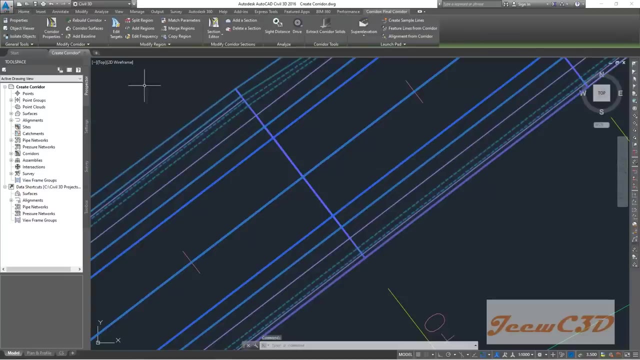 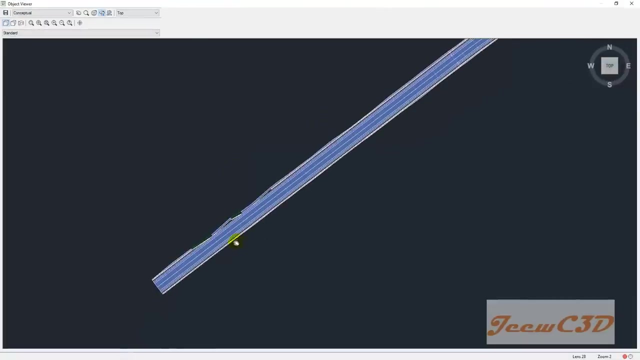 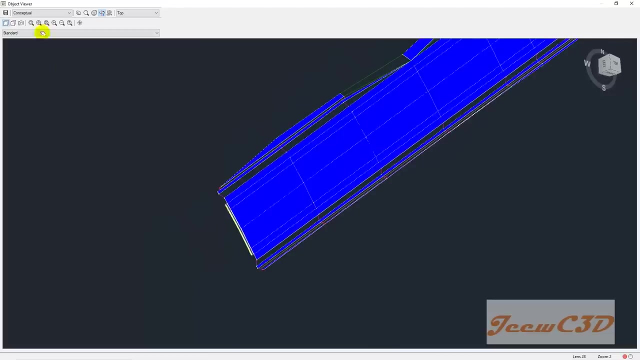 uh, something is happening at the bottom. now our corridor is created. you can see, something is created here. i will select this color line and then i go to object to be there, and i will just zoom this one a bit so that i can see the things clearly. i will change the style. 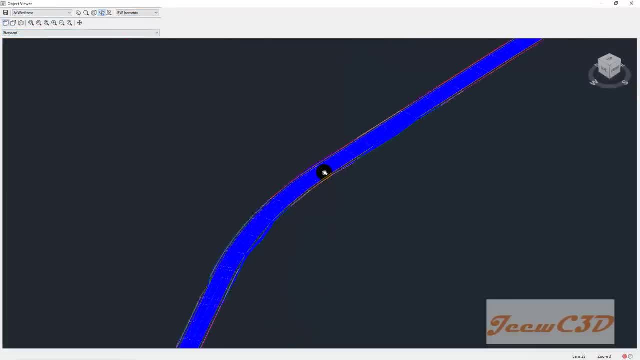 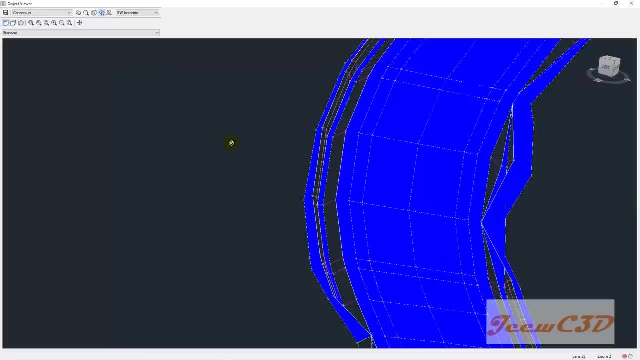 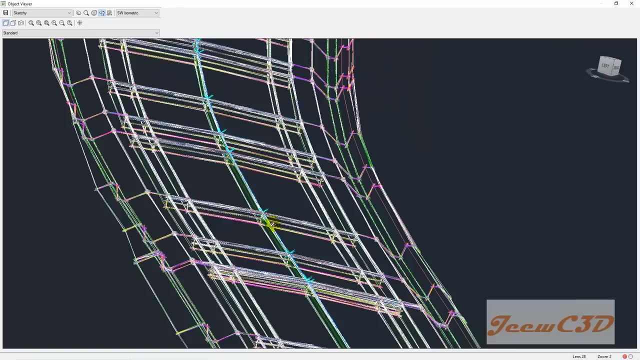 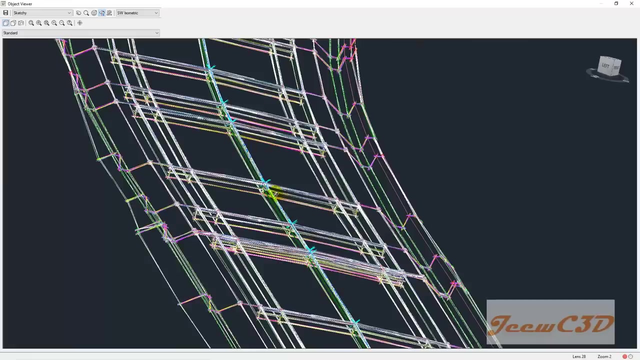 a bit. so this one you can see what has happened here in the, the. this is the おい. you can see. this one you can see. you can see what has happened here in the. here is here you have the center line of the road, so you have the profile of the road here also. 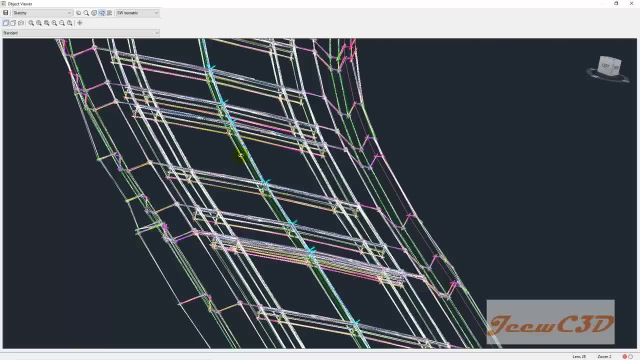 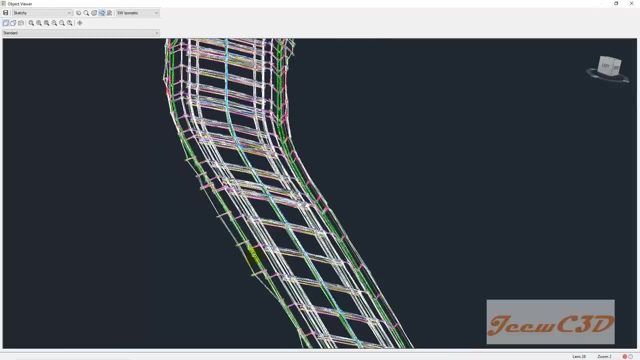 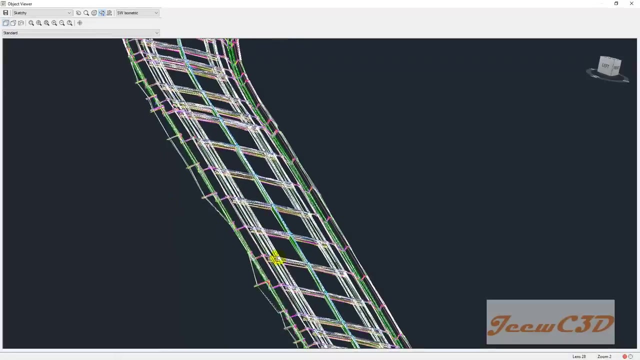 because profile is drawn over on the center line. then what we are doing is in the, in creating the corridor, you are placing those assemblies we talked about we created in the assembly creation section at the interval specified by us. so that means you can see these are at kind of 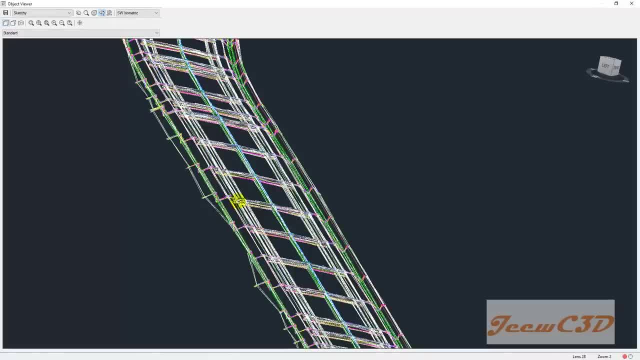 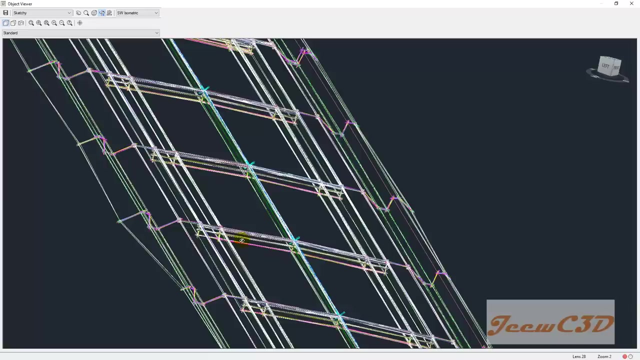 some intervals. so we are placing those first sections at the prescribed interval and then we link those first sections of the typical assemblies using lines and it will give us a really model. so that is called the corridor, so we can see so here, little more. you can see these. 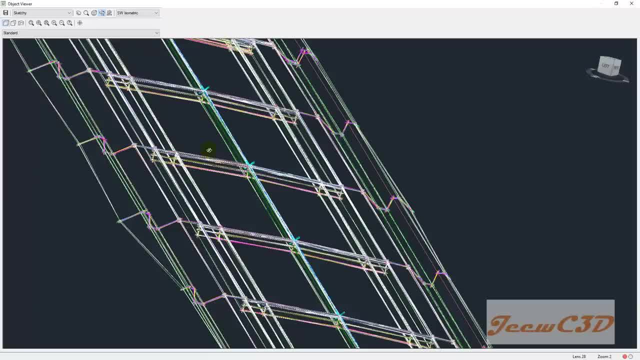 chromosomes are placed on the alignment at the interval. this interval is called the frequency of the corridor. so you can define how how much frequency you use to create the你说ido at each section. that means x mate- how much frequency you need to create each section in a moduleight. 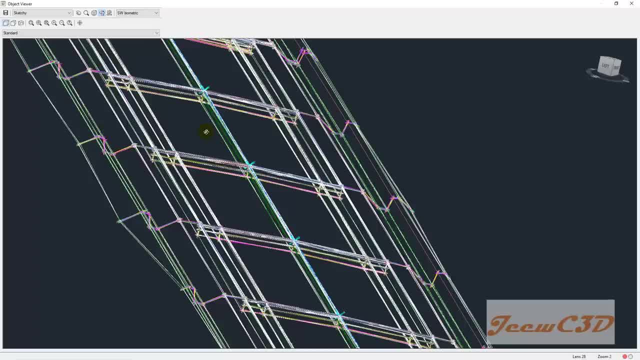 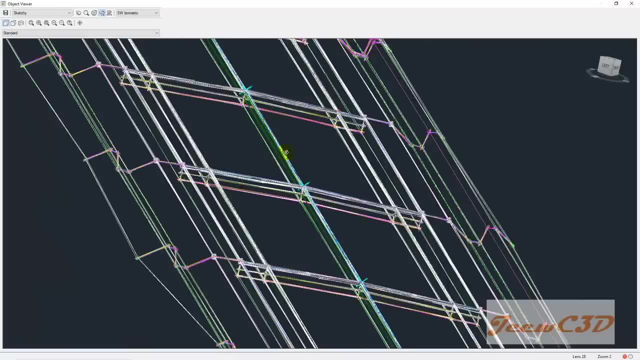 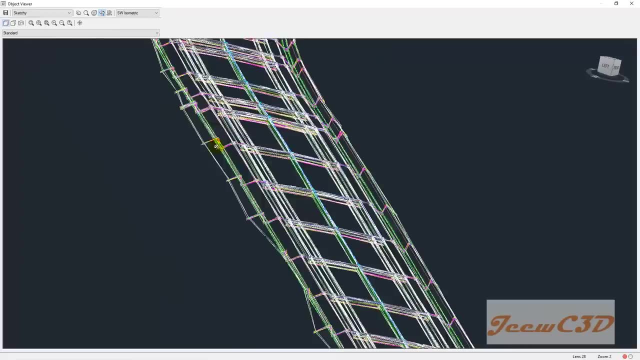 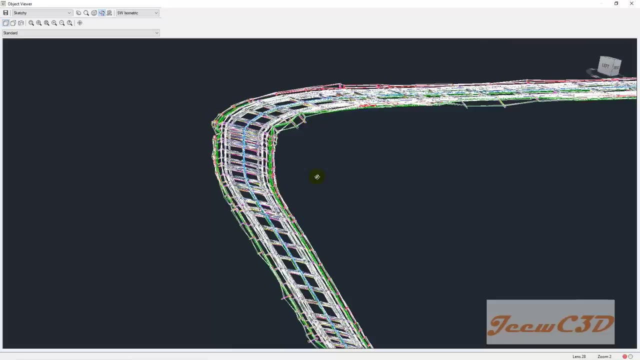 frequency, after how much frequency? so also, you can see we are connecting the top part from top part, then the middle to middle, bottom to bottom. like that we create a 3d model of the road, so that we call it the corridor of the road. so in this creation of 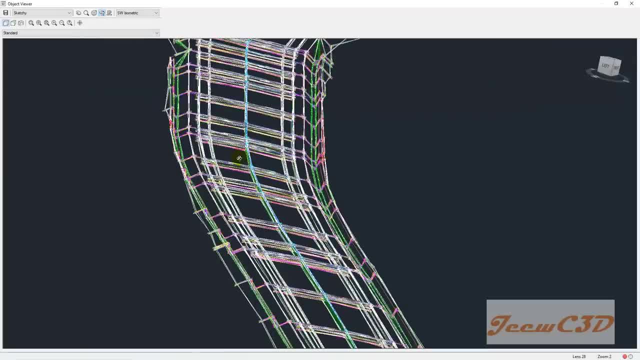 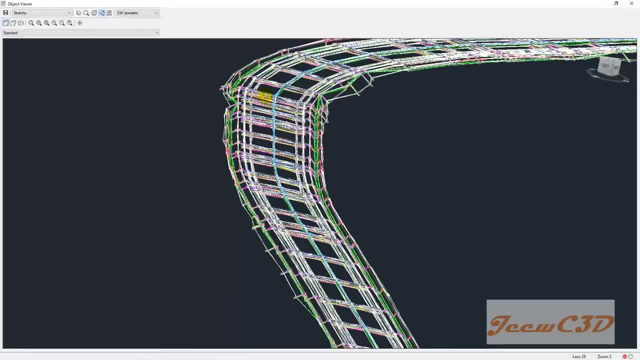 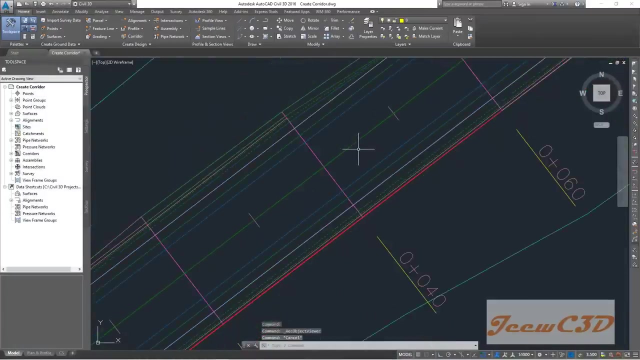 corridor. we will consider the super elevation also. you can see we have a curve here and you can see this part is super elevated to the left side because of the curve. that means this corridor is getting super elevation from the alignment also right. I will close it now. we have some idea about the creation of corridor. 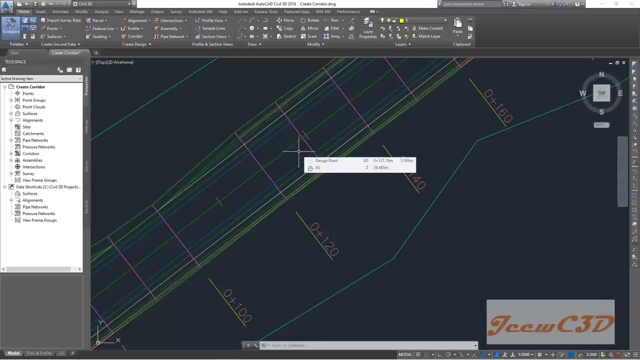 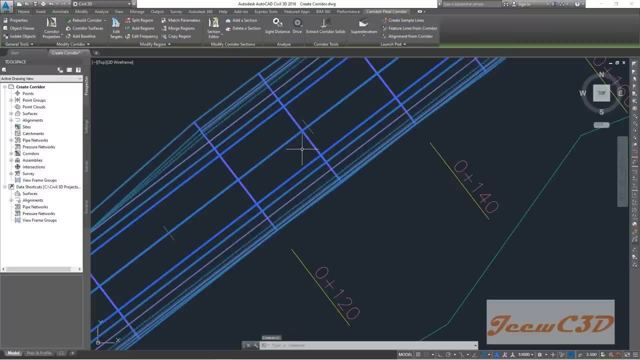 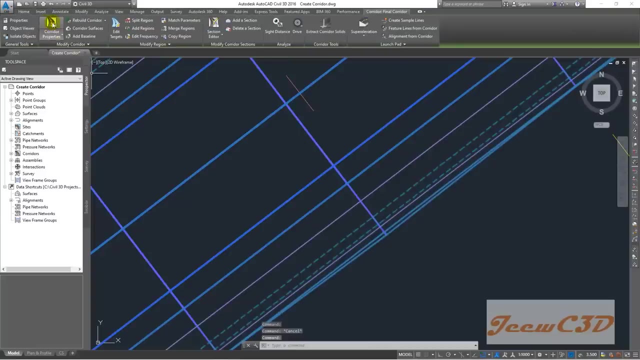 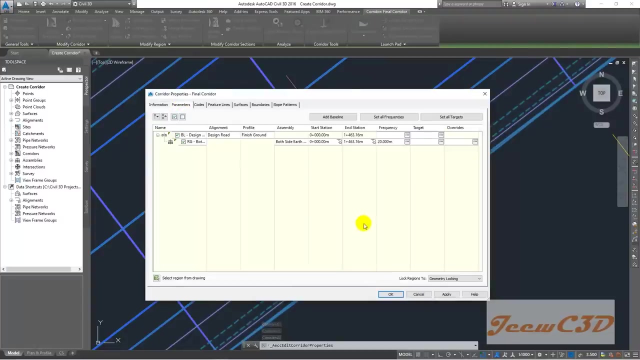 then I will explain how the frequency is applied to the corridor. to do that, I select this corridor. I will select it somewhere from here, from this magenta color line. then I go to corridor properties, then I go to parameters tab. here you can see my frequency is 20 meters. 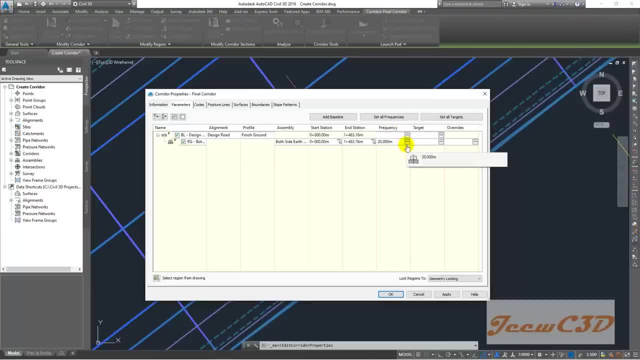 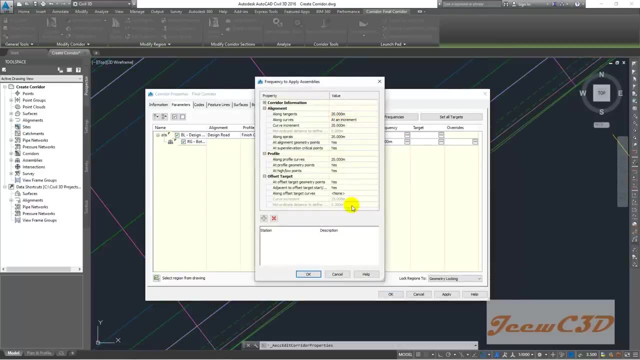 so that means I will be applying the cross sections at 20 meter intervals. so if you like to change it, you can click it here and you can click they, you can change the settings here. so at this point, along tangents we are, our sections would be placed at 20 meters. 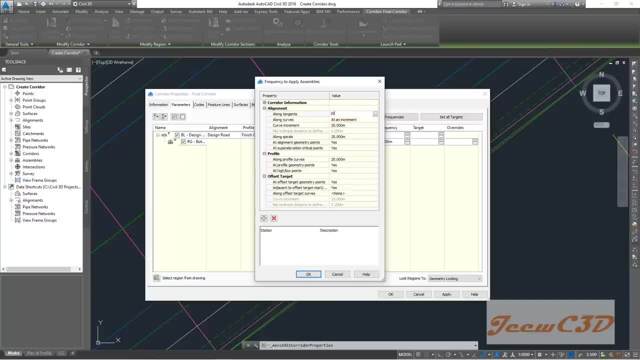 meter intervals, so we change everything at 10 meter interval and these points will say: no, this will make sure that this one for profile curves you use a larger value, like 100, so just type these values, just if you like to learn it, 3d in depth, you can learn them you. 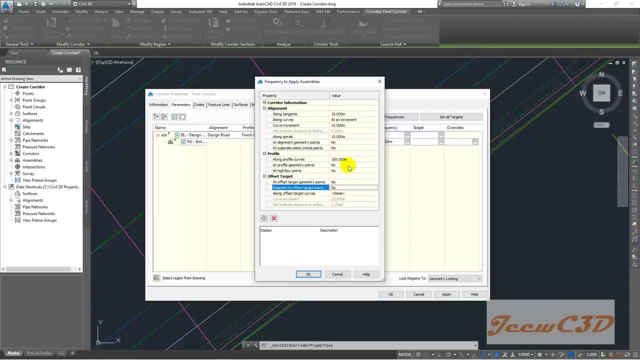 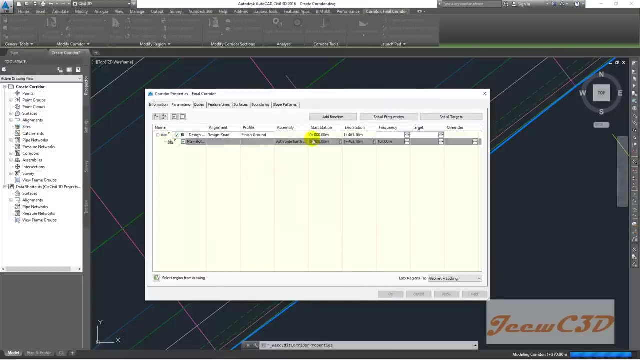 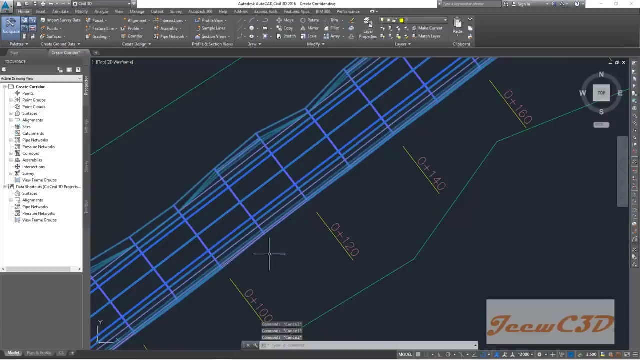 can learn why these things are changed like this in these windows. but for the moment this: it is okay to have these values like this. you might click ok again and create the corridor. you will see more frequency lines will be displayed. so if you want to see the at 10 meter intervals, then click on this and you will see a line. 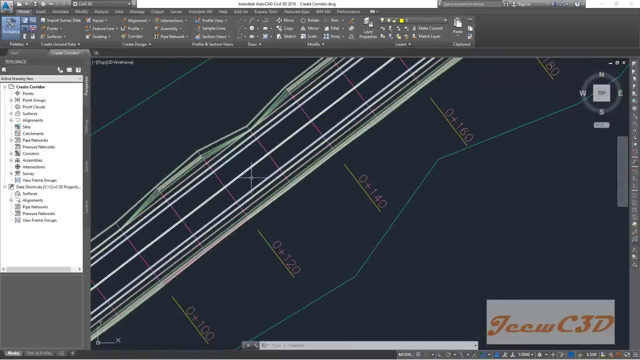 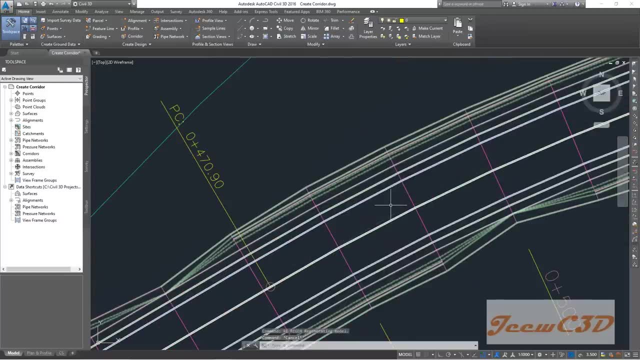 is already appearing here, so now they are appearing at 10 meter intervals. here you can see, in between this, magenta color lines are the frequency lines. you can see there at 10 meter intervals. now every have initially been at 20 meter intervals, so that is how you create. 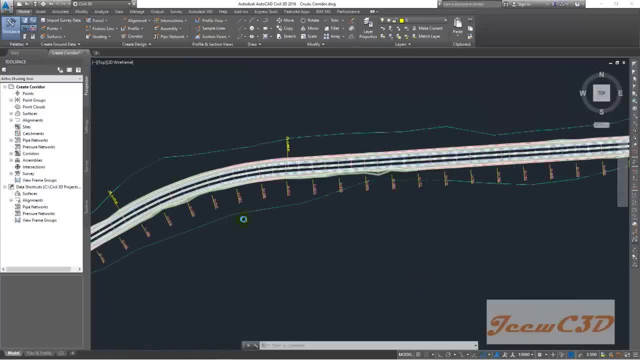 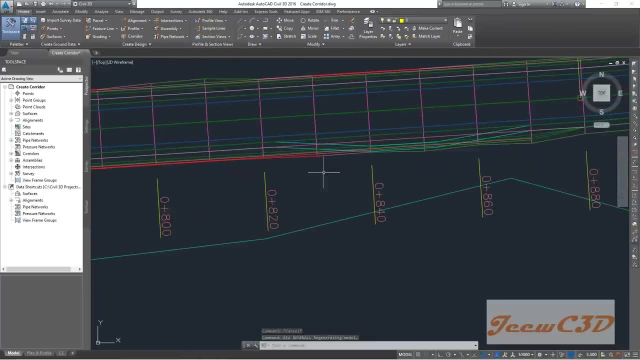 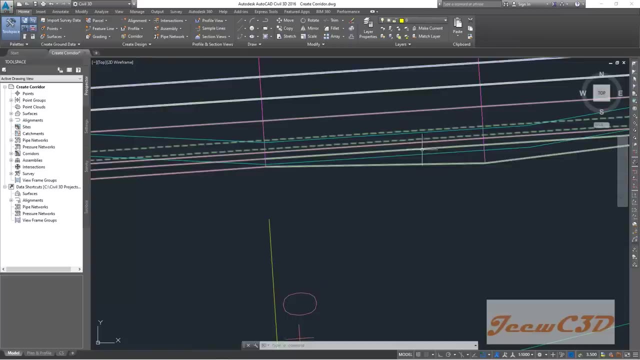 the corridor, but still there are something you can change if you want something like that. so that is how you create the corridor, but still there are something you can change to be modified, because at 820 I said we have a bus bay, so our window should be modified like this. currently it is not modified, because you can see. 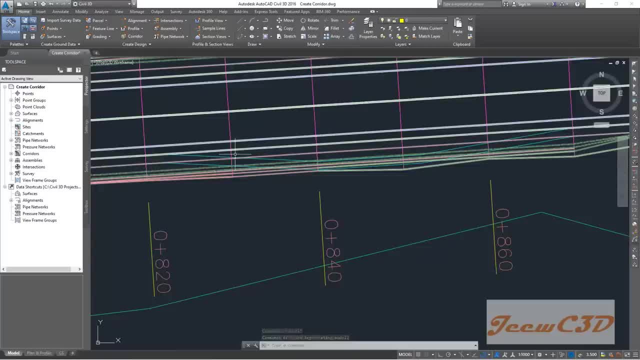 this area. you don't have actually this area. you only have the road up to 4.5 and this shock shoulder. but it should be widening up to this point, so it is correctly widened. this green color line should come up to this point and this gentle color line. this should come up to this point, so currently it is not matched. 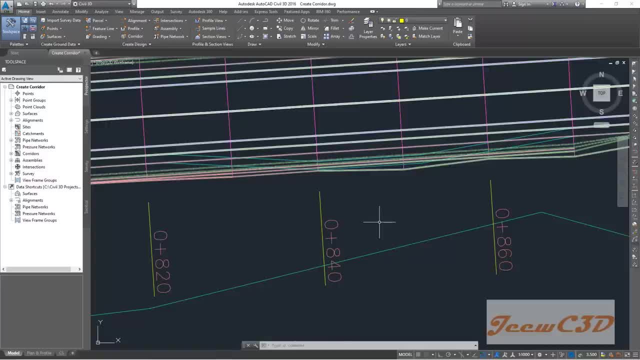 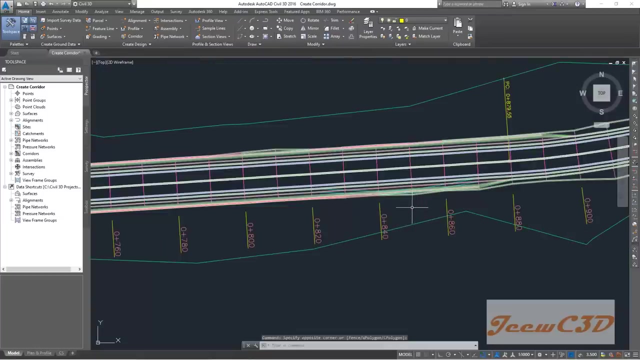 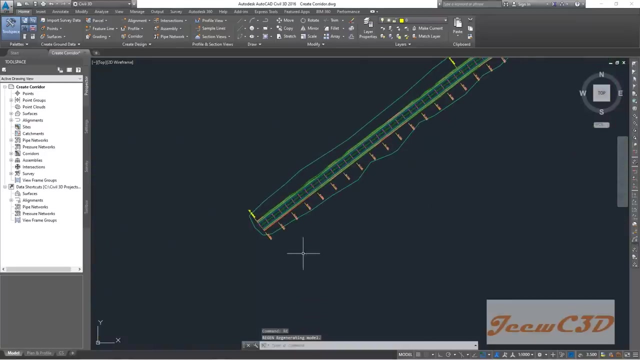 so in the next video we will be going to match these things to the correct targets. we call it target mapping. before that, we will save this drawing in this video. what we are going to do is we are going to set these targets or we are telling CV3D to target the alignments, to create the corridor. that means. 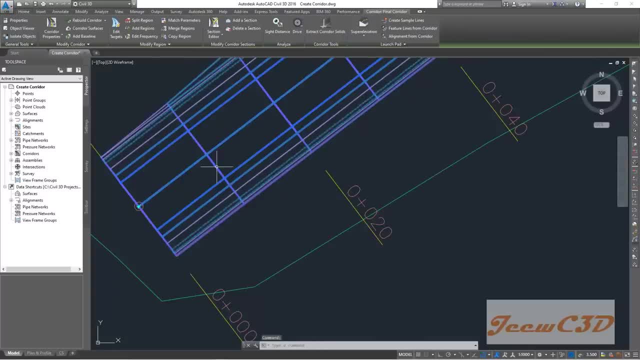 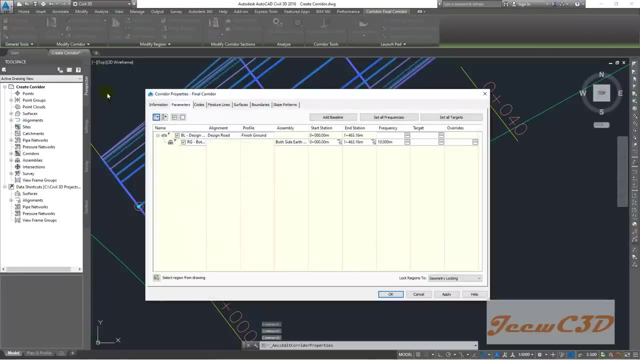 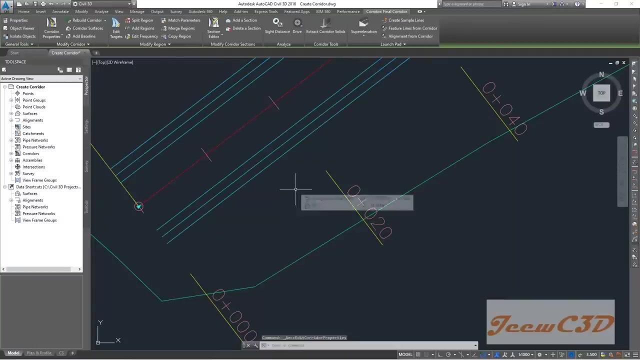 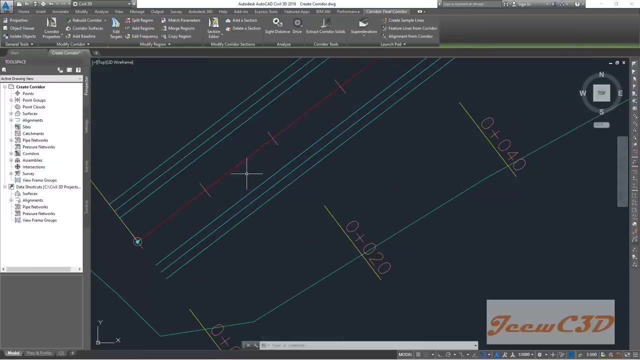 like this: I will turn off this Corridor function. want to do that, select this corridor properties and from here I click this button to turn off the corridor and click the key and we will get the corridor. so your corridor will be turned off now by target. nothing. what we are doing is we are telling CD3D to get these targets. so if I 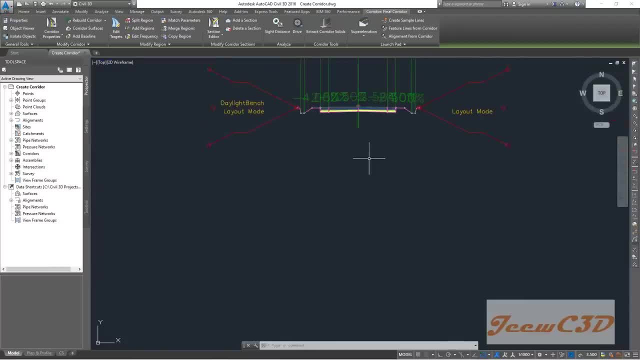 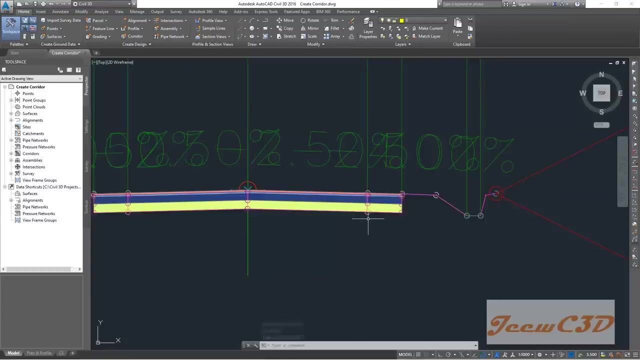 go to my assembly. this is the assembly we used to create the corridor, this one that is both side joining. so first I have my clear net, then I have my half shoulder, then I have my half shoulder. so if I select this one, this should be right lane, this should be right half shoulder. 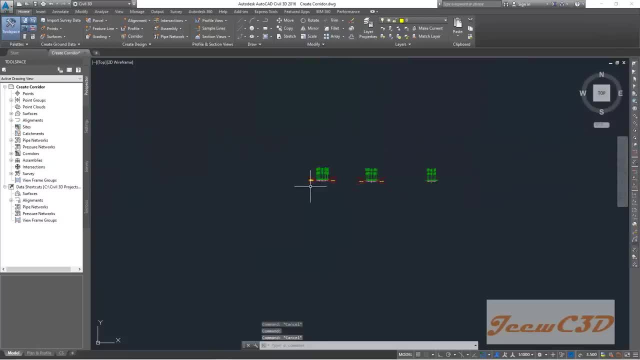 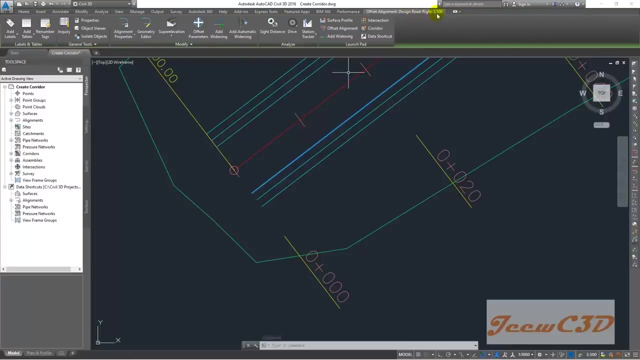 and this should be right half shoulder. so what I'm going to tell you: cave, CDTHC, right lane should catch this, offset that. yet design road right side. then hard shoulder should catch this one and the soft shoulder should catch this one. so this is how to do it. now, since my corridor is turned off, I can turn it on by clicking. 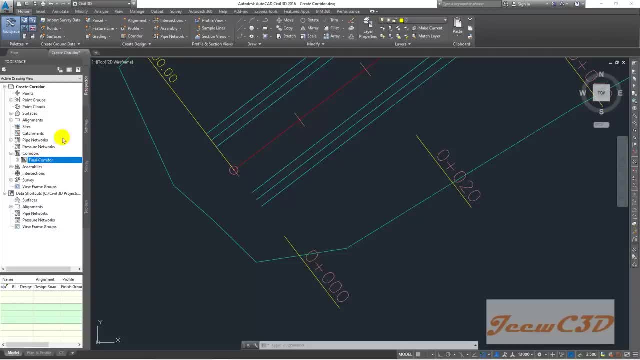 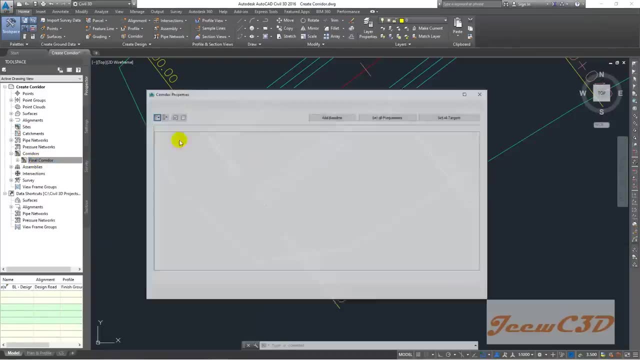 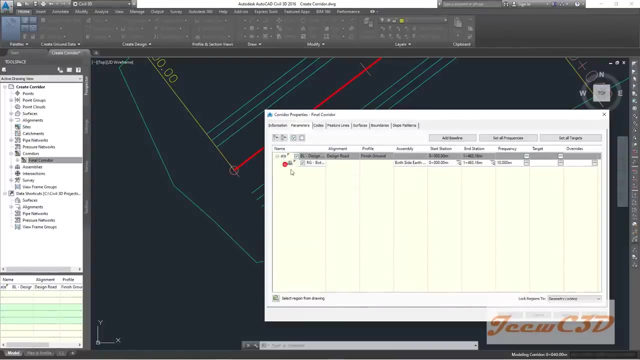 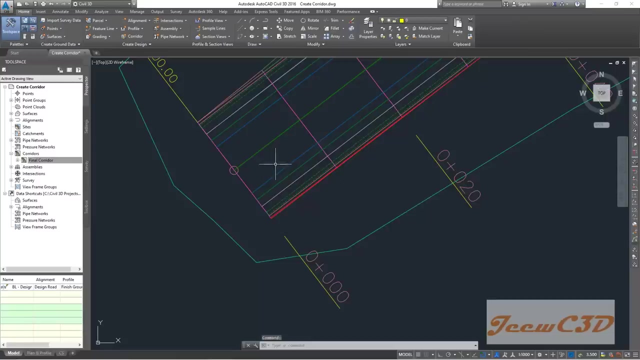 here in my prospector I go to corridors. my corridor name is final corridor. I right click and go to properties. then I can turn on my corridor. this is how I turn on the corridor. now you can see, currently these are matched because there is no width changes at this point. but at this 820 location there is a width change, so this is not. 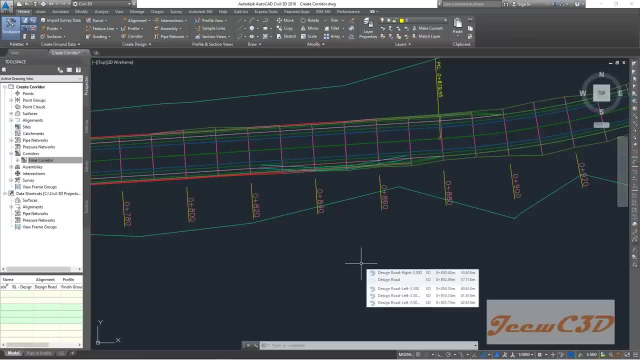 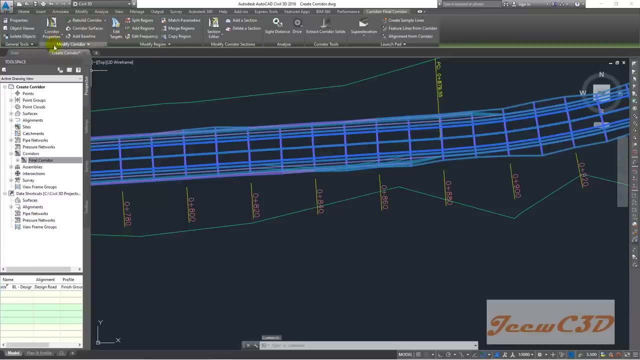 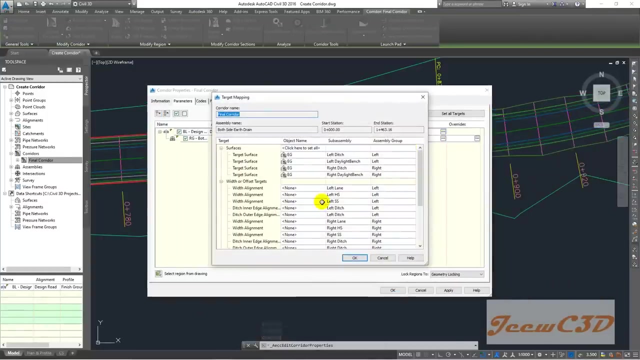 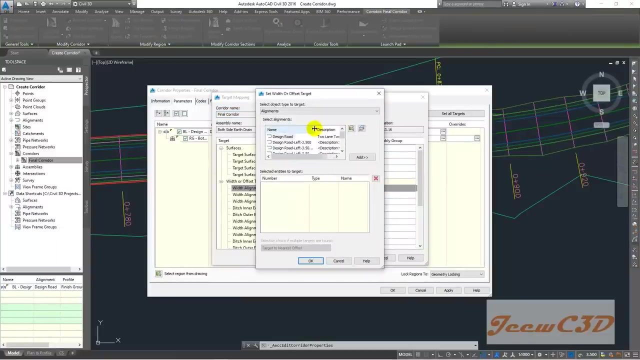 matching. so what I am going to do is I tell cellulcd to catch each alignment, to target the lines of the assembly. so I click this corridor and go to corridor properties. here I go to target and I tell my left plane to select the line. I can see that the flag has been идon the way I can. Now I am going to change the. 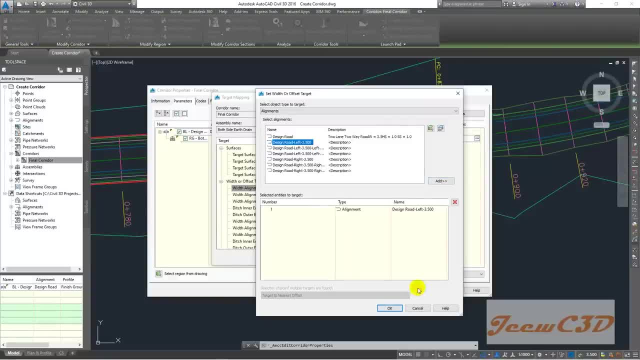 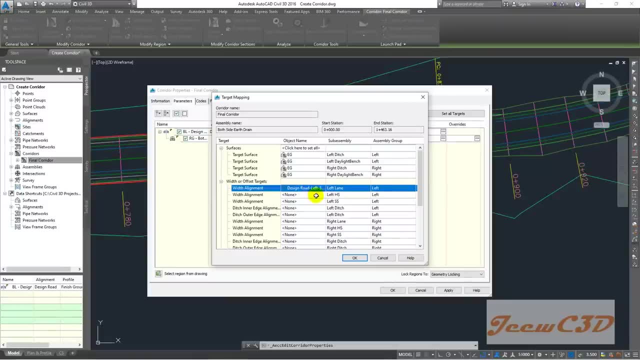 right axis of the fold by selecting the edge of the fold line actions, usually for u to flip out, which is 0.38 at this point, unbelievable. Now I am going to do right distance. shall I go to normal approach and select left ago, 0.3.. 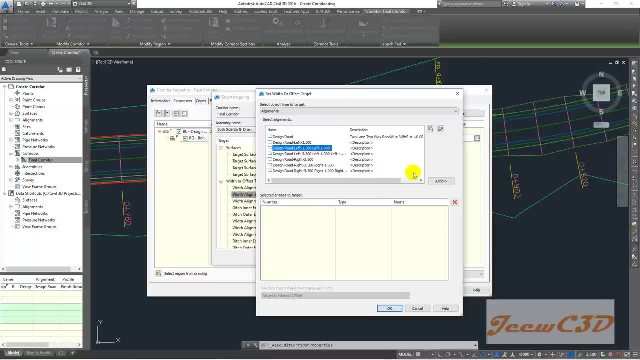 which is now 0.38. yes, minus 3.5, ok, minus three point five. hoof depth plus three point five. I select one, then I click here to edit, click OK, and my sub-shoulder will be this one and for the right side, my right leg should be height 3.5 and right half shoulder will be this one. 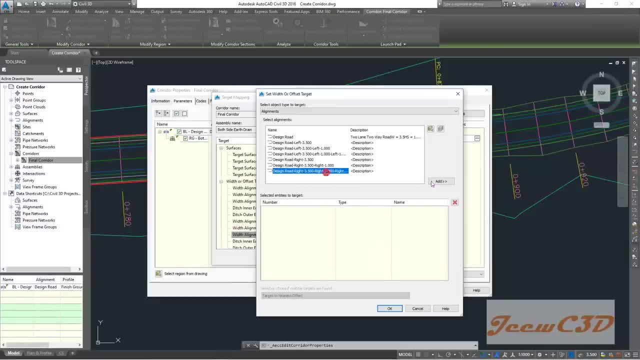 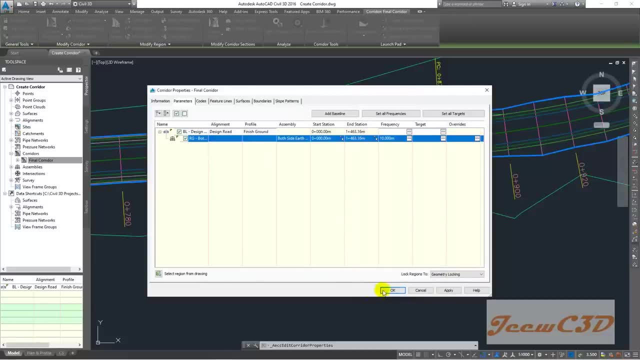 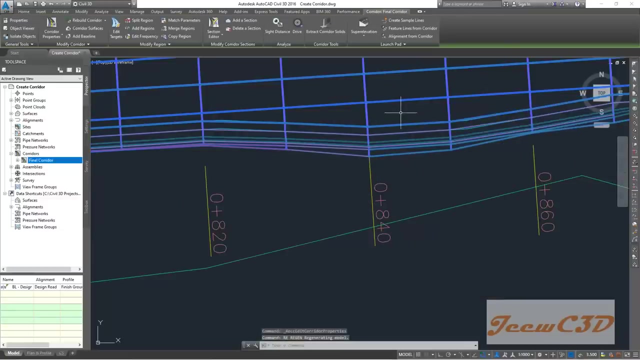 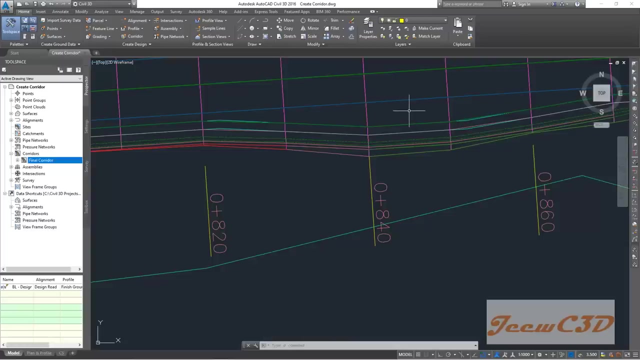 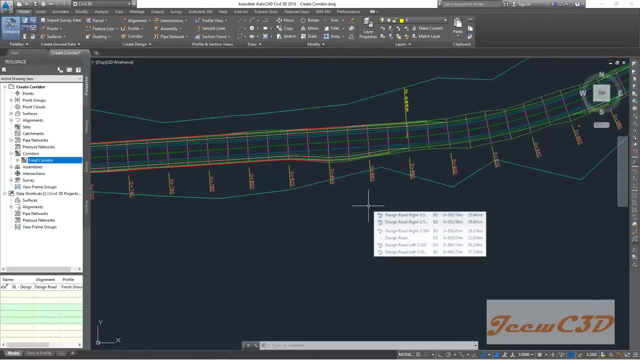 and my sub-shoulder will be this one. so I have set all the targets. then I click on OK. my corridor will be rebuilt. now you can see at this location, all these are now clearly matched. so that is what we done by target mapping. we call it target mapping, but up to this. 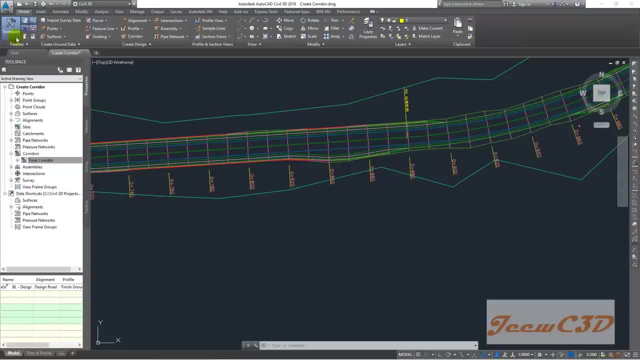 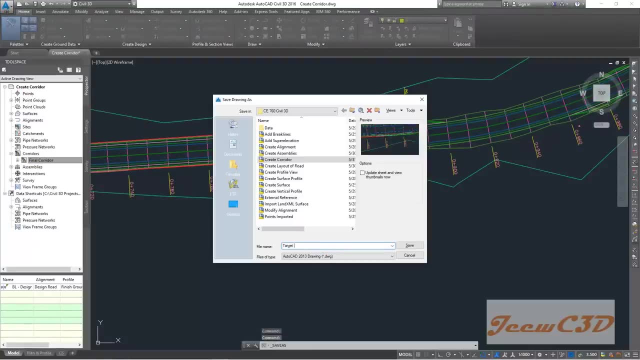 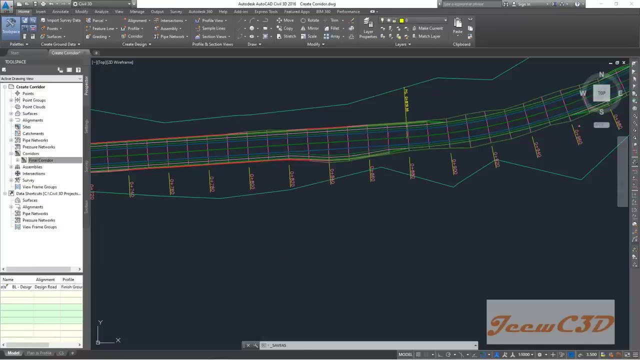 point. we haven't save the drawing, so I will save this drawing as target mapping. click save. so up to this point we have create the corridor with Part, so the part mapping session is now over. next another see how to split the per Delta cause. we can also regions inside this courage. 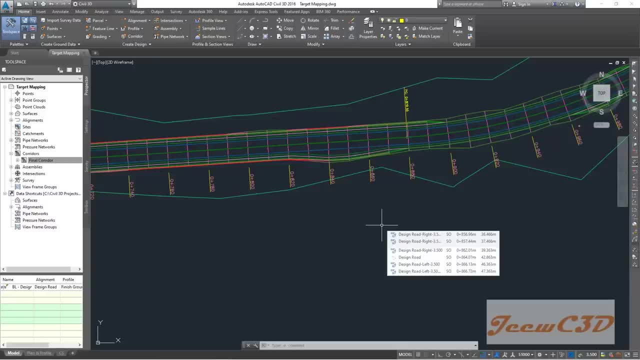 the force. you can remember, I, in the start of this section, I told you your regions are this bold site. then we have this region, then we have concrete points from this region, then we have bridge in this region likewise. So in the next section we will do something called 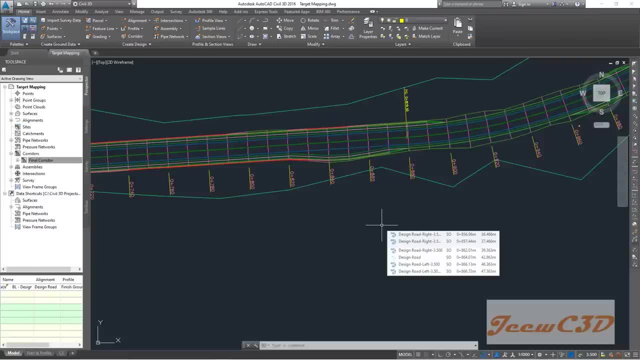 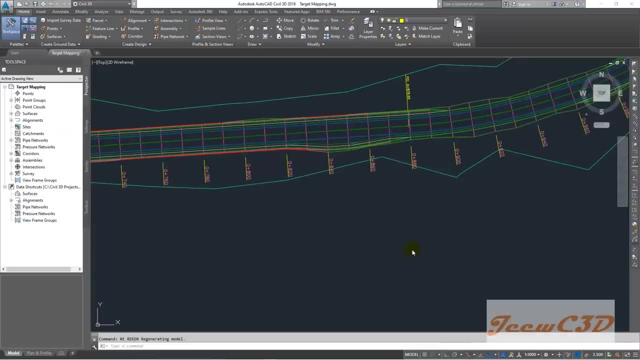 splitting the corridor to have the correct region. In this video, we are going to learn something called splitting regions, because we have a set of regions in this row, So we have concrete grains, we have bridges, we have a bridge section. So, if you recall the region table which I gave you in the earlier 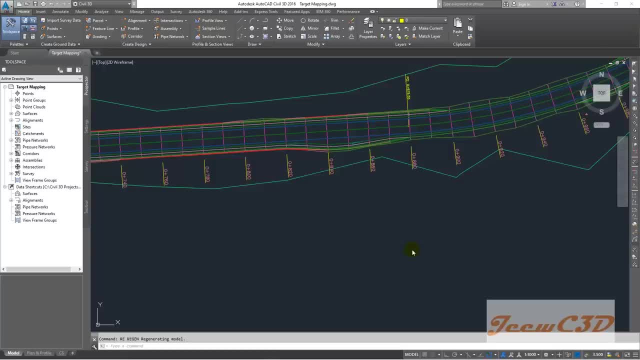 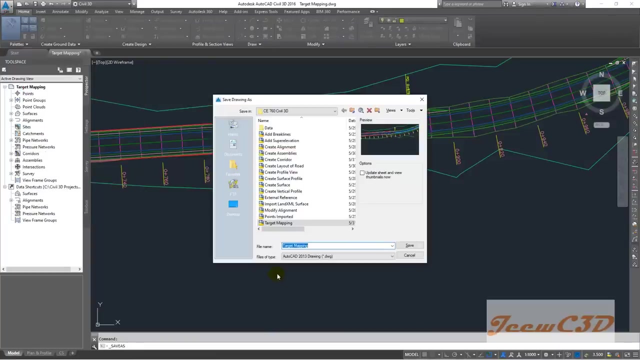 video you can see there are three cross-section types and there are four corridor sections in this row. So by splitting corridor, what we do is we are creating four corridor sections in this row, So I'll do that. before doing that, we will save this rowing as splitting corridor. 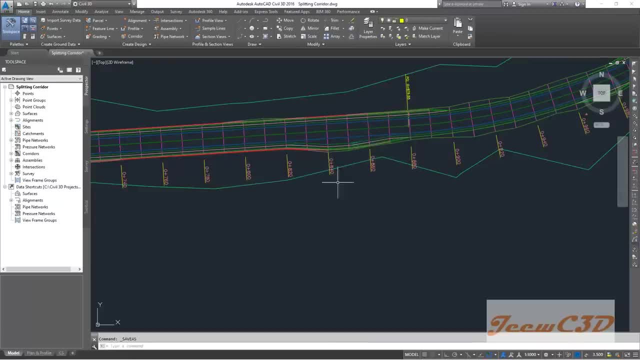 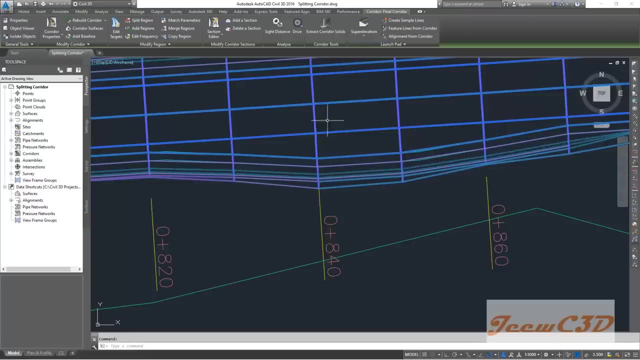 then I select this corridor. somewhere here this magenta color line, I select the corridor. So once we select this corridor, we will add thisуютy row for splitting the corridor. Then I select this corridor. somewhere here this magenta colorline, I select the corridor트. 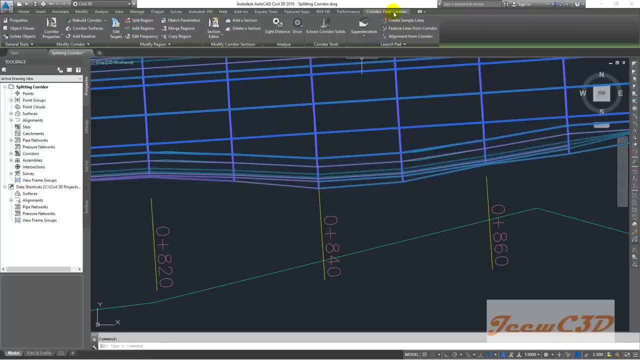 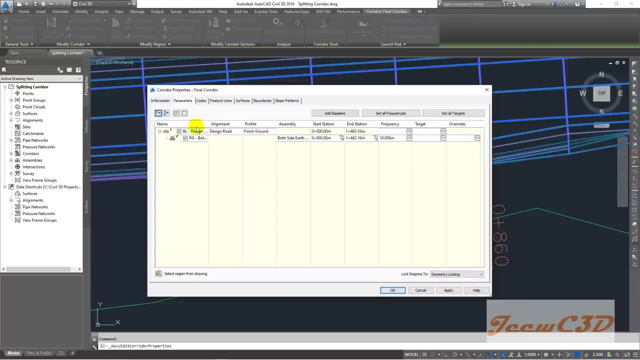 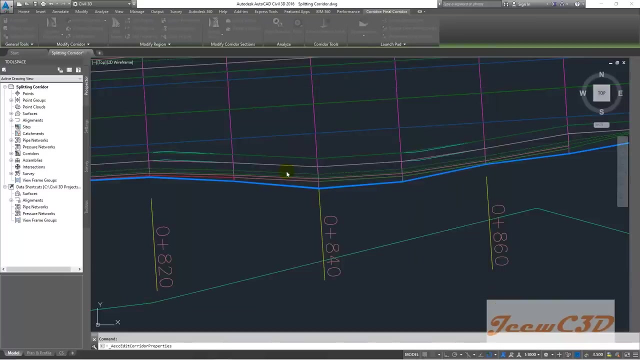 select. you can confirm it by having this name, because our name is final corridor, so i go to here, corridor properties. then on the parameters tab i select this region line and right click. so you have to select the bottom row. then you right click and go to split region. then you have to type what. 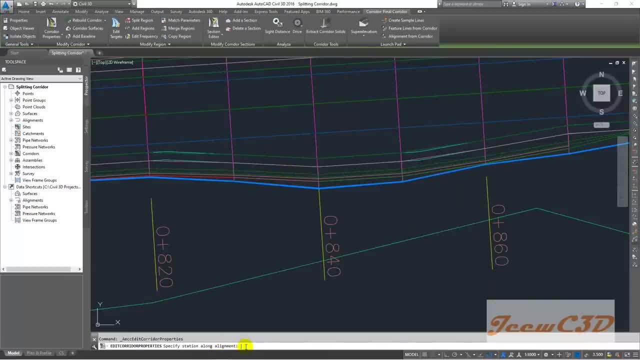 are the regions you have to divide this corridor into. so up to 960 you will be having the grains, then 960 to 1045, you have grain grains, then 1045 to 1060, you have this section. 1060 to end, you have the complete section, so you don't have to split. 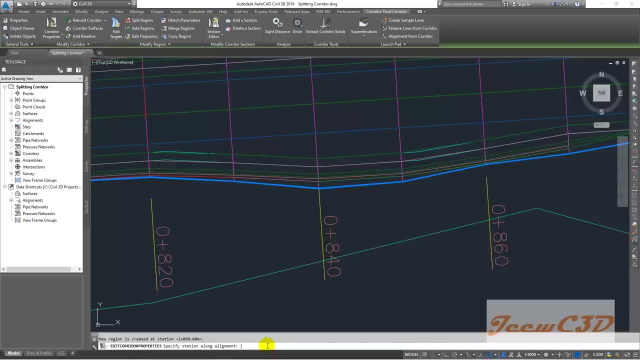 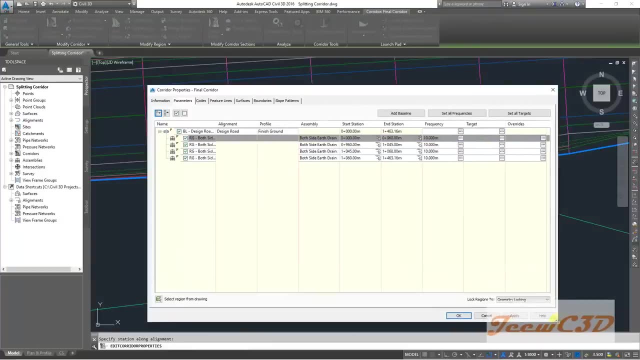 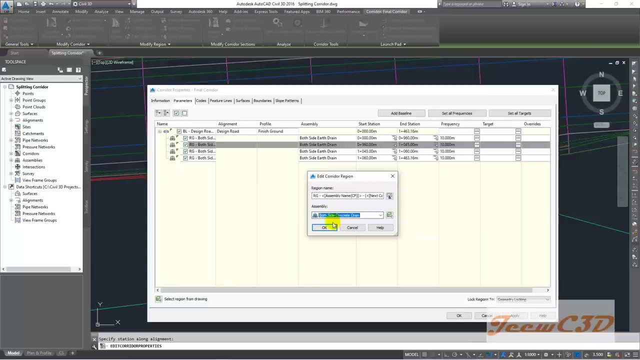 the end point, just click enter so you will see our regions are now divided by splitting the corridor. now each of these sections. currently my assembly is both side at the end, but you know from this, for this session it should be assembly, should be both side, concrete grain. this is how to change it. you click here and you select the correct assembly. 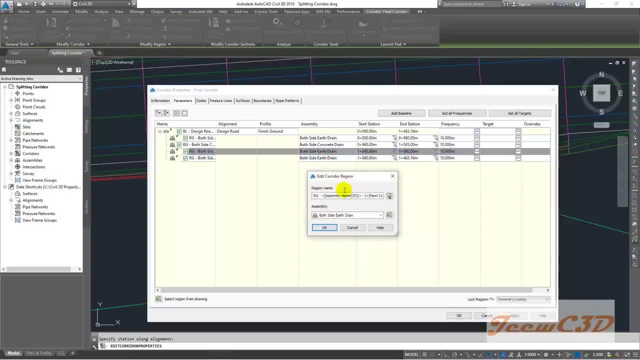 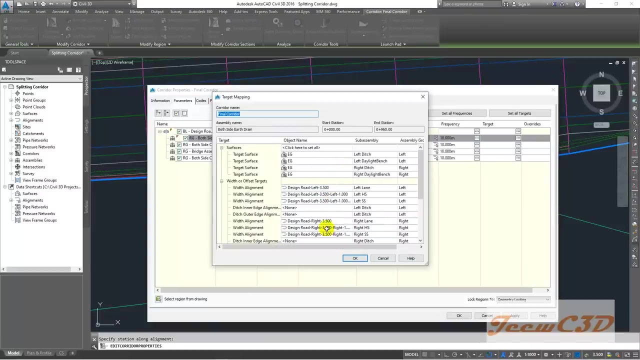 click. ok, here it was. which assembly? here it was concrete train. so that part is okay. but we have to make sure the targets are also correctly placed. so in earth drain we set the targets. so if you go to this target bar you can see the targets are set, because you have. you will see all the names here. 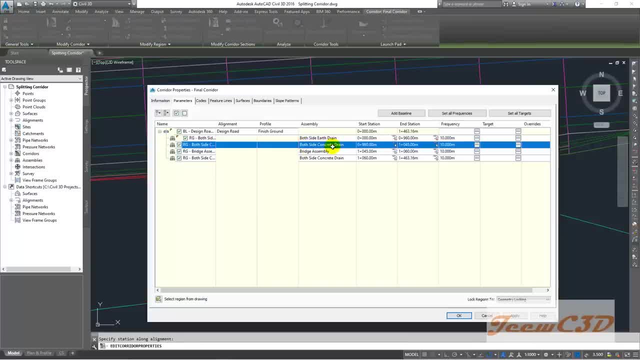 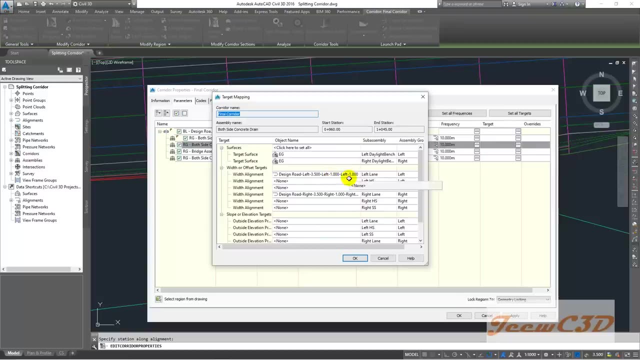 correctly so. but if you go to concrete drain you have to make sure the targets are still there, because we change the assembly at this point, so we go to targets. you can see, even though you have something to left lane, it is wrong, because for left lane it should. 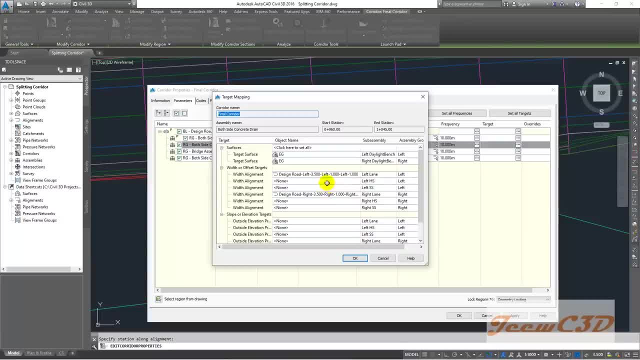 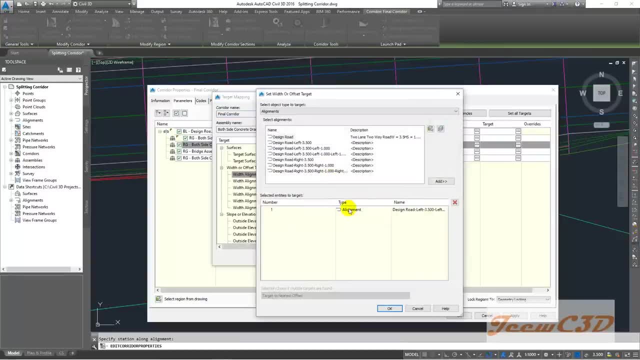 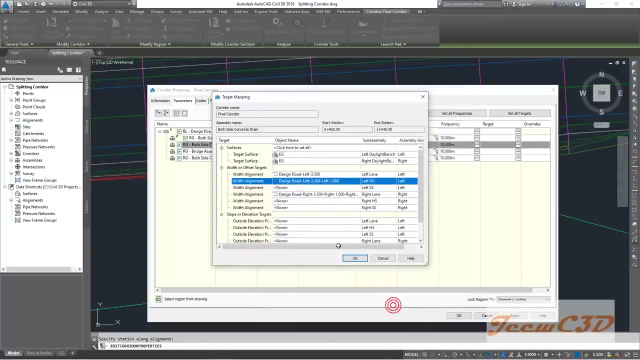 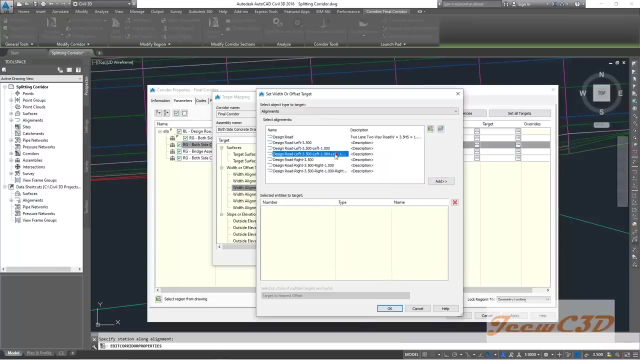 be design dot left 3.5, so this row. you have to define them. then you click here: this should be removed, so i click here to remove it. then your plate should be this one: click ok. then your left arch is there is this one, click ok. and search folder is this one again. click ok, so this one, and i click ok again. 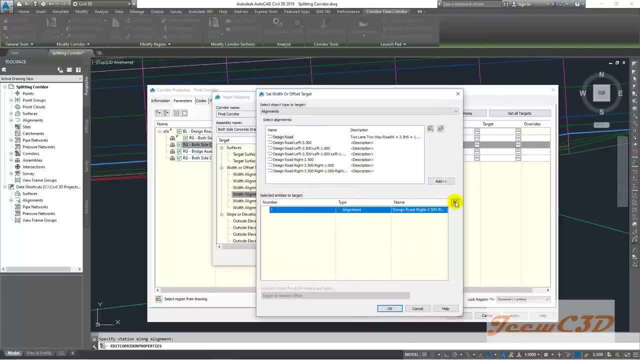 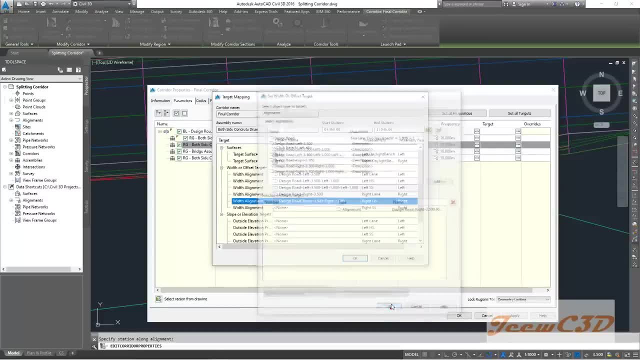 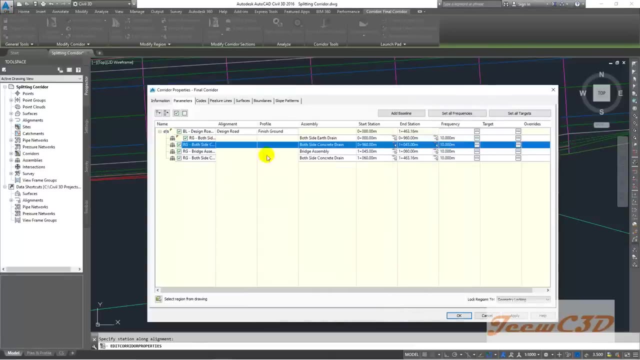 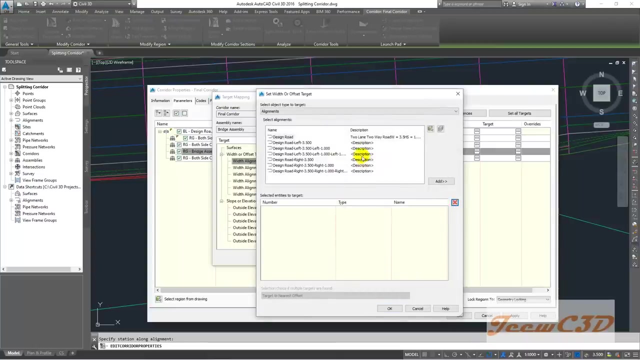 so for the right side also, this is not the correct one. i delete it and i set the right values to these planes with the correct target mapping. so far we have done with this one. then i go to the bridge assembly and this has the same problem. so i will. 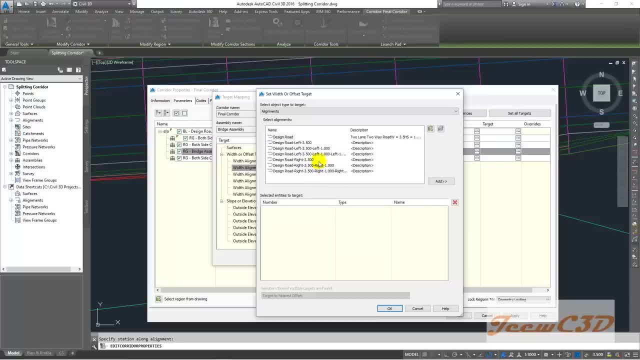 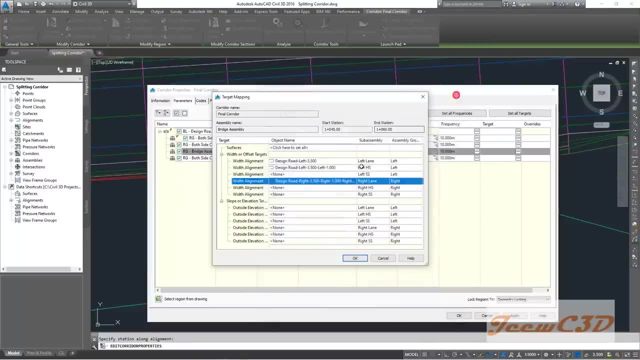 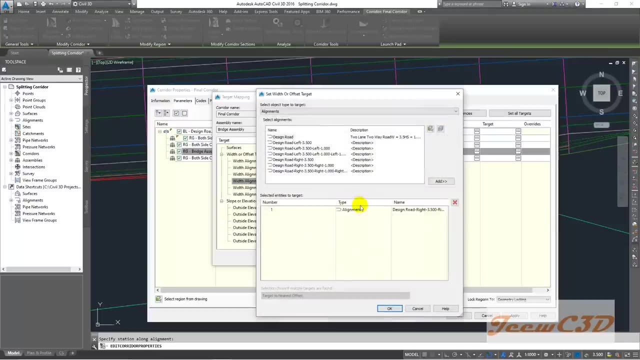 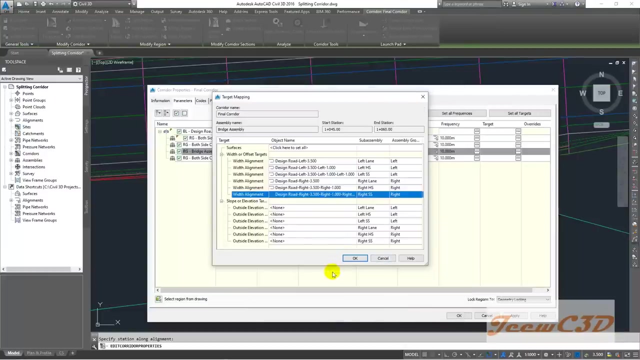 change the things according to the correct version of the assemblies. here also, i have to change the soft shoulder, then i go to right plane, so i will change all the parameters now. so we have changed all the parameters now, everything ok. again i have to go to the bottom one, which is the concrete drains. 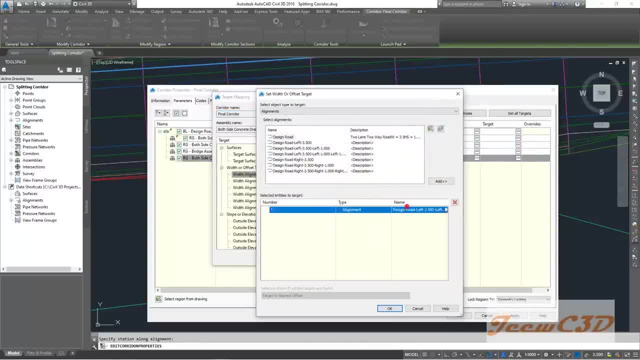 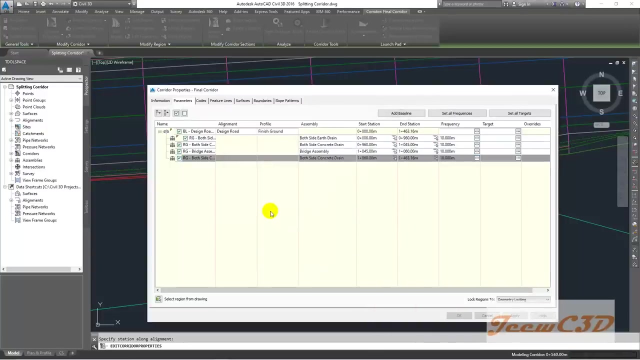 so now delete this one and again. i will complete all the parts. correct click to get the correct matched on the target. so, as you can see, we have done with this one. so i will change all the parameters now. OK. now everything is OK, so I click the OK button. 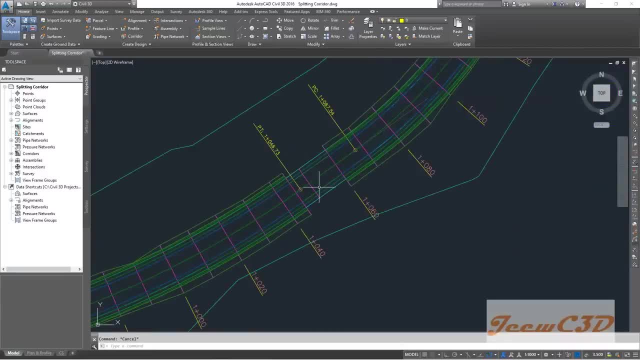 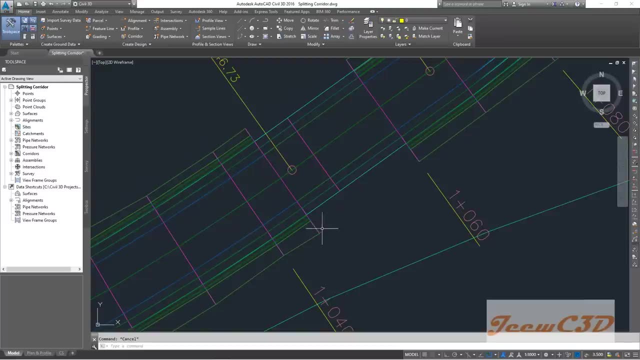 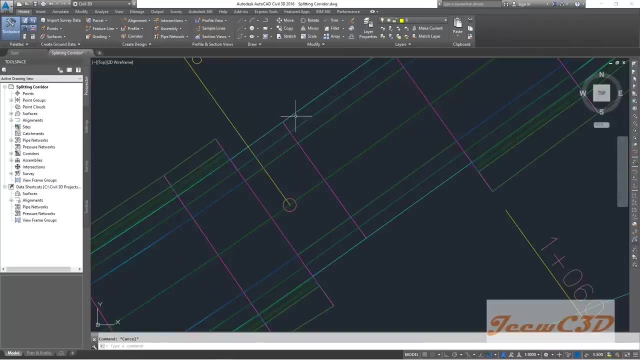 So you can see you have a big section here, you have concrete drains here, so you don't see that, but they haven't been applied because you can see from the big section here you don't have much corridor here. so that means you have the red target targeting also. you 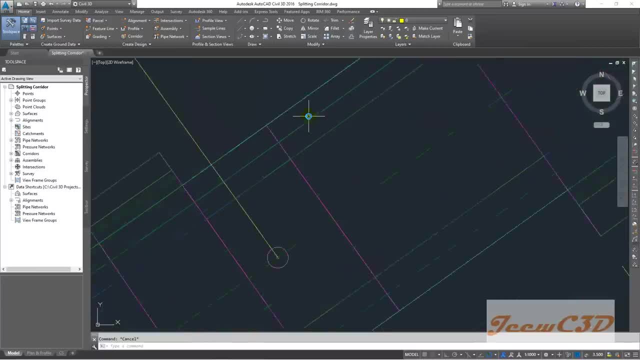 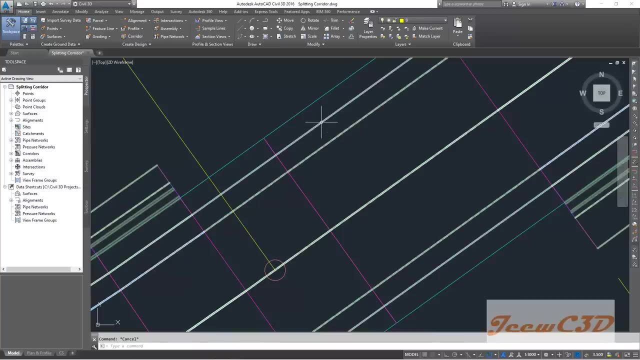 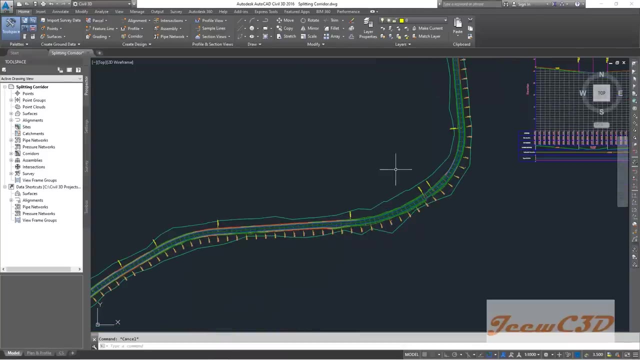 can see that soft shoulder is not available in the big section, because you can see that in the big section you don't have a soft shoulder, only you have the hard shoulder. So so far we have now created the corridor regions by splitting the corridor and we have 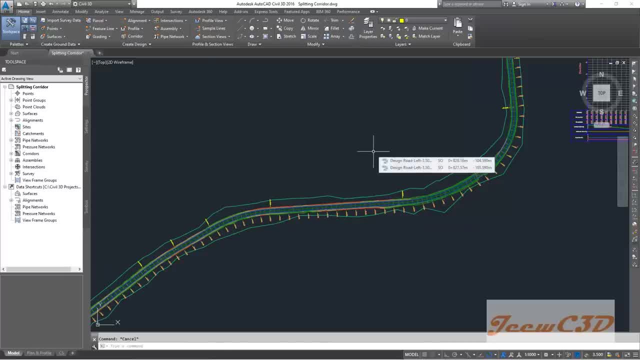 set the correct targets. also, In the next video, we will be looking at how to create the corridor surface. Now in this video we are going to look at how to create a corridor surface. before that, I will save this drawing, this splitting corridor drawing. so it will be saved and then I will. 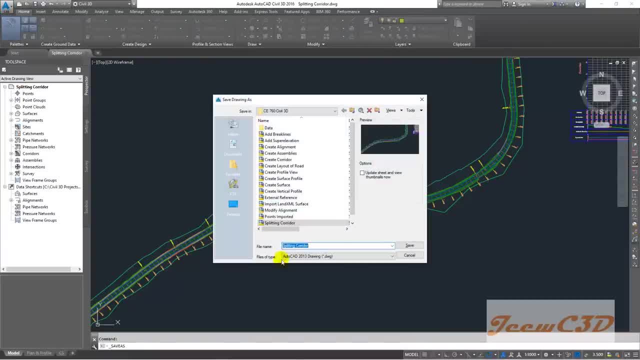 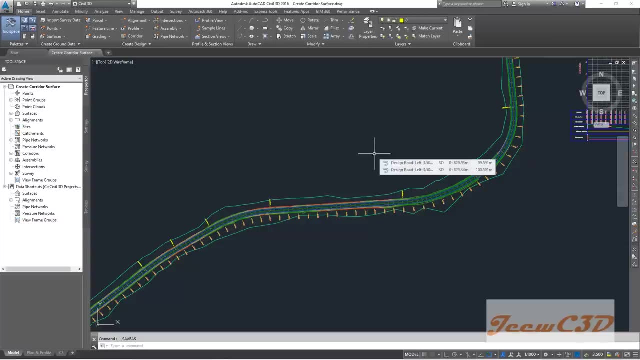 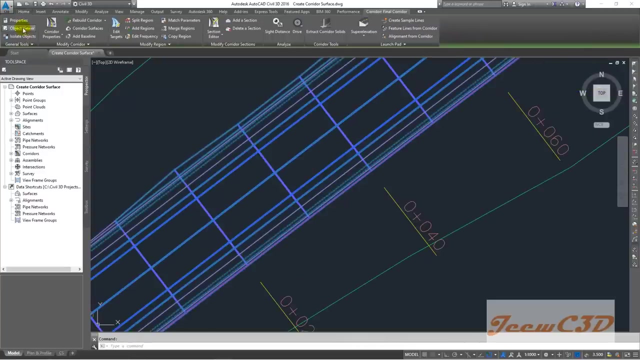 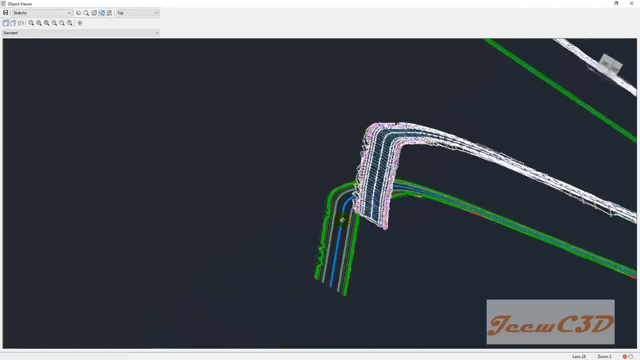 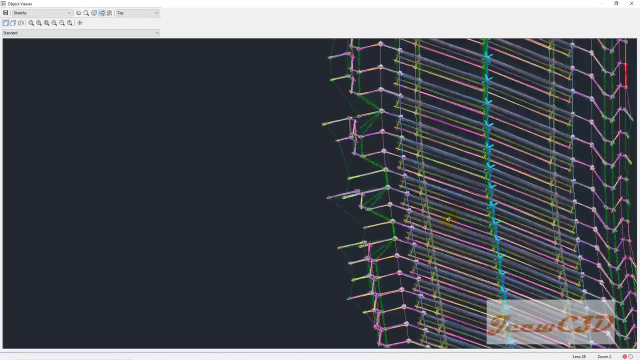 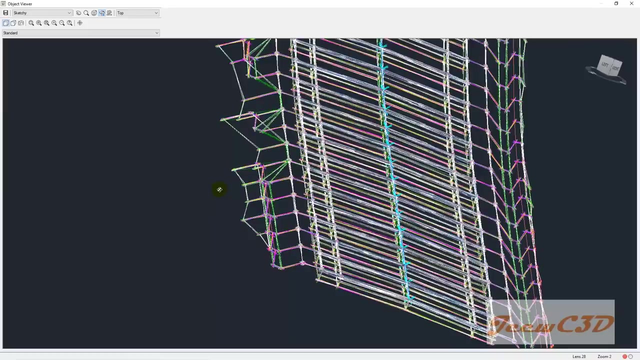 save as the drawing. as: create corridor surface. So creating corridor surface. corridor surface means something like this: if I select this corridor and go to Object Viewer, I told you earlier a surface means a flat surface plane. so what we are doing by a corridor surface means what we are doing by a corridor. 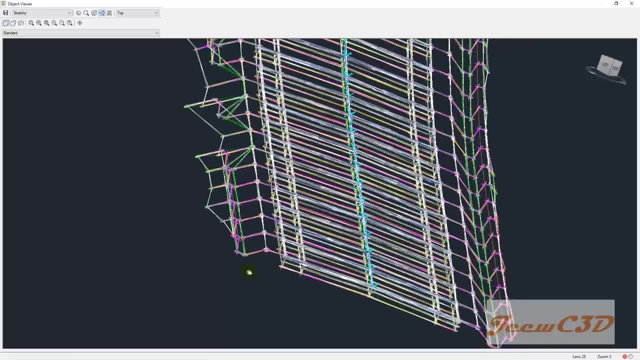 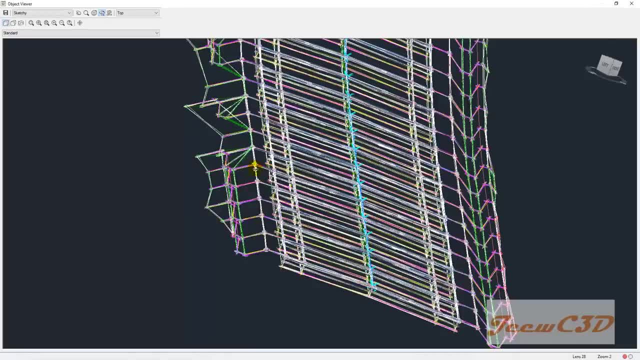 surface is we are connecting the top points of these cross sections. you can see the cross sections are applied at any time to us. we will be connecting the top points of the cross sections For the assemblies and we are creating the plane connecting all those top points so that 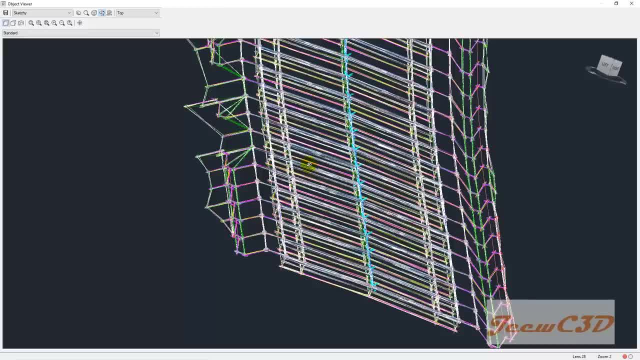 plane is called a corridor surface. we call it corridor top surface, the surface which is, which is created by connecting the top points of the corridor. so we call it corridor top surface. so when the connecting points are covered, top coat, so we have, we are. 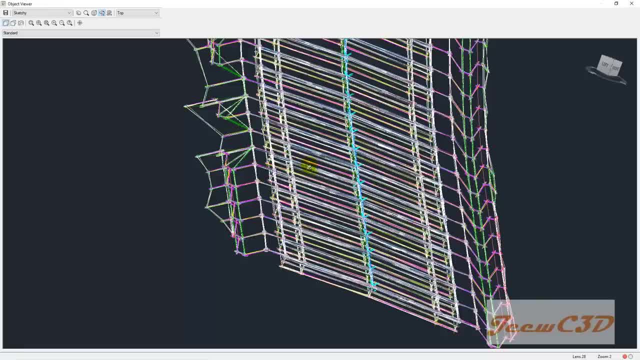 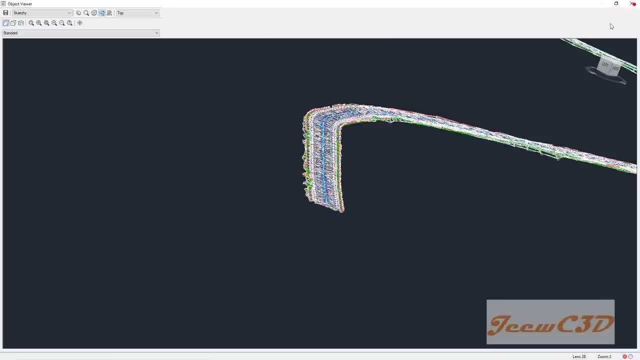 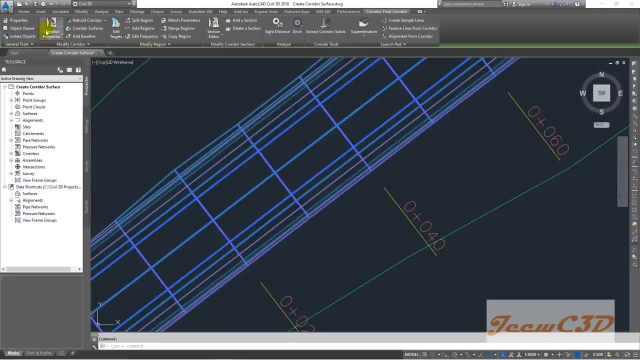 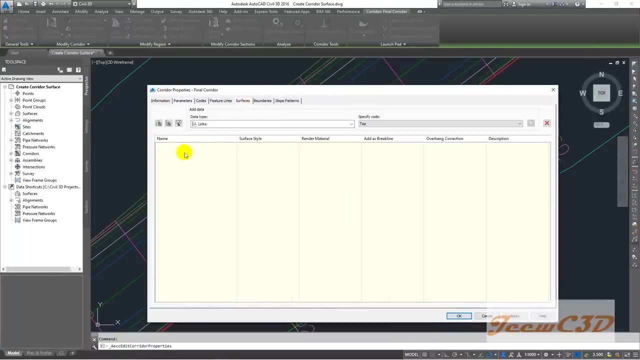 connecting the top coats on the assemblies and creating the corridor top surface. I will close this one here. so here, to create the corridor surface, you have to select the corridor and go to corridor properties. then I have to go to surfaces tab. then at the left corner, 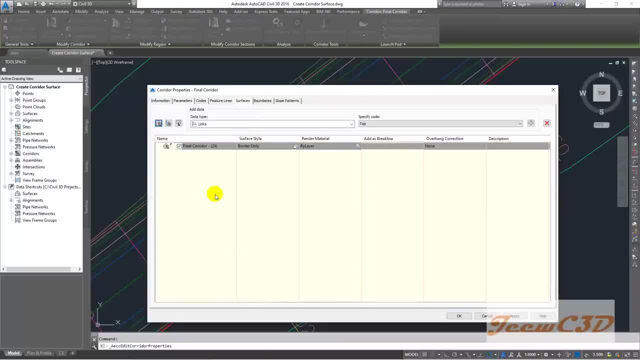 you have create corridor surface button When you create the corridor surface, since we are then automatically, you have a name for the corridor surface, so it will be a top surface. that means that means we are connecting the top points to create this surface. your surface style would be border only like this: 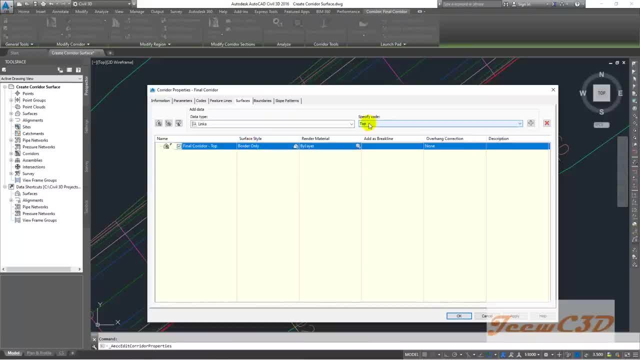 LG surface. then we are connecting the surface by. we are creating the surface by connecting the top coats of the top points. then we add it here so that civil 3D knows we are creating the surface from top points. then just have a tick here to address break line and then 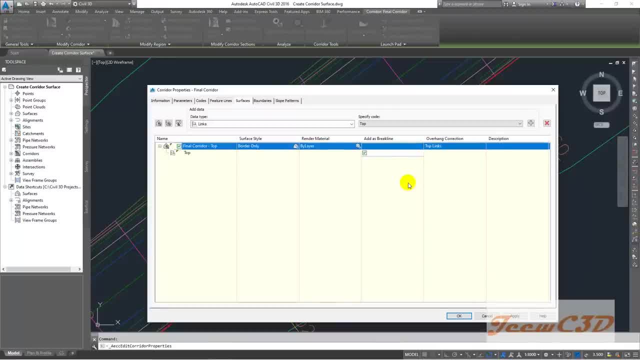 for top surface. just change this to top planes. Since we are creating a surface, we have to define a surface boundary also. so we have to go to boundary, So we have to go to this tab and then right click this surface name and use corridor extent. 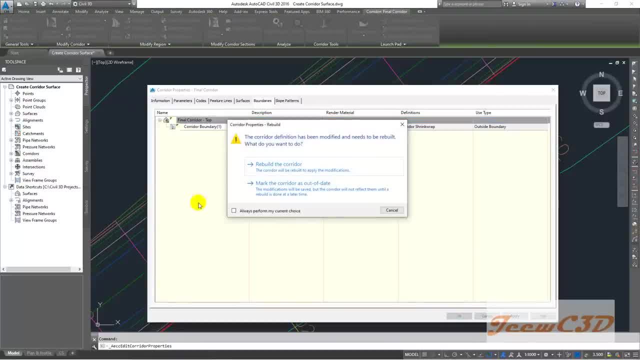 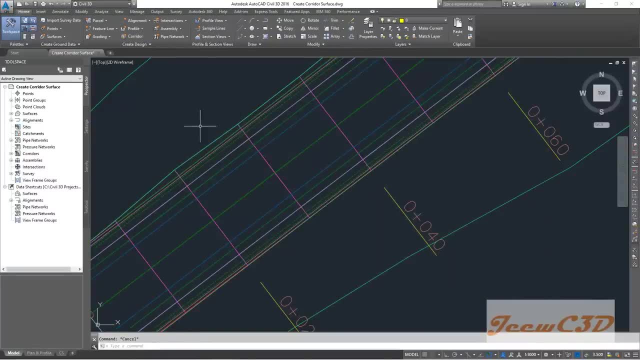 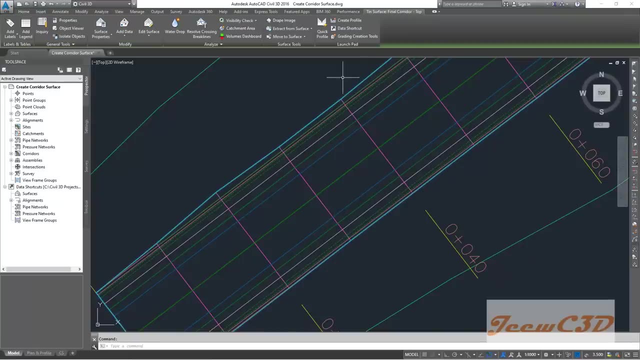 as outer boundary and click ok and we build the corridor. So you will see, if I press k there is a surface at the outside of the corridor. if you click here you will highlight a surface here, final corridor top. so if you go to 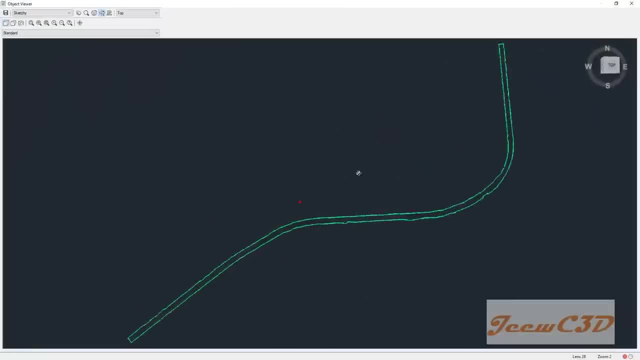 object we will find the final corridor top. So from here you will see that surface. you can change the style and see how this is the top corridor surface. you can see here at the section. here you have bridge. the corridor is bit long. 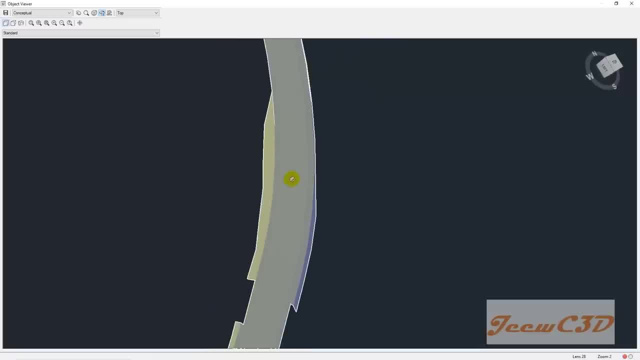 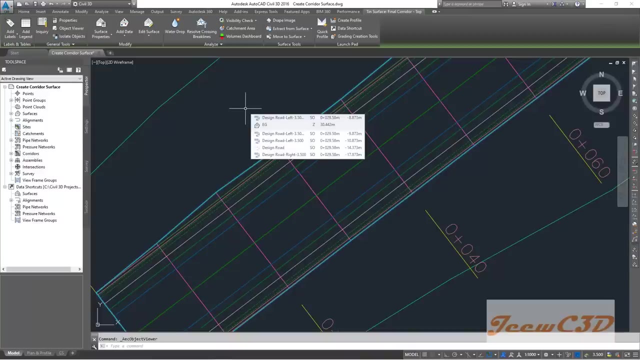 So that is how the corridor is created with top surface. So that's about corridor surfaces. In the next video we will be looking at how to create sample lines and section views. So that will end this video, Thank you. 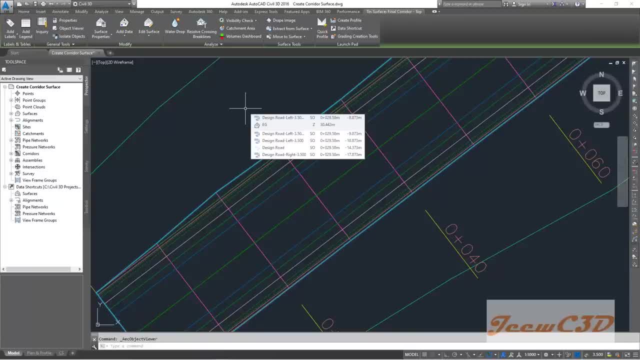 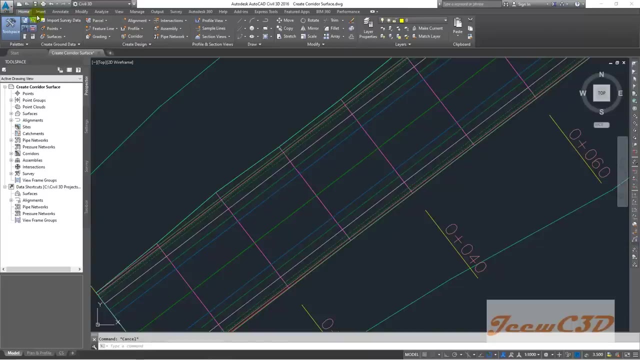 End the civil 3D session after we create the first sections, and in the next video you will see how to do that. Before that, I will save this drawing before moving on to the next session. In this video we are going to create sample lines and section views, or else the cross. 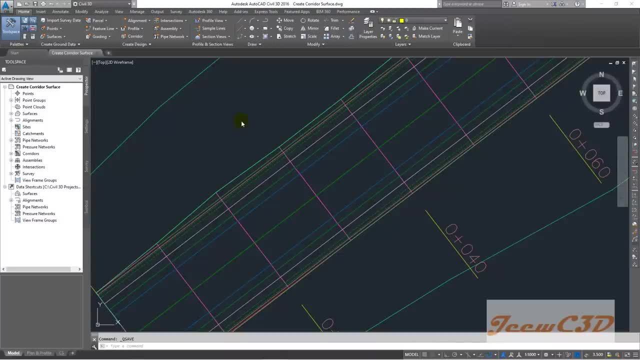 sections. In the last video I told you to save the drawing. If you haven't done that, you can save it now because we are going to change the name of the drawing. So once you change, I go here and save as the drawing. 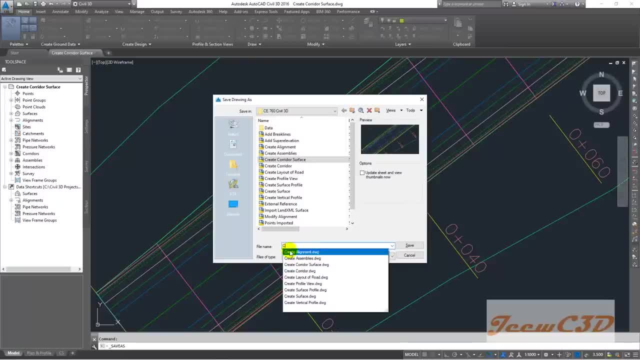 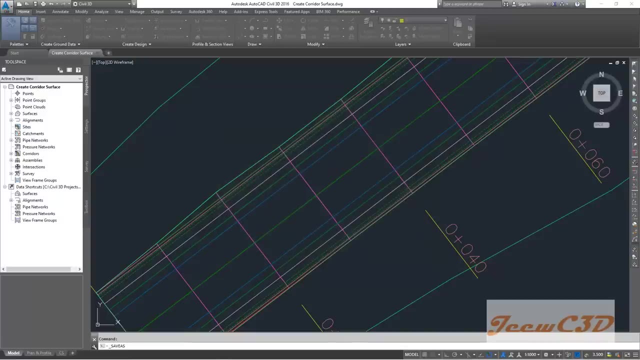 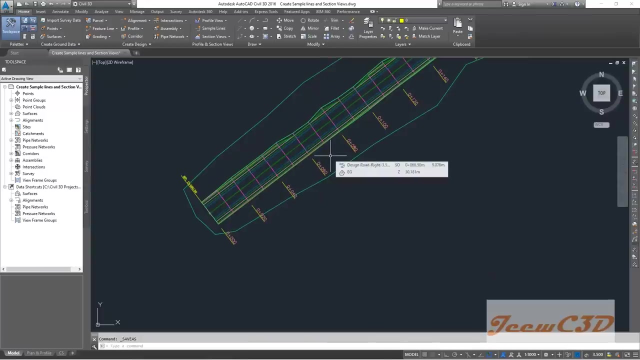 Create sample lines and section views. So once you change, I go here and save as the drawing. Create sample lines and section views. Okay, Sample Lines and Section Pills. Now what I am going to do is something called creating Sample Lines. Sample Lines means, that is, the locations where we get the cross-sections. 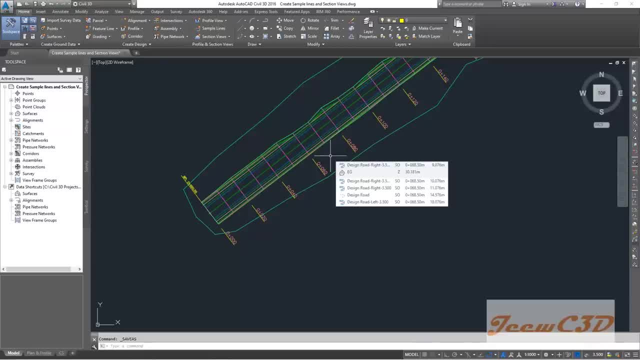 So a Sample Line is used to gather data inside that area to create the cross-section. So cross-section would be displayed depending on the cross-section of the Sample Line location. We will see how to do that. So you have to go to Home tab, Go to Sample Lines from here. 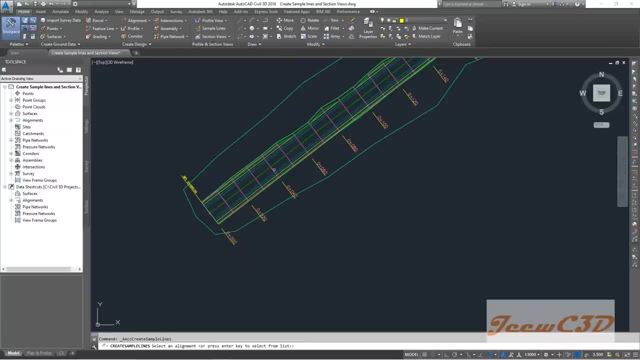 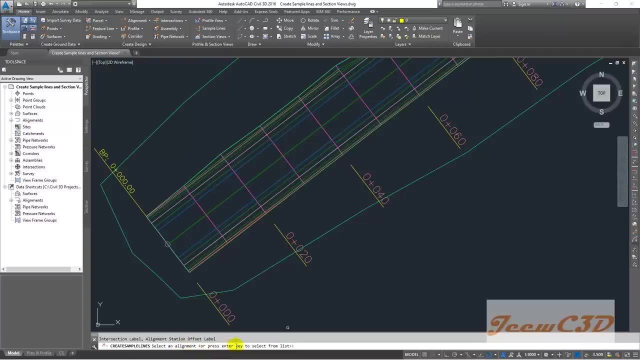 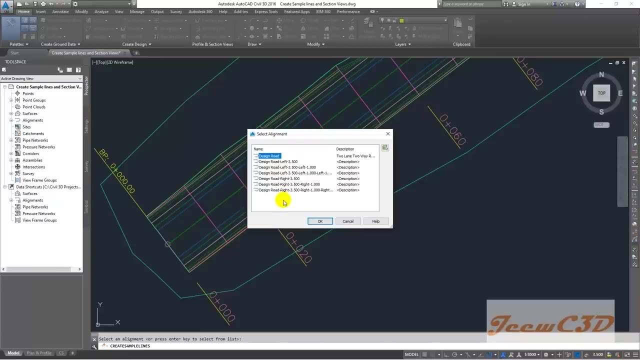 Then you have to select this Center Line. If you can't select this Center Line straight away, You can press Enter to select from the list. So you have so many alignments because of this Offset alignments, But you have to select the Center Line. The Center Line is Design Gold. 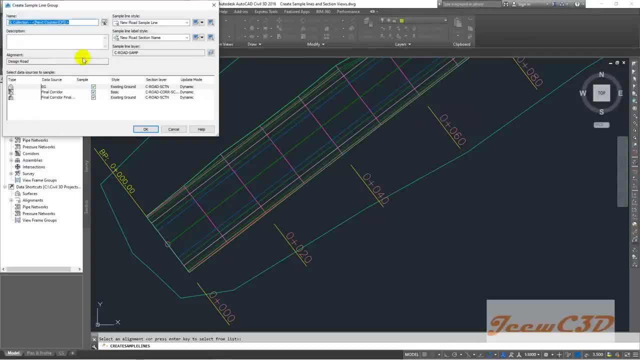 So you Click OK, Then you will have the data which is available to Sample for this surface, Because when you are going to create the Sample Lines We have to give data to the Sample Line. So it will show us the available data in the drawing Surfaces and Corridors. 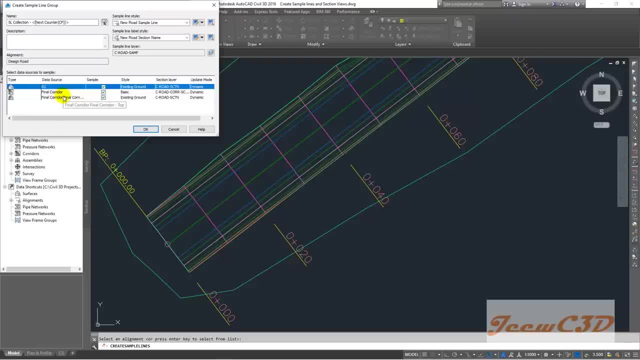 So it will. let us see all the Corridors And Surfaces here, But for the moment I will skip one And go forward to show how To show one more additional thing In a later part of the video. So I will skip one. That is the final Corridor I have skipped. 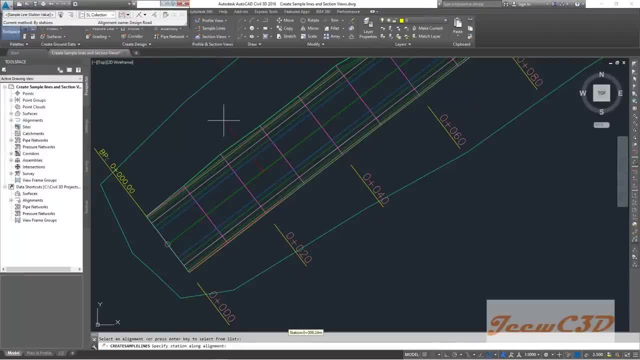 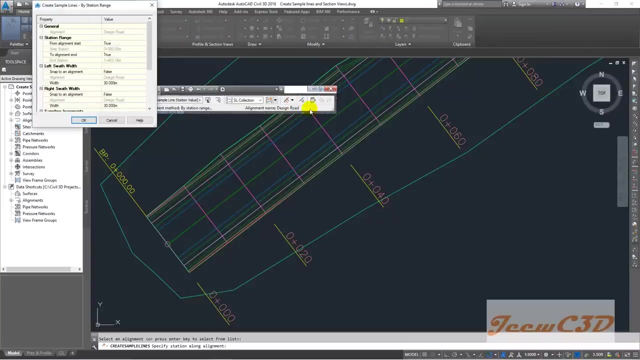 And I click OK, Then a small Toolbar will be appearing here. So you will see here Small Toolbar. From here you have to select By Range of Stations. Here you have to go to this, Go to this drop down and select By Range of Stations And we are having the 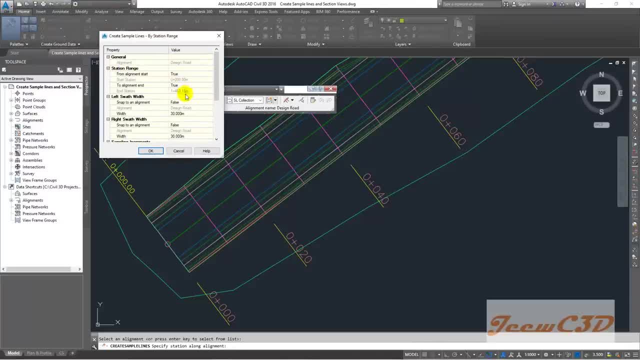 Sample Lines from Start to End. So if you are not going to have Sample Lines from Start to End, You can modify it by Making it False here. But currently I am making it True Because I used complete code section to Create the Sample Lines. Then it is asking: Left Short Width. 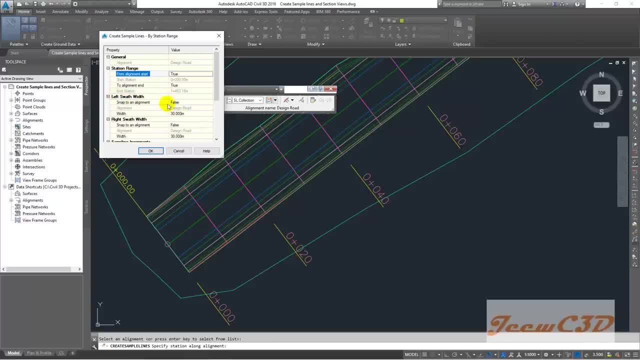 That means How much to the left you need Sample Line. So the best thing is to Take the Length more than the Corridor. So we will be thinking this 30 meter is OK. Then again we have the right side. So let's say 30 meter is OK. 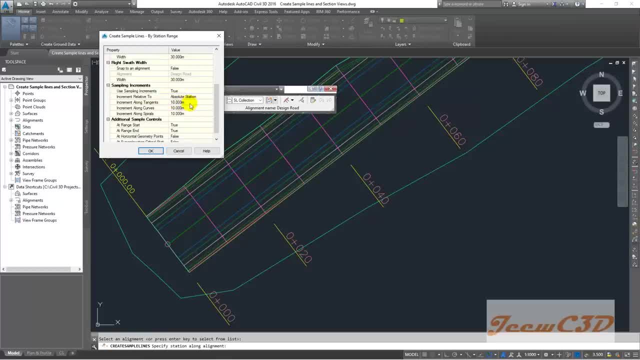 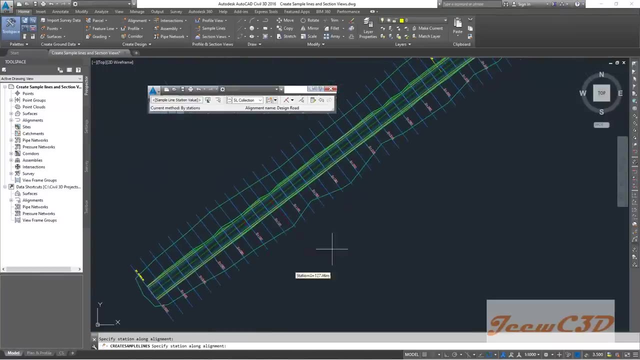 Then it is saying At what interval you need the Sample Lines. So we say At 10 meter Intervals, And these values we are not going to change. Then I click OK. So you will see The Sample Lines are created At 10 meter intervals along the Corridor. 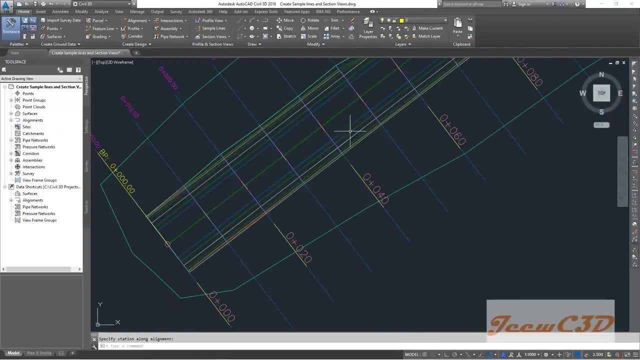 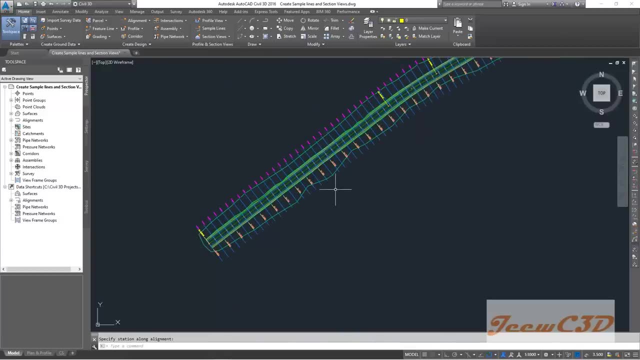 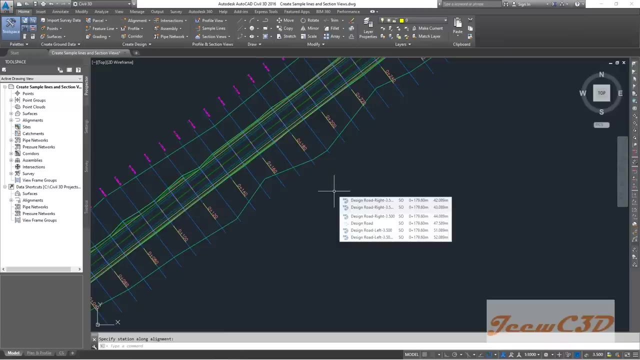 So I click here to close the Sample Line Toolbar. Then you can see The Sample Lines here. So suppose we forgot to add some Data to the Sample Line? If you can remember, I purposely Avoided one Corridor Without adding to the Sample Line. So let us say: 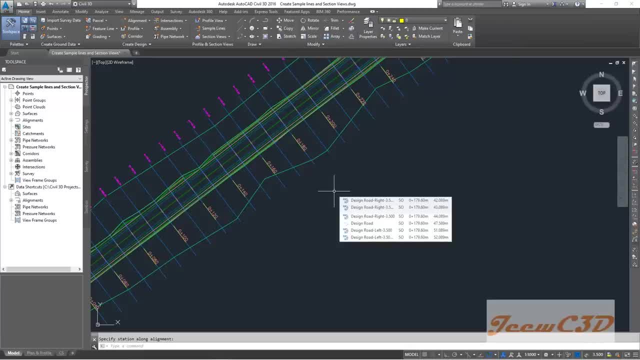 If we have forgot one Corridor or one Surface To add the Sample Line, So in that case you can Go and add it again. Now I am going to add that Forgot, But at that, Now I am going to add the Skipped Corridor to this Sample Lines. 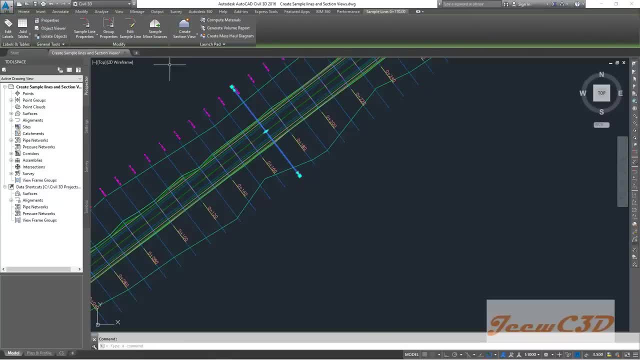 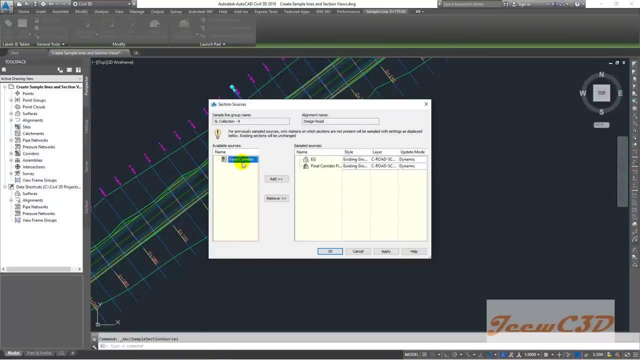 So I click here. Then I go to Sample More Sources. So in the left side We have the available sources, This source for the final Corridor- I haven't sampled into the Corridor, So to Sample Line. So here I click Add And I have to. I will change this style to. 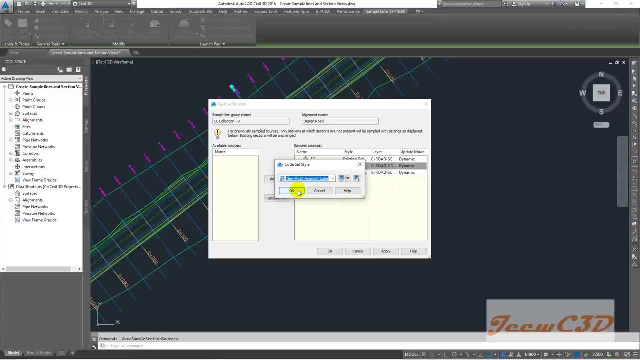 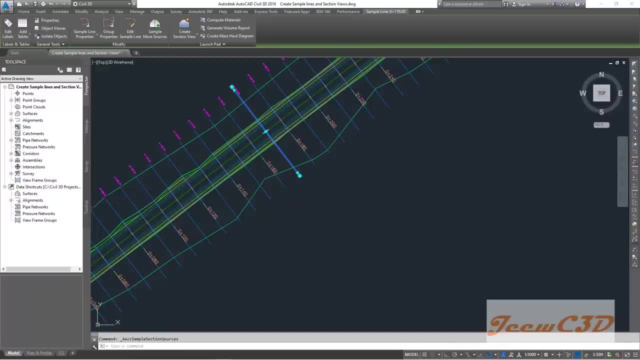 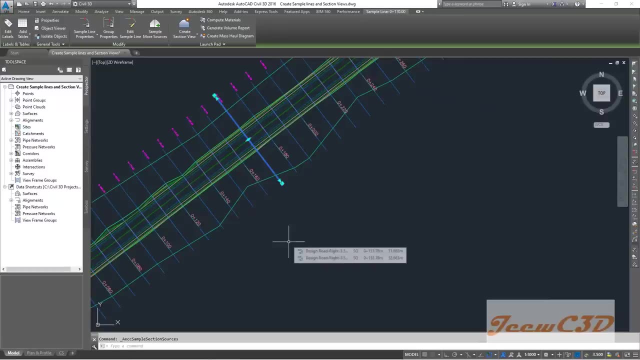 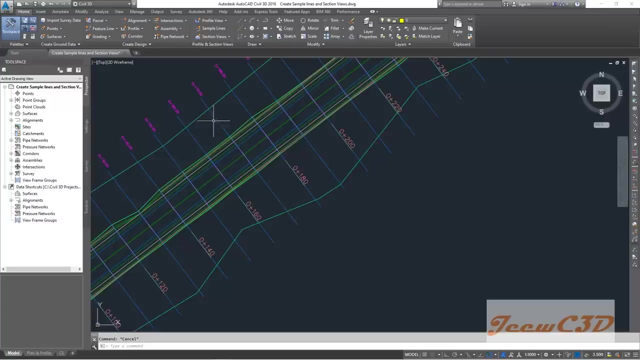 New Role Assembly Labels And click OK And finally click OK. So once you select one Sample Line And add some Data, It will be applied to the Four Sample Lines. So I press K to Deselect the Sample Line. So what will happen is, At this point, the Sample Line 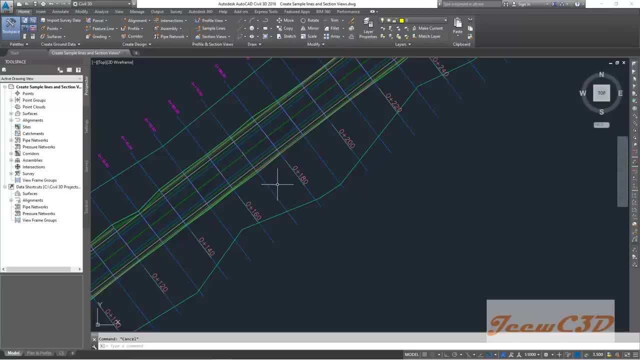 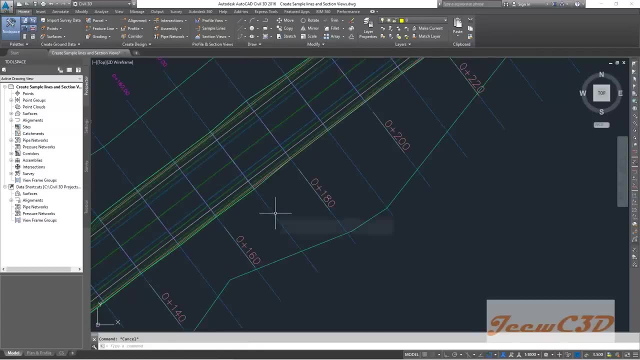 Take all the Data To this Sample Line According to the Sample Data. So we have Sample EG Existing Ground Surface, Corridor, Top Surface And Corridor to this Sample Line, So it will be having this Data inside This. Now what we are going to do is Create Section Views. 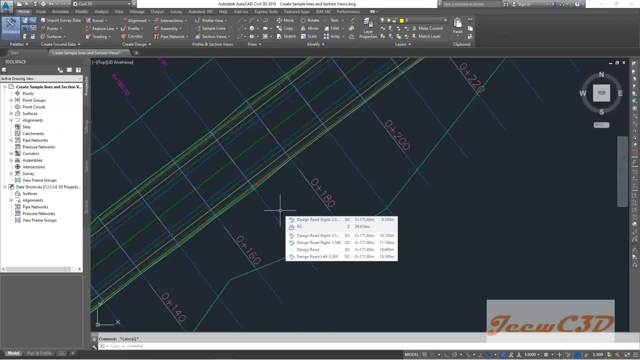 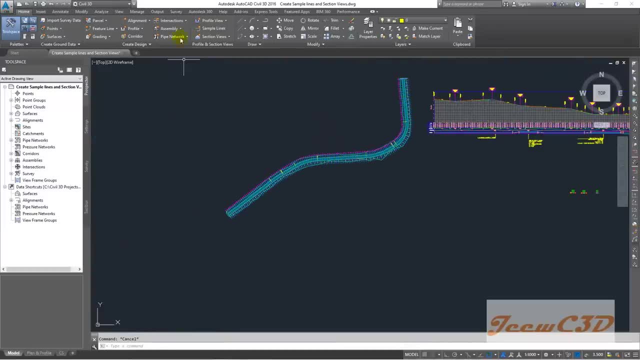 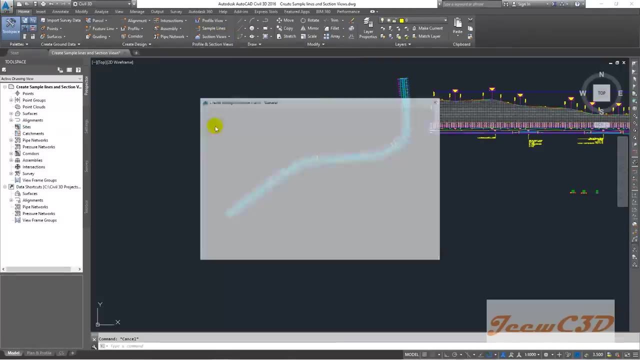 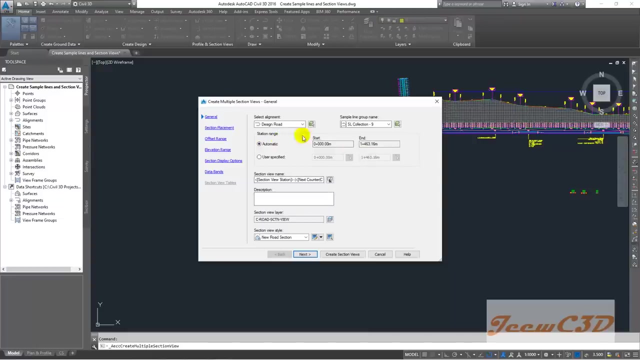 From this Sample Lines, Because without Sample Lines We can't create First Sections. Now, to create First Sections, I go here Section Views, Then I go to Multiple- Create Multiple Views. Here it will be giving Available Data here. Since we have only One Sample Line Group, We show the 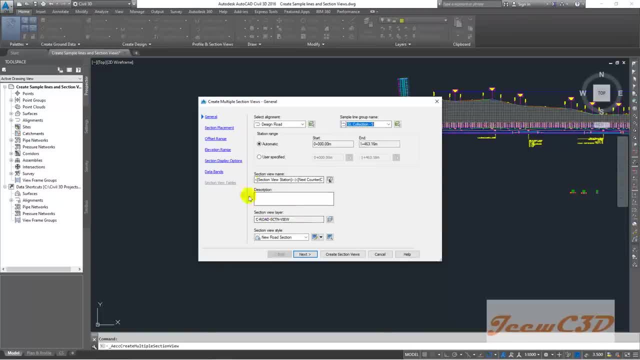 Only Sample Line Group. You can Change this, Set things if you need, But Here we go with These Sections, Then we create Next here, And Also We are going to Place this Draft Section Views Without creating any Sheets, And To Press Next again, And Next again, And Next again. 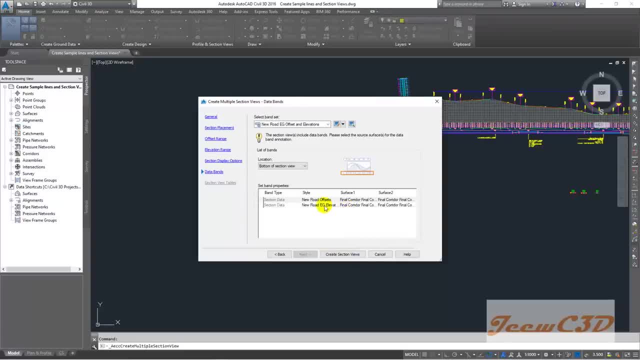 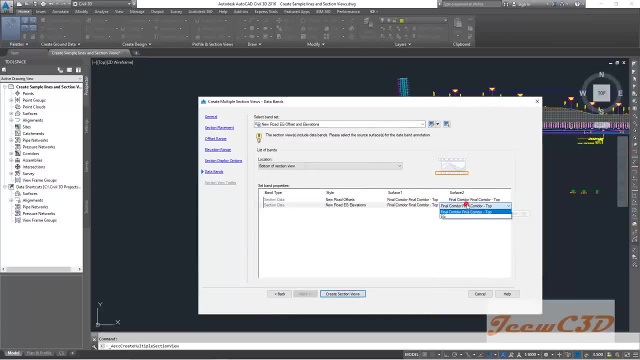 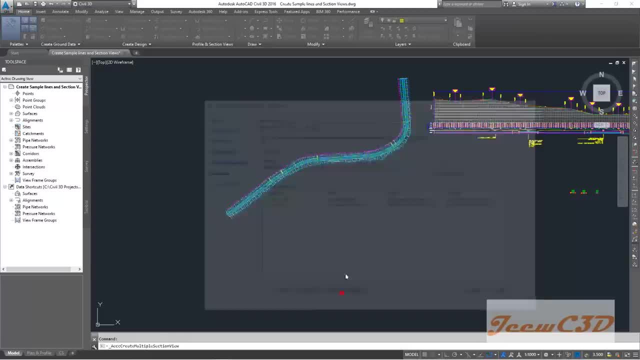 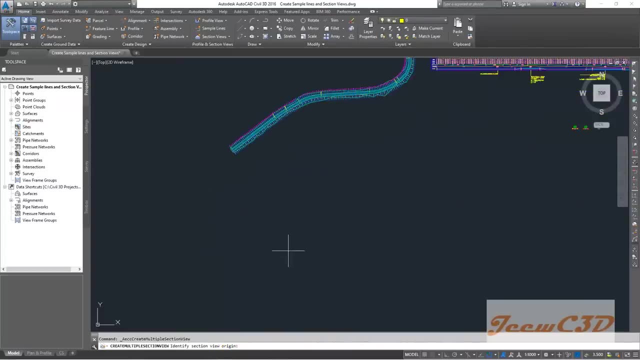 Section Views By Creating Here. So it is asking Where you have to Place the Section Views. So I will be Selecting Somewhere Here. Here you have Enough Data, Enough Space To use Processions. To use Processions. I will Click here Now. You will see A set of 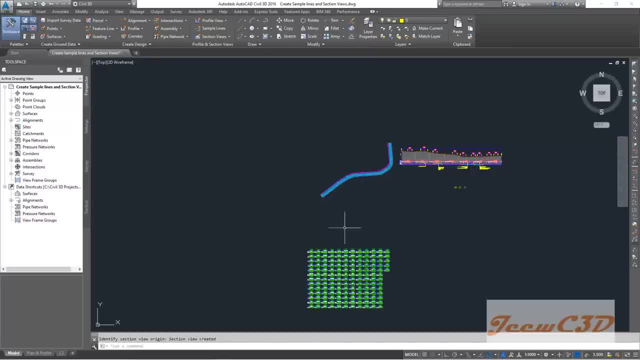 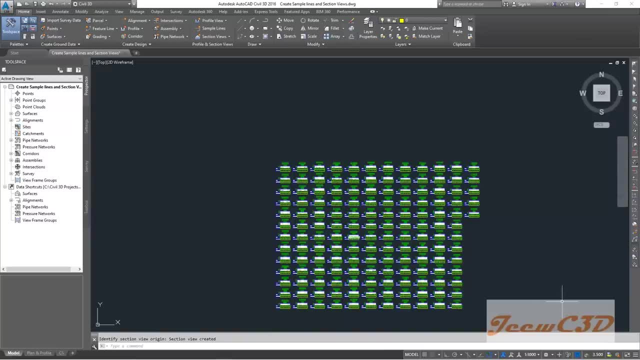 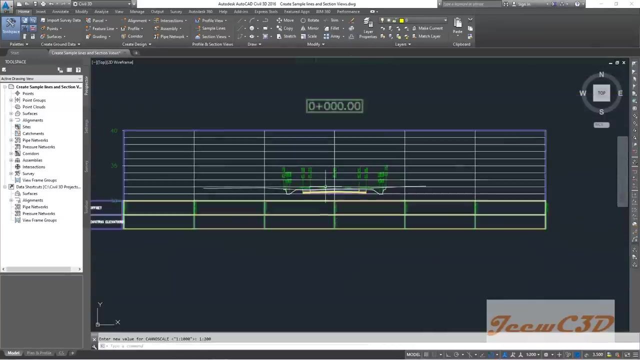 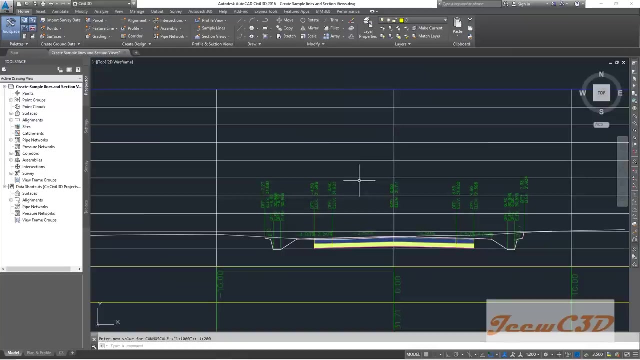 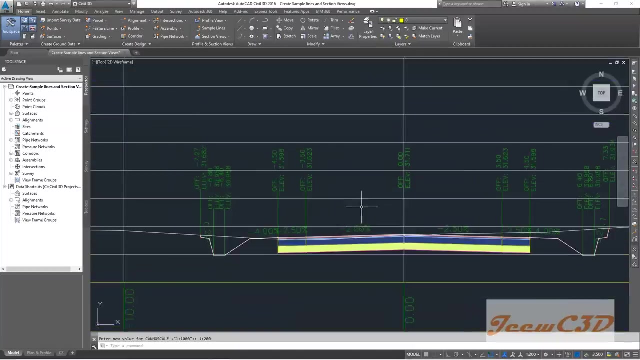 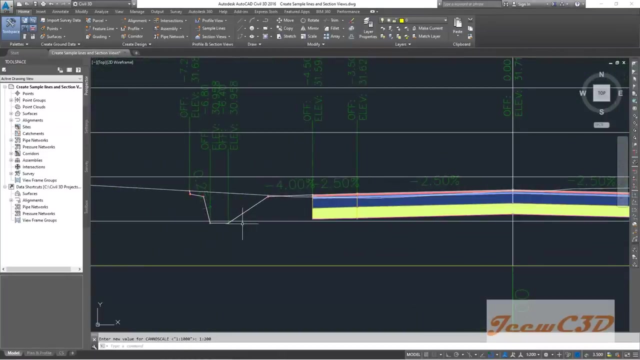 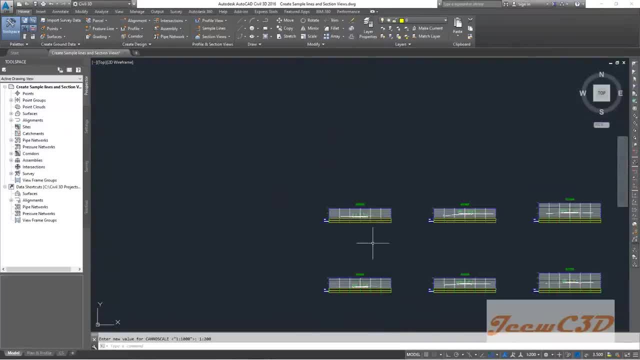 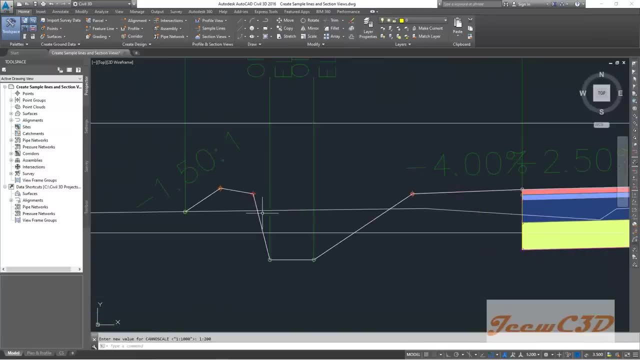 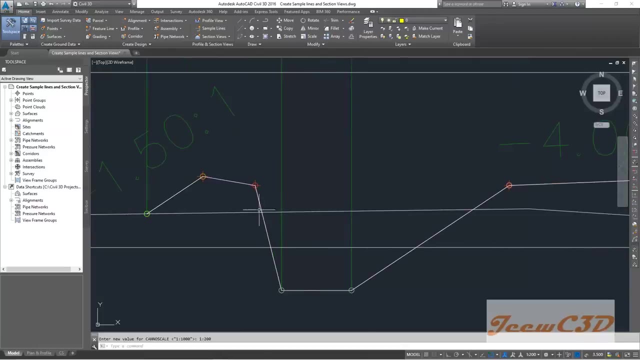 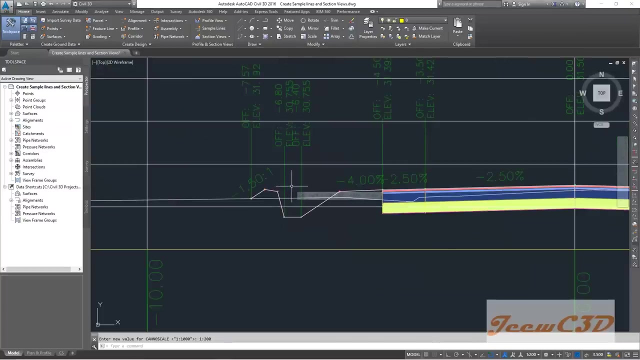 CD, CD. CD CD can see you have this cut section. some of this data you need to manually modify because you can't have a section like this. in that case you have to trim off this drain somewhere here and this part will not be there. so we have to do manual modifications. so if you are getting 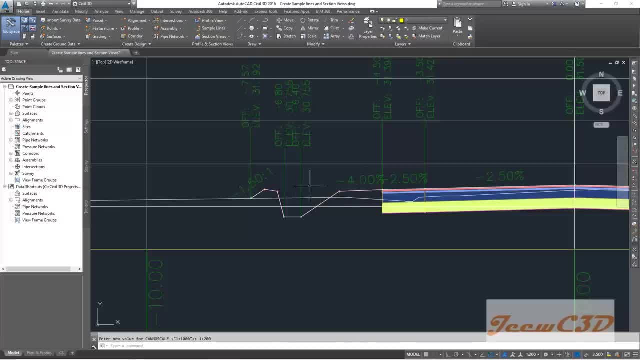 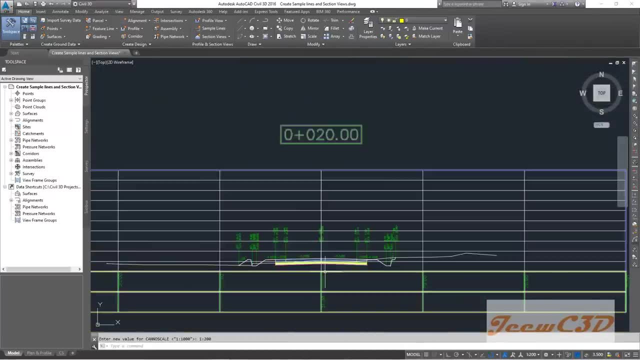 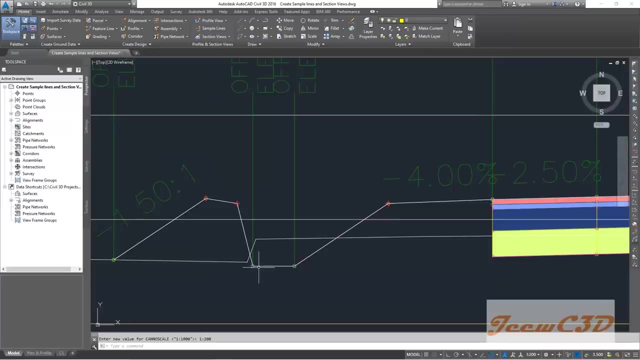 taro. with 3d, you will know how to do the things without making much of these modifications. so that is how we get these things here. also, we have a problem, little bit of a problem. this part will not be here in the actual case, so we have to modify before sending these things to. 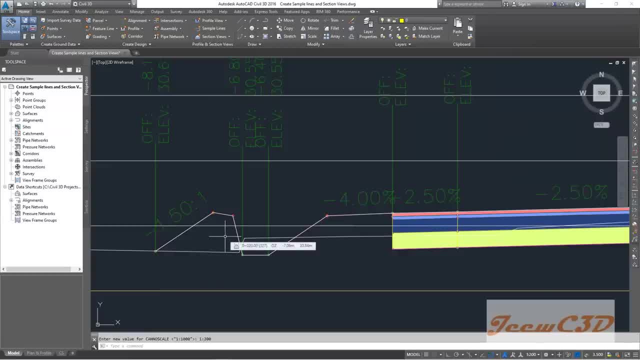 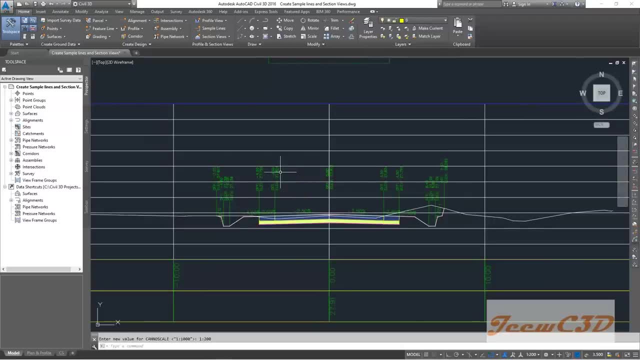 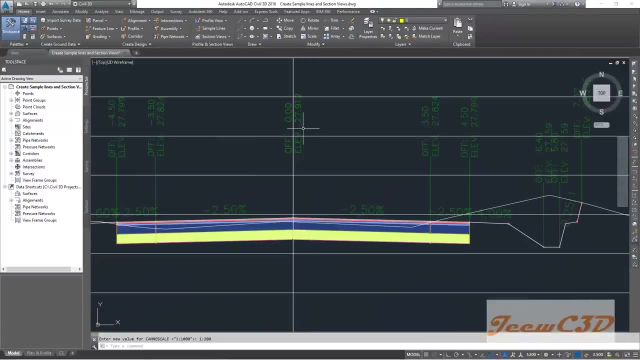 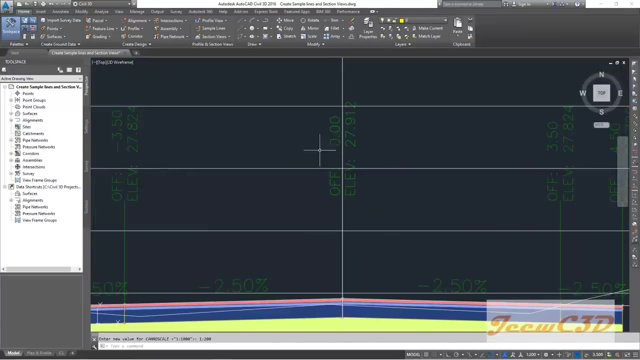 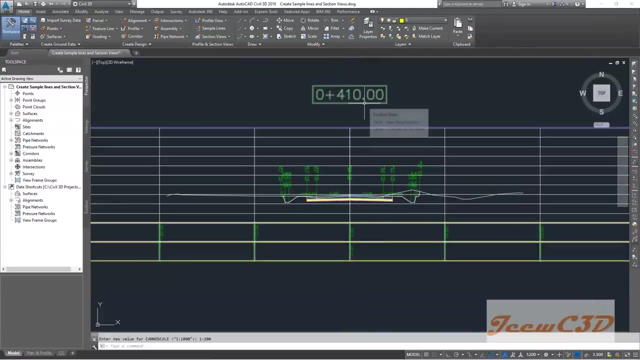 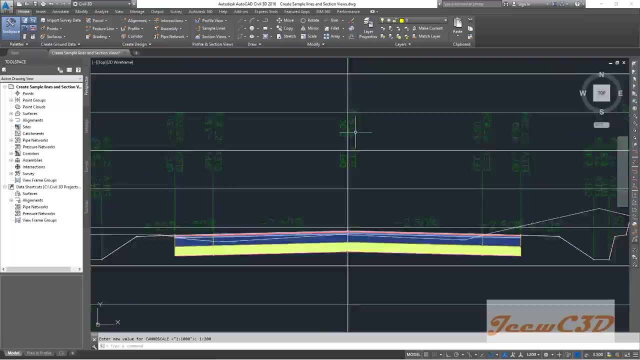 site when we are preparing the final drawings. so if i go, furthermore, and one more thing, i have to tell you this- here you have the layer base of the final crown here. this is the finished round elevation at under 410 station. so if you check the finished round elevation it would be 27.912 at the center. let us check it. 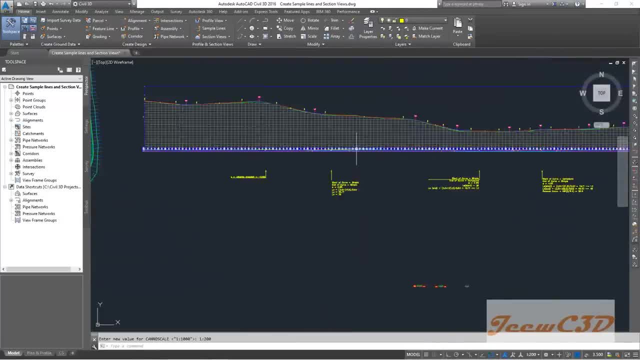 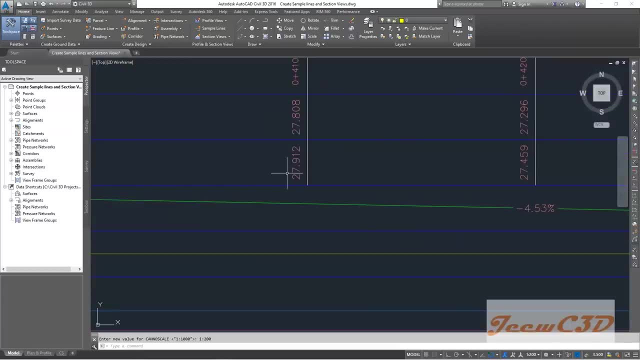 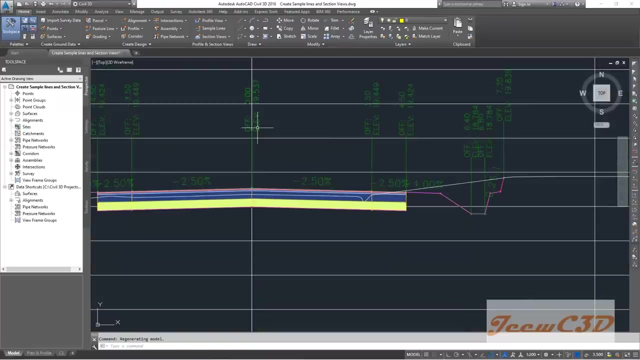 here finished round 27.912. likewise, you have all the data nicely visible inside these cross sections in here you have the. you should have the existing round data, but around 27.912. you should have the existing round data, but around 27.912. you should have the existing round data, but around. 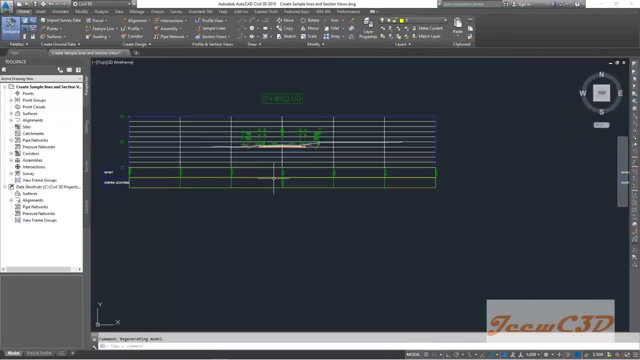 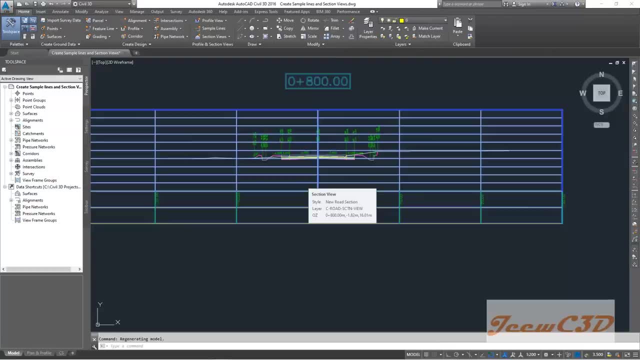 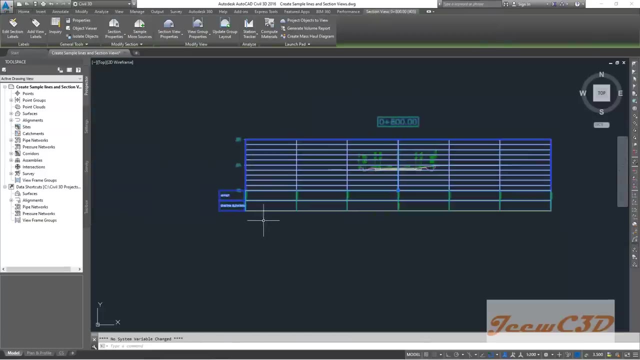 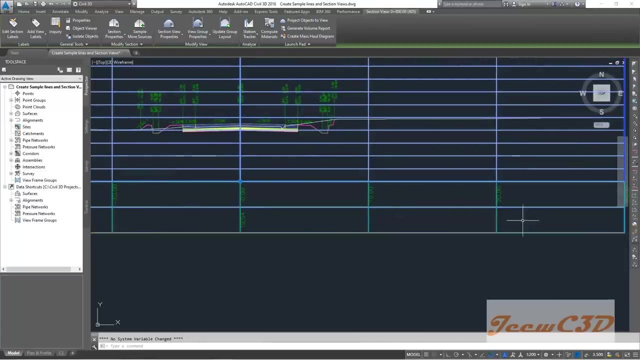 currently it looks like you don't have that data, so i have to modify the cross sections to do that. i select this first section. what i am doing is what i'm doing right now is we have the offset and existing elevation. this existing elevation band is not that clear for me, so what i am going to do is i select the cross section. 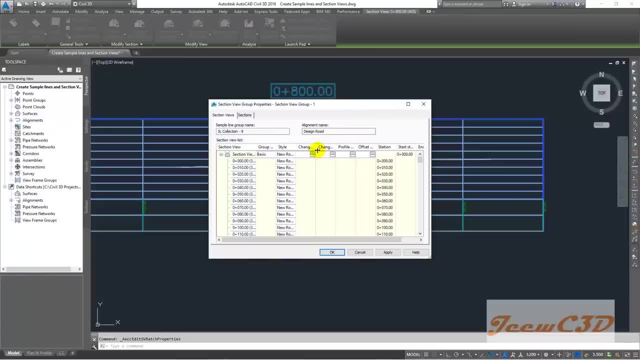 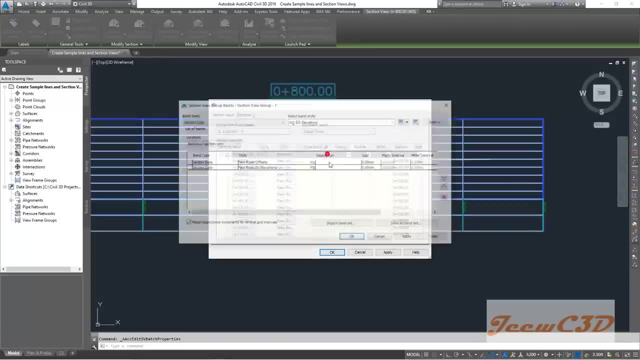 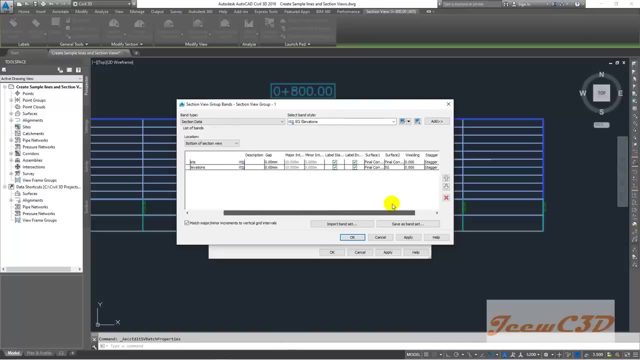 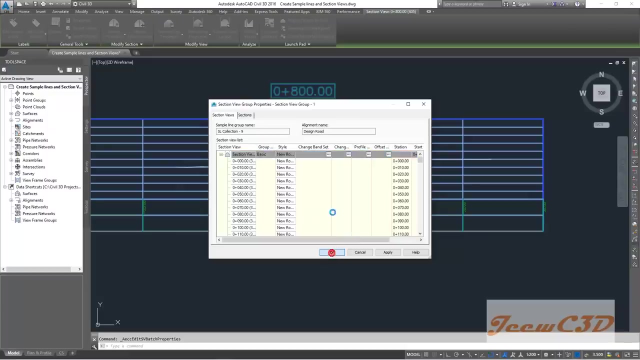 and go to view group properties, then i go to this, i will expand this tab to expand this column, then i go to change band set and i will see what has here. so should be. i think you have to use both these things and this one should be eg os. i think that is how correct that one. 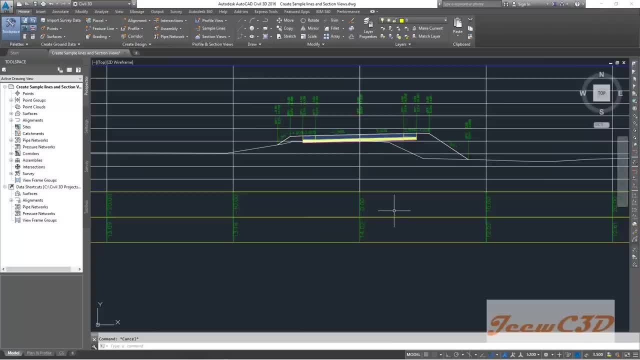 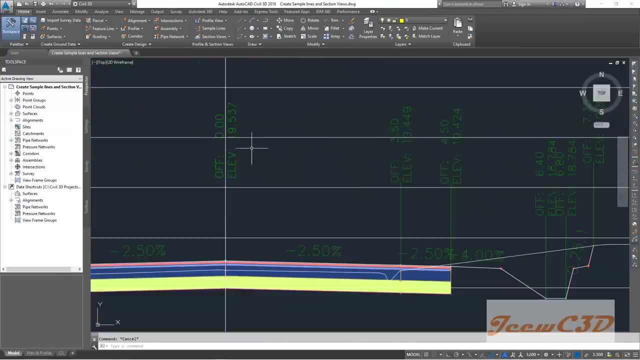 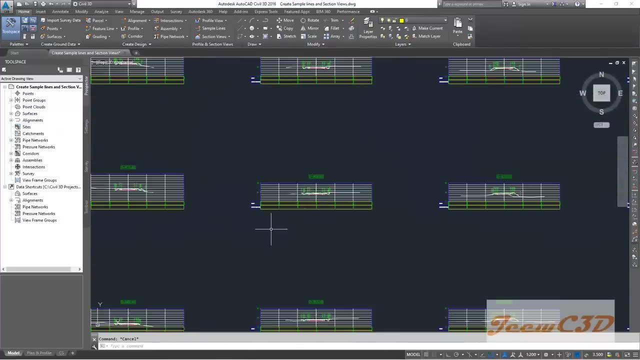 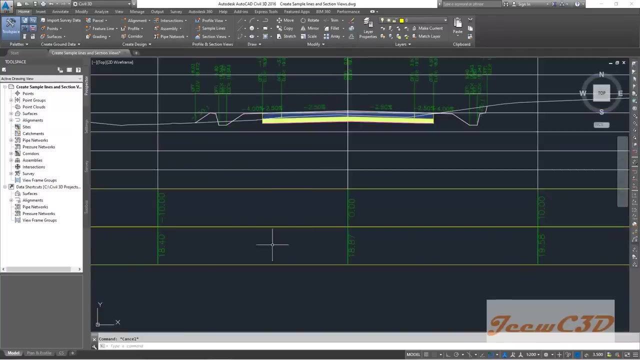 uh, we are getting some data in the cross sections. yes, now we are getting some data in it. times per section set: 10 meter intervals. existing ground data: 10 meter intervals. if you need, you can make more ground data here. so if you are getting corroborated, you will know how to do these things. 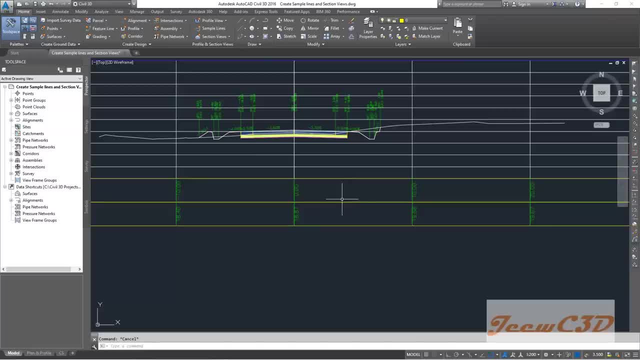 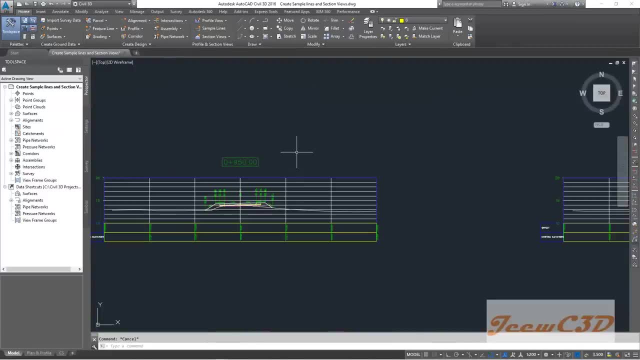 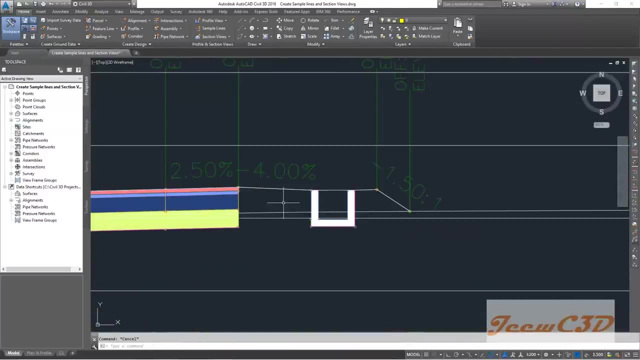 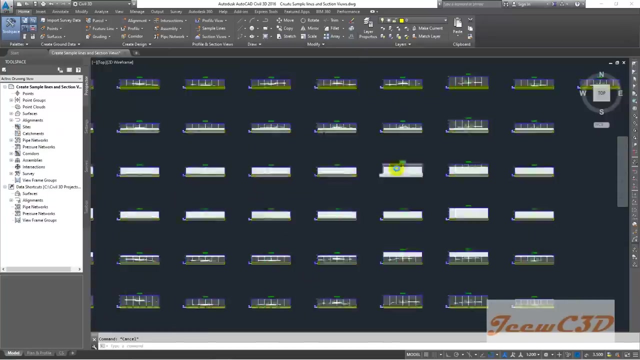 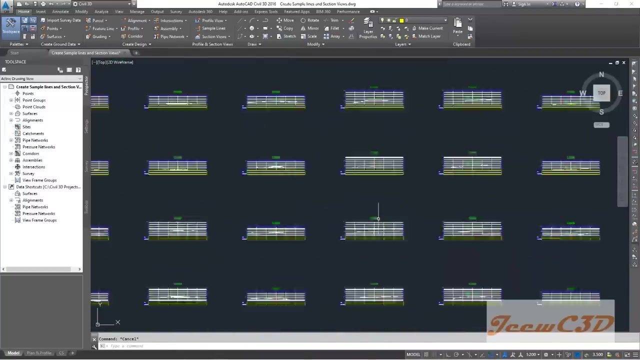 but at as a demonstration, i will strip to these simple things. so, if you can remember, at 960 we go to the concrete drains. you will see these concrete drains are now appearing from 960, then 1045, you will be having the 45 and 50. here you have this bridge assembly. 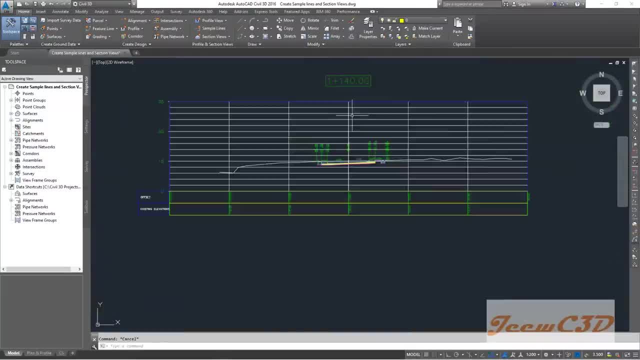 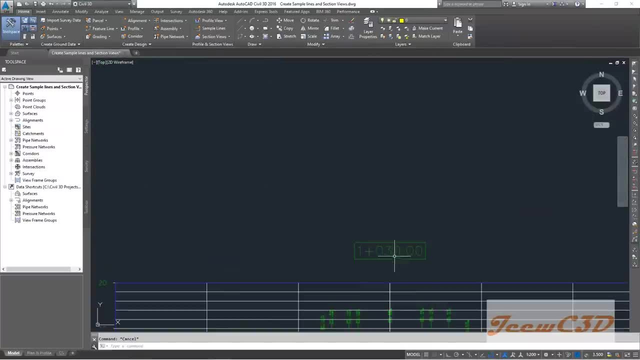 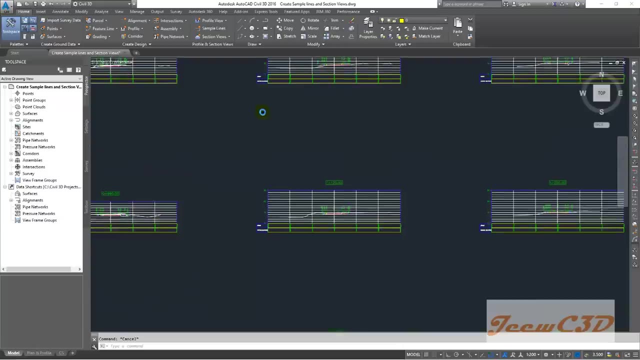 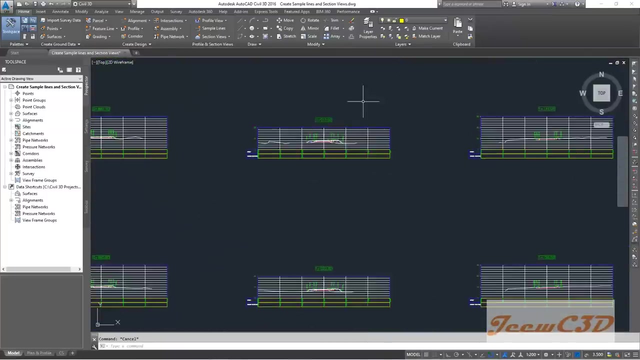 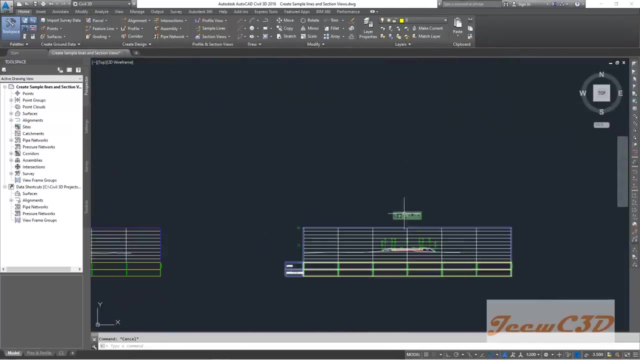 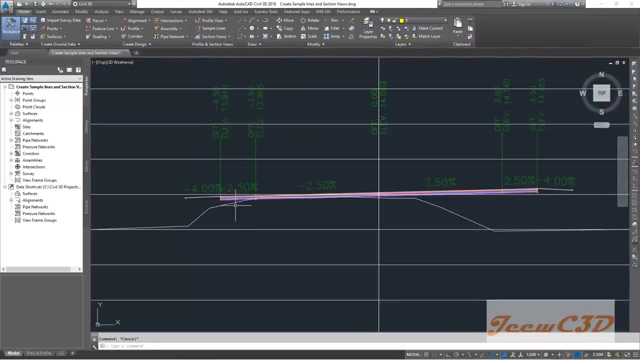 um, actually it seems like the bridges in these- not, it is 1050 actually here. it should be somewhere here. here you can see now they have the bridge assembly and also you can see we have only two layers here and also you can see you have the super elevation values in these. 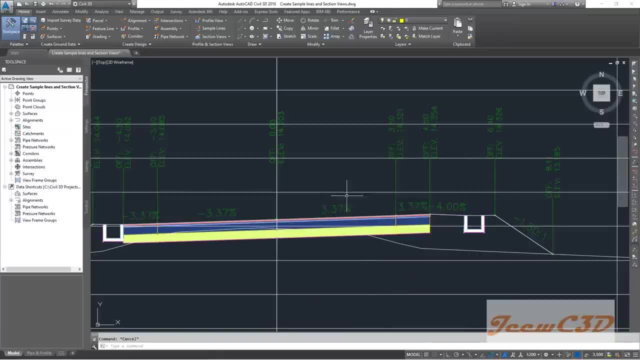 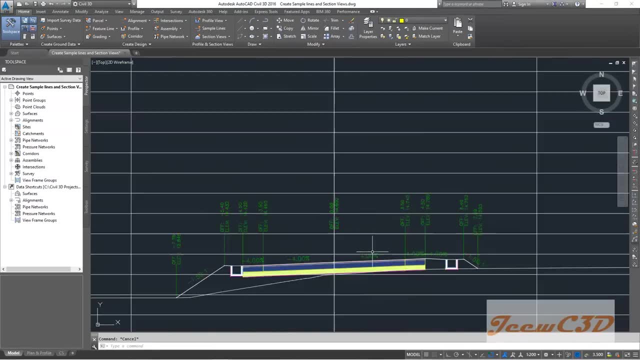 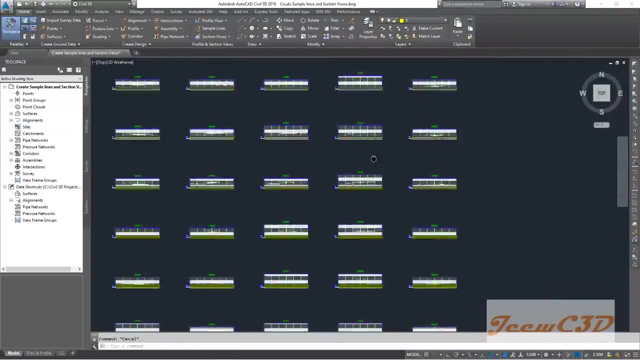 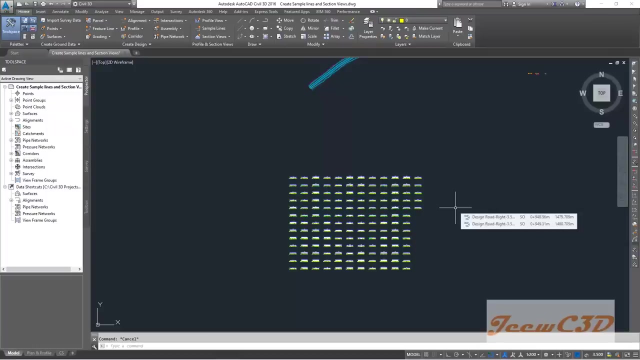 problems. also here you can see the super elevation transition sections where you can see the whole super sections. you see these values are applied to the corridor. you can see again the transition section. So those are the processions we created. So that is a brief introduction. 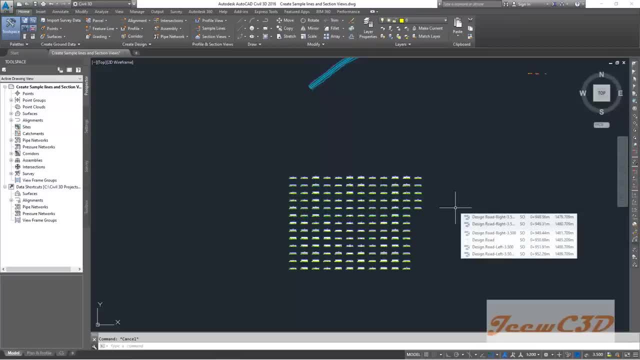 about creating or designing a horizontal alignment or designing a road design for a road project with Civil 3D. But this is a very simple introduction. So Civil 3D is much more than that And also, depending on this very limited time, so we can't go to more detail. So if you were in the classroom, 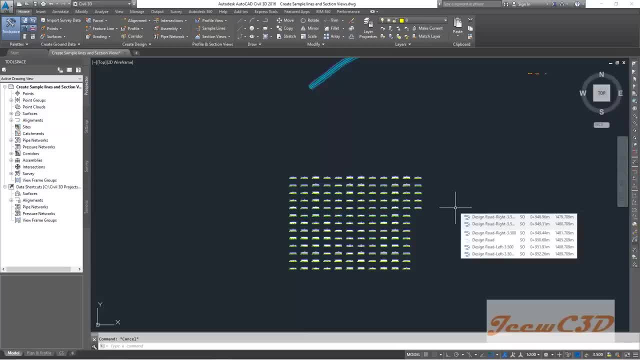 we will be only having one day to do all these things. So if it was so, sometimes we may not have time to do all these things. So I think we have done a lot of things with this, But there are a lot to be learned with Civil 3D. So if you are like to, or if you wish to, learn more Civil 3D, 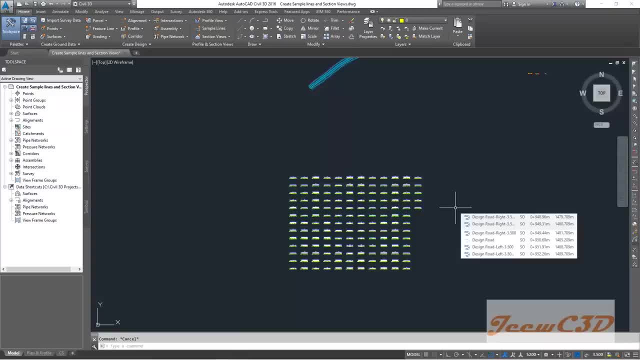 or if you are currently doing work with Civil 3D, you can refer some other tutorials, videos from YouTube or other internet sources to get more idea or understanding about Civil 3D. So that will conclude the part of Civil 3D And, again, it will conclude the highway design session for this CE760 subject.